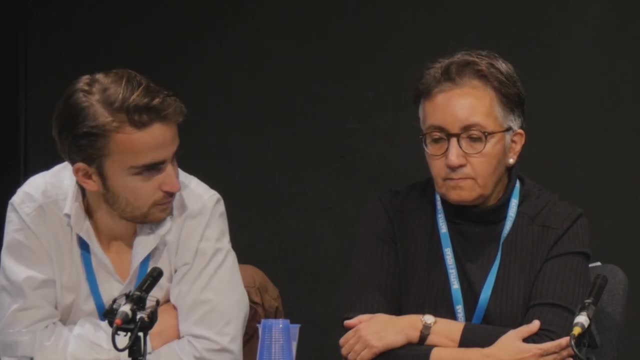 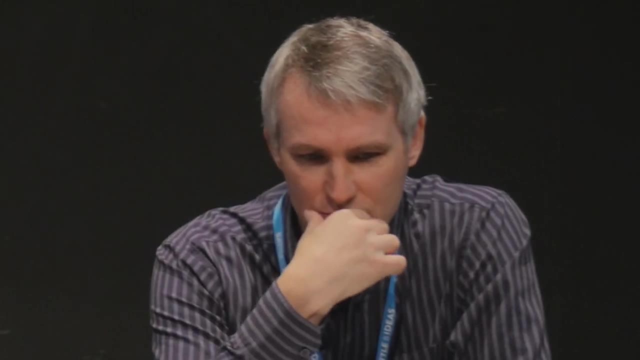 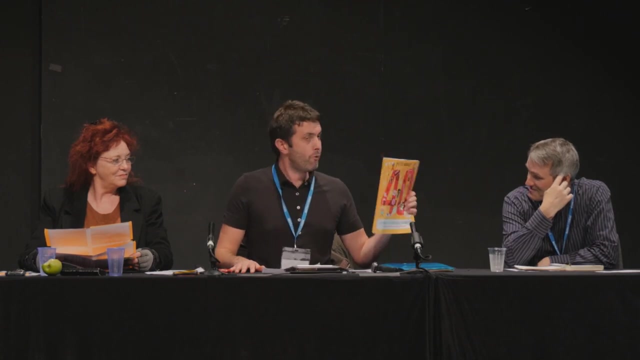 charity which explores how we might use philosophy within education. To my immediate left and speaking afterwards, is Peter Worley. He is the CEO of the Philosophy Foundation and the author of this publication. Lessons to Get Children Thinking. Forty lessons. Forty lessons to get children thinking. Speaking last: Alka Sagan. 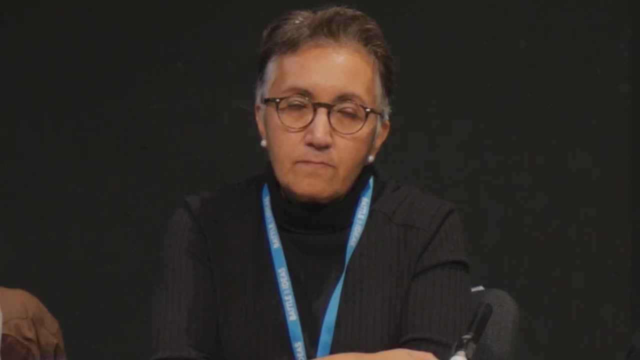 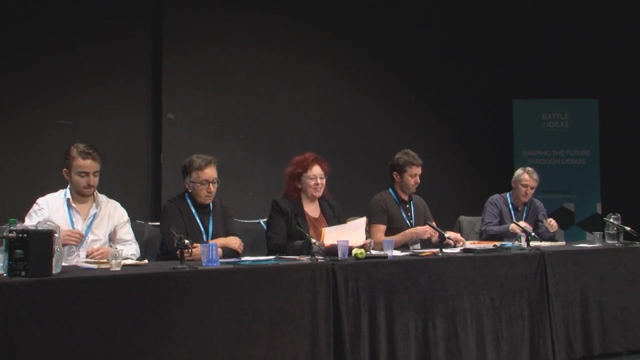 Thank you. And she's an English teacher and a PhD researcher at the University of Cambridge. So, Catherine, would you like to start us off? Thank you very much. Thank you for the introduction. So the question is: can children do philosophy? 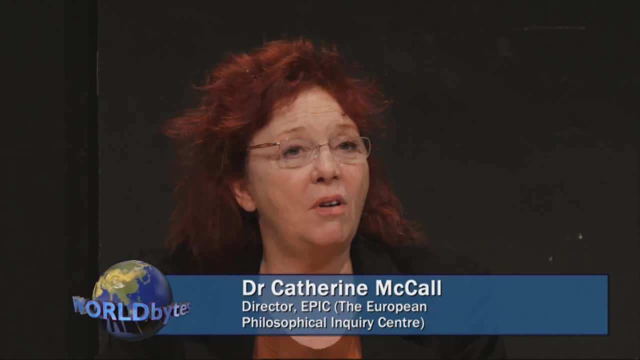 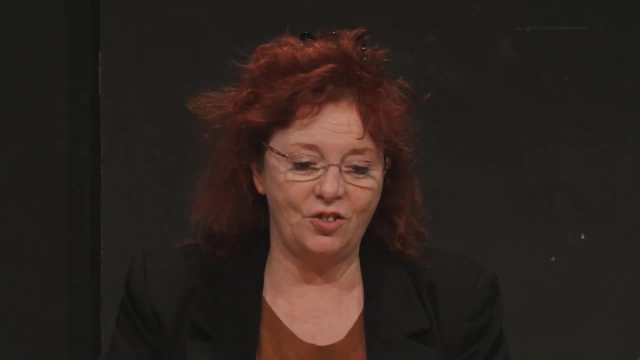 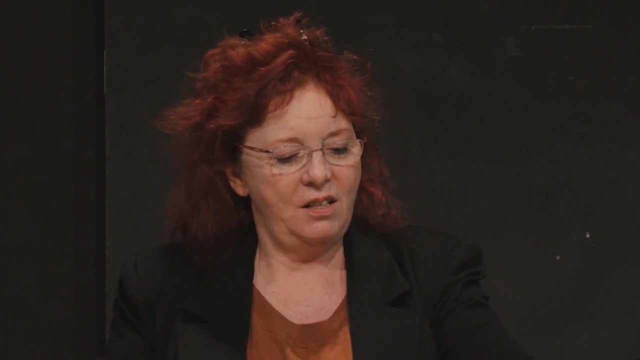 And being a philosopher myself, you won't be surprised that I'm going to say it depends on what we mean by can do, philosophy and children. So I'll come back to that later. but I'd like to start with putting a slightly different question to you: Can children do maths? So, if it means that they should understand algorithms? 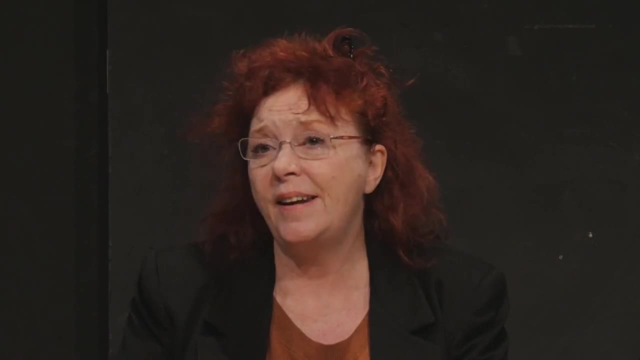 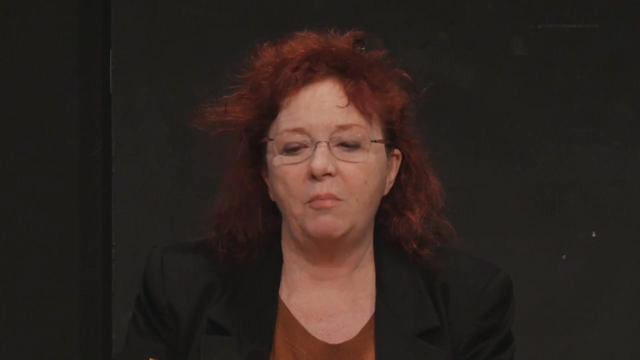 for solving linear and binomial systems of equations over finite fields. we might say no, However, if it means that, for example, my nine-year-old son won gold in the maths challenge. He's not understanding binomial systems, but he was using complex fractions which 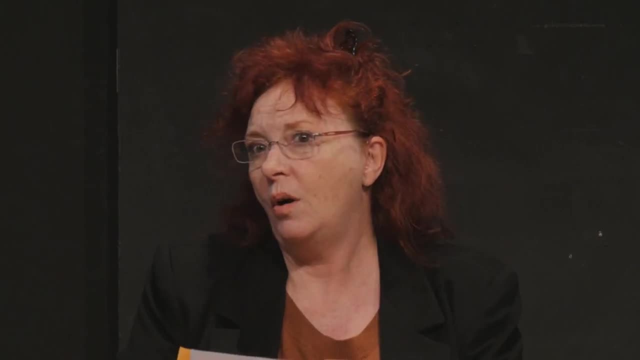 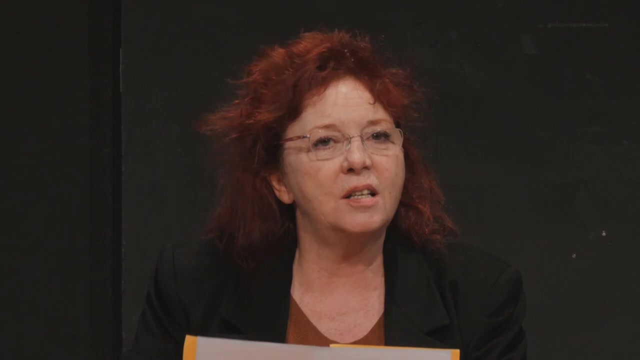 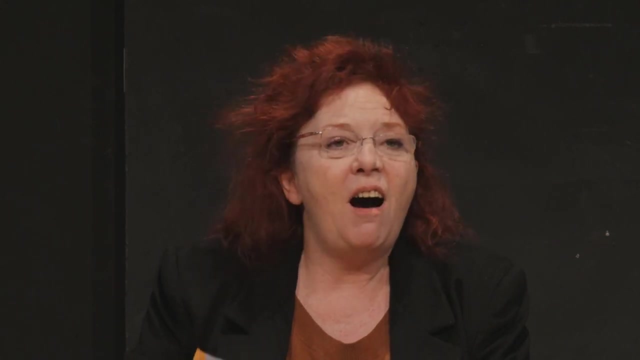 actually many of us, including me, can't use now as an adult. So if we say that children can do maths, it doesn't mean they're doing university-level maths. So I just wanted to get that point across. When we ask, can children do philosophy? again if it means, can they understand Kant's deconstruction. 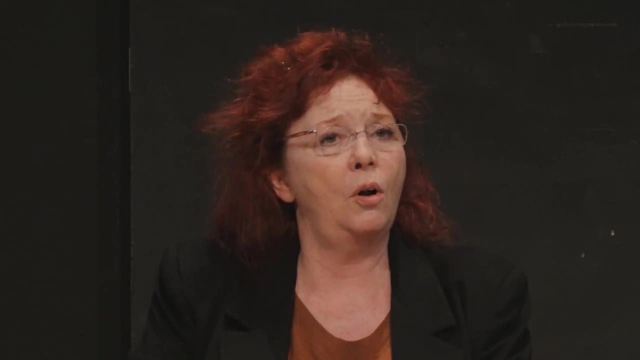 of the principle of sufficient reason, then probably no, although perhaps on A-level students might, But five-year-olds, eight-year-olds, probably not. But again, my five-year-old son was doing philosophy for children, COPI, the Community of Philosophical Inquiry, which 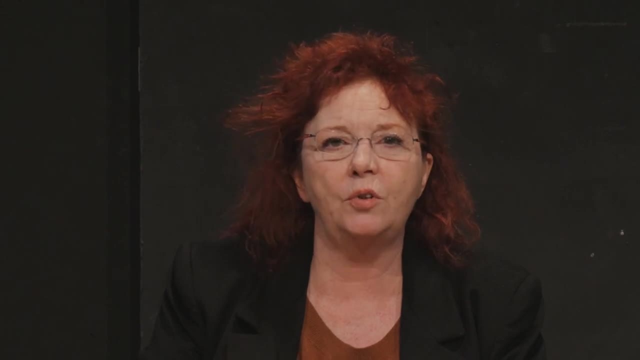 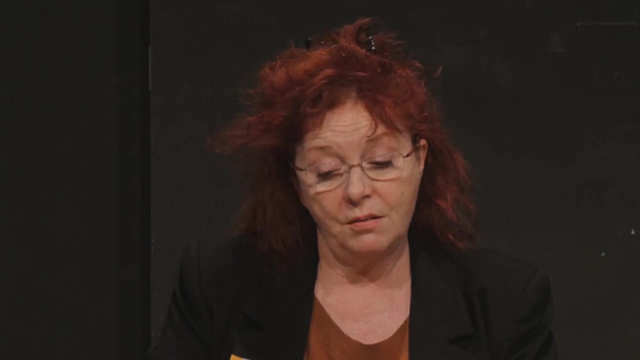 is the specific method that I developed for doing philosophy with groups and engaging in valid hypothetical reasoning about abstract concepts, For example in philosophy of mind, And I want to give you a little taste of the kind of thinking that even young children, five- and six-year-olds can do under certain circumstances. 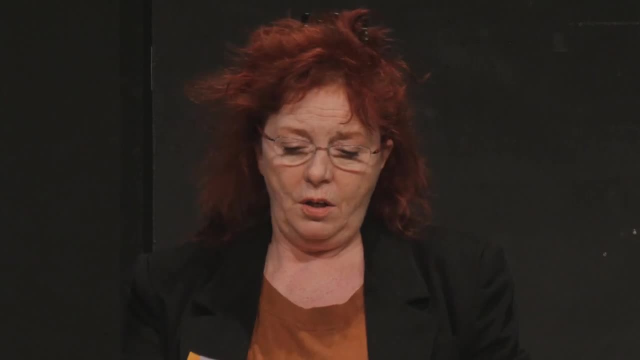 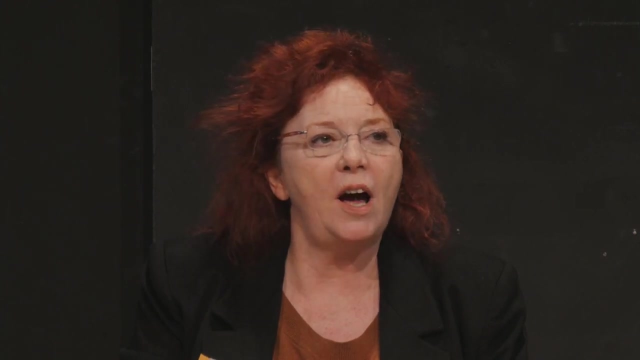 So we had a question. is dreaming and thinking the same? So this was a question being addressed by a class of five- and six-year-olds. That's the end of this dialogue, which, by the way, ran for an hour. And if anyone would. 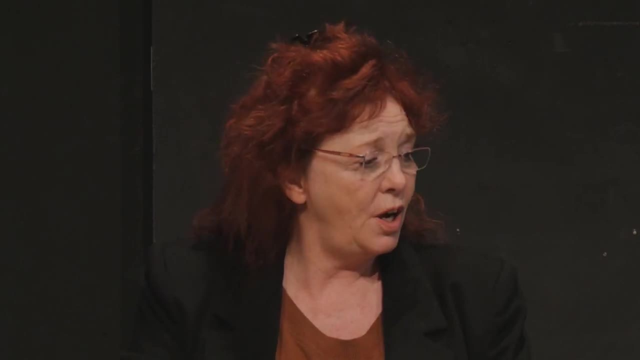 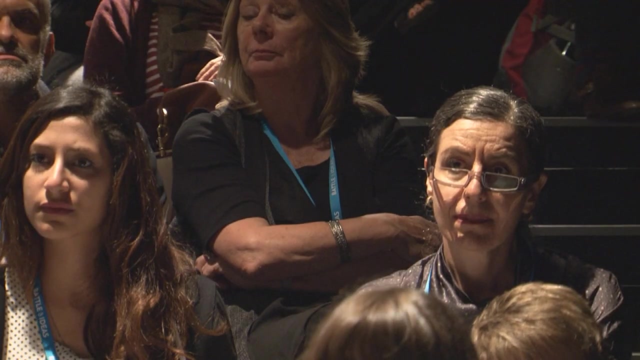 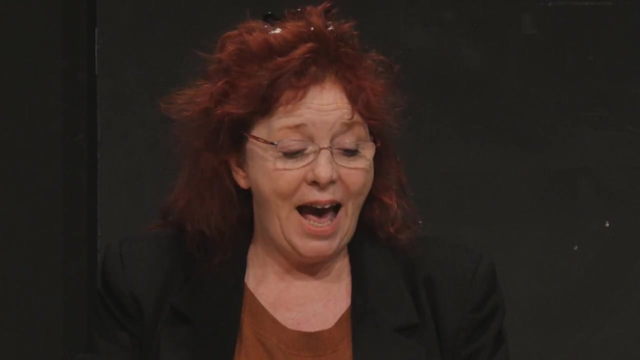 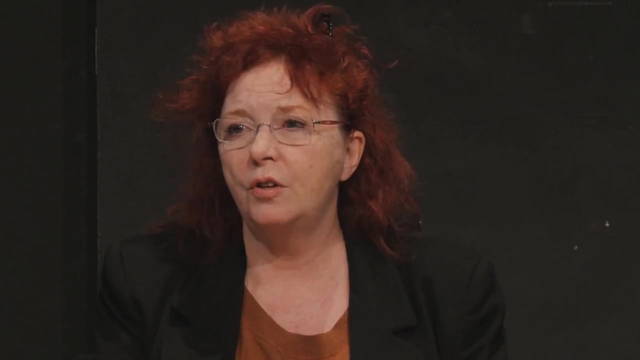 like to read the whole dialogue. it is in my book that Toby mentioned, called Transforming Thinking- Philosophical Inquiry. in the Primary and Secondary Classrooms One child comes in to say: if your dreams are in your imagination and your dreams are different to your thoughts. now he's rephrasing two other points two other children have made. 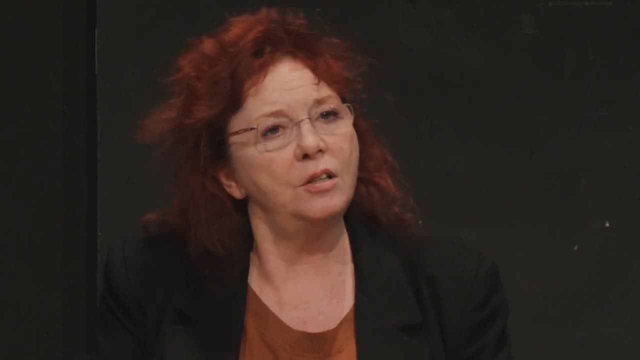 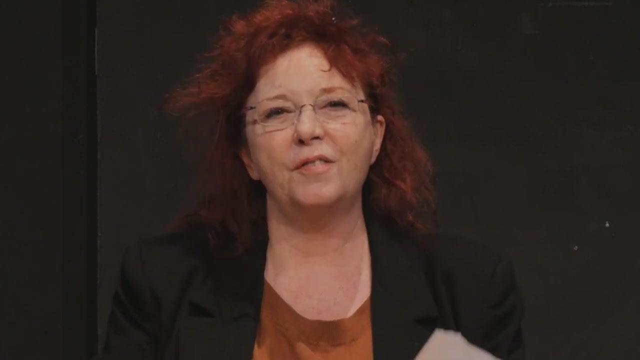 here, Then how can your thoughts be in your imagination? But you could think in your dream, in your imagination. So this is really complex thinking And it's hypothetical reasoning. It's putting together two different ideas that he's heard from other people and trying to put them under a kind 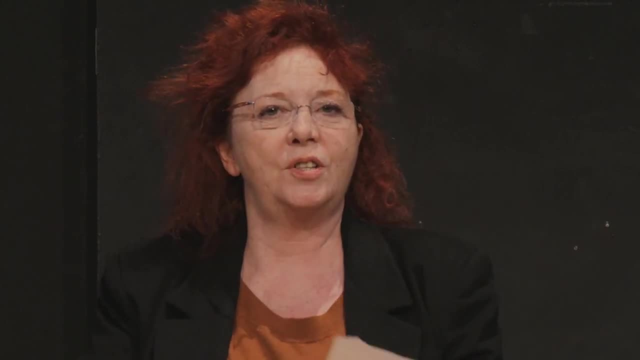 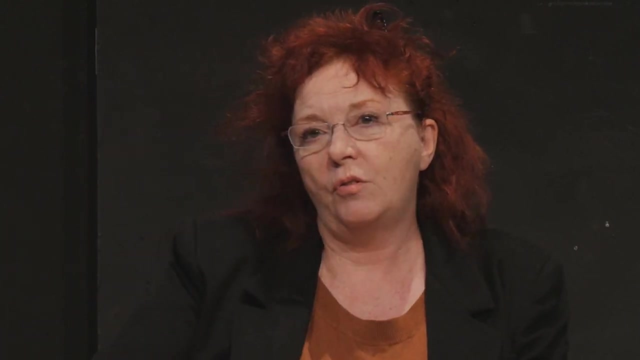 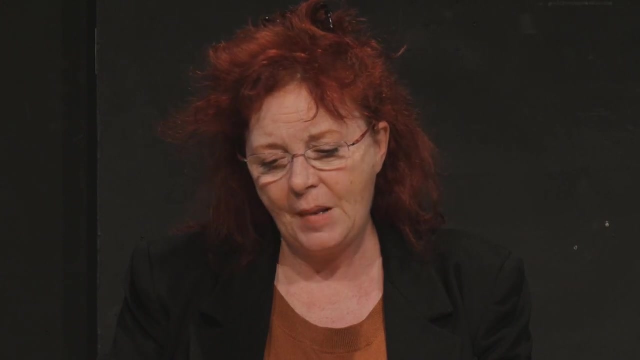 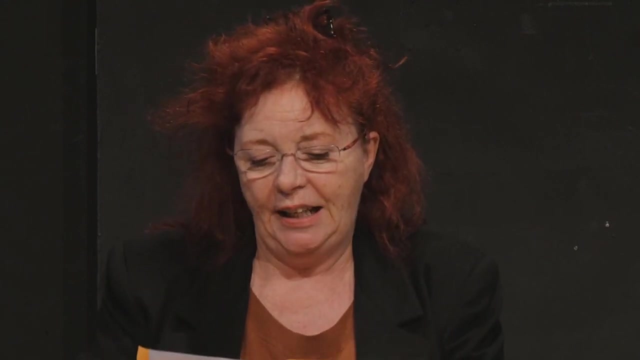 of set theory structure actually to resolve, to see if there's some way that you can get all these different concepts. So Mehmet, Team and話 as men together. And this is a five-year-old, So although he might not be reading Kant, I would say 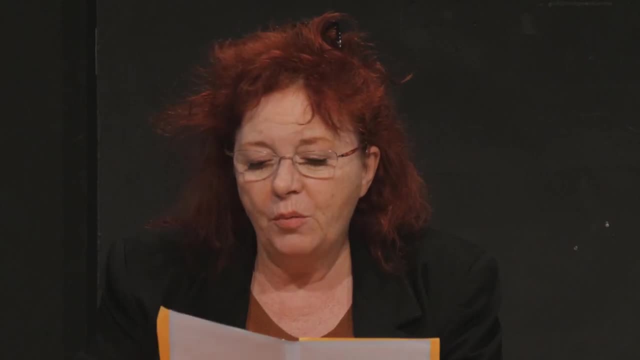 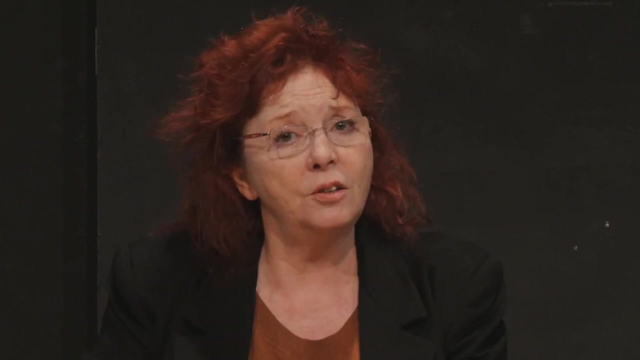 that is. So let's get back to what we mean by can children do in philosophy. With philosophy I would mean making arguments about philosophical topics, And if that's what we mean, way, can children do it. so these are. 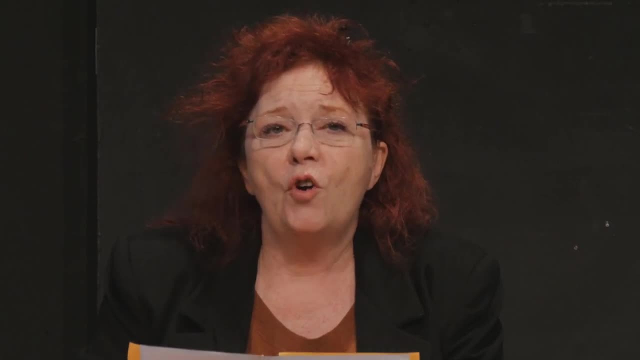 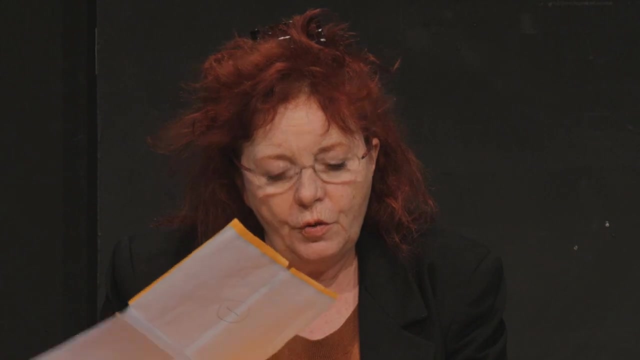 two things Again. I would refer you to the Battle of Ideas website. Under this session there is actually a link to a video where you will see six-year-olds philosophising using this coping method. But not all philosophy for children or P4C is the same. 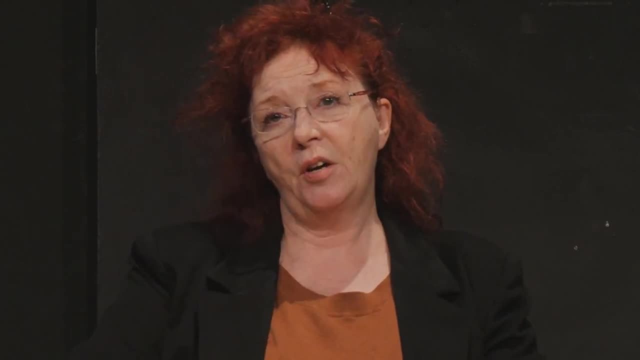 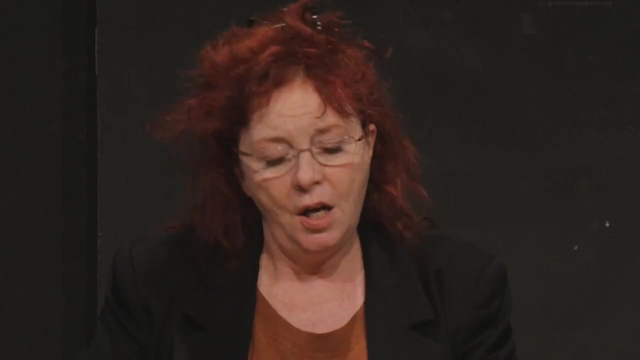 Sharing opinions and sharing experiences, in my view, is not philosophy. It's very nice discussion, it can be very good for children, but it isn't philosophy. When I say children can do philosophy, I'm certainly talking about the work that I've done. 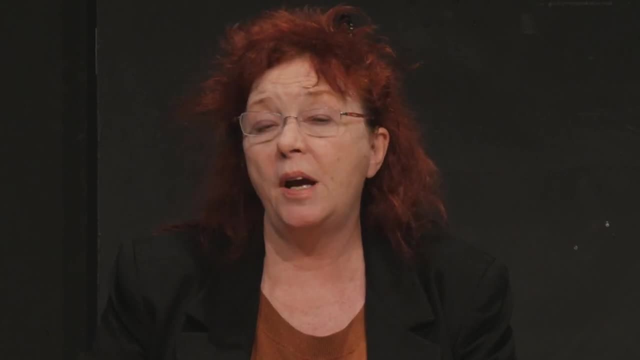 which involves them putting forward ideas which they may or may not agree with themselves. making a case, making an argument, They have to give reasons, they have to make arguments And not necessarily coming to an conclusion. in fact, the work that I do with little children and adults and business leaders and professors- 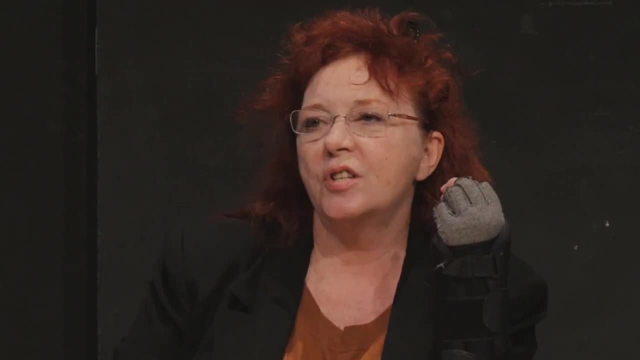 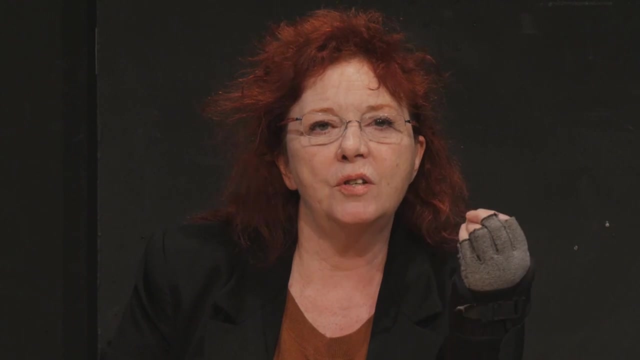 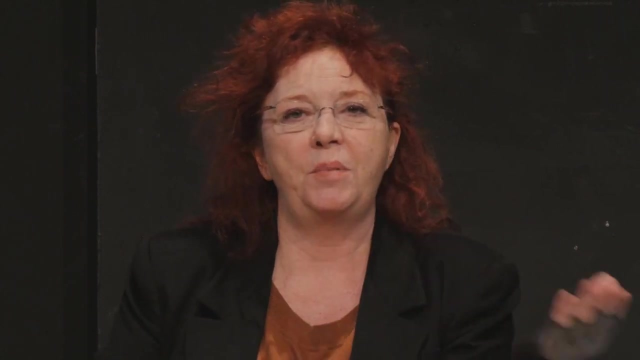 encourages difference, encourages disagreement. I'm looking to pull out different ideas because the more difference there is, the more rich the dialogue and the more you're likely to discover and create. You don't learn anything by listening to people who think exactly the same way as you do. 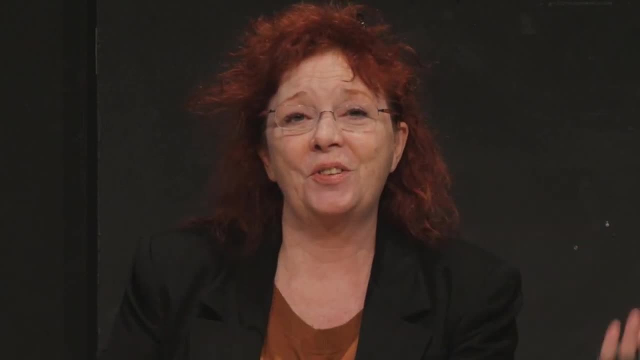 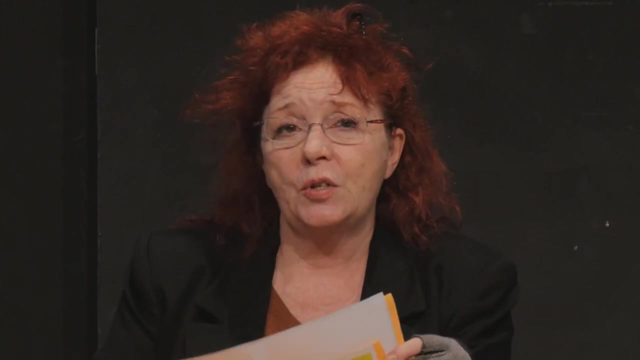 It's cosy, it's nice to share your opinions with like-minded people, but that isn't doing philosophy, in my view. So children can do philosophy, but it takes a very special environment for them to do that. So what do we mean by children? Well, we generally mean an age range, so that goes, say, from 3 or 4 up to, I would say, about 13,, 14-ish, I think. beyond that they're really teenagers, not really children. but it's a bit fuzzy. 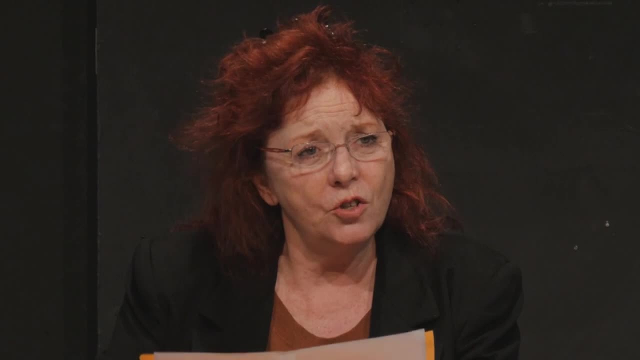 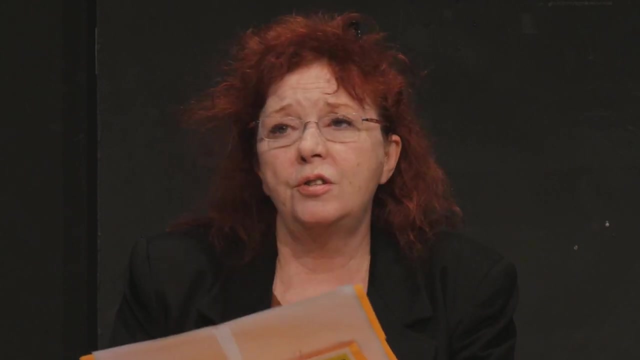 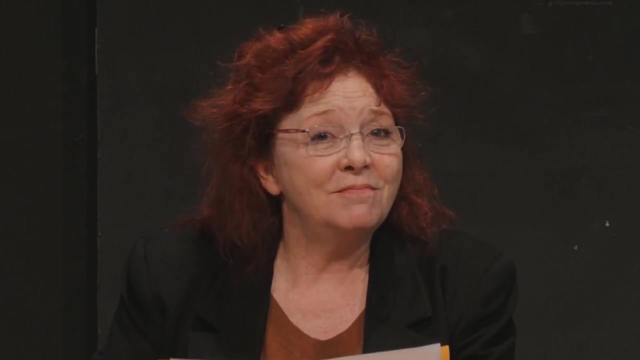 In the question: can children do philosophy? does this mean all children? Can all children do philosophy? Well, not all children are the same. Can all children do maths? If you do maths badly or wrongly, are you still doing maths? It's a question somebody might be able to answer for me. 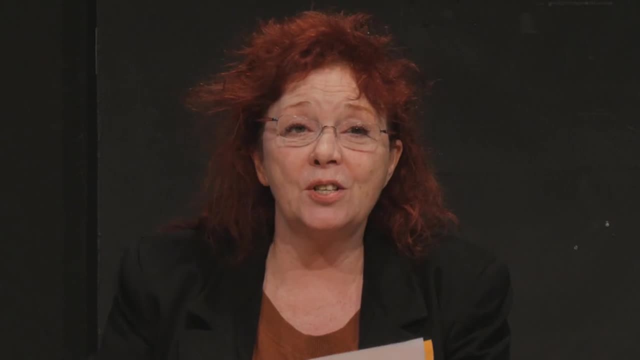 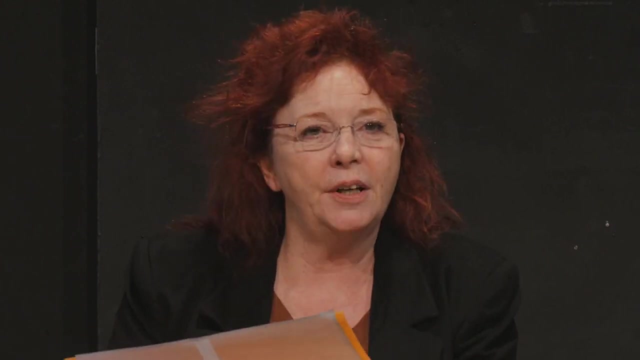 So if you do philosophy badly or wrongly, are you still doing philosophy? I think you probably are. you're just doing it poorly, like you could do maths poorly or art poorly. If you do art poorly and really enjoy it, it's still doing philosophy. 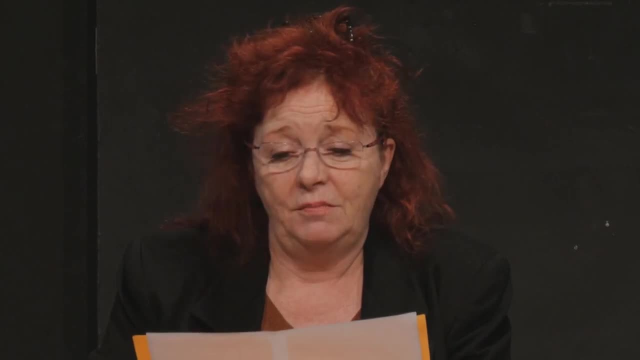 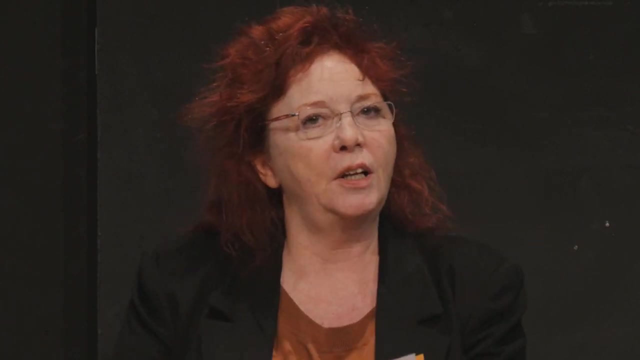 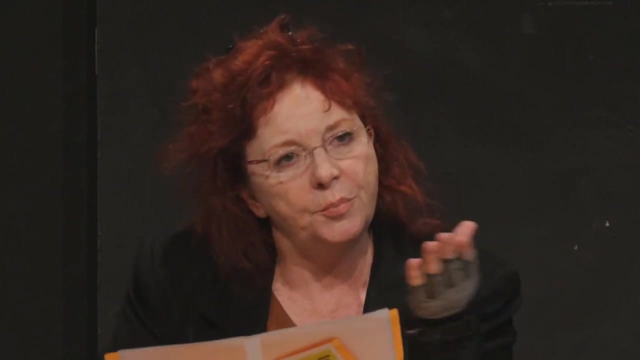 Again, sharing your feelings is not philosophising, It's not doing it badly, it is simply not doing it at all Your feelings, except for examining the nature, at an ontological level, of what feelings are, that would be philosophical. but telling people how you feel is nothing to do with philosophy. 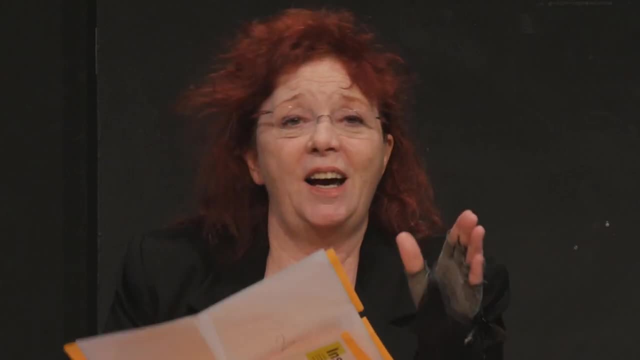 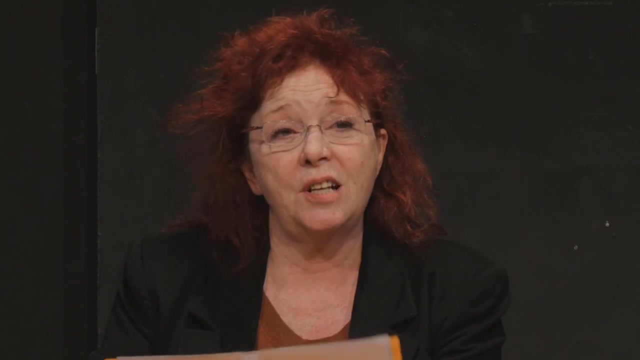 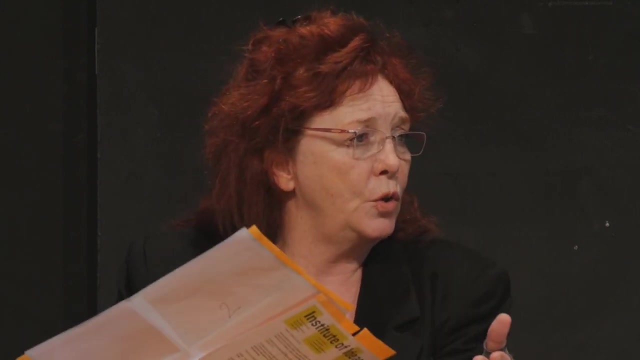 So what I mean by philosophy, I have to say, is what professional philosophers do in more or less universities, because that's where you find them. I really don't mean one's personal philosophy of life, or so-called Eastern philosophy, or mystical ideas. 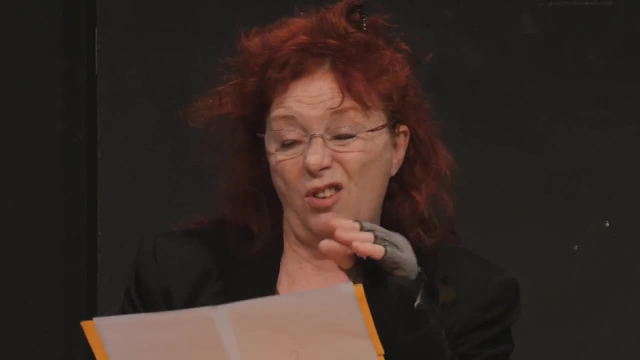 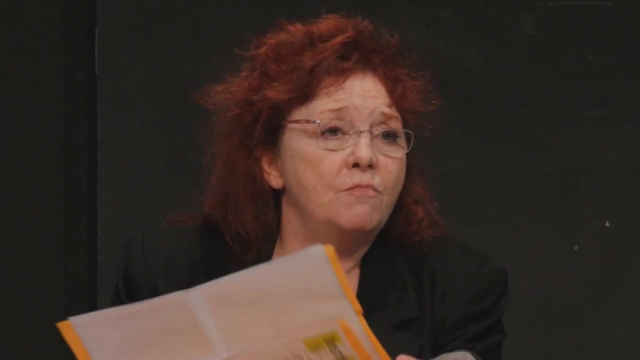 So it's a very probably Western- I would not say particularly male- but it's a concept of philosophy that is the one that's been running for 2,000 years, since Plato. So we come to can. Can children do philosophy? 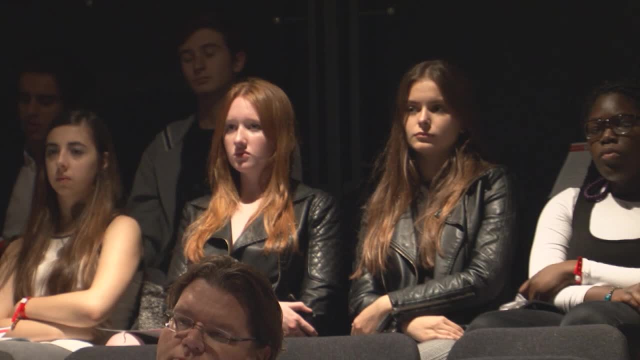 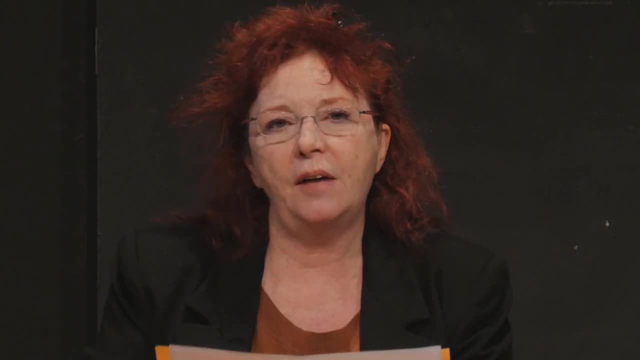 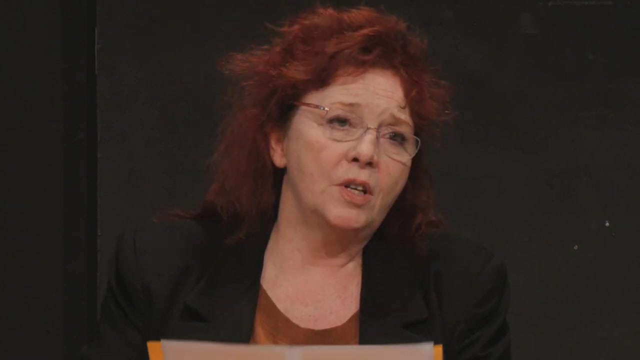 It depends. Does can mean: do they have the capacity? Are they able to? Are they somehow inhibited from being able to because they haven't reached the right stage of cognitive development? I would say no, And again, I argue this quite extensively in my book. 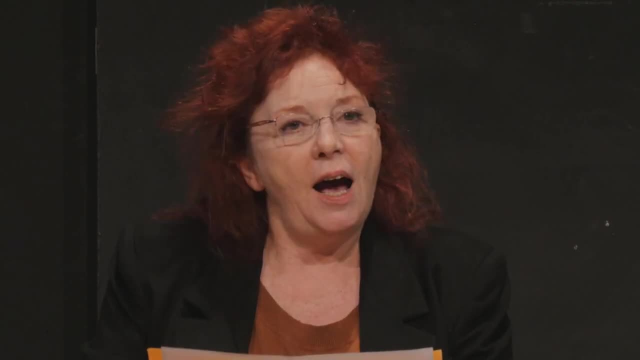 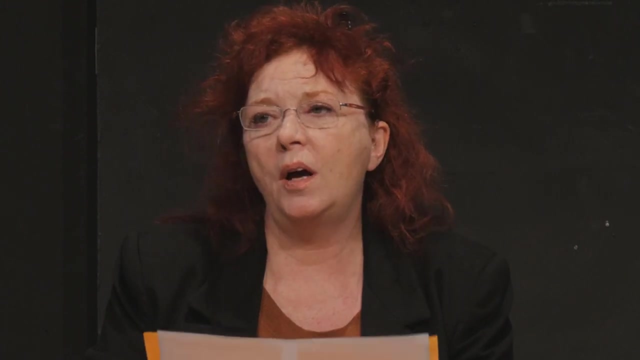 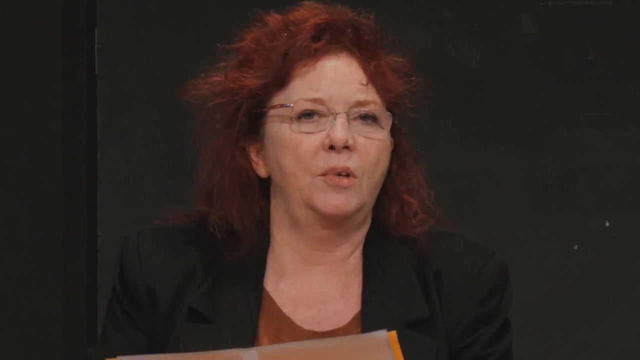 Transforming Thinking. I think they have the capacity. I think stage theory as outlined by Piaget and all his followers that has been so influential in education, is not correct. It's an analogy to physical development that was very neat and handy and was verified over and over. 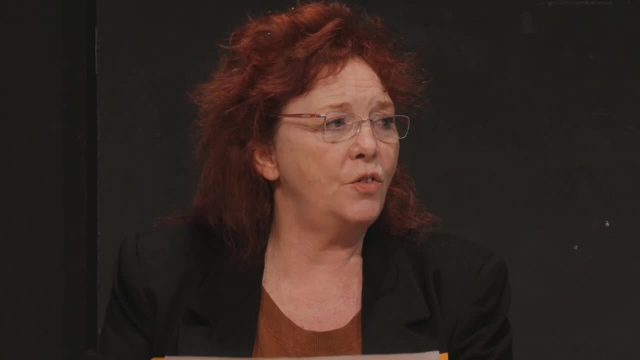 But, as you may know, in empirical psychology that's part of the methodology- is to verify, And you're allowed to discard results that falsify. That's your hypothesis. So I've always questioned whether Piagetian stage theory was correct. 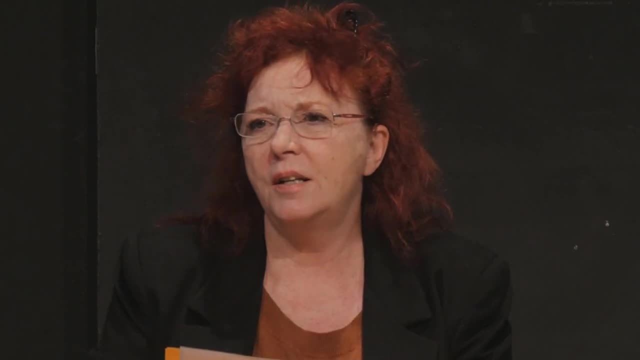 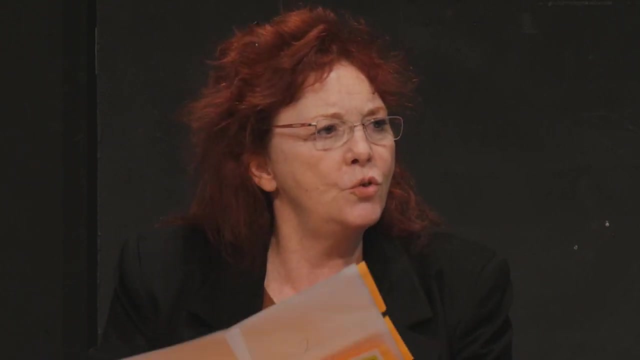 because it seemed to me quite obvious. if you talk to a toddler and say if you go out without your coat you'll get cold, you're using hypothetical reasoning about a future state of affairs which is not in the present. It's not concrete, It's not here. 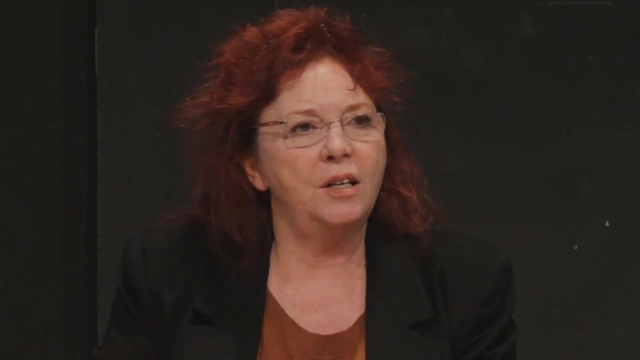 So they are obviously capable of understanding abstract ideas and hypotheticals And doing simple, simple but logical operations. So I would say that all children have the capacity, just as all children have the capacity to swim. They have within themselves that they would be able to. 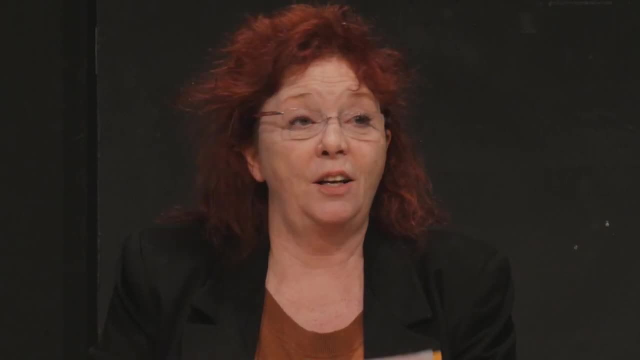 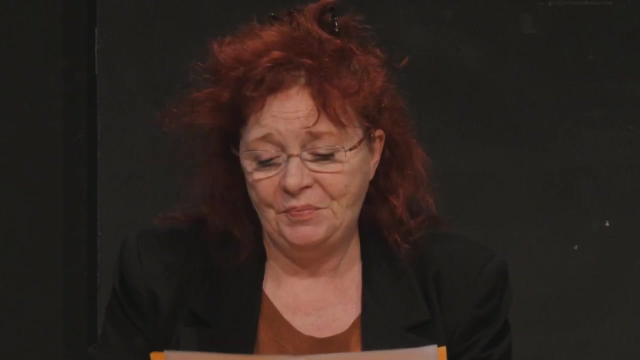 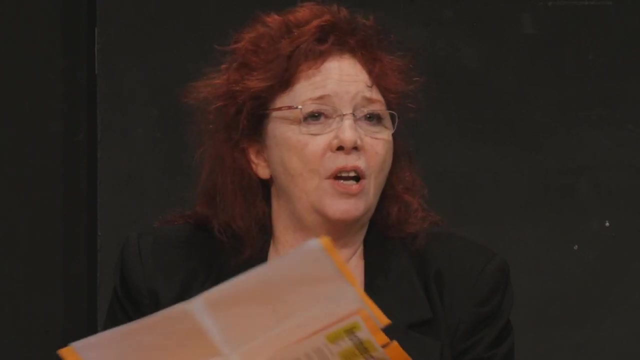 But they don't just swim. They have to be in the environment that encourages swimming, that is water, And they really have to learn how to swim. And it's the same with doing philosophy or really doing almost anything: The children have to be in an environment. 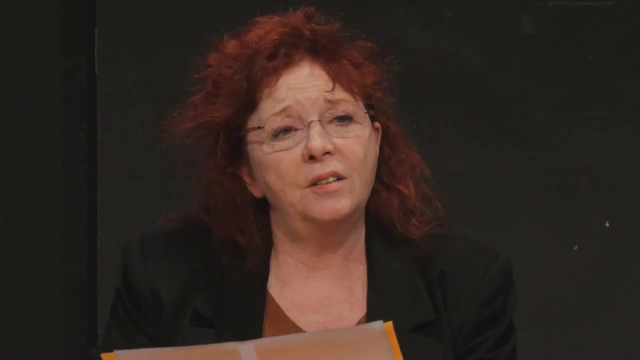 where they actually learn how to reason philosophically, and they have to have practice at it. It's not something you will find them doing naturally in the playground. They will wonder. they will come up with words that are philosophical sounding, but really to be doing philosophy is. 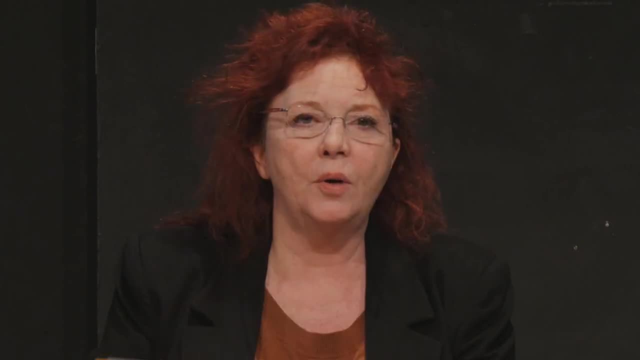 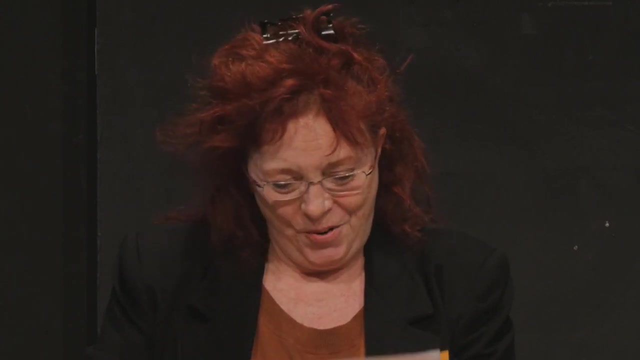 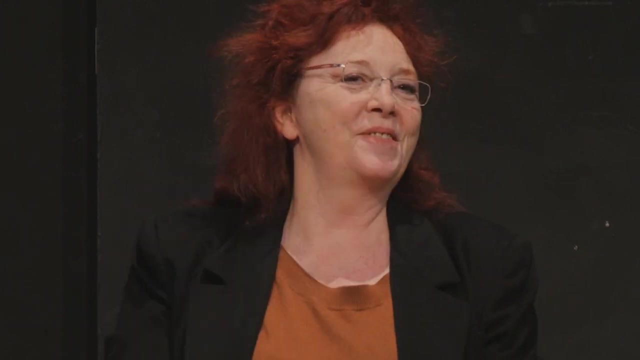 as I say, to be making a case, to be arguing about abstract ideas that are not necessarily your opinions. In my view, So, and there's another meaning of can, and I'm actually segwaying and squeezing something else into this talk here. 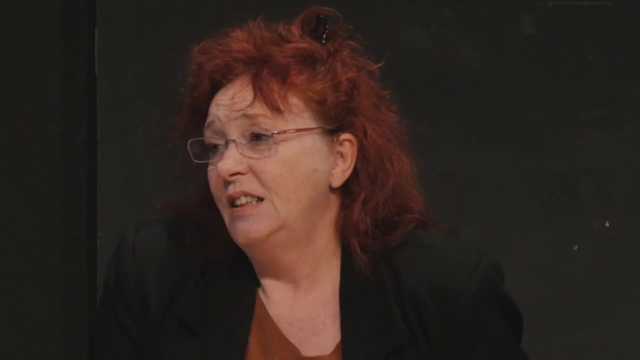 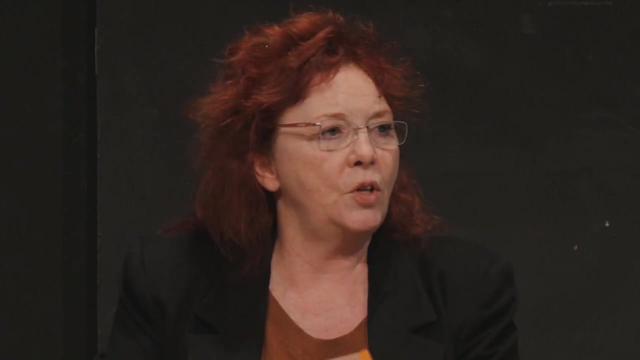 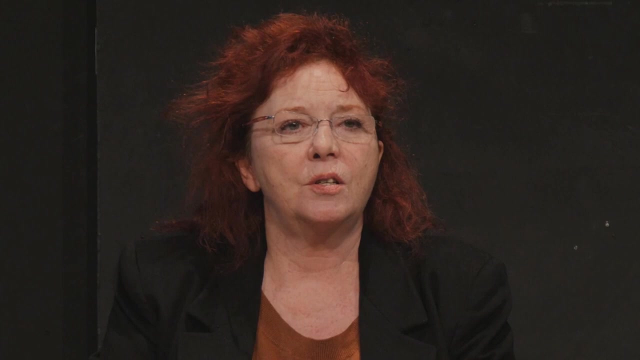 quite deliberately, which is: may May they do philosophy. Well, there are critics who think that, while it's possible for them to do it, it's not a good idea because it leads them to question authority. And to do it in schools means disrupting. 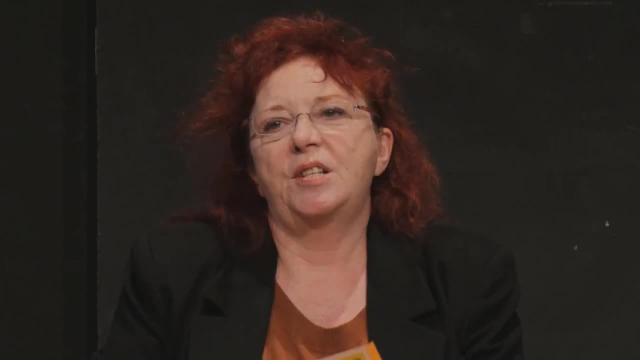 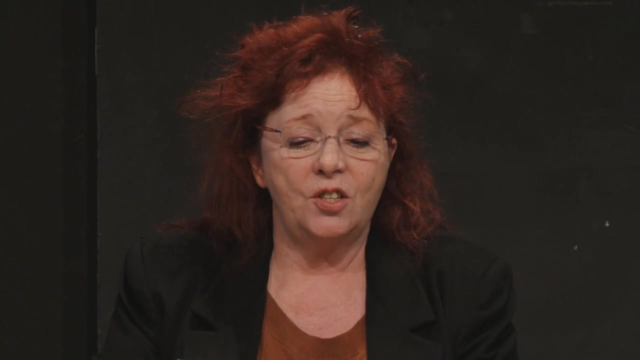 the the running of the school. I would say that's an empirical question that somebody should research. However, my argument is that certainly the kind of philosophy that we do in EPIC is essential for developing a respect and engaging in free speech, Because within this kind of philosophical dialogue, 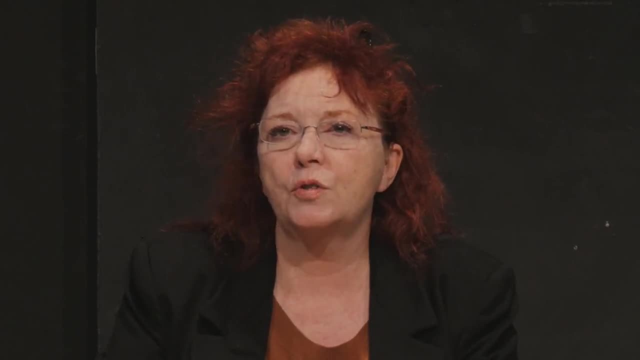 you can put forward anything that the, that the dialogue calls for absolutely anything. You're free from having to put forward your own opinions. It's not about your opinions. It's not even about your thinking. I use the thinking of participants. 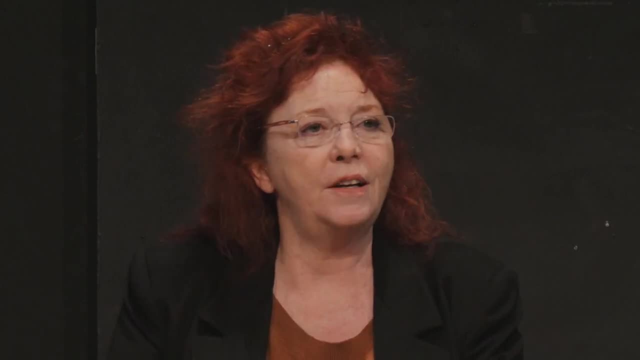 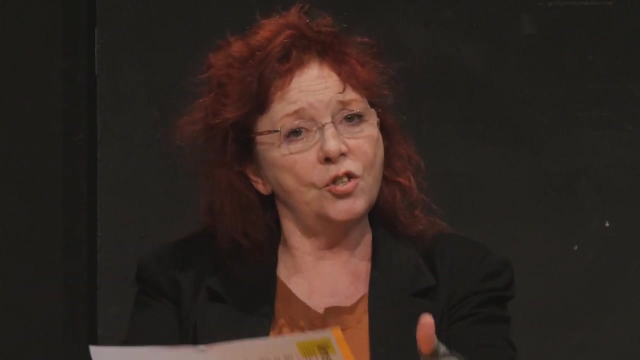 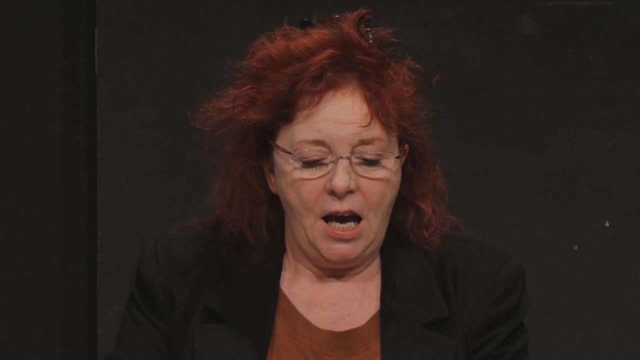 adults or children to create the dialogue, but I'm not investigating your personal thinking. Whether you believe this or don't believe this is irrelevant to the investigation of the topic. So it's excuse me. so it's not an opinion and everything can be examined. 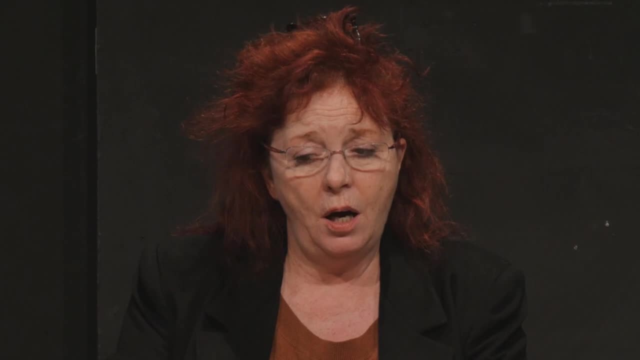 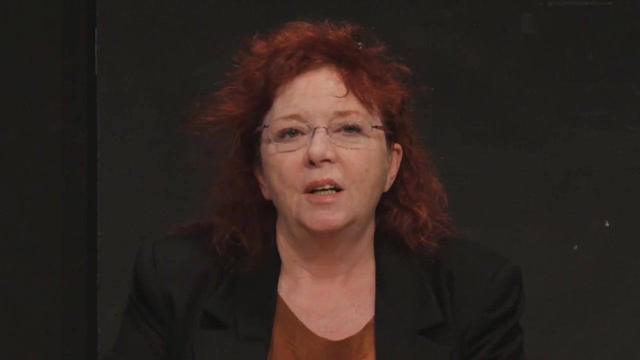 So, for example, you can examine whether FGM is a good or a bad thing. female genital mutilation: This is not outlawed. You can actually- really you can- examine everything, So I'll give you an idea of how that might go. 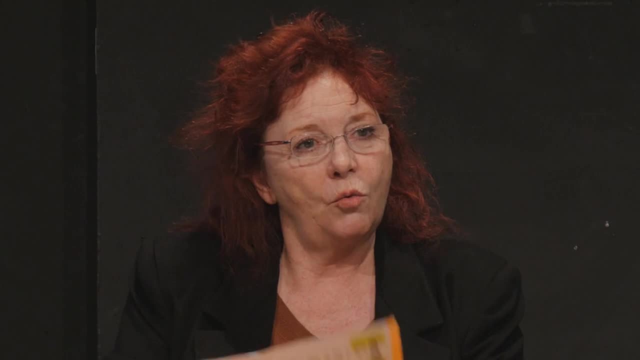 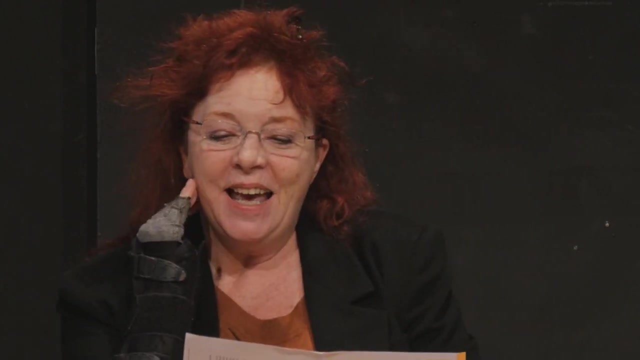 Somebody will say it's a bad thing, and then they have to give a reason why it's a bad thing. because I have to wind up, I'll drop these parts like that, Sorry. Yeah, It mutilates the physical body. So. 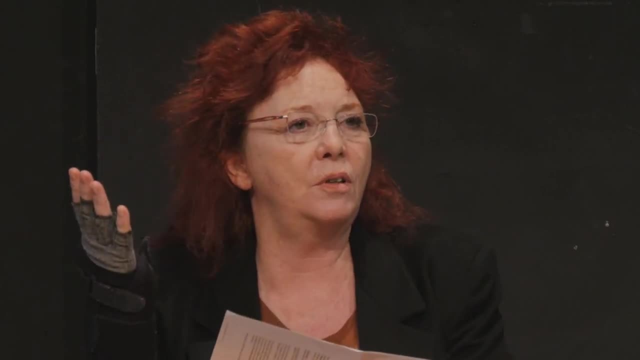 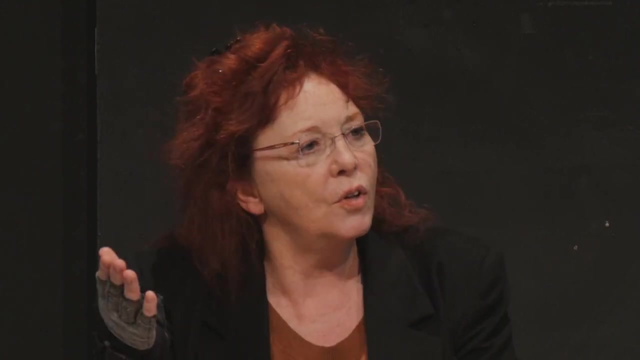 a counter argument. I disagree, because piercing your ears mutilates and that's not bad. Okay, then it's a bad thing because it causes pain. Someone else disagrees. well, but having a tooth out causes pain, So that doesn't make it bad. 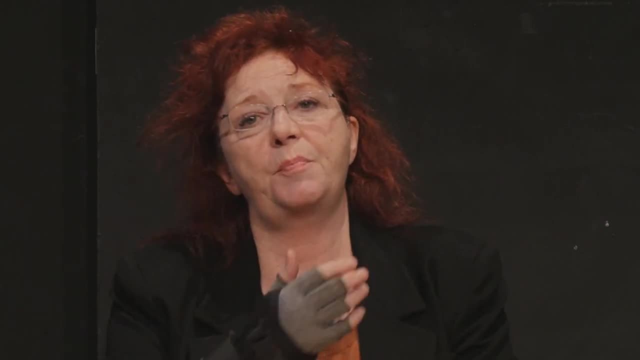 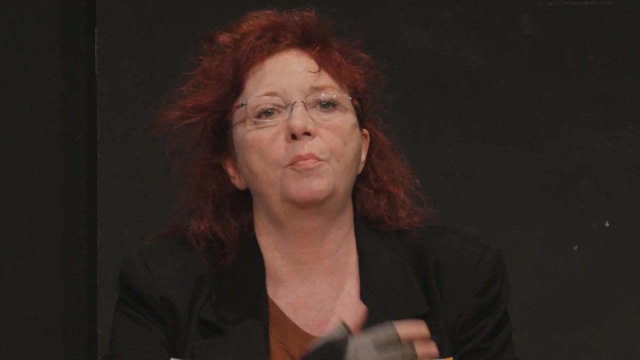 So you have to go deeper and somebody then says, yes, but it's pain for a good benefit having a tooth out, Whereas FGM is not for a good benefit, someone else will argue. but it is for a good benefit because it does make you. 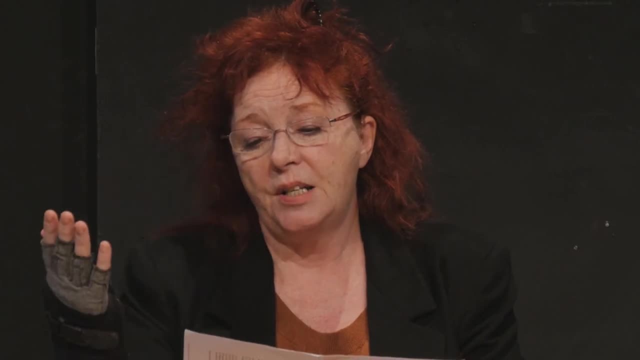 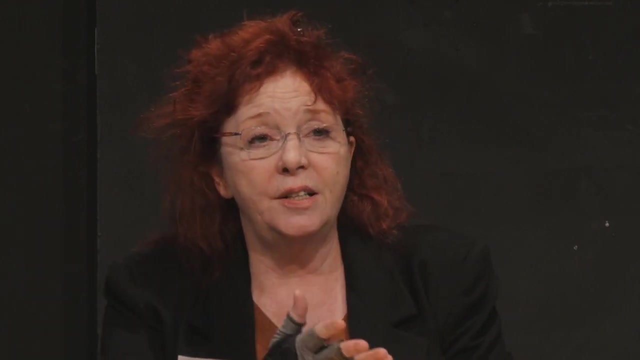 blah, blah, blah, more socially acceptable. Then finally, somebody says it's bad because you're mutilating somebody against their will. So the underlying philosophical idea here is that it's bad because it's against your will. Then the child is always going to say: 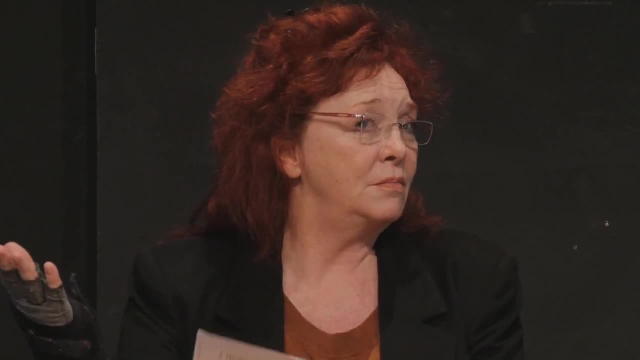 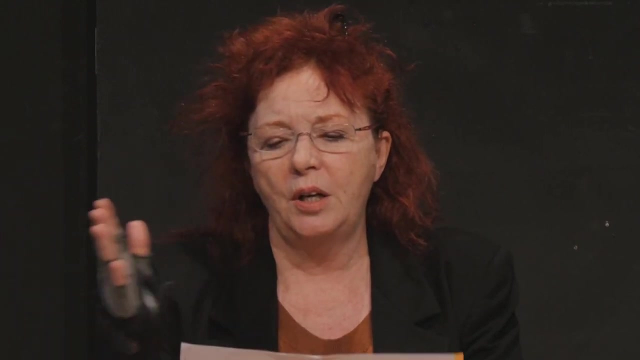 yes, but I'm going to school against my will. Is that bad? So what you do? this is a very, very rough sketch. is the person who's chairing it- like myself or someone I've trained- is digging for the underlying philosophical assumption? 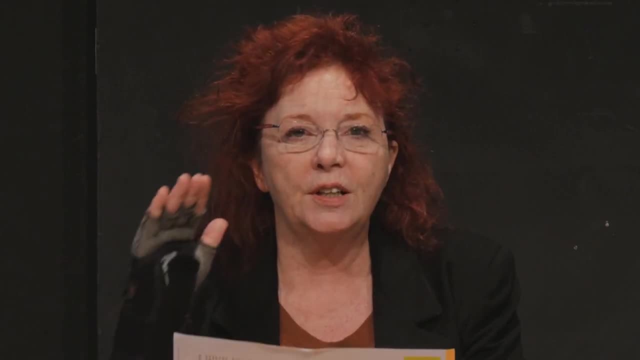 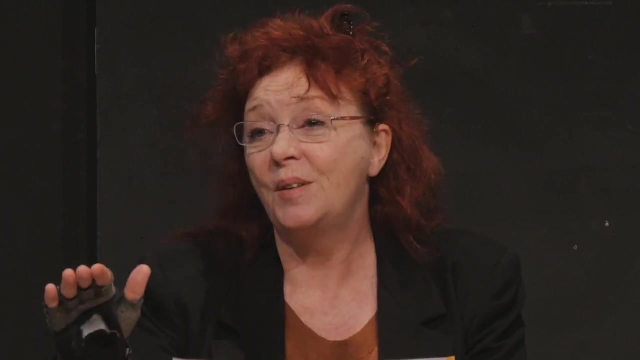 Why is this bad? So it's perfectly fine, within a COPY session, for children or adults to be putting forward the arguments as to why it's good. In fact it's necessary. We have to hear it. There will be a chance to come back. 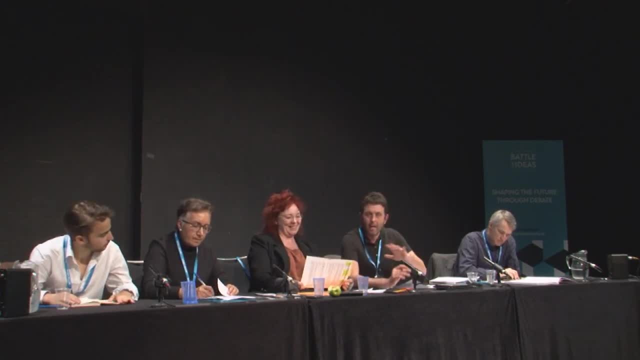 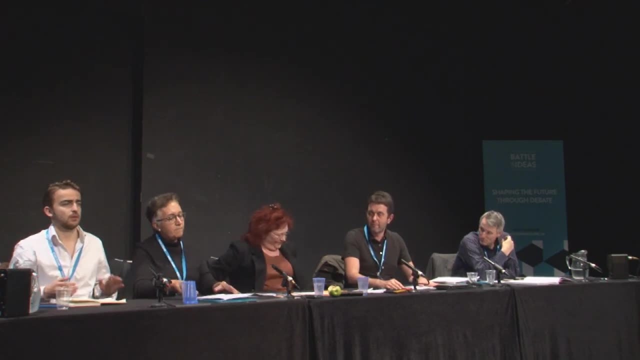 and add more detail, I promise, Just so we can get everybody in and then get out to the floor. Sorry, Catherine. So I'll just finish by saying yes, they can, and I think they should. Excellent, Thank you very much. 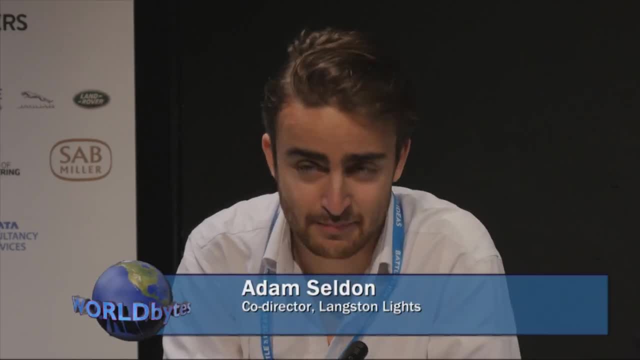 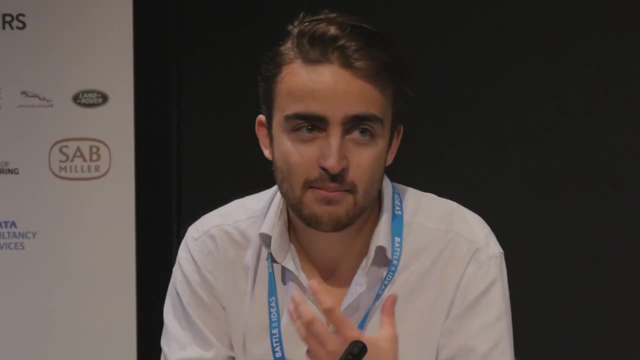 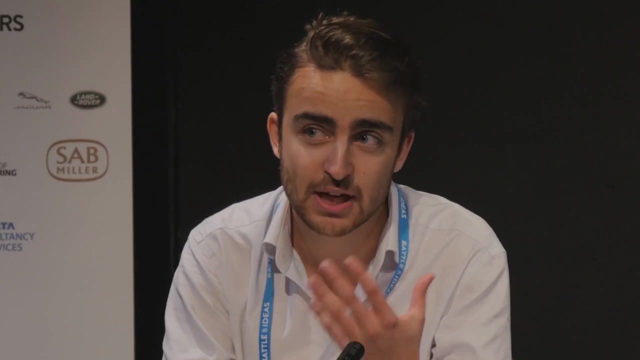 Ladies and gentlemen, thank you for having me here. I must confess, I do feel like something of an imposter being on this panel, Compared to my fellow panellists. I do lack in their academic and educational expertise in philosophy, And nor has philosophy been a major commitment. 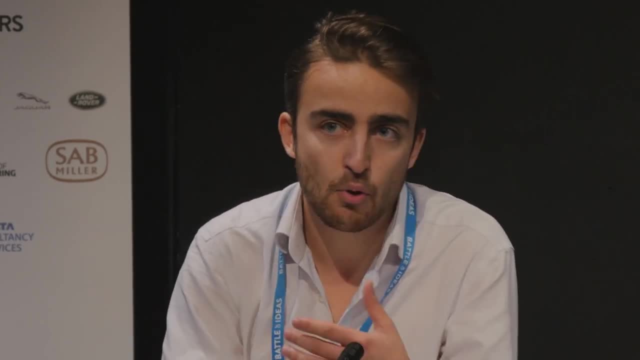 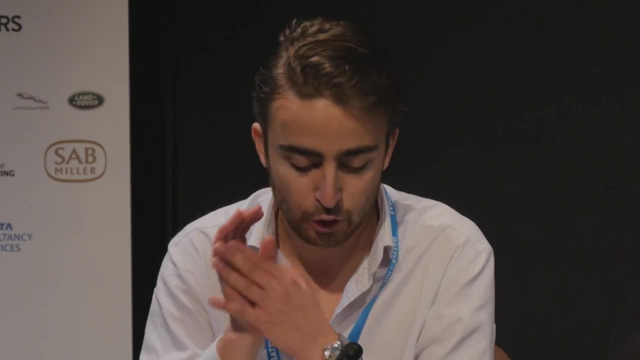 of my life so far. So I'm not going to, for example, discuss the research evidence of whether children can do philosophy, But I am keen to make some sort of contribution, not least to avoid shaming the reputation of the battle of ideas. 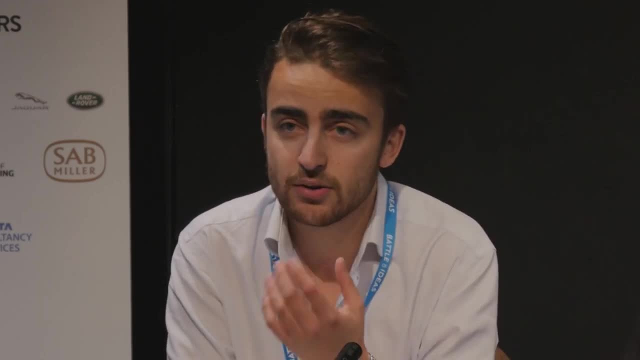 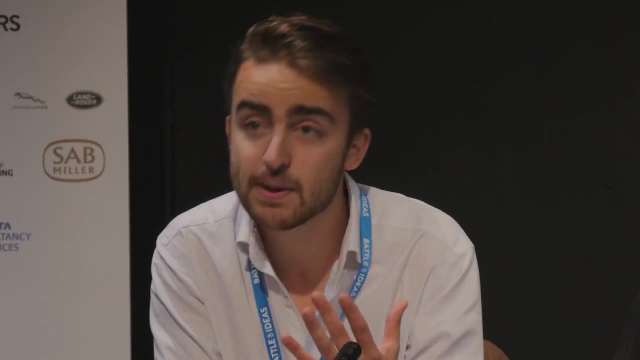 So I'm going to make an argument based from experience- or to use the appropriate philosophical term, because I do know some philosophy- an a posteriori argument. Is that right? Yes, Very good. And my experiences are based on two things. 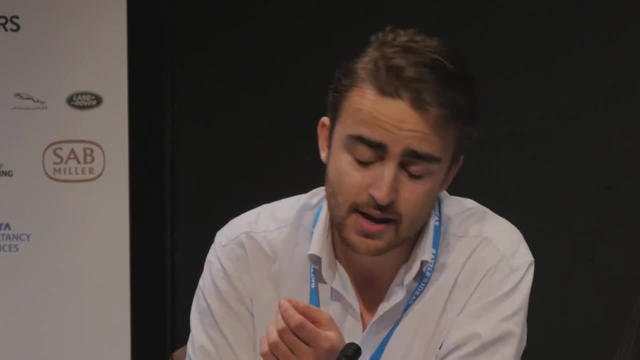 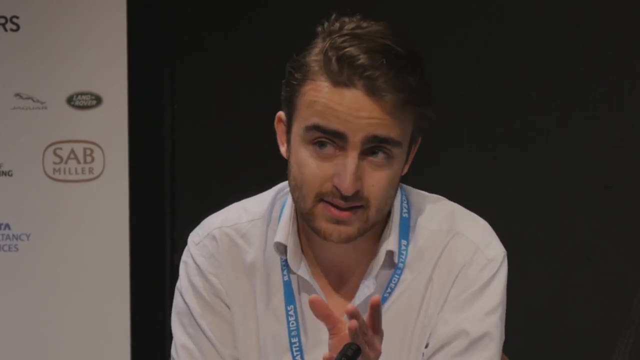 Firstly, I'm co-director of an education charity called Lauriston Knights, which I co-founded at university a few years ago, And Lauriston Knights runs summer camps for high-ability, socio-economically disadvantaged 11-year-olds where philosophy for children 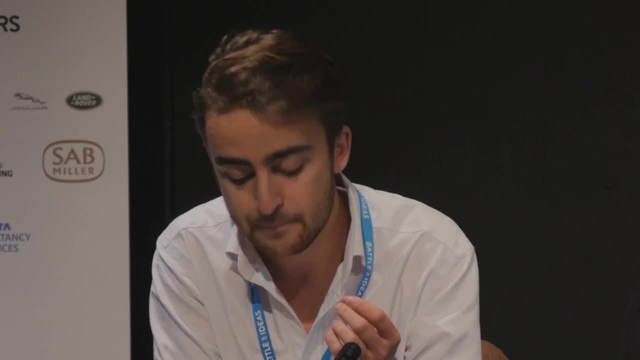 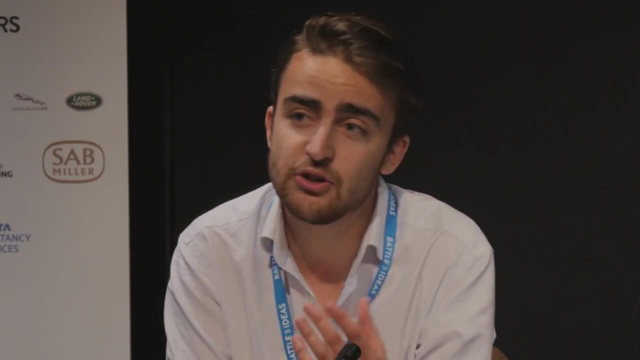 plays a major part of the programme. So I need to relay some of the philosophical ideas that the children have had on these camps to show to you that they can do philosophy. And I'm going to- and I apologise if with all the name-dropping- 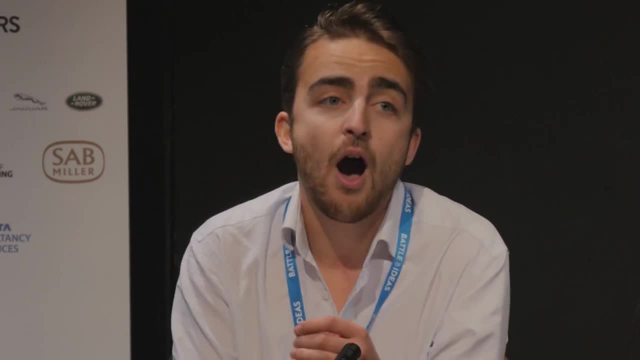 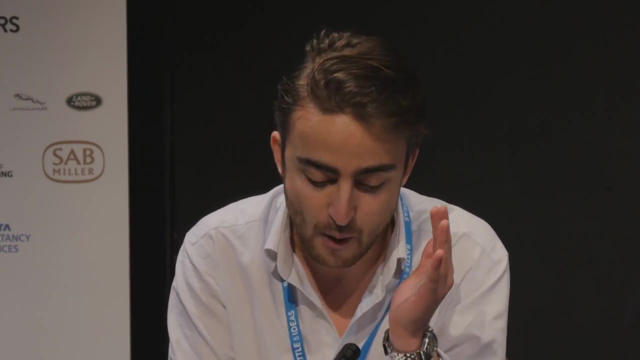 of children's names. that I do. you feel like you are listening to Jeremy Corbyn at the Prime Minister's questions. And my second basis of my experience is that, although compared to my panellists I do lack in philosophical and philosophical ideas, 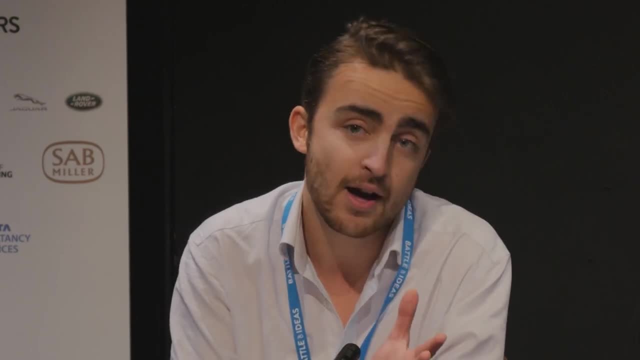 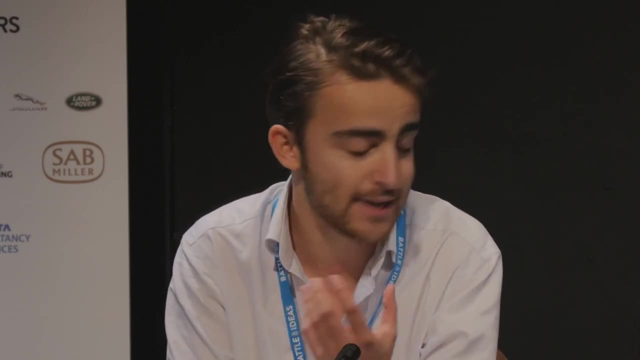 I do lack in expertise I do make up for in youth. So my point being that I am, only a few years ago, a child who tried to do philosophy in school, So I'm going to try and draw on that experience. 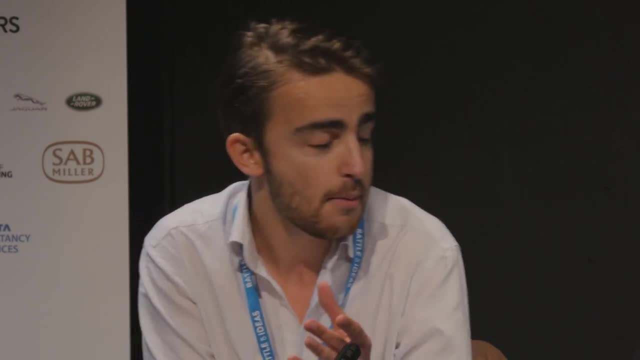 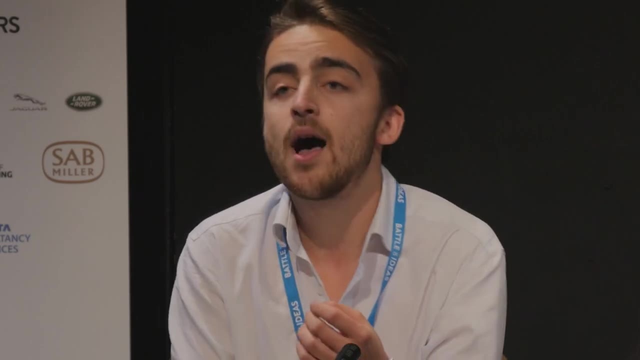 as well. So I'm going to show, argue, that children can do philosophy by showing that they can do three key aspects of what it is to do philosophy. Firstly, they can use and discuss philosophical concepts. Secondly, they can undertake critical thinking. 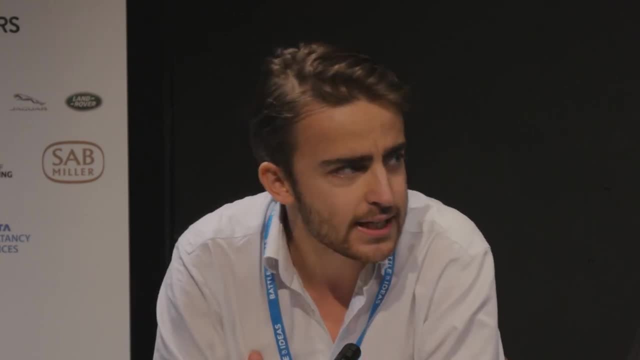 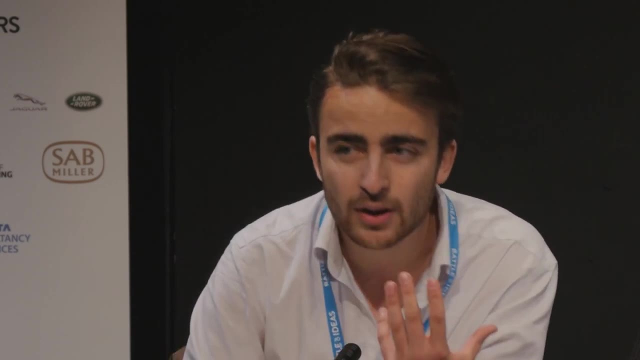 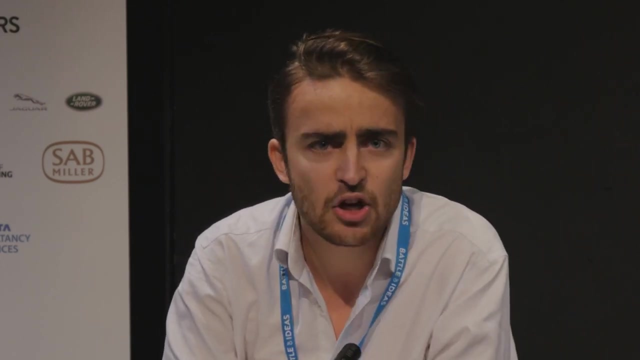 And thirdly, they can discuss philosophical concepts. I've seen children discuss and use philosophical concepts such as free will, liberty, equality. One child on a camp this year called Elvina suggested that there is equality in society when, even though there are different, 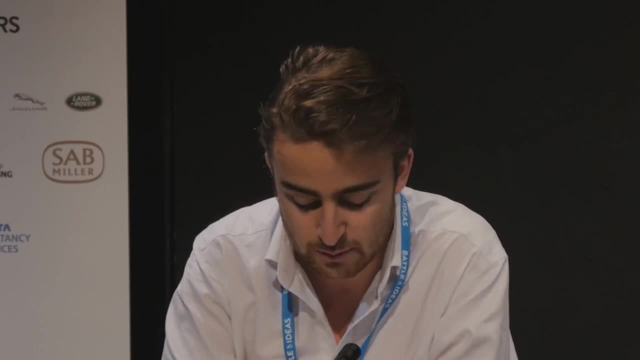 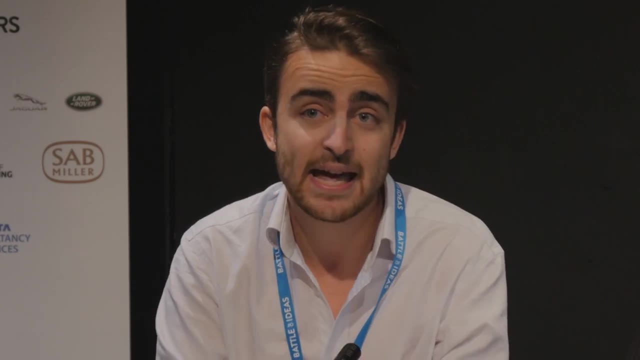 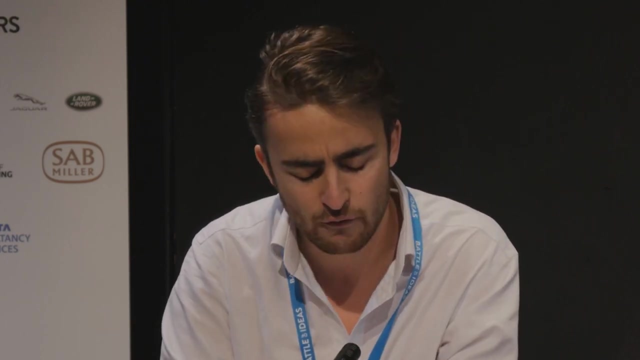 perspectives and ideas and personalities and looks. everyone is treated with equal respect. Now you could say this is not proper philosophy, because it's only proper philosophy for the use of concepts to the views of great philosophers. However, how fair a criticism of children. 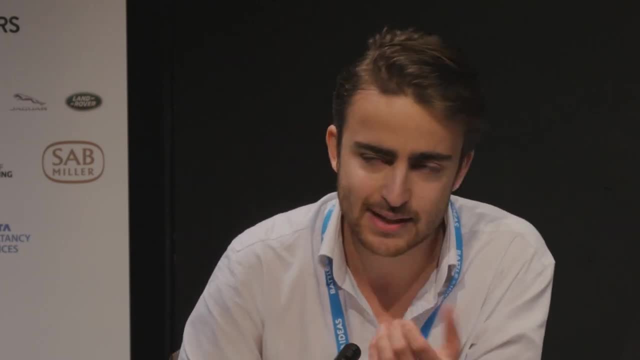 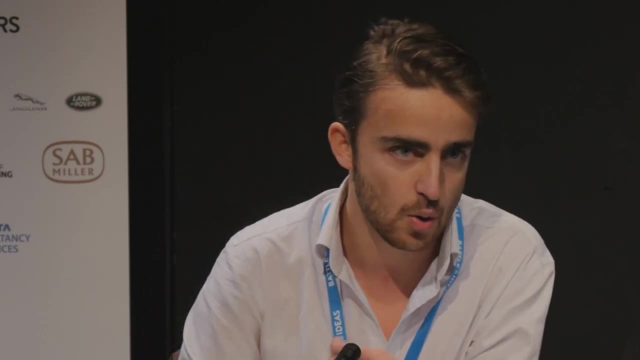 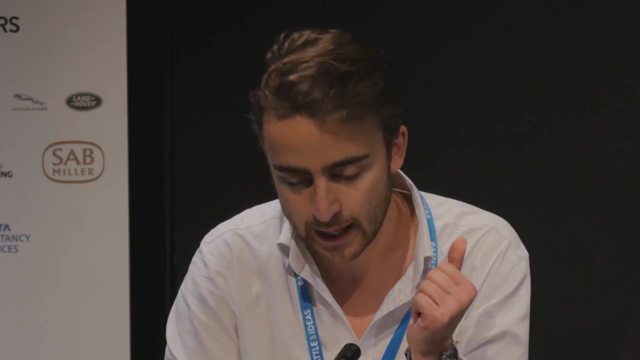 is this if we consider the record of adults in society. How often do we see politicians in Houses of Parliament or panelists on Question Time link their views on equality or justice back to John Locke or John Rawls? I'd say all too rarely. 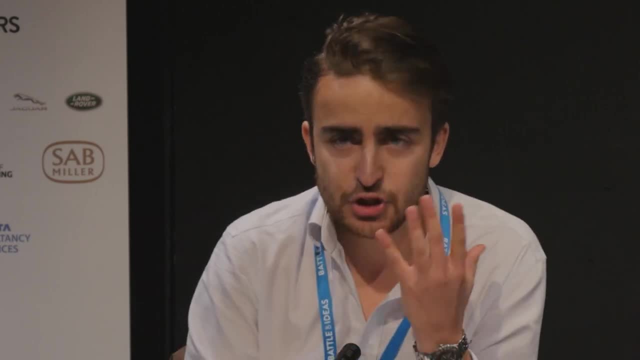 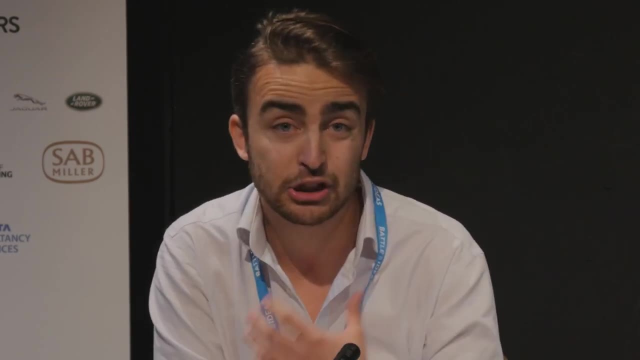 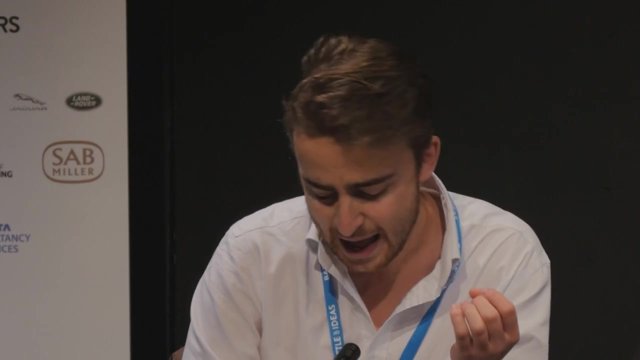 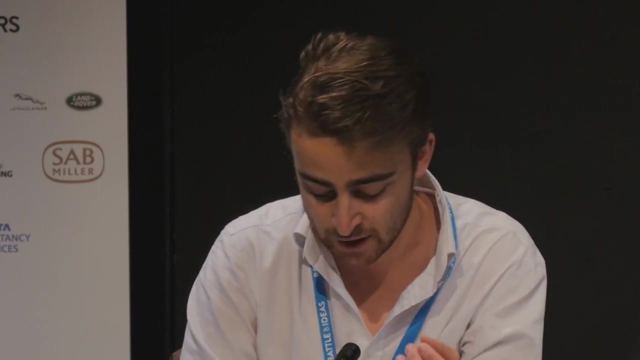 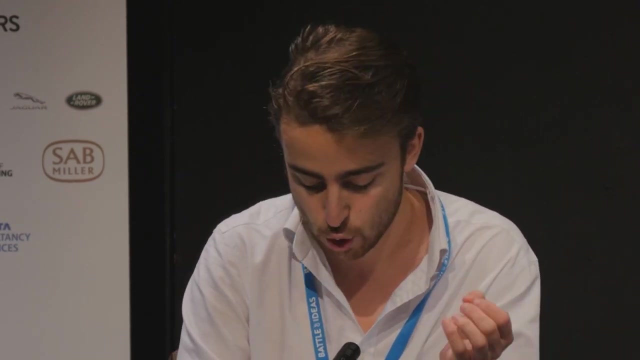 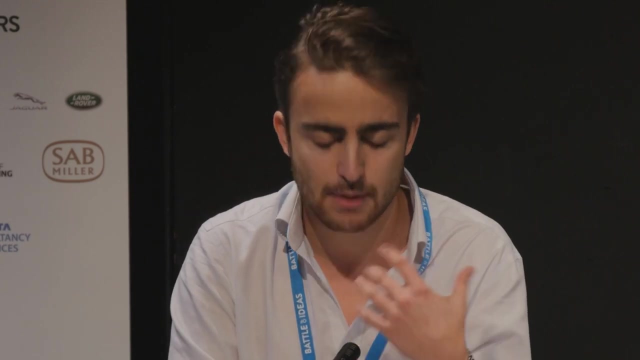 unfortunately. Secondly, I think that the way that we think about the value of society is not just the value of society, but also the value of society, and the value of society and the value of the world. And I think that the way that we think 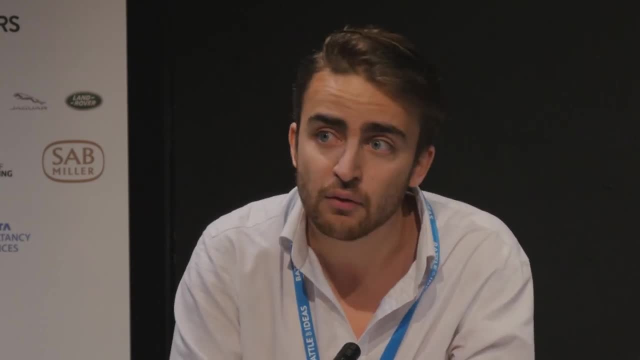 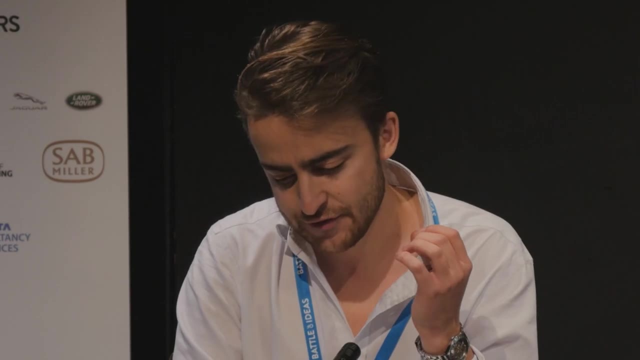 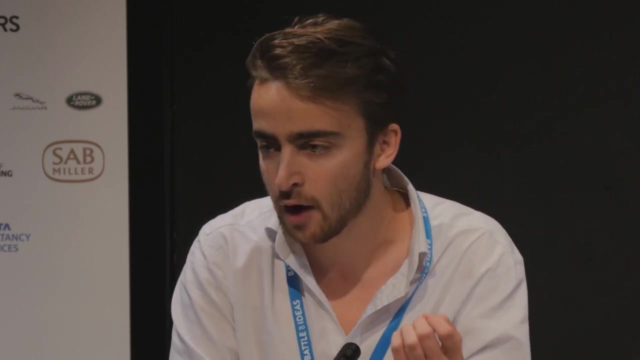 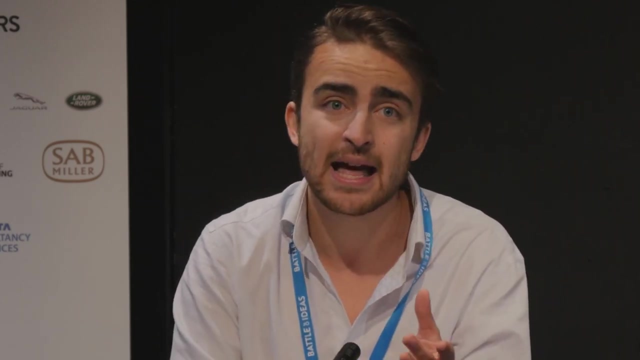 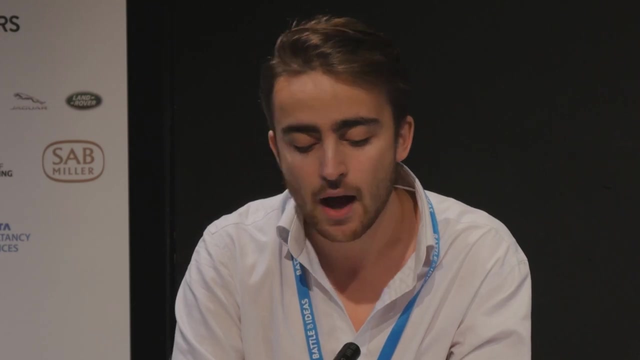 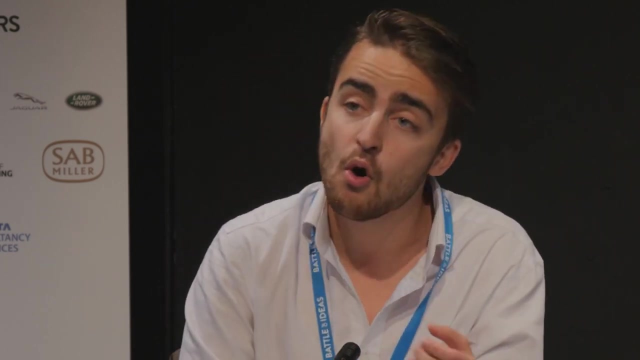 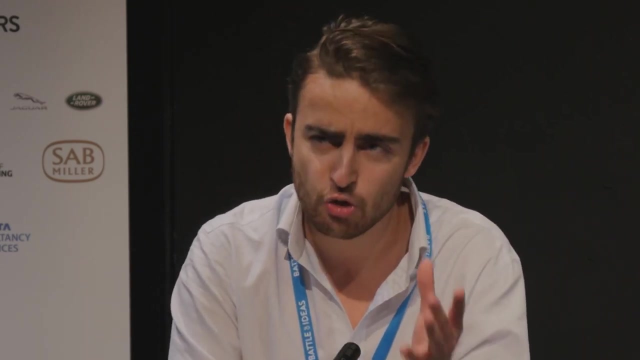 about society is not just about the value of society, but also about the value of society, And I think that we need to think about the value of society and the value of society and the value of society. So I think that we need to think about 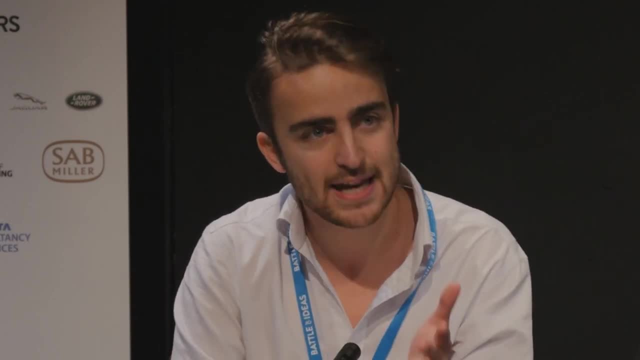 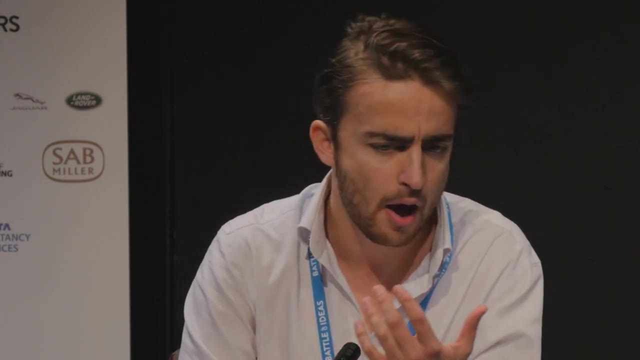 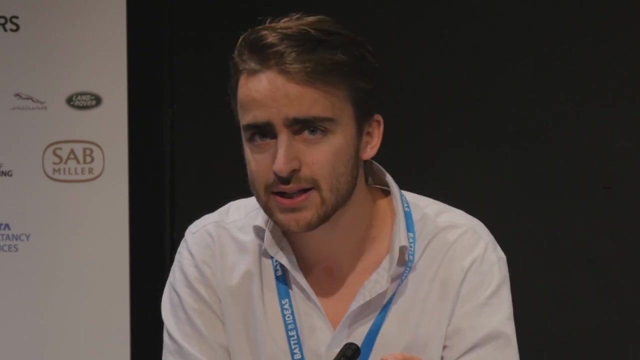 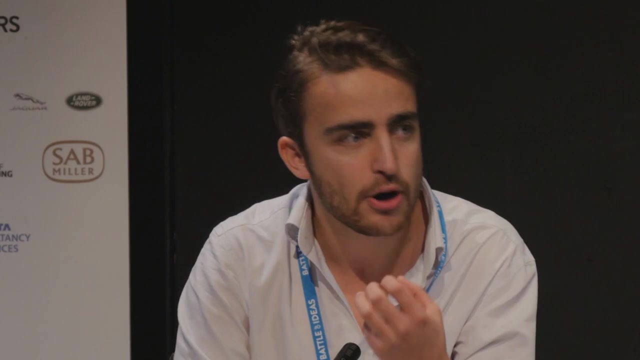 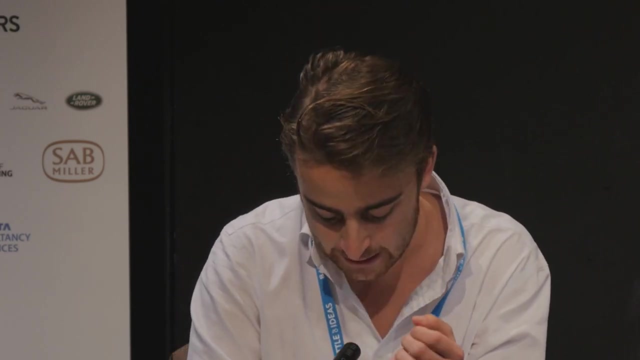 the value of society and the value of society as a whole. So I think that we need to think about society and the value of society and the value of society. So I think we can also think about society as a whole. I think we need. 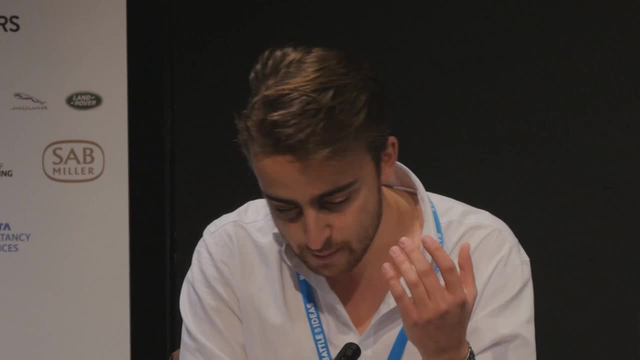 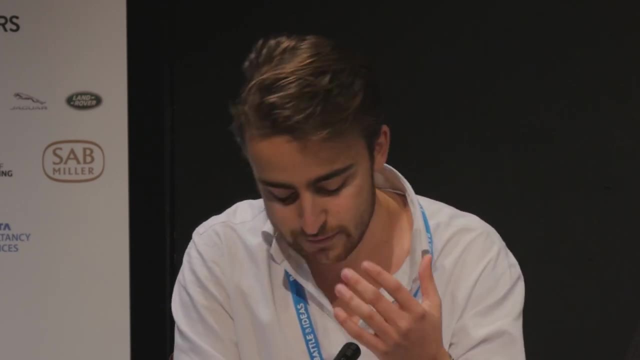 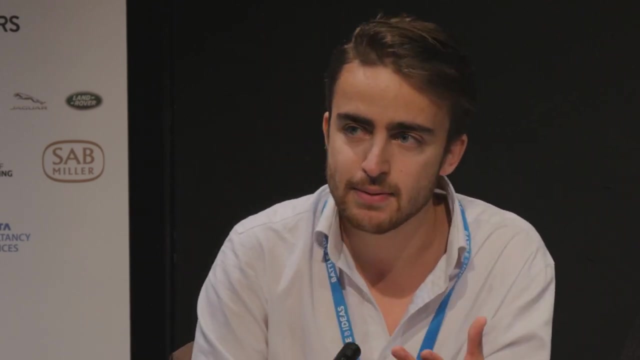 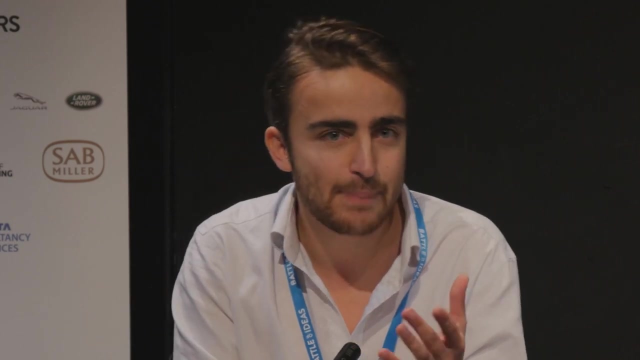 to think about society as a whole. I think that society is no more a place where society can maintain the survival of society. We need to think about society as a whole. So I think that we need infant deity, who afterwards abandoned, ashamed of his lame performance, really inspired a curiosity. 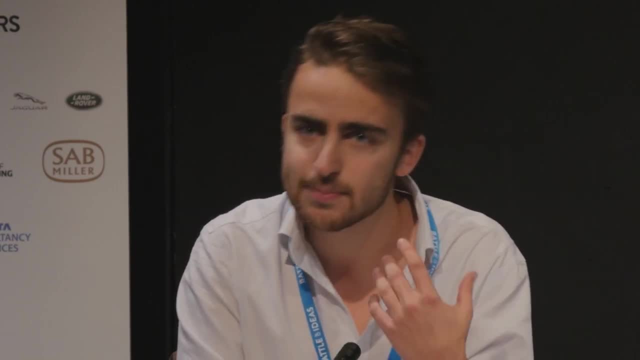 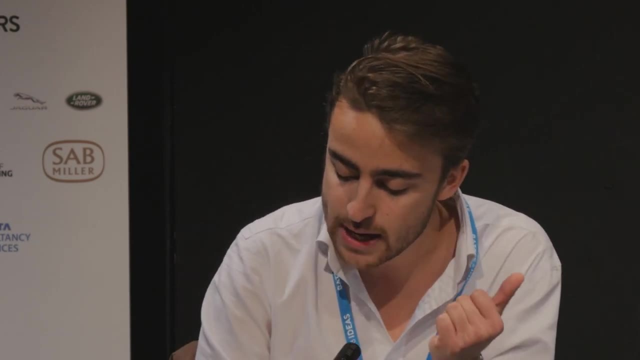 in me about how philosophy bared on science and cosmology and on mathematics. I think this kind of experience can and does happen for other children as well. So, in summary, I think children can do philosophy. It's not only inaccurate to say they can't do philosophy, it is also education. 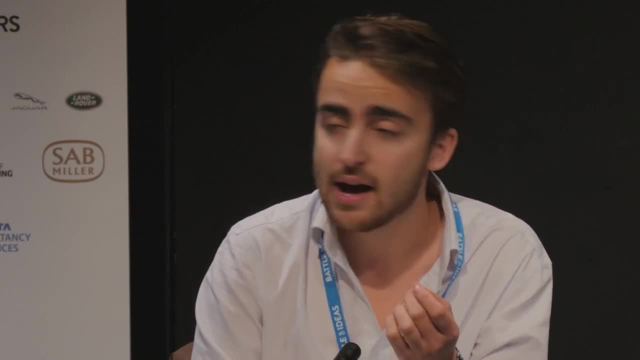 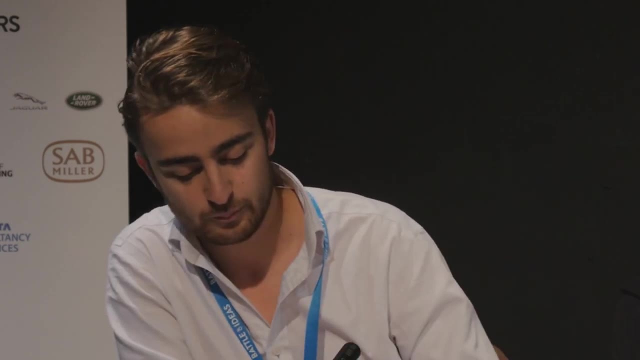 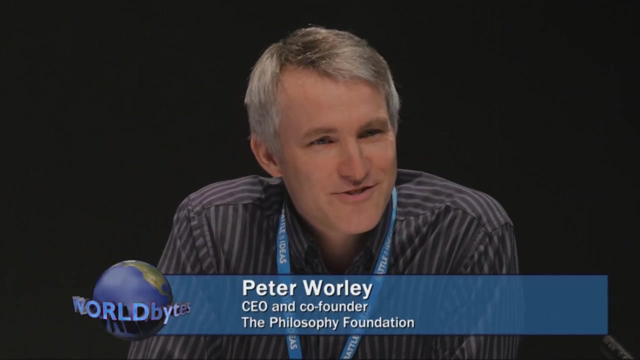 irresponsible, for it would limit the horizons of children and it would limit their capacity to develop both as children and as future adults. Excellent, thank you very much. Thank you. I'm a bit conscious of the fact that I'm the third person now who's going to be saying yes to this question. 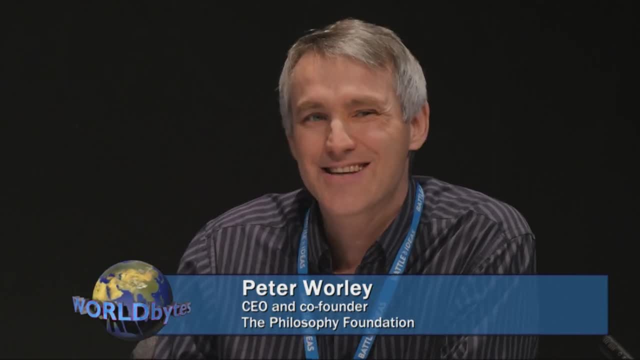 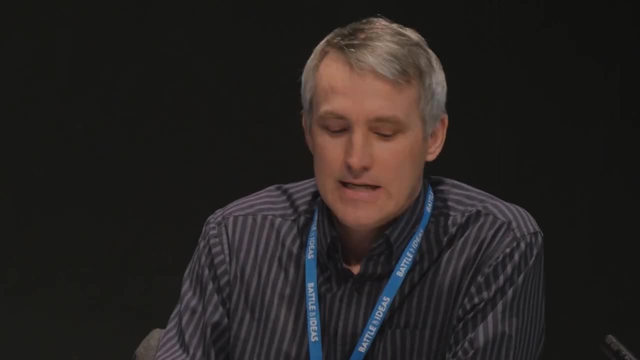 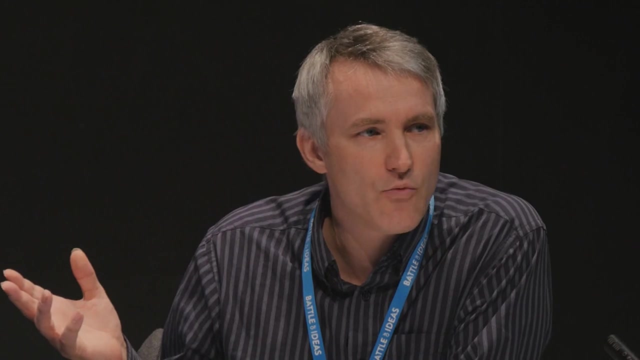 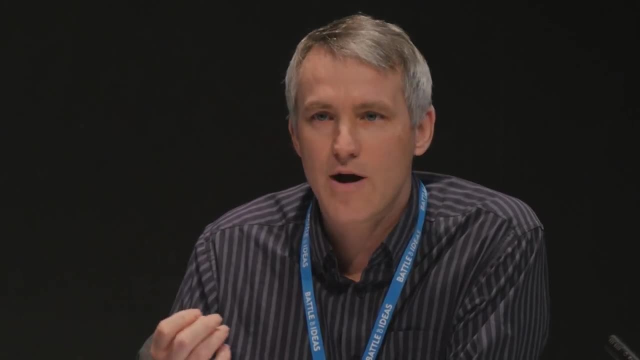 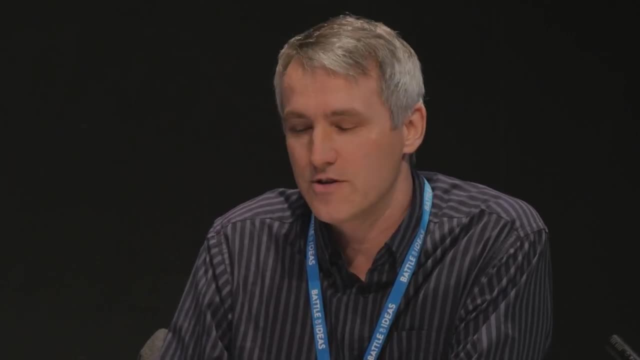 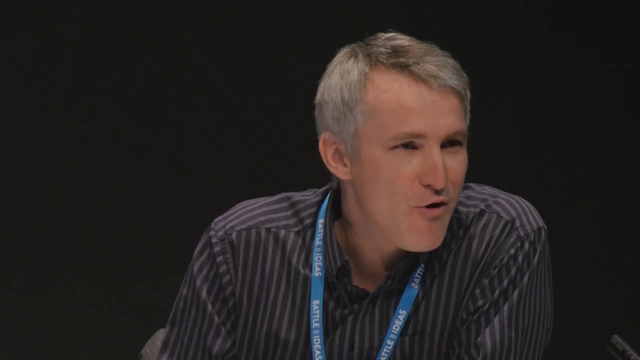 when they try and do this. So let me outline four ways in which one can answer this question, four ways that it's usually done. One is a sort of slightly flippant way. You often get this with people like GE Moore, who was asked what philosophy is and he just 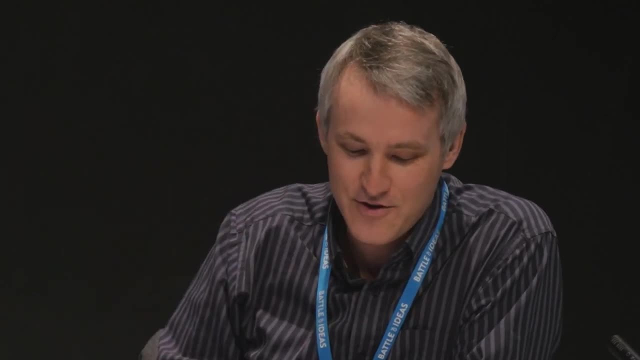 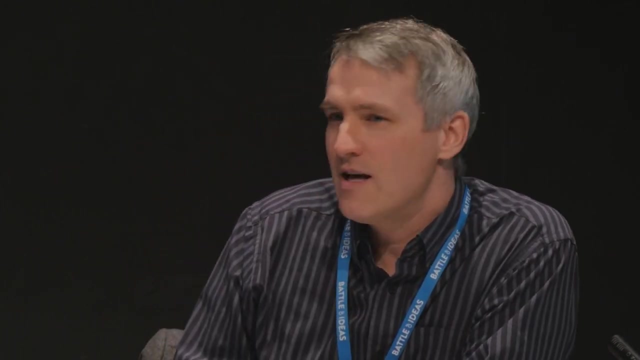 pointed to his bookshelves and said: all this You get. I can't remember who it was that said that it's incomprehensible answers to insoluble questions, Things like this which are slightly flippant. they're obviously not going to bring us to. 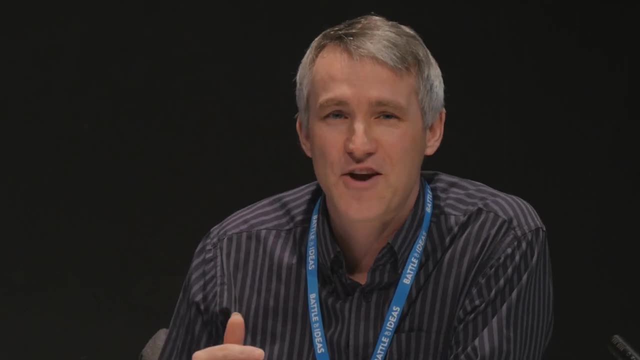 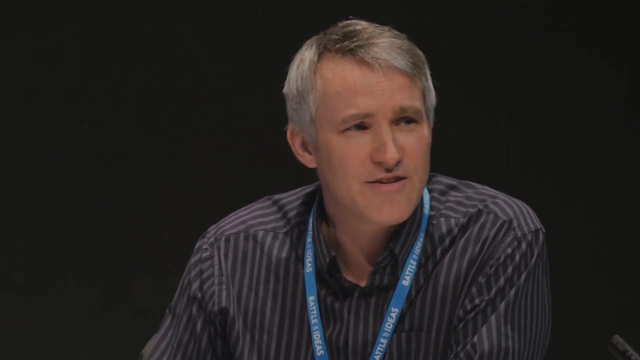 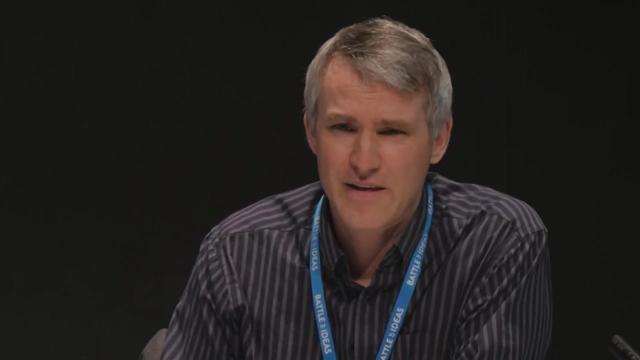 the second way of answering, and that would be to try and draw up a list of necessary and sufficient conditions, which, of course, is the really tricky area, As with poetry and various other things and art, philosophy is notoriously difficult to pin down And, in fact, anything other than a square. 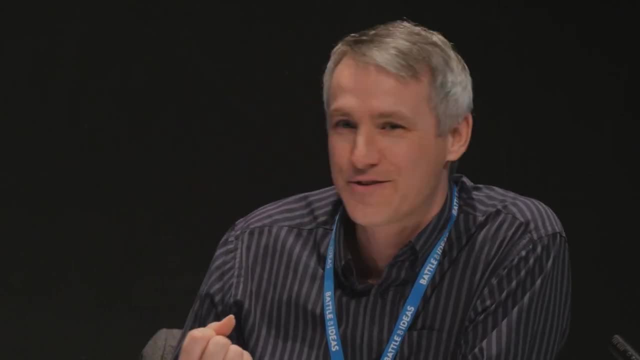 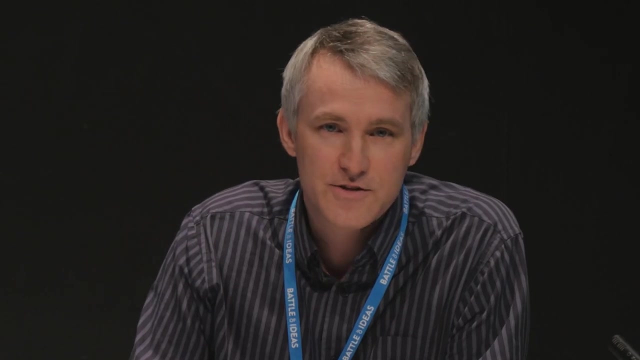 Is pretty difficult to pin down in necessary and sufficient conditions, as Socrates found out. So I think that's always problematic, And that's partly to do with Wittgenstein's response to this, which was to do with, which was saying: well, that's a mug's game. 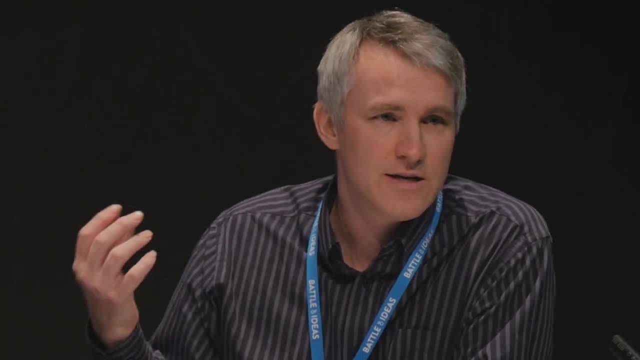 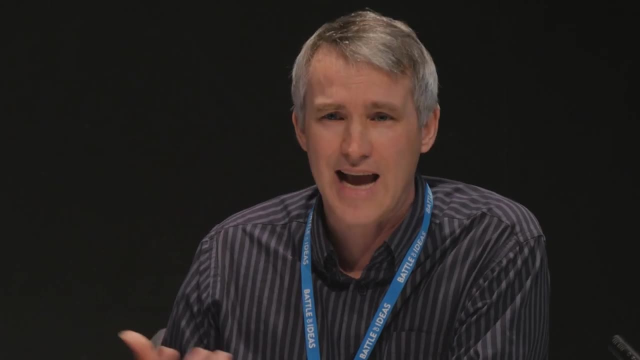 And he started to say something about family resemblances. okay, so that there are certain features that will be cropping up When philosophy is being done. there are certain things that you might expect to see happening. However, they're not always going to be the same things that are happening. 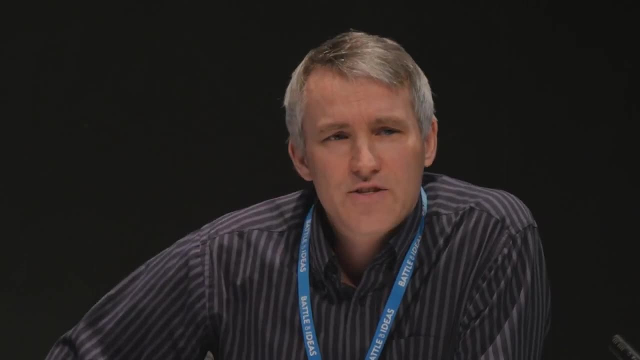 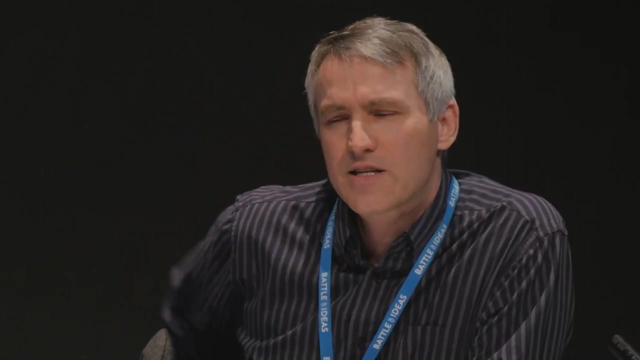 And the last way to approach- it is the way that I've chosen to do so- is to do it in the terms of a framework. So, as I think a lot of people often say, as Catherine said right at the beginning, it depends what you mean by 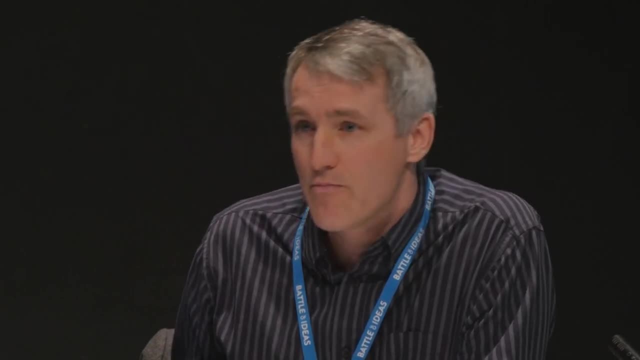 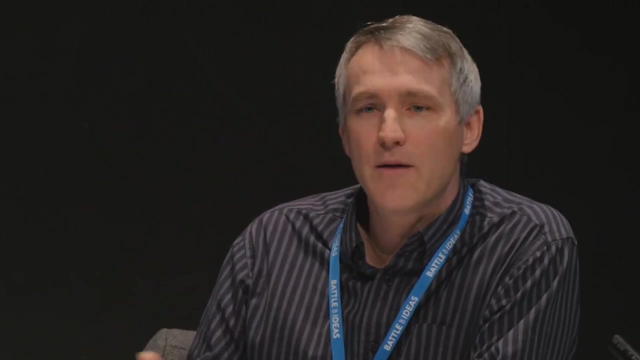 Well, one way of providing a framework is to say what you mean by. So what I mean by when I talk about philosophy is: and then I can start to talk about it. I'm not necessarily claiming that this is exhaustive or that this is the end of the 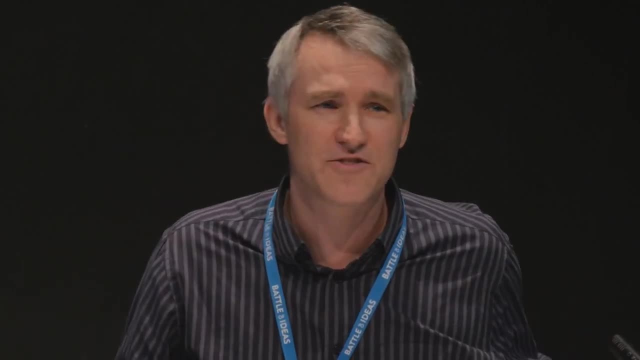 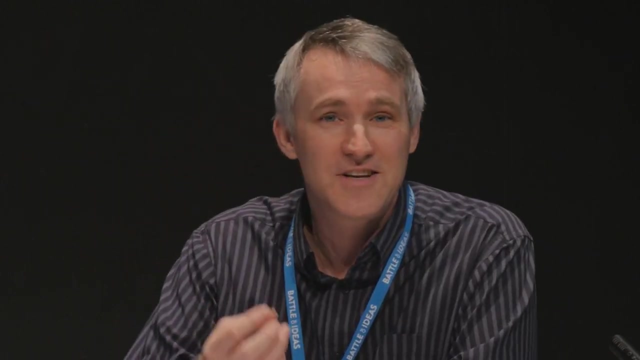 general. I'm not necessarily claiming that this is all the things that might be considered relevant to discussing what philosophy is, But I can say something about what I mean by. So, if you read my books, for instance, or if you are listening to me talk about it, 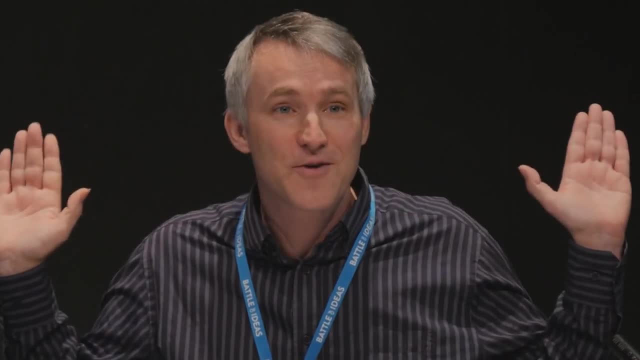 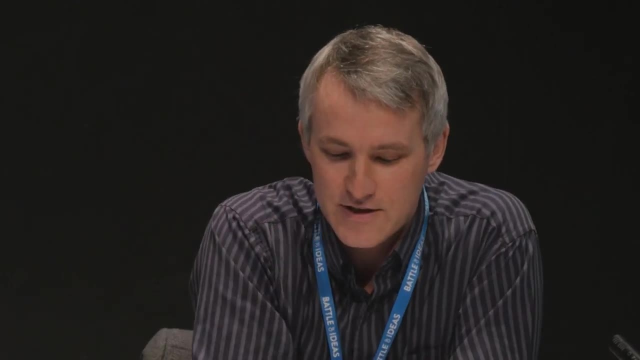 you get some idea of what I'm talking about, rather than just avoiding talking about the actual thing we're talking about. So I might- I'll have to draw upon a written text for this, because it's that kind of thing, isn't it? 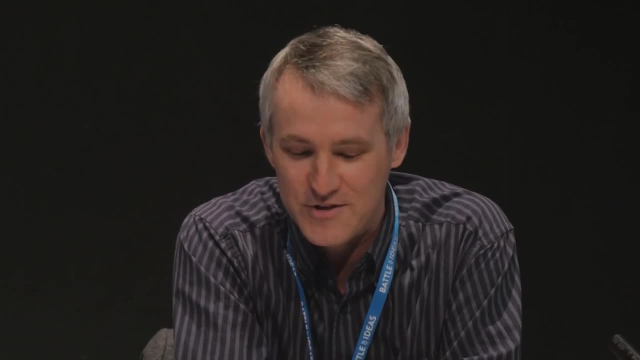 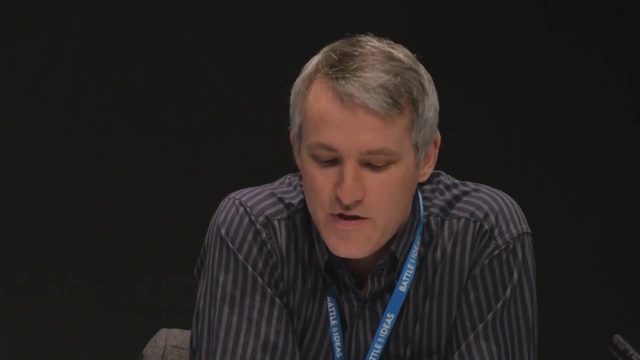 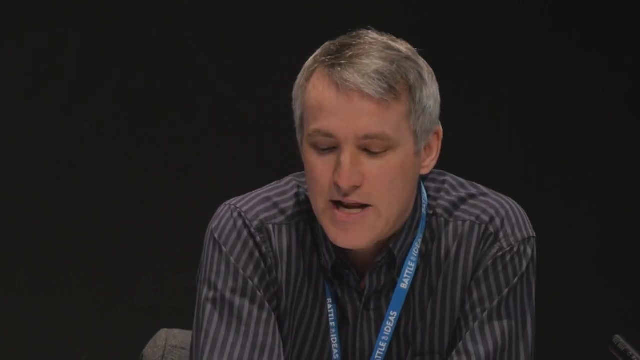 So here's my bold attempt to say what philosophy is. when I do philosophy, when I'm working with children, Philosophy done well. Philosophy done well should be rigorous, structured, sequential conversation with others or oneself that is both collaborative and oppositional, that attempts to explore, explain. 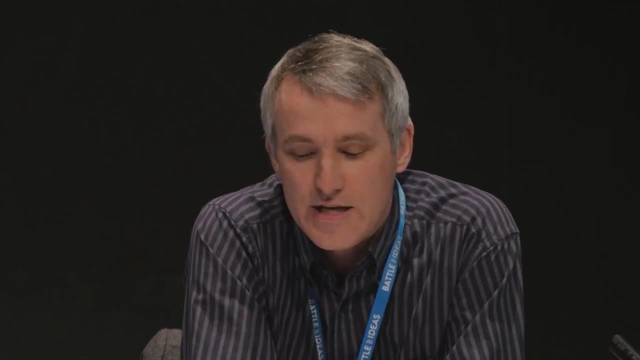 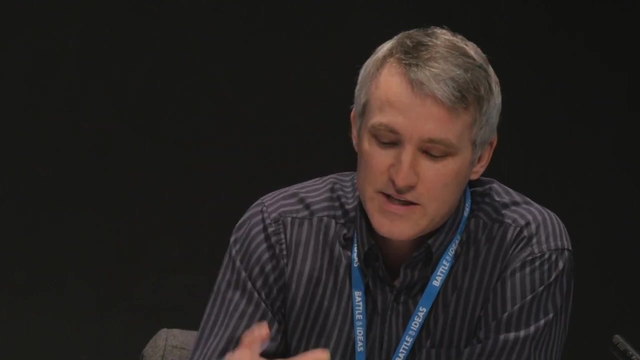 and justify the structure and content of our thoughts in response to perceived problems and puzzles about reality, knowledge, value and meaning. Philosophy employs a method, process, more often than not ongoing, of reflection, reasoning and reevaluation. Why? Employing the appropriate intellectual virtues or principles? 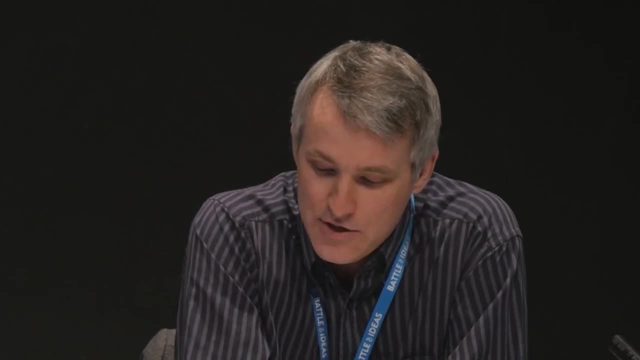 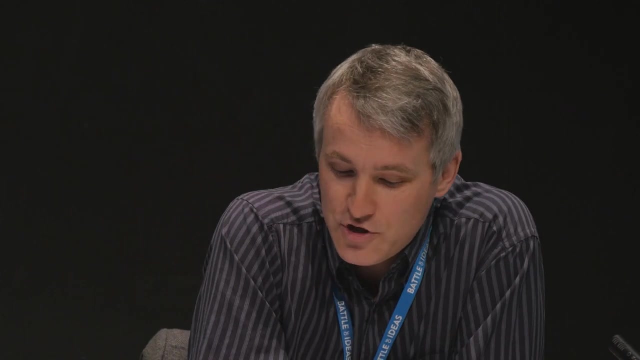 Why? Why Cultivatingדriving the parts of our de blastsor excellence in order to make good, though provisional, judgments about what seems metaphysically true, morally right, logically coherent? The aim is to improve our understanding, also understanding what we don't understand. 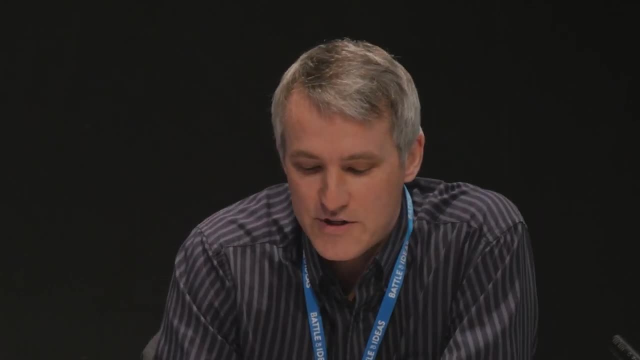 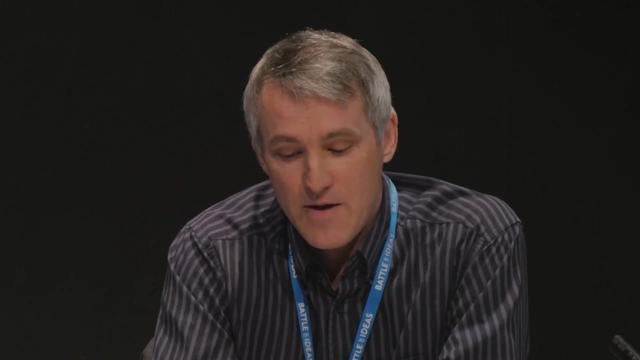 or such things at the work ourselves, our experiences and other people By refining how we think about those things. The hope is that by doing philosophy, we learn to think better, to act more wisely and thereby help to improve the quality of all our life. 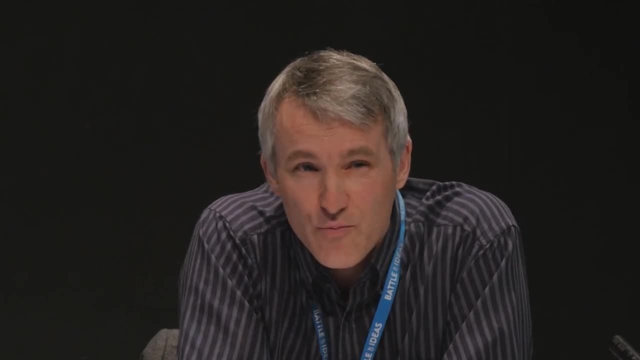 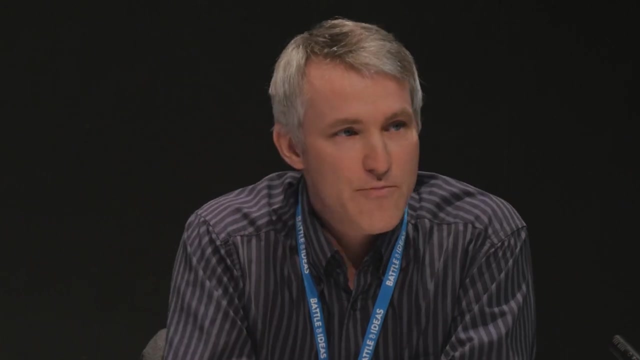 the quality of all our lives. I must underline that that last bit is hope. I'm not saying that that is what it does, That's another question. So that's kind of what I mean by philosophy, And that's great. I've put that out there, that you can all challenge me on that now, which is of course. 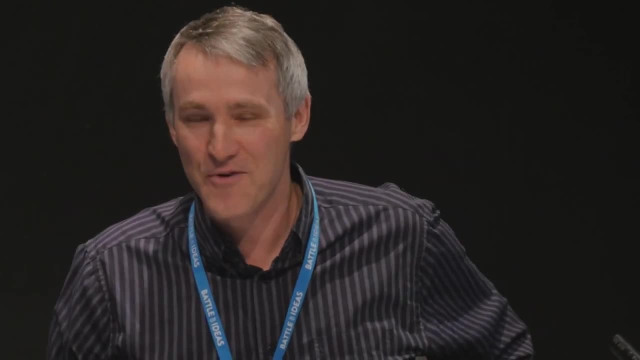 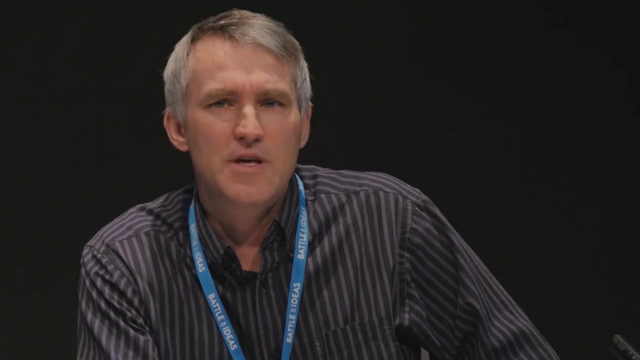 what people avoid happening by not saying what philosophy is. But the other thing is that when I do look at the list of things we see in philosophy, if you like, the family resemblances model answer what sort of things are going on. Well, you might expect something like a priori. 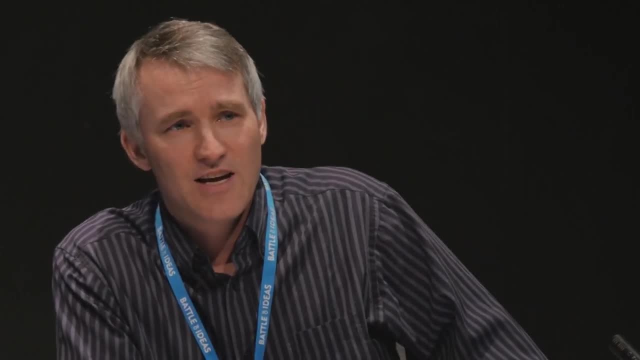 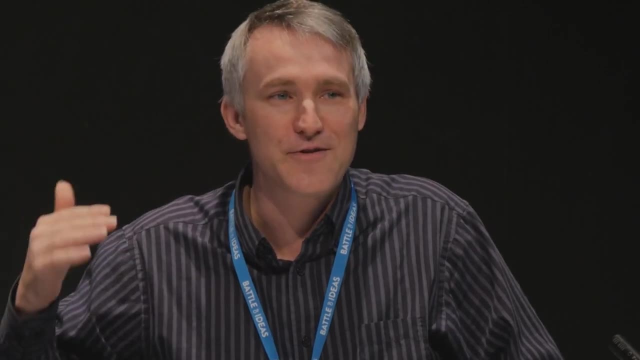 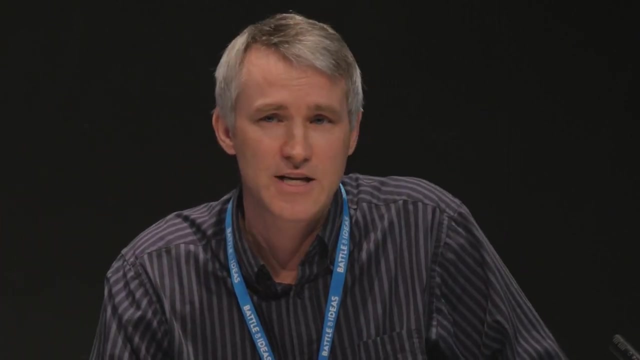 reasoning, You might expect something like the use of argumentation. I've got loads of footage on our website, which is wwwphilosophy-foundationorg. There you can see lots of YouTube footage of children. On the homepage there's footage of children discussing whether or not. 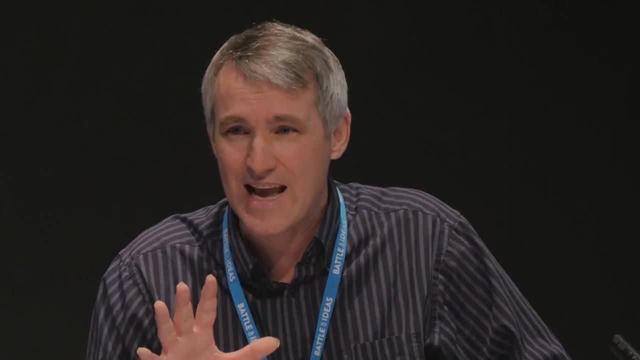 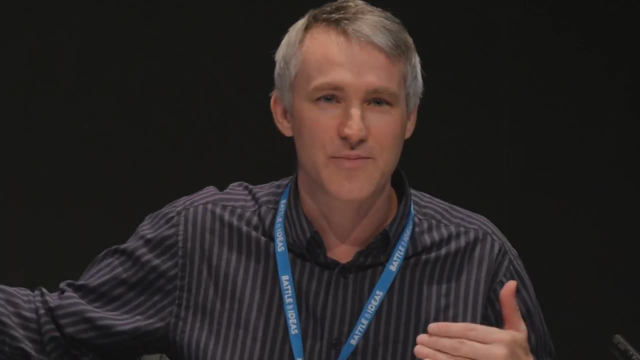 you can step in the same river twice. I think that whether or not they can do it can be cleared up by just looking at what they do and seeing if they're doing a priori reasoning, Seeing if they're using arguments, et cetera, et cetera. And I'm quite convinced, quite happy. 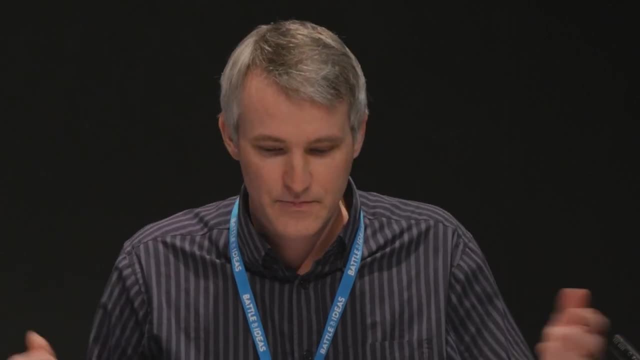 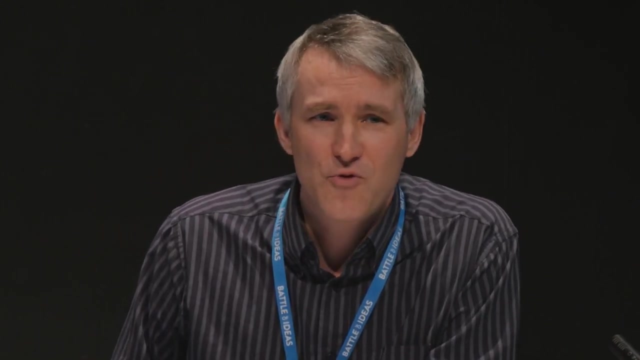 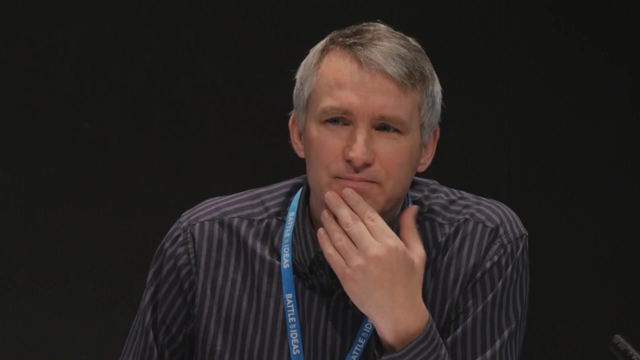 that they are doing philosophy when you look at what they can do, And if you go, you can see. I think there's a TEDx talk called Plato- Not Played though- where I'm quite rightly upstaged by Noah and Alice. Noah says: I've invented a new thing. It's called an anti-thing, And he goes on. 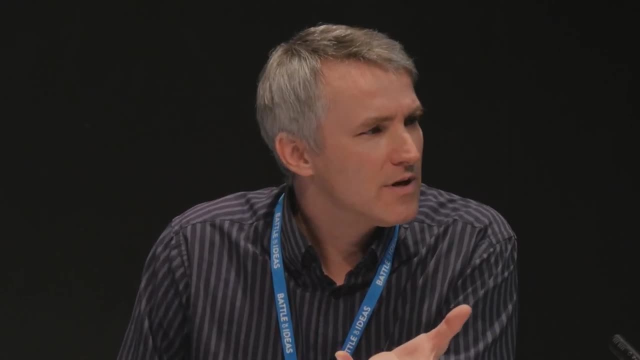 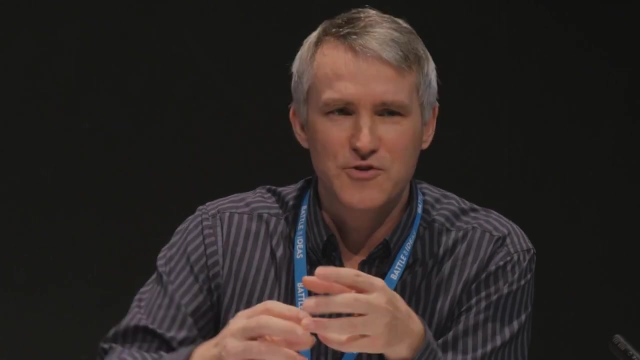 to say that anti-things have no properties, but they have consequences. And he goes on to say that they have consequences. And he goes on to talk about time, motion, gravity, And he goes on to explain in great detail how this works. And if you look at the piece on the footage, don't take my 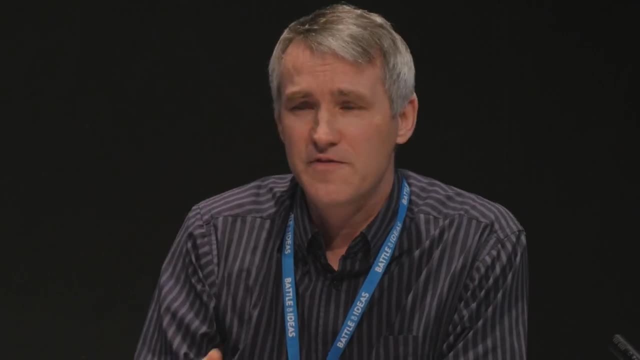 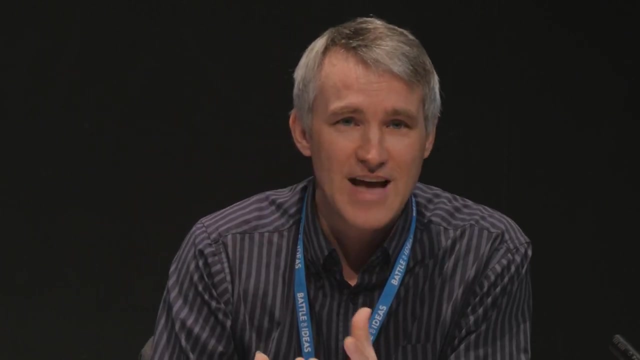 word for it. just watch him say it, you'll say: well, there's a lot of philosophical features there. He's talking metaphysically, He's constructing an argument, He's coining new terms, He's dealing with really rather abstract and difficult notions. He's tackling these difficult things. 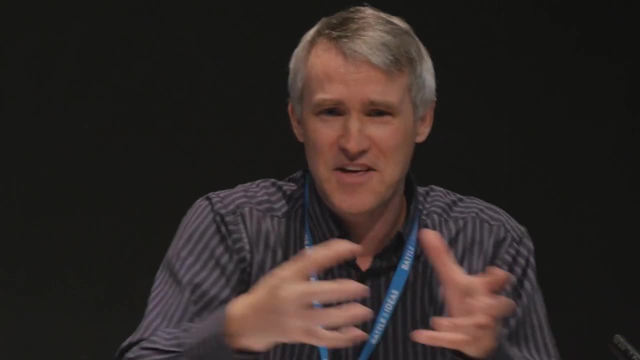 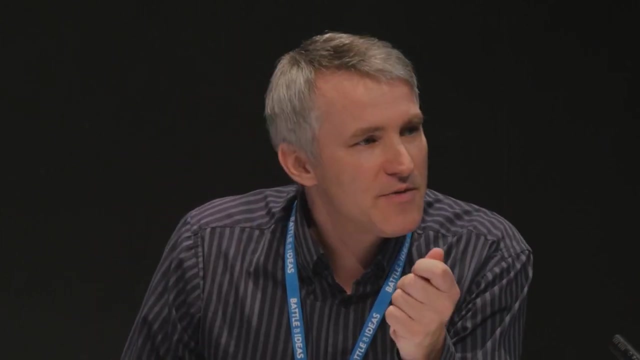 such as gravity, which is not a thing like love, But it is a thing like love: It has an effect on the world. But what exactly is it? So you could say that this is philosophy, But I would say there's something fundamentally missing. And when? 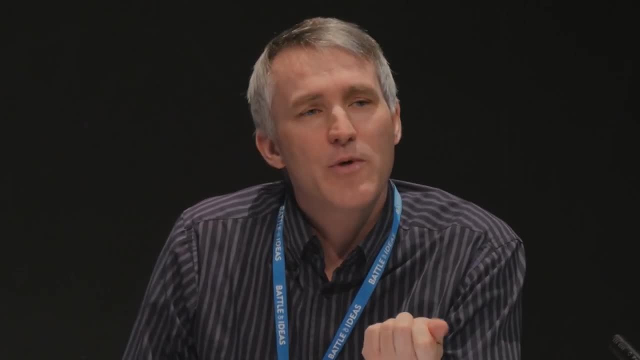 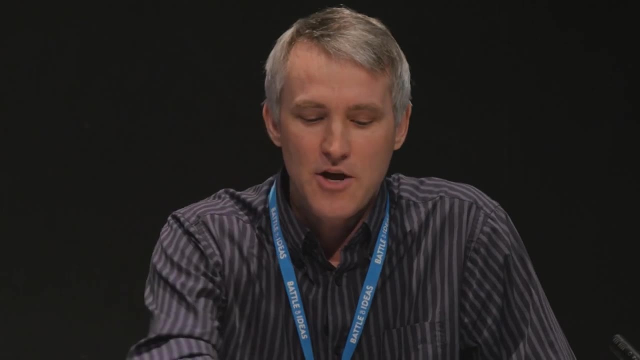 you look at the Wittgensteinian model, what you can say is that we can come up with some candidate, necessary conditions, the sorts of things you'd expect to always be there, or at least very often, And I would say that one of those things- I've got four R's that I've identified as candidate. 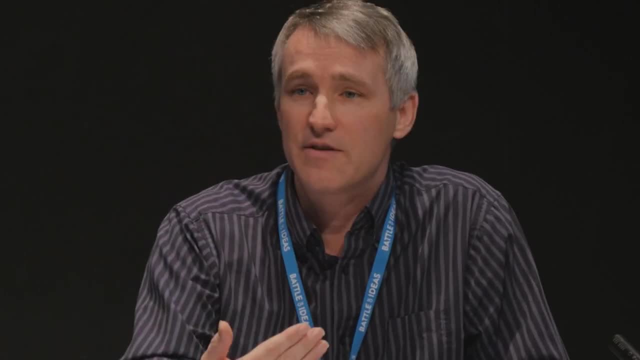 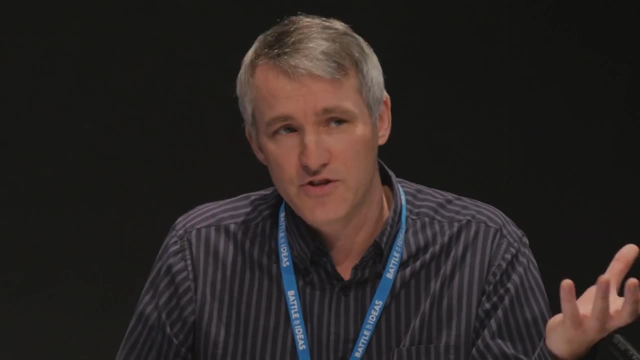 necessary conditions for philosophy. Philosophy has to be responsive. It has to be responsive, It has to be reflective, It has to be reasoned. All of which Noah is doing. But there's one thing he's not doing, which Alice, who's three years younger than him in the footage. she's 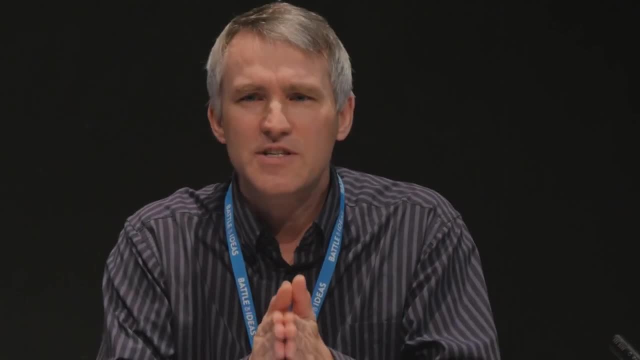 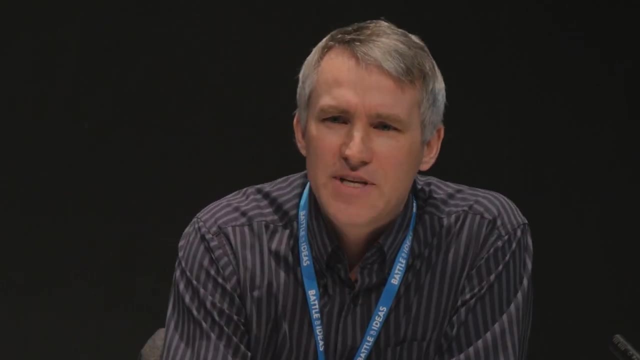 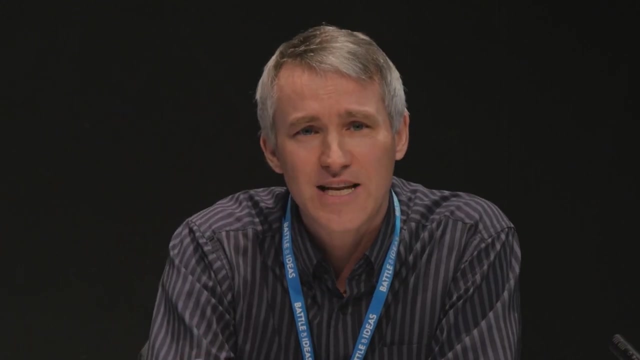 only eight and she says: but Noah? she says: but this thing anti-things, how can a thing have no properties? She says, the property of having no properties is itself a property. She's coined something important here, perhaps Alice's principle that all existing entities. 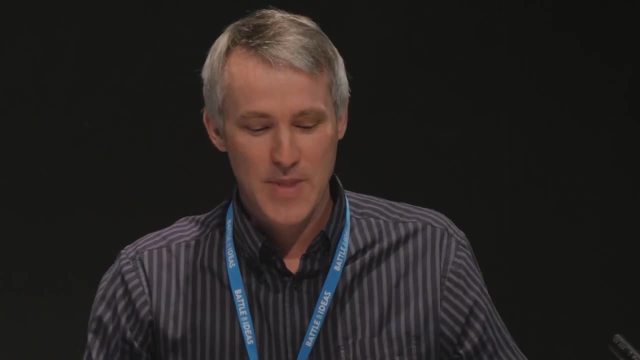 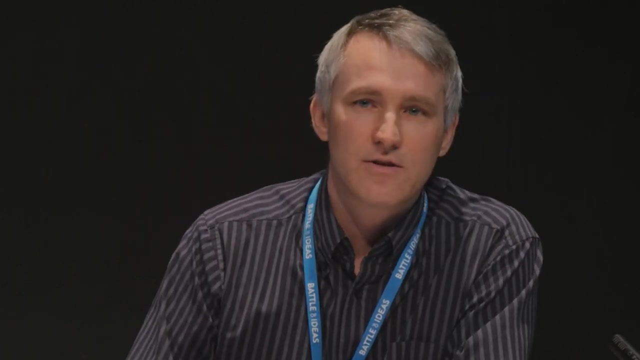 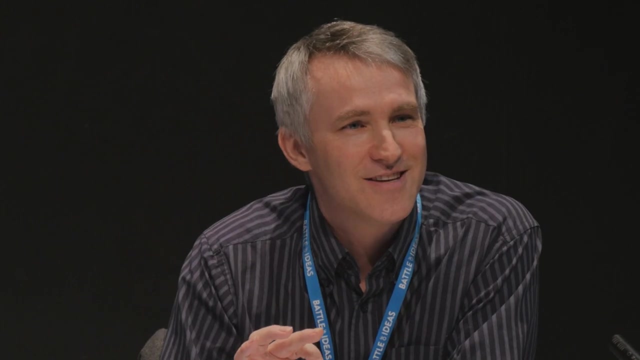 must have at least one property. Now, what she's done here is: she's done the four R, She's been re-evaluative, She's been critical. Noah wasn't, He was simply constructing a theory which sounded philosophical. But until you take the critical stance, it's not philosophy. And what we notice? 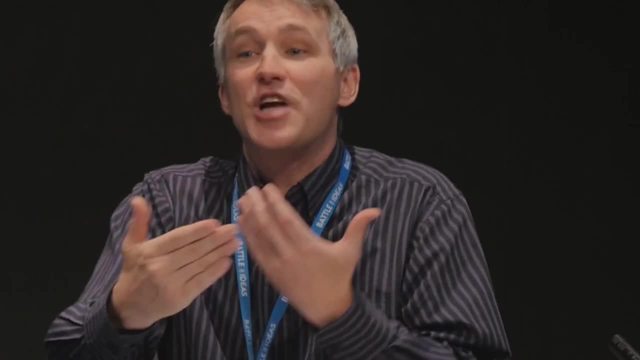 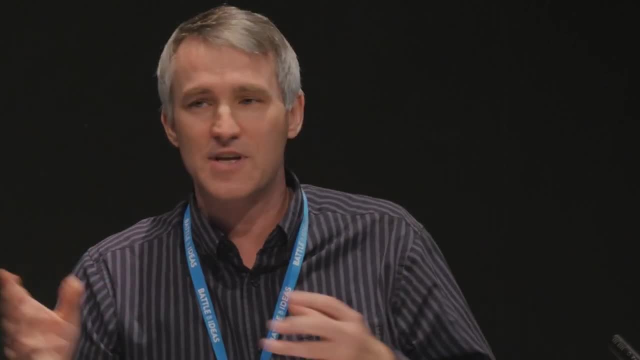 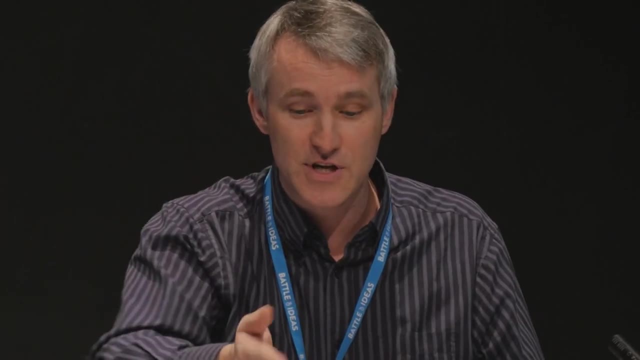 conversation of sorts, a special kind of conversation, not any conversation, as Catherine said, But that exchange must, either with oneself or with others, as I also said at the beginning, that exchange must have, I would say, the necessary feature which is to be critical. 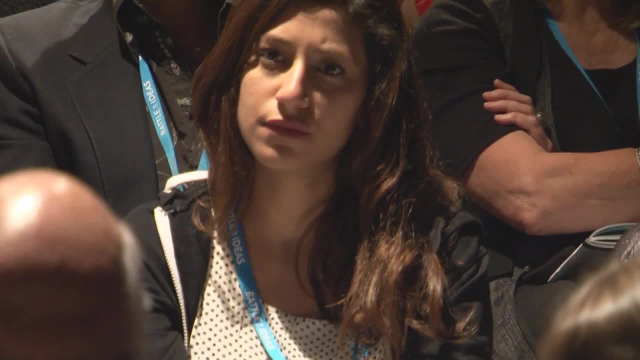 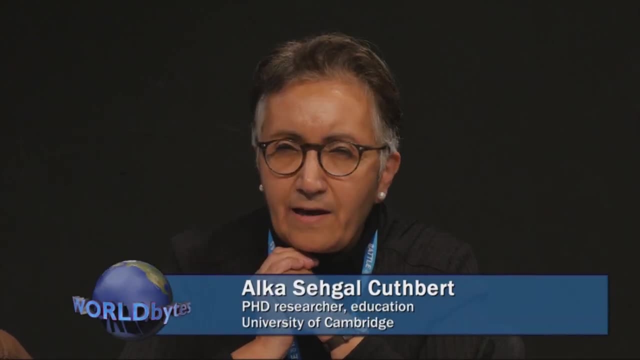 to be re-evaluative. Excellent, Thank you very much, Hauke. There's sort of two things I want to talk about in this. The first is: why, now really, Why is philosophy for education? Why is philosophy for education? Why is philosophy for education? 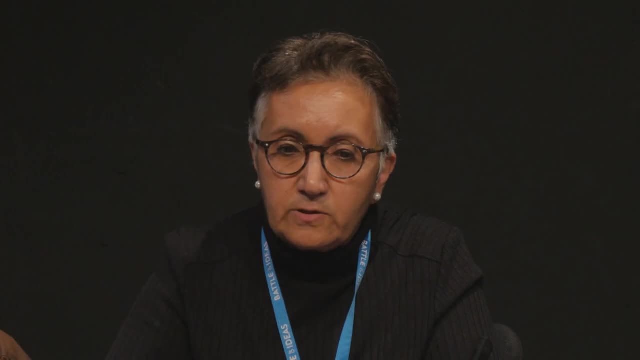 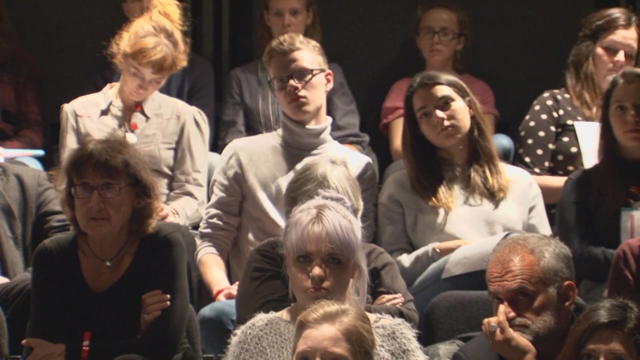 Why is it come to the fore now in educational discussions? Why is it seen as a good thing, as a solution to some problem? And the second thing is to put my tuppence worth in what the other speakers have addressed is: can children do philosophy? The question of why, now you know. 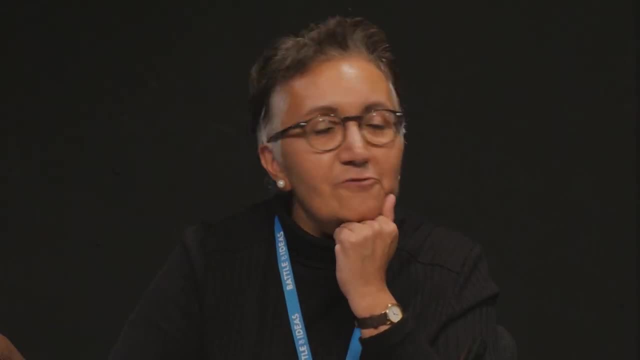 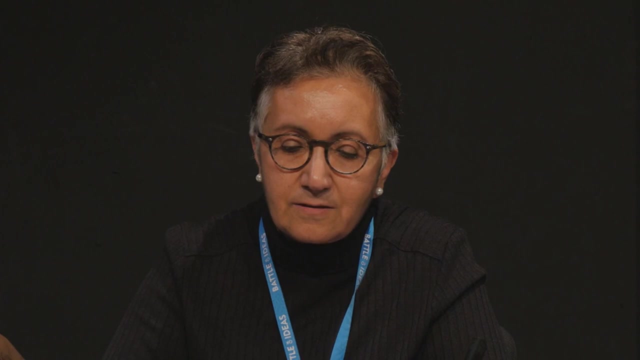 it seems so lovely just listening to this. You know, children are generally very curious, I agree, and inquisitive and come out with all sorts of quirky and endearing questions and insights. And it's often lovely to hear that And I think it's a great question. I think it's a great question. 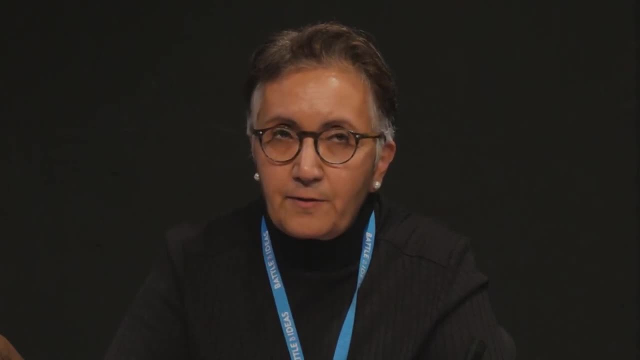 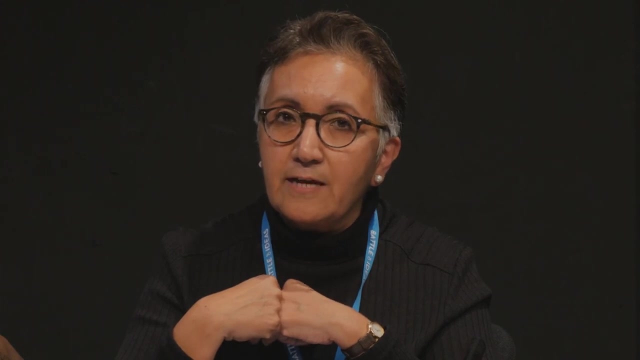 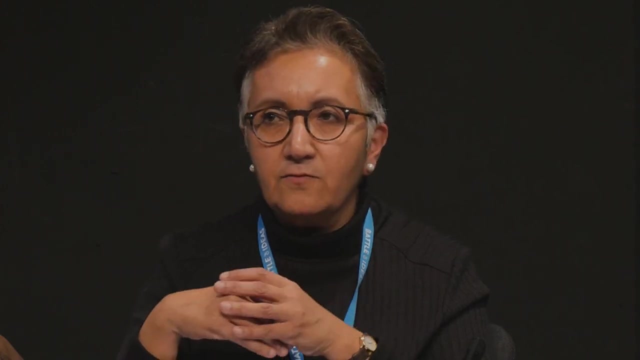 Lovely to have those conversations with them And I think you can, And I think I think in a way there's a response to an intuition that a lot of what goes on in today's schools and what goes on in contemporary education is missing, that There's a sense that perhaps after decades of instrumentalism, 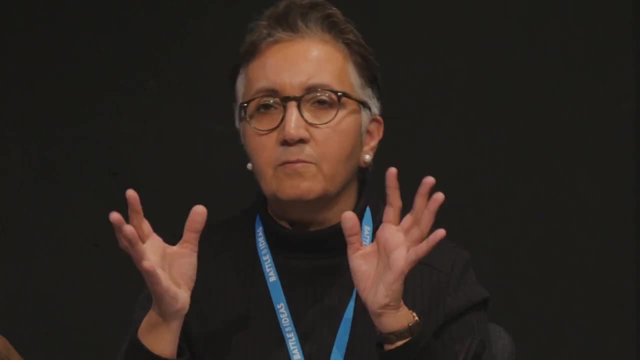 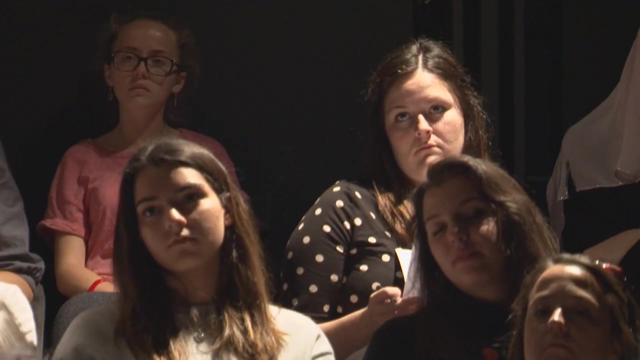 and targets and assessments and levels, and blah, dee, blah, dee, blah, dee blah, that teachers are just, you know, teaching to the test, which generally they often are, and that children are, are being sort of trained to jump certain hoops at the cost of having the more effective and 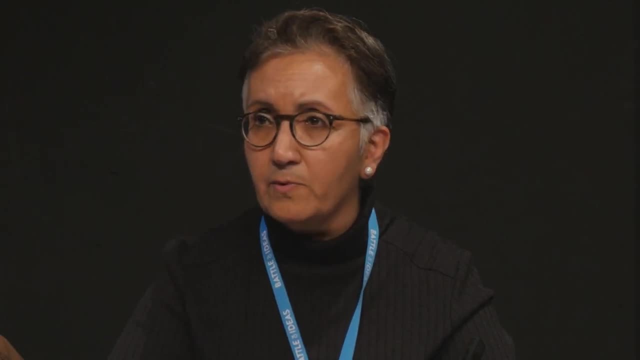 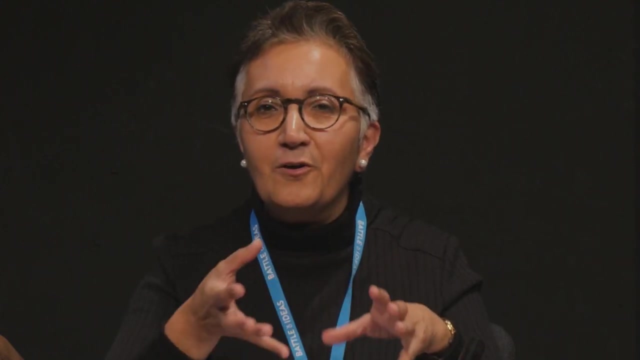 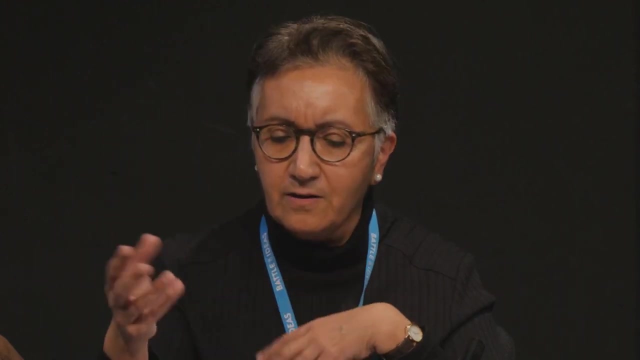 subjective and humanistic aspects of what we would like an education to be about. So that is often interpreted as as an over overloading of knowledge. This is often seen well. all schools are interested about is to put too much knowledge in, and they don't care about the discussion and 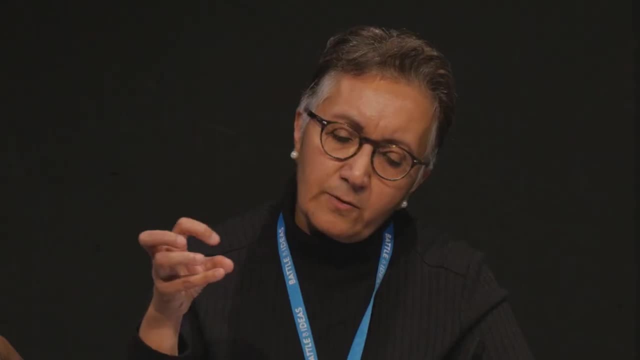 the. you know the effective, expressive sides of things. And so it's seen that if we can put, if we can bring back philosophy, we can bring back the. you know the, the, the, the, the, the, the. 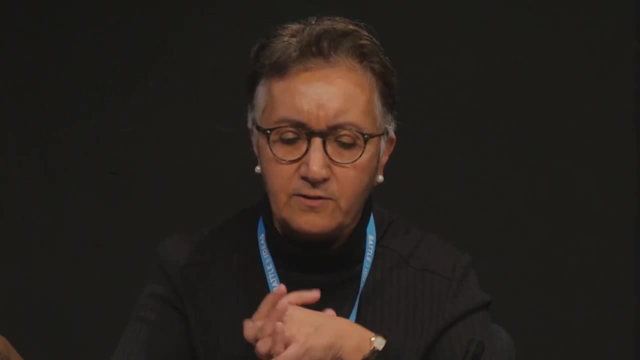 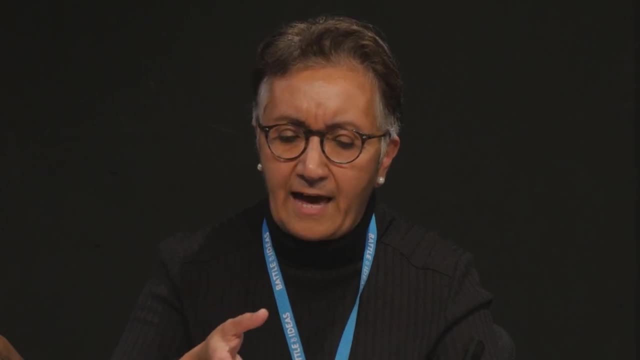 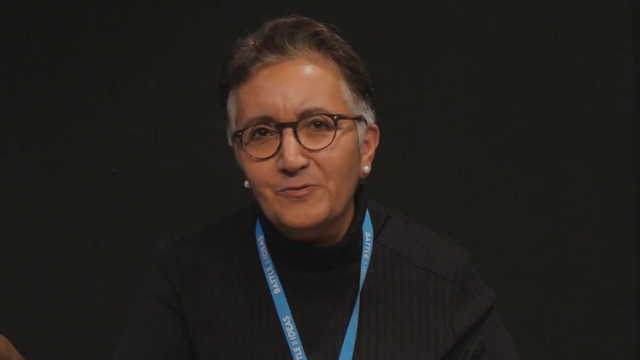 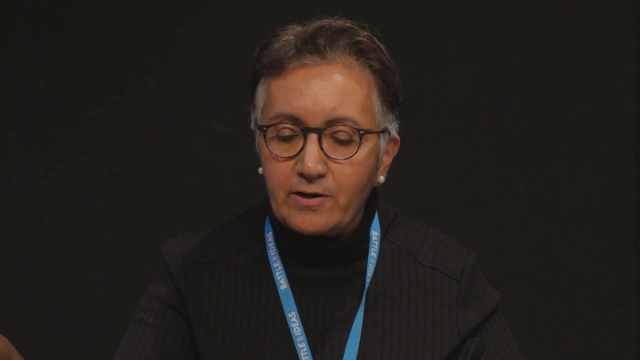 that will somehow redress that, this lack. And I, you see, I think you know to a certain I agree, if you like, with that description of the problem. I do think a lot of education is rather desiccated and technical and instrumental, and there is not enough time for those things. 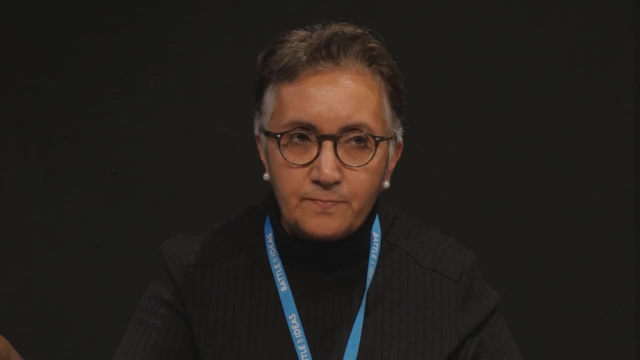 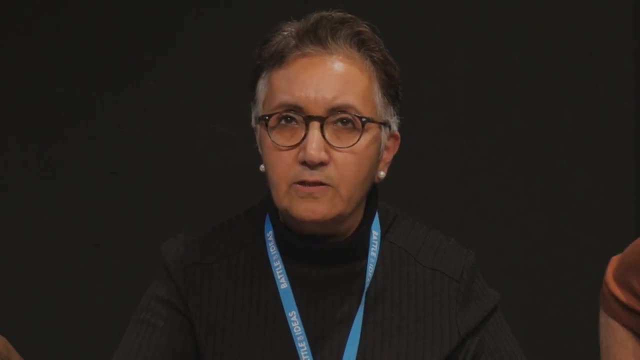 having been really hollowed out and reduced to its most kind of empirical aspects. I I actually think all of the things that the speakers have said- the questioning, the discussing, the hypothetical questions- are things that actually should be done in the subjects and 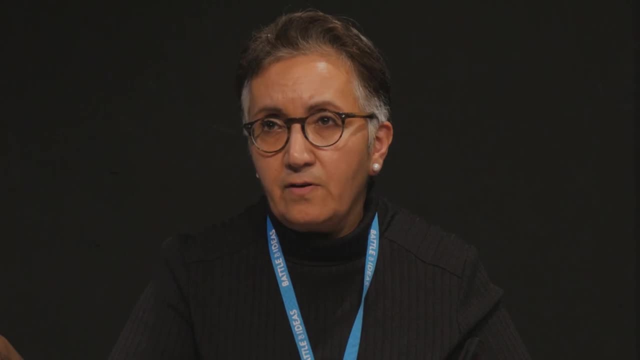 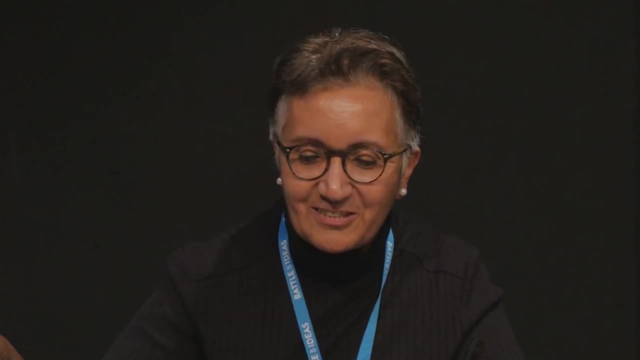 through the subjects. You know what if? what if King? what if Shakespeare's version of Richard the Third? what if he? you know he didn't actually have a hunchback. You know, look at historical records. You can have a perfectly interesting and fairly wide-ranging discussion. 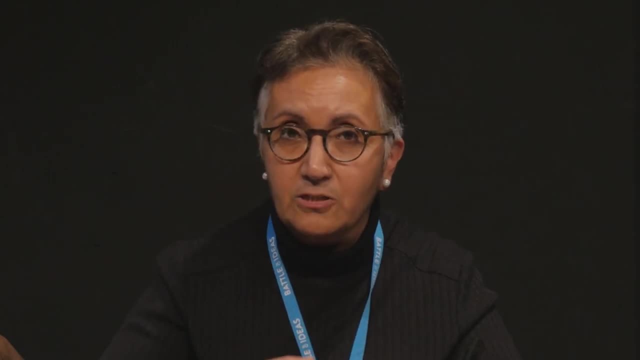 with history and where they're gaining subject knowledge as well and being introduced into a very specific formal language and criteria. you know conceptual criteria, that's germane to that subject. Likewise with with English literature. You know the idea of questioning and giving. 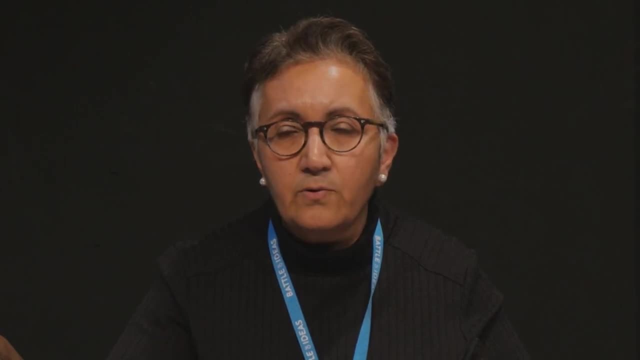 reasons is: is has traditionally been done in the form of, you know, the, the, the, the, the, the, the. you know fairly lever-sight, close reading of the text and asking children questions on that. 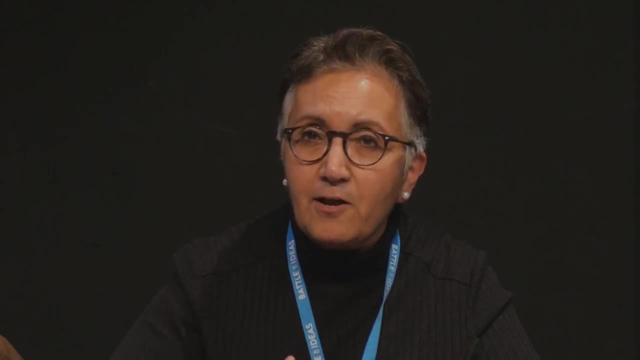 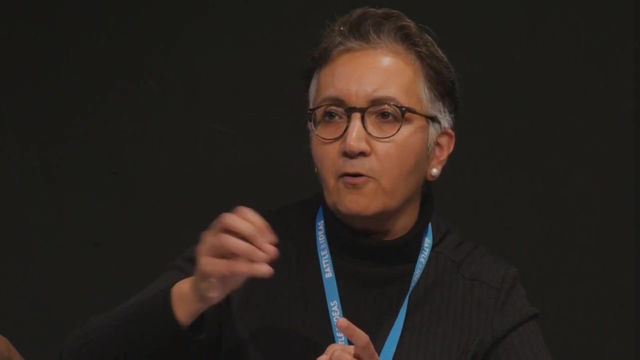 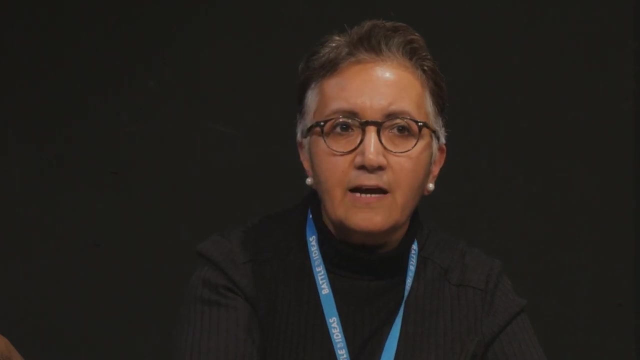 So, and I think that that is in there, there is a big problem because philosophy for education sidesteps that. Yeah it. you know it's sort of responding to this problem of there not being enough discussion because the subjects have been hollowed out and not tackling that, Not tackling. 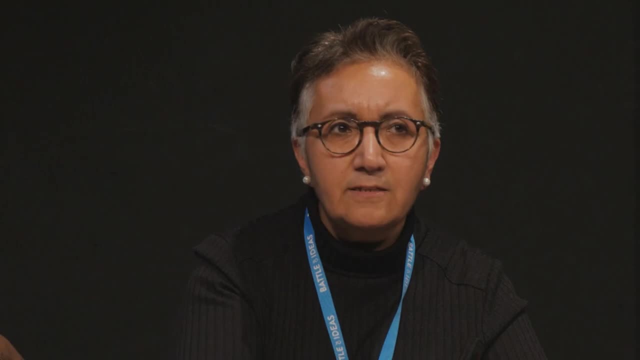 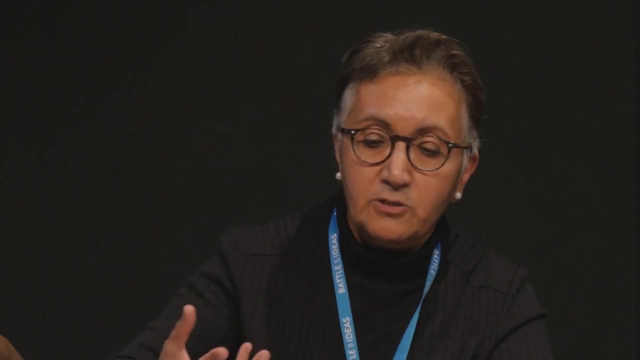 well, why are the why? why has knowledge been seen like this? Why does it? why do feel unconfident of you know, in being assertive or authoritative in teaching their subjects in, for example, a didactic way that they might need to sometimes, as 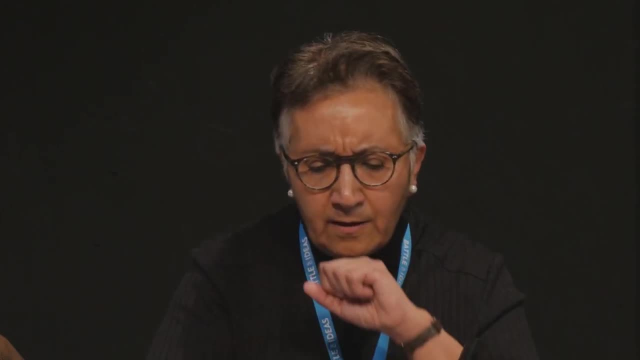 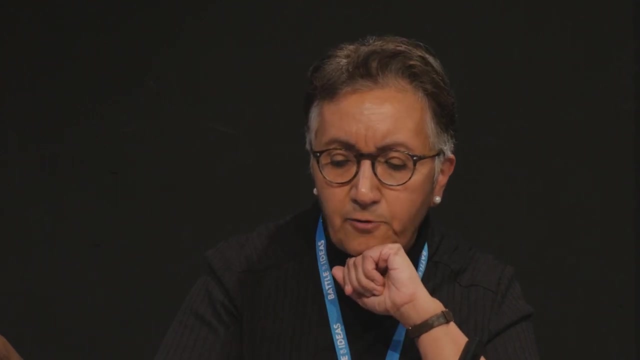 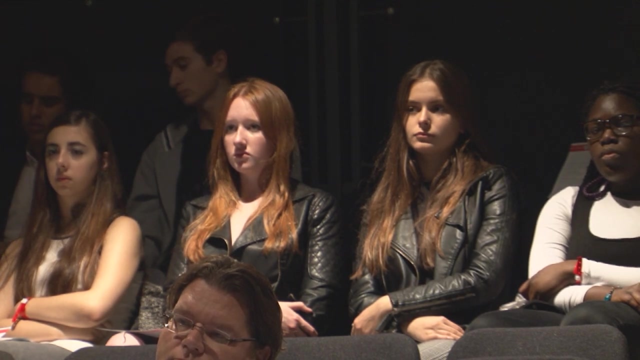 well as having the conversations. so, in other words, I think it's a correct description but a kind of wrong attribution of the cause, and I think it avoids tackling the problem of creating better ideas around knowledge and how that knowledge can be made into school knowledge. you know, in doing that kind of 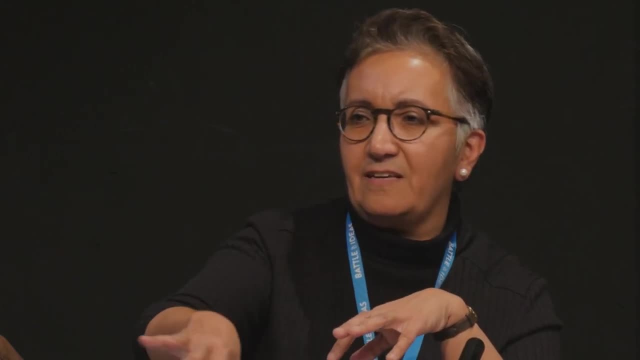 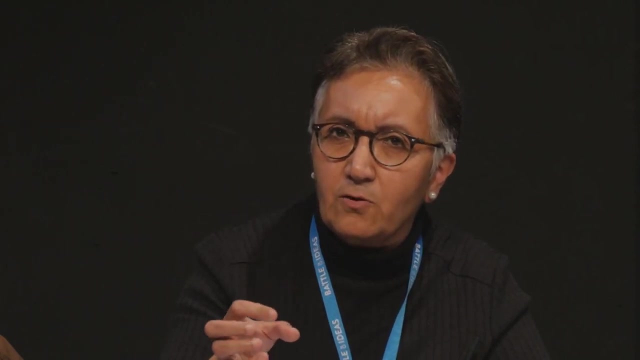 entrenches this idea of: oh well, you know, those are the subjects, that that's the knowledge you're doing your subjects. but here, this is the really philosophy is where it all happens, and philosophy without that subject knowledge, I think, becomes something quite trivial actually, and I'm going to come on to that in a 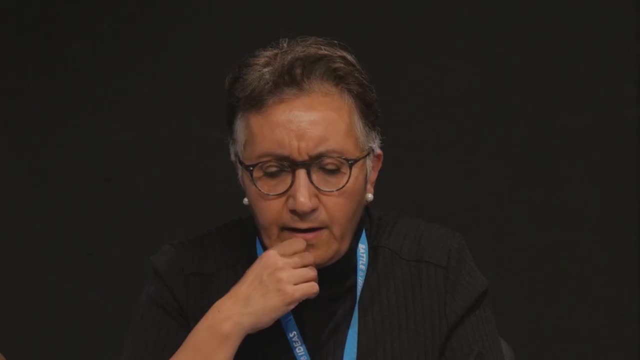 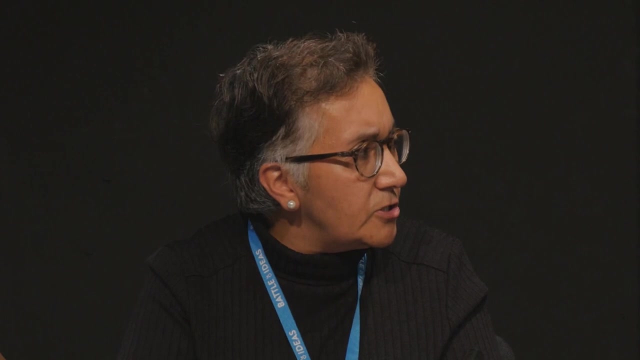 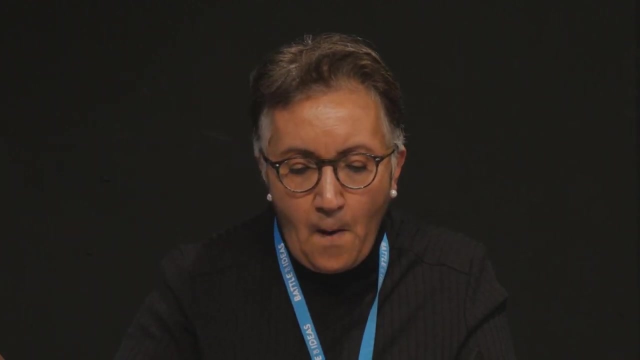 minute. can they do philosophy? and I have to say that I don't think they can. I really don't think they can. Catherine, I take your point about. you know your issue with them. you know mental and cognitive development doesn't run a long, the same lines as physical development, for example- but I think you 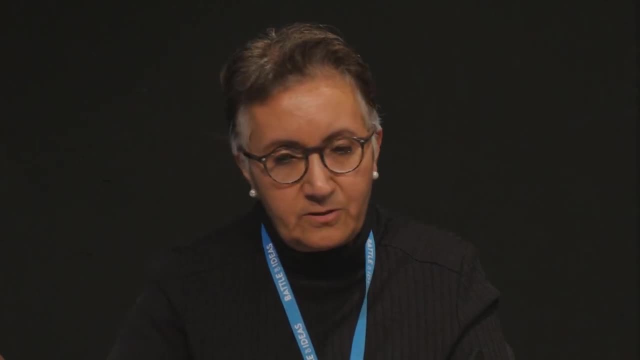 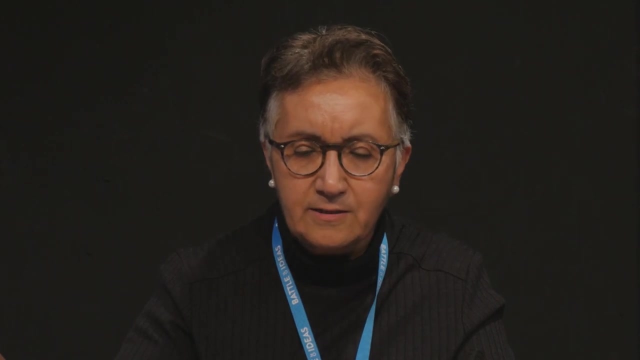 know, for me, whatever methods you use in philosophy, for me I would say it is fundamentally about a search for truth. it's about the truth of up ourselves, how we stand with the objective world, what reality is in our place in reality. those are quite big things and children are not removed from that. obviously they are. 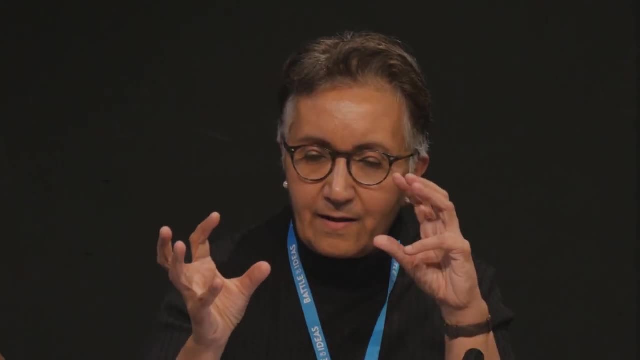 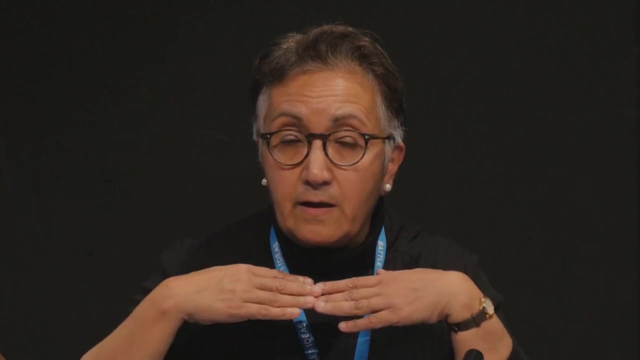 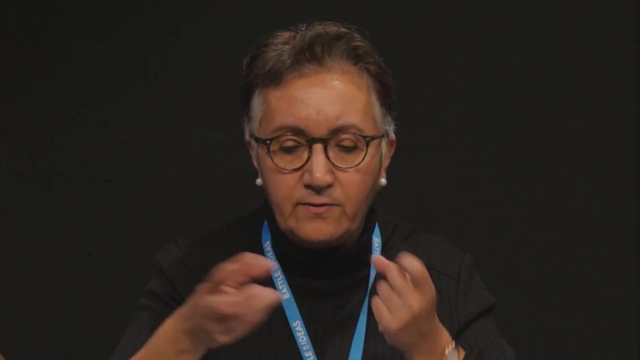 part of reality, but- but I think that's a good point, and I think it's a good point. I think the the actual what it requires as philosophy are two things: it requires an experience, if you like, experience, but it also requires a very abstract, formal thinking, and it's a constant move between the two, between subjecting, the 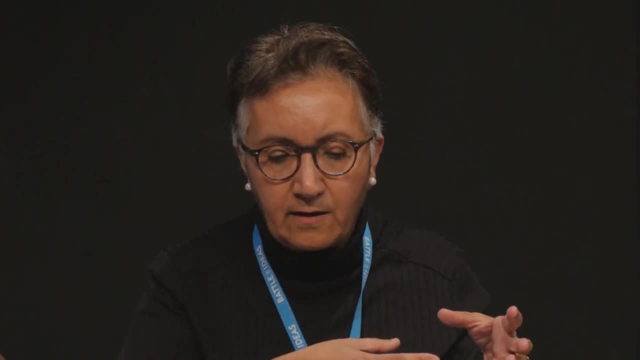 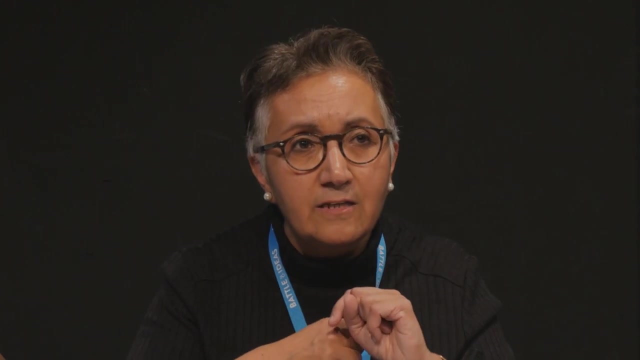 claims of experience to the claims of your theoretical understanding, and I think that takes quite a long time to do. and I think, more importantly, this is why children can't do. it is as a society we have a thing called childhood, and that is a big cultural achievement: the creation of 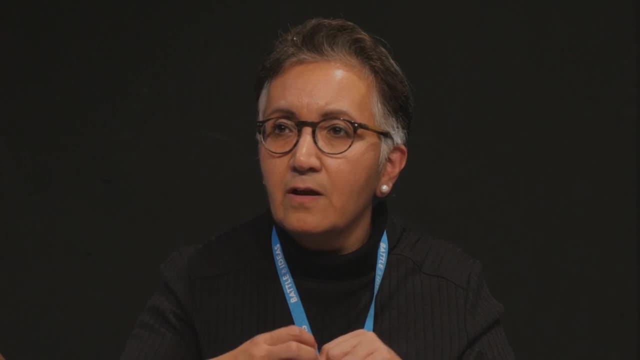 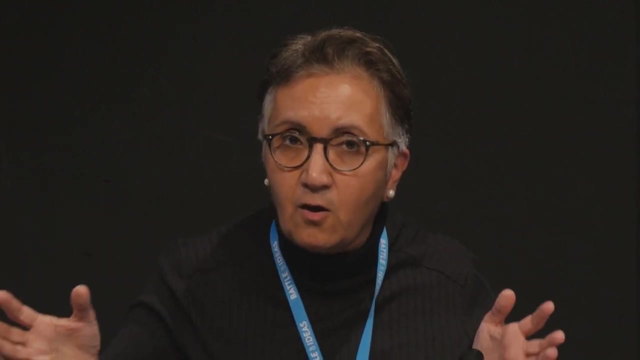 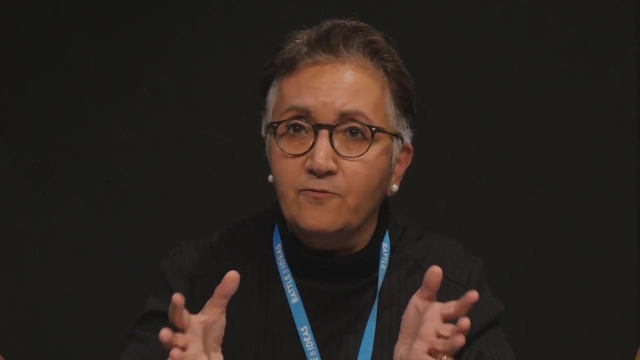 childhood and a space and a time where children, their experience socially, is limited. we do not say, yes, it's okay for seven-year-olds to go out and have sex or fight wars or do all things that adults might be required to do. so their experience is necessarily limited for good reasons, de facto. that's going to me. 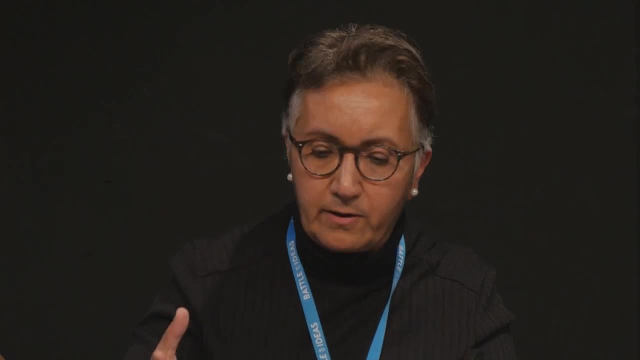 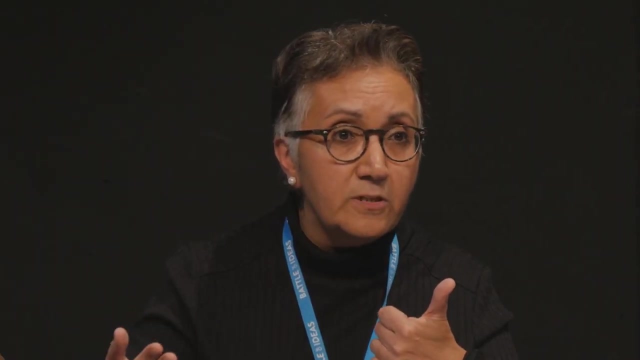 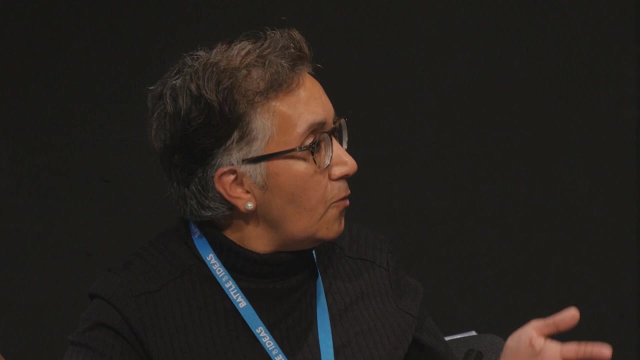 their ability to do philosophy in the way I've described is also going to be limited, and I also think there's a real danger of philosophy being trivialized. you know, I've heard somebody say the thought experiment in P4C is: does a smurf turn blue when you strangle it? and secondly, I think it's conform. I think 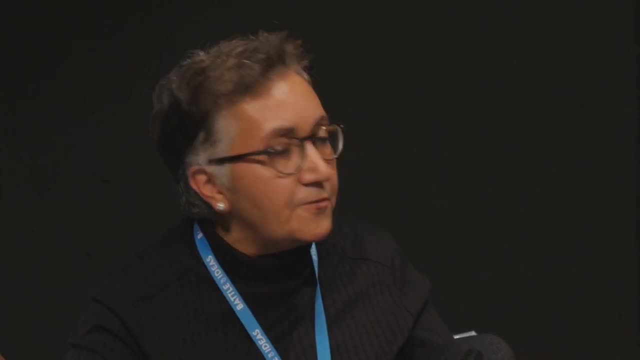 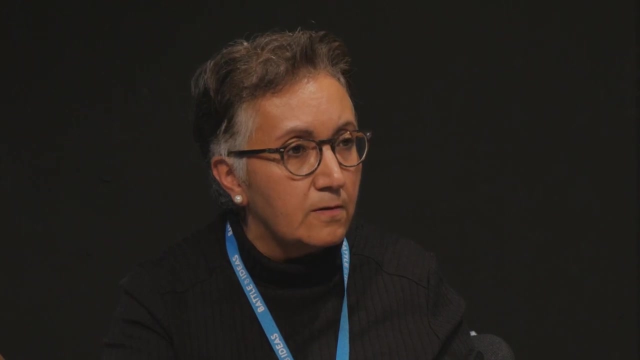 there's a danger of conformism and, Katherine, you know your point about the FGM is, I think, really important because I'm sure you think, and other people might think you're- you're trying to get individuals to be critical and maybe an older point, at older level, that might be the case. you need an awful lot of factual knowledge as well. 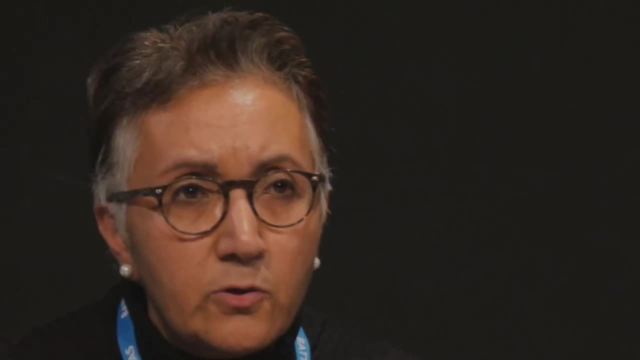 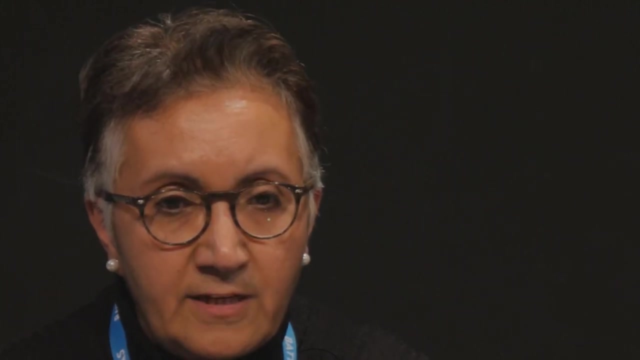 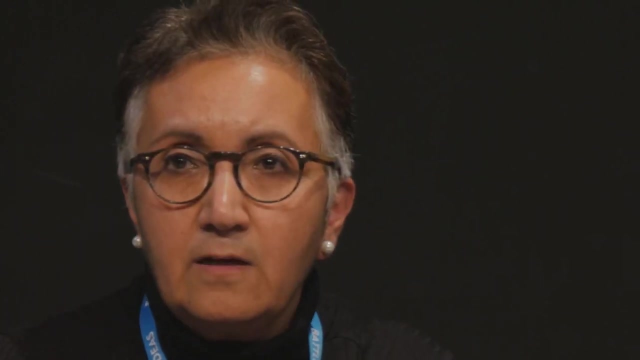 numbers and figures. you need empirical knowledge. you do it at a younger age. what you're doing is just incur your, your think you're doing that. what you're actually doing is reinforcing the idea that a problem that has been is controversial and contested in the adult world. you're introducing it de facto as 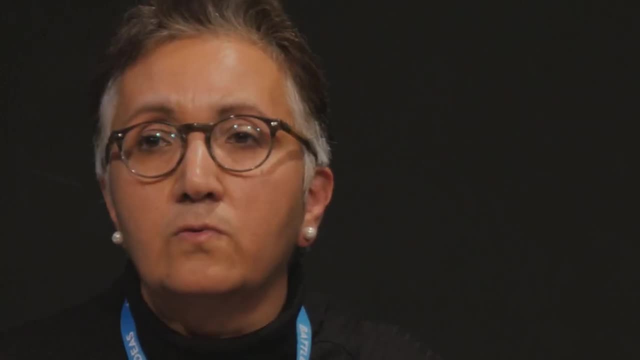 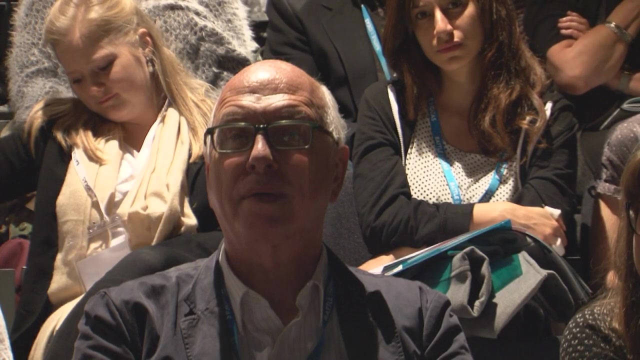 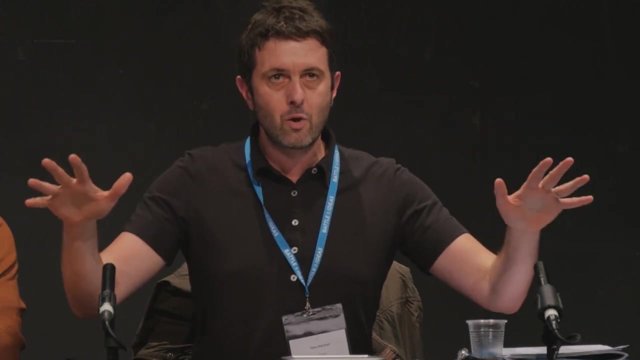 if it were an actual thing, into, into school, into schools, and they do not have the knowledge or the capacity to truly be critical of that. okay, I'm going to hold our panel back for a second. okay, so you just have to pause and I am going to go out to the audience. I'm not. 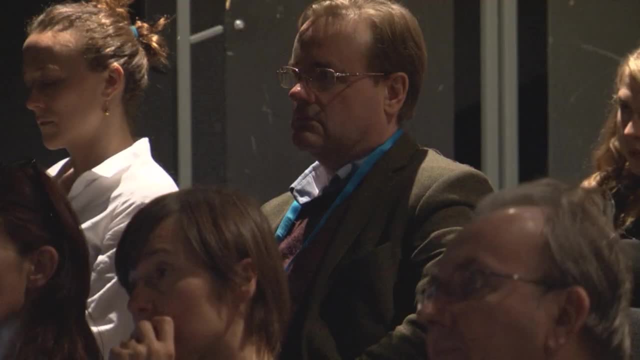 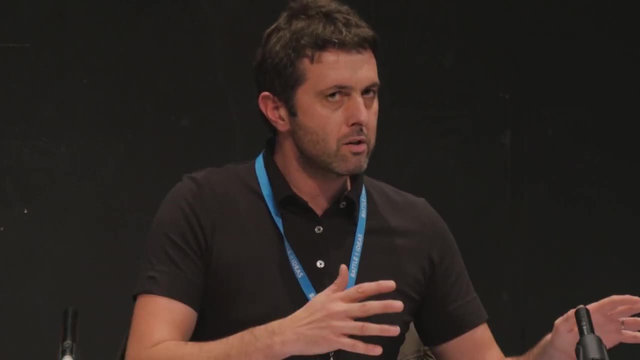 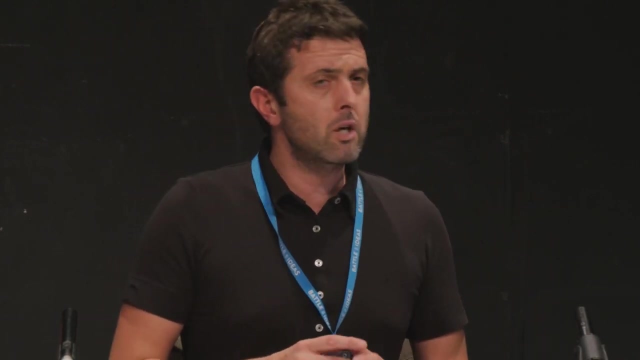 a philosopher and I don't want anyone to feel that there's any question beneath our panel, so everybody should, because there is a sort of mystique around philosophy which I think we need to sort of set aside, okay, so it strikes me that this is both a philosophical discussion, but this is also a discussion about 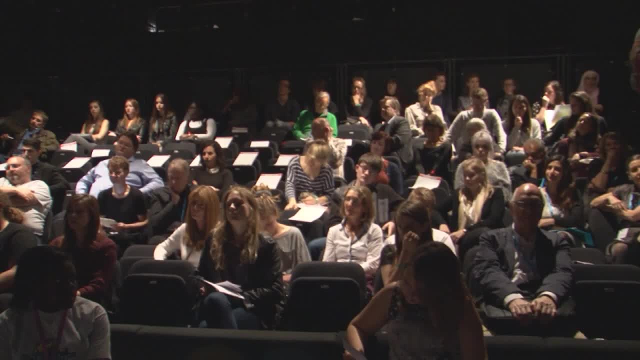 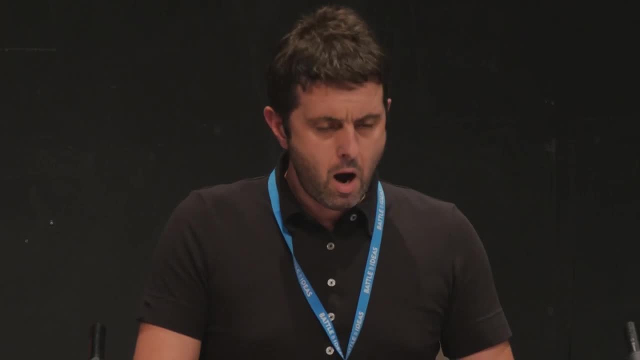 education and about the curriculum, so everybody should have a chance to contribute to this, and two things that seem important to me, but by all means take it in a different direction. if that's where you want to go. what I would like to know is: what is the special claim that is being made of philosophy? 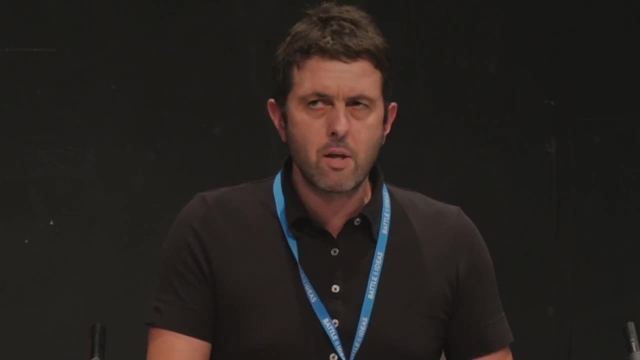 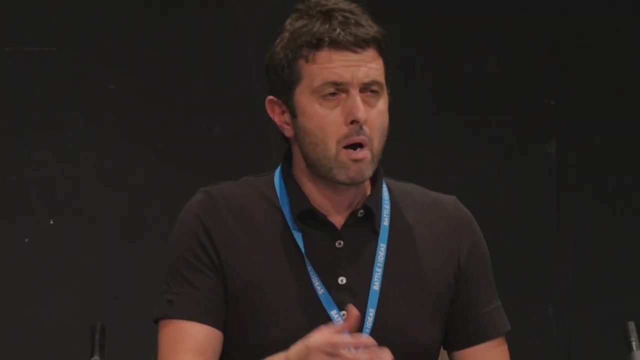 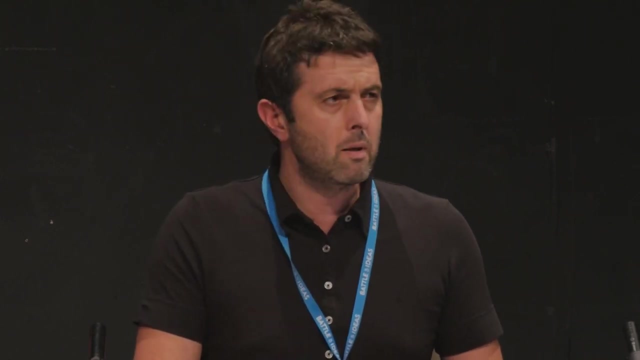 in comparison to other subjects. there are many things that are worth knowing and there are many subjects that are worth studying. my PhD is in sociology. that might be something that is worth studying in school. history is important, English is important. art is important. there are many important subjects that 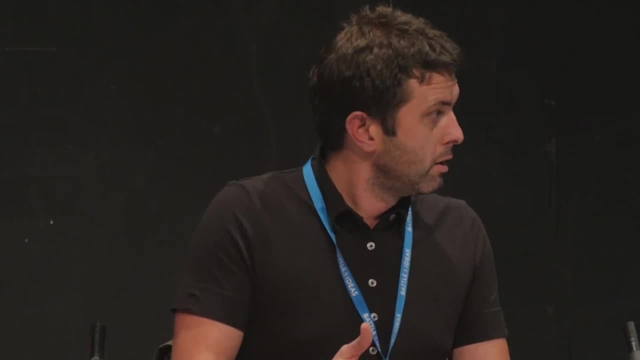 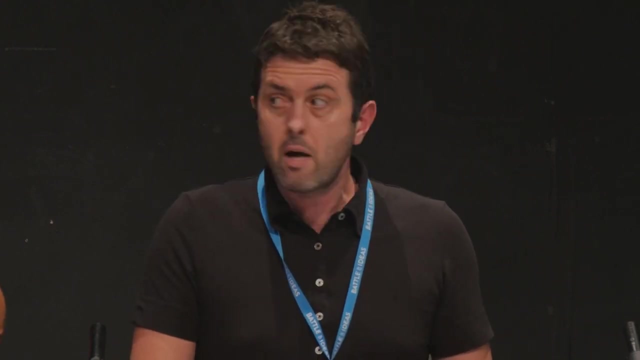 we can learn from, and I think that's quite the same for me, and I would say that the only thing that I would be interested in is the question of what is the answer to this question. so I think that's a question that I would like to. 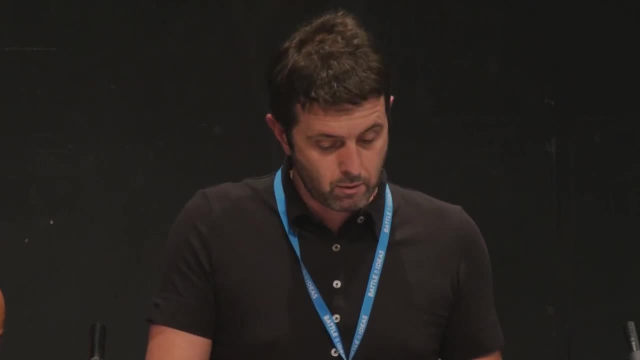 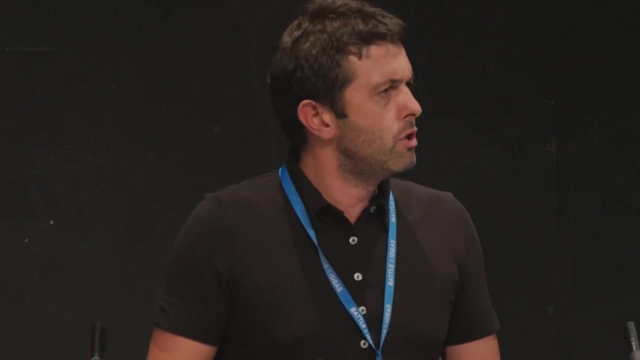 ask myself- and I don't want to give you an answer to the question, but I would like to ask myself: why do we choose one subject over another? there is an infinite time in the school curriculum and other subjects have a claim on that time. so I think that's an interesting thing for us to kick around a bit. but I 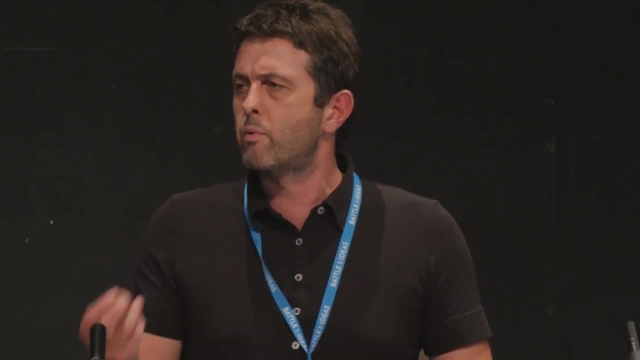 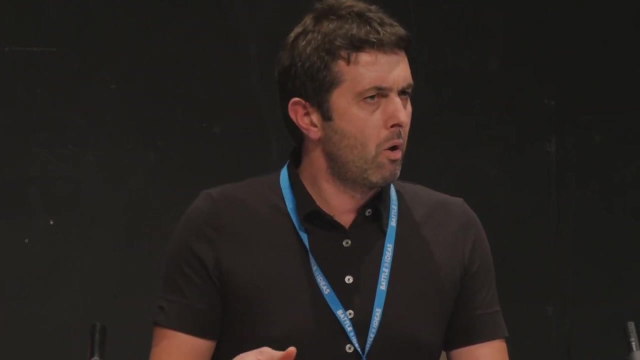 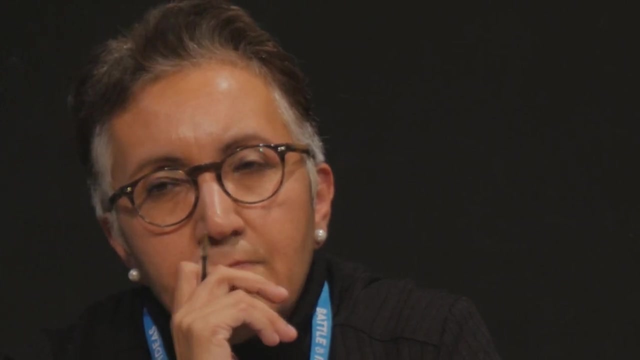 suppose maybe this is the same question in another way enables people such as myself who are not philosophers to assess the claim that is being made on curriculum time by this subject. Okay, so over to anybody to make points. I'm very much in favour of children using creative thinking and problem-solving techniques. 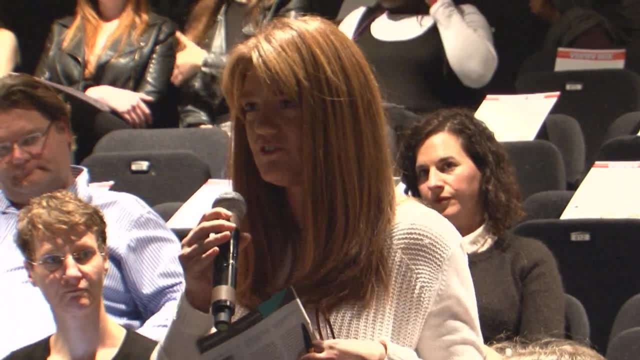 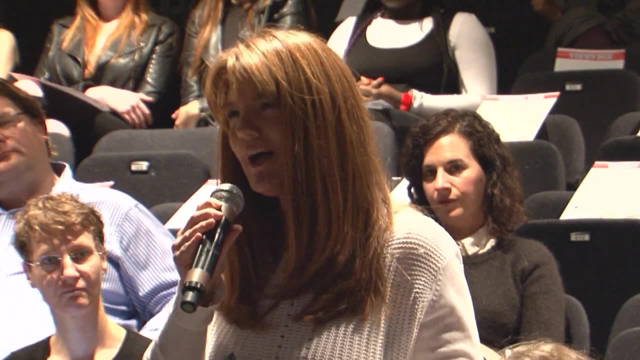 and so I was very curious about this subject, as to whether or not, having done a philosophy undergraduate degree myself, whether or not, how I would feel after this discussion. I was with you for a while, Catherine, and then you mentioned FGM. 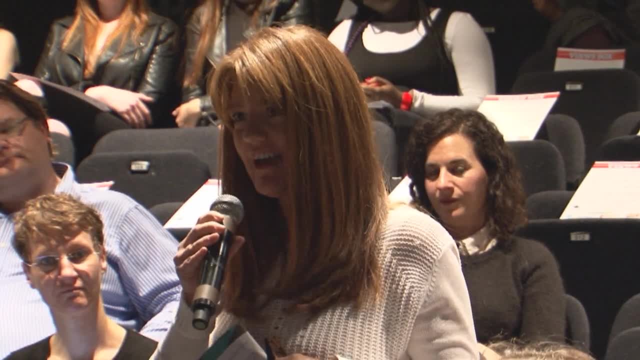 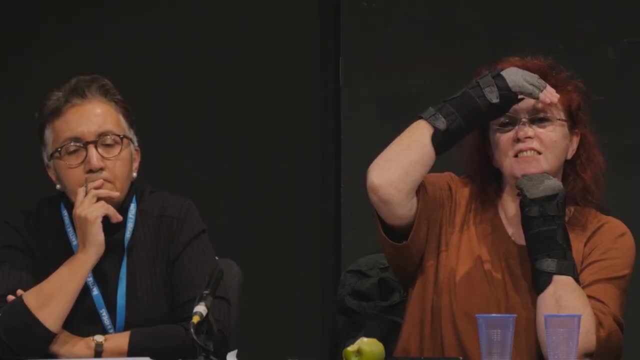 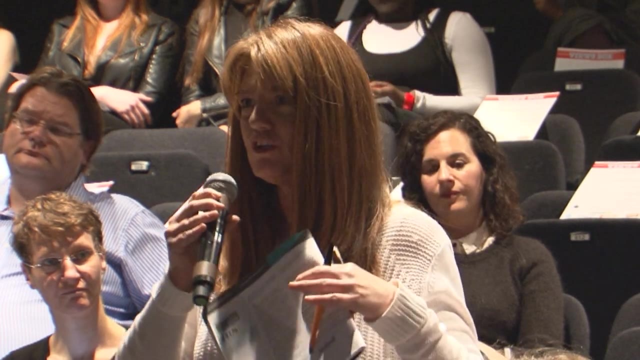 Philosophers have always asked the questions that they ask within a certain historical context, so Plato wasn't talking about FGM. It's very much a question that we ask of ourselves. today. It doesn't happen so much in the West, so we have a very definite ethical, cultural. 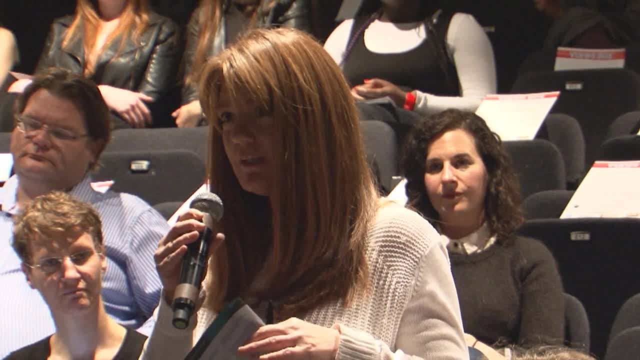 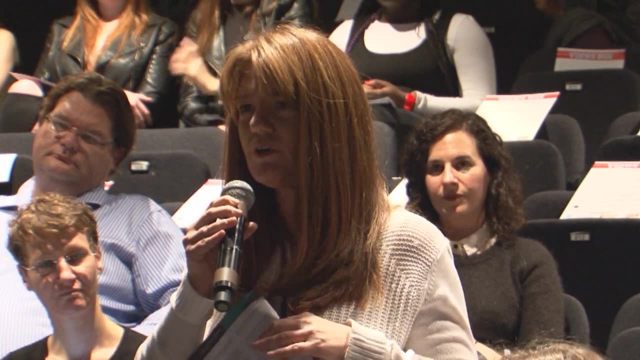 response to that, If you're talking to young people- and I'm imagining we don't talk about FGM with five-year-olds- but even if you're talking with 12-, 13- and 14-year-olds about it. the first question: 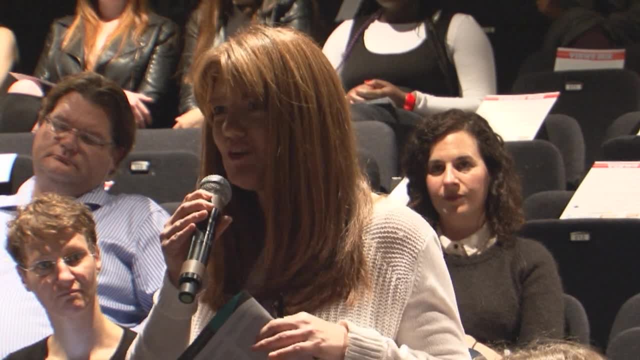 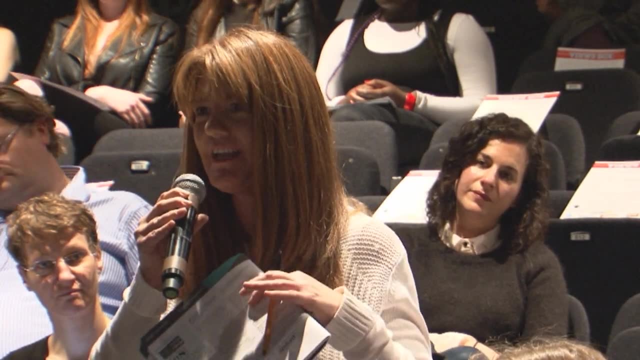 is what is mutilation? I'm sure lots of young people know what mutilation is from video games and all the rest of it, but it's a word that may not be familiar to everyone, so automatically you are now setting an ethical framework for that question, because mutilation has negative consequences. 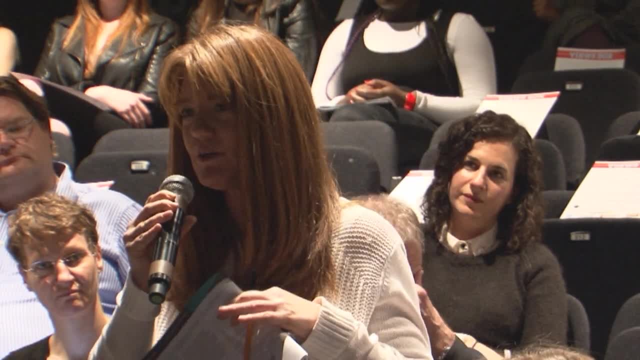 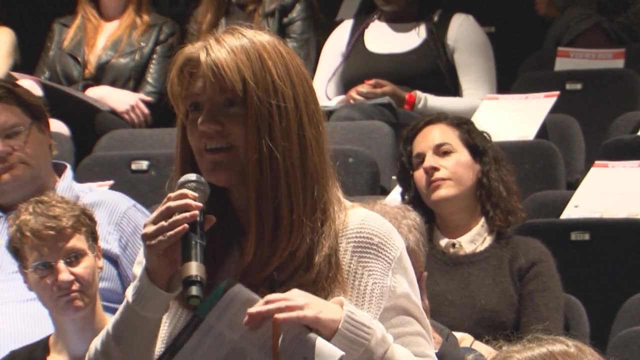 Now I'm not saying I agree with FGM, but I'm saying that the context in which those questions are being asked are very culturally and socially and historically embedded. The second thing it reminded me of is that, in terms of philosophical branches, ethics, 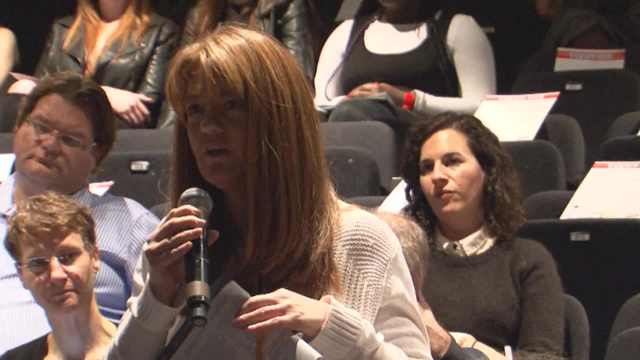 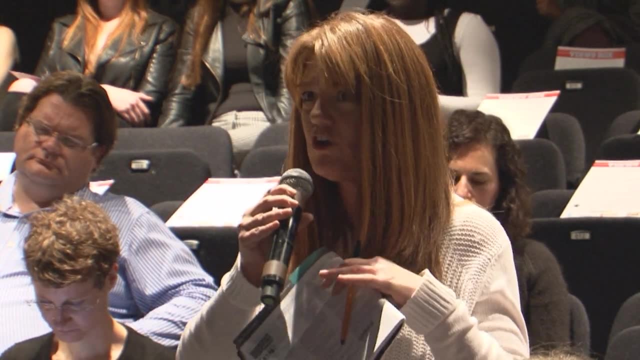 is the one that we tend to talk about with children. It's what children are interested in, not what is truth, but what is good and what is bad. And don't you think that by teaching children who have not had the experience that the last 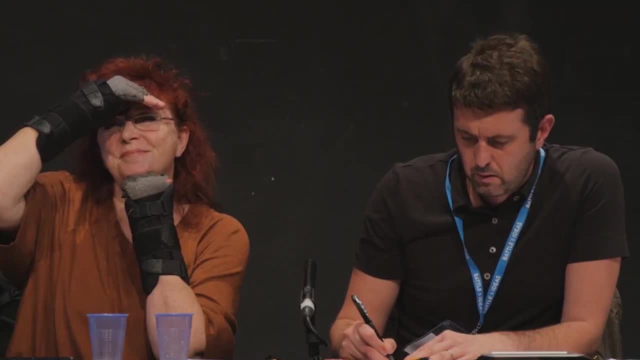 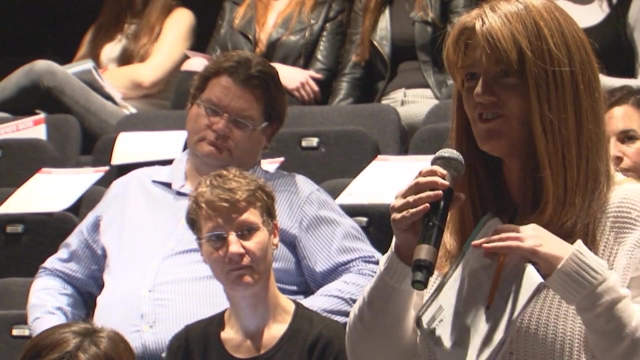 speaker talked about, in terms of war and sex and adult experiences, that in actual fact, what's happening is that children are being kind of taught to think about philosophical questions within the dominant ideology of the time. Thanks, Okay, that's a very interesting point. 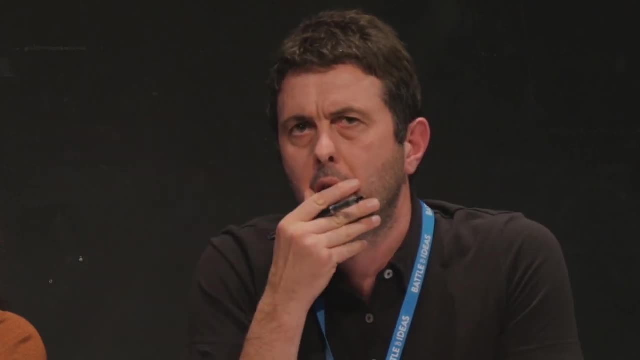 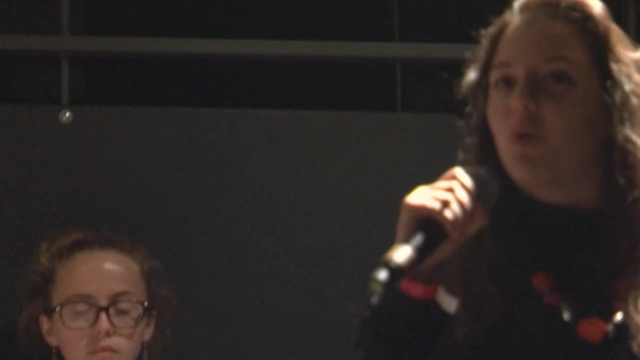 Okay, there's a couple of questions up there at the back. I'd just like to pick up on that childhood point. What about the idea that our young people have to grow up a lot quicker than they would have had to in past years? in today's society, 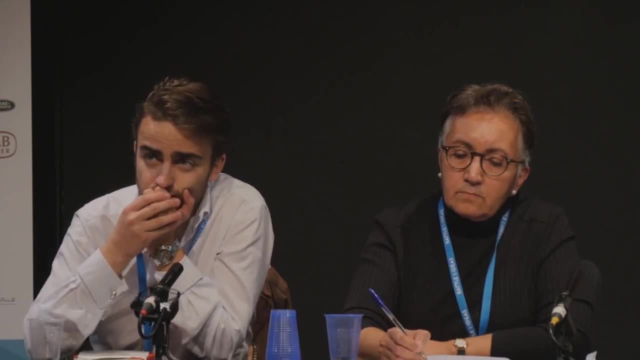 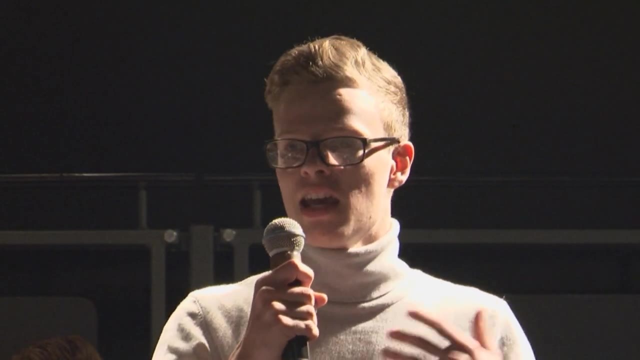 Okay, it's very interesting. When I was very young, my mother passed away, And when she did, I was thinking about myself. I thought about the big questions: What does it mean to be alive? What does it mean to What does death essentially mean? 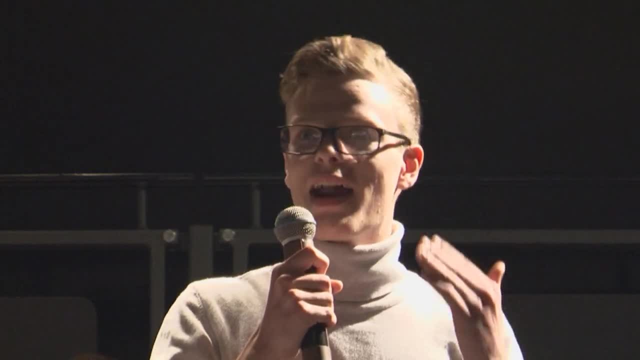 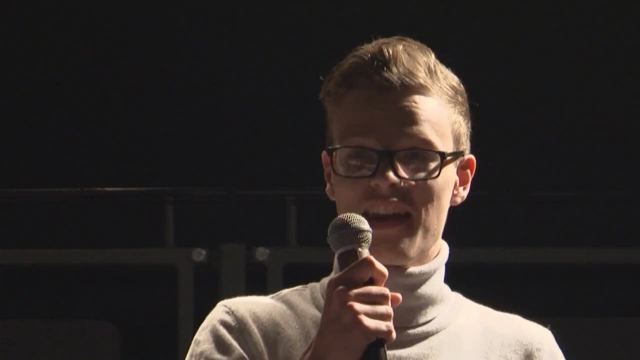 What happens when we die. So I'm thinking I can't physically comprehend how you can say that children can't do philosophy, Because I was seven years old at the time And I was thinking these sort of ideas. So I can't understand how you can say that children can't do philosophy when I clearly 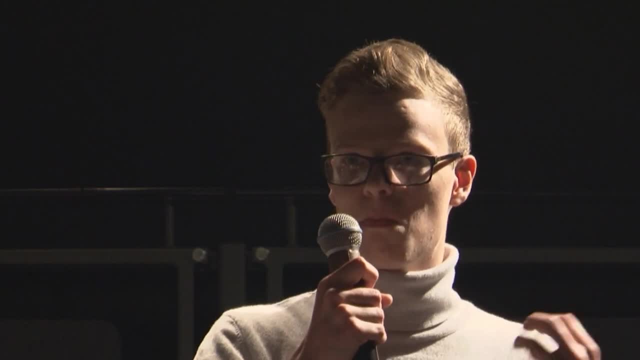 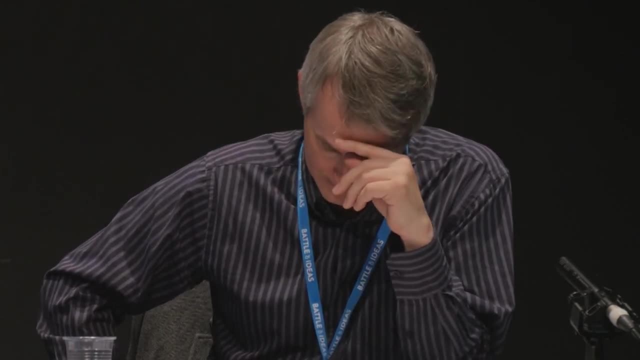 was doing some sort of thinking towards myself and what it means to be me. Okay, thank you. I love philosophy. I'm doing an A-level in philosophy and ethics And I want to teach philosophy to secondary school students and young people of all ages. 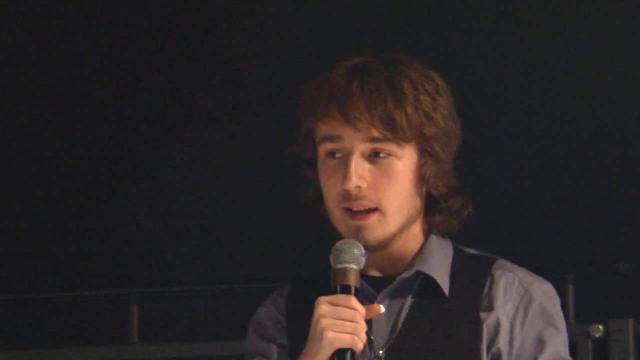 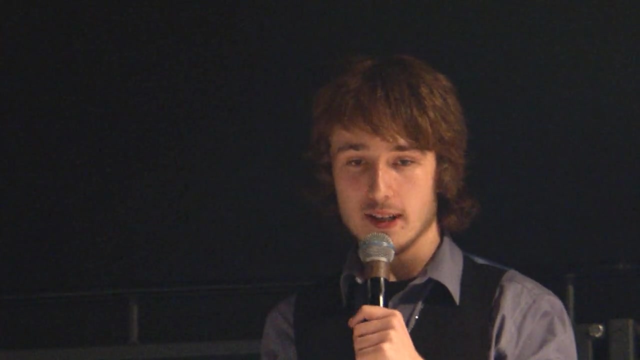 Because I feel passionate about this, Because I feel like it's incredibly important that children are given the opportunity to do philosophy, Because I feel like they have the potential to be very good at it, And obviously that's an Aristotelian idea- potentiality and actuality- and whether they 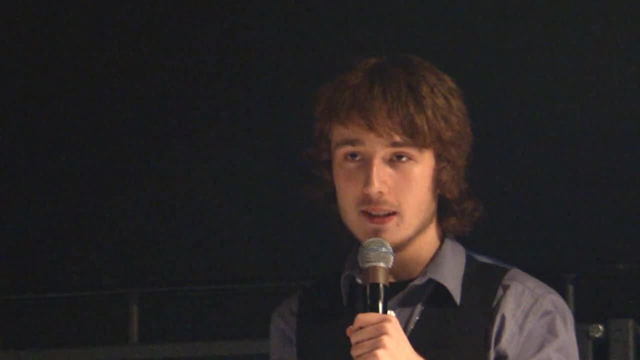 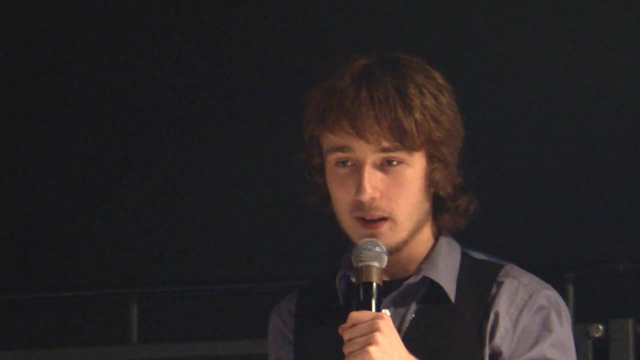 will actually be able to do it, But they need to be given the opportunity Because in this world that we live in at the moment, we have incredible amounts of horrendous problems And I think that people don't ask enough questions. And I think if we can get people to ask questions from an early age, it becomes natural to them. 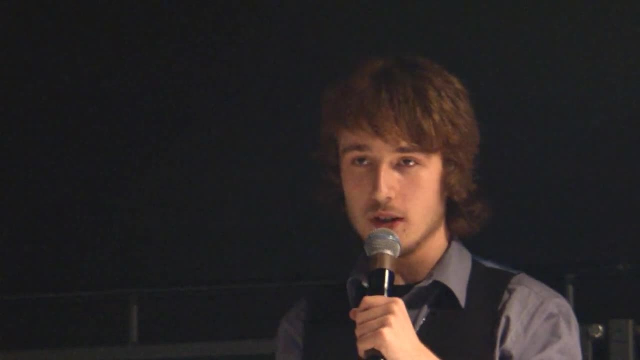 They won't be afraid when they're older. There's probably a very good reason why we don't allow people to ask questions: Because the establishment doesn't like being challenged, But I think we need to get that idea out the window, Because we're not going to get out of the situation we're in in the world at the moment. 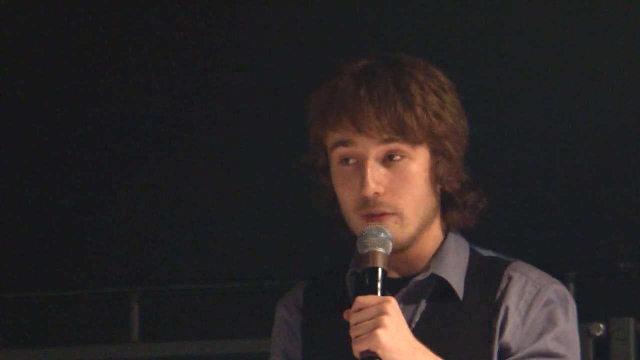 if we don't encourage people to ask questions. Well, I think that's a good point, Thank you. Thank you. Whether they'll be good at it, whether it will actually be very philosophical of them, that doesn't matter. We need to give people the opportunity. 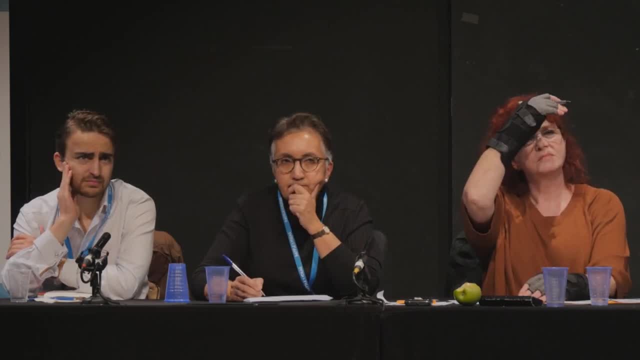 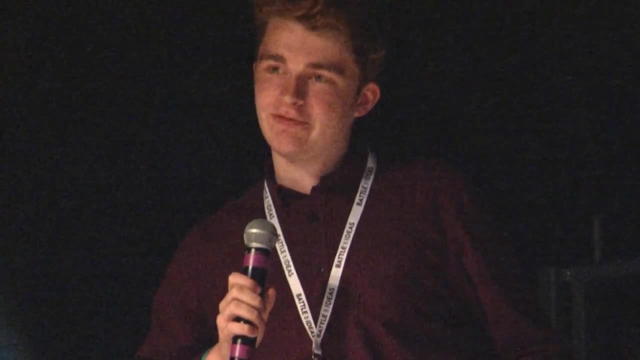 I'd just like to start off by saying that to some people here I would still be considered a child. I'm turning 17 in like a couple of months, so I think this is quite a relevant point to me, And I'm obviously interested in philosophy because I'm here. but my interest in philosophy 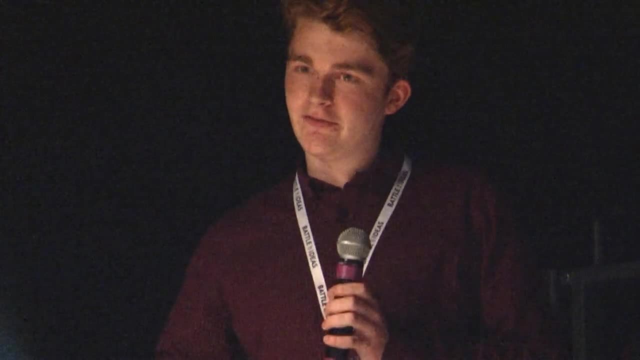 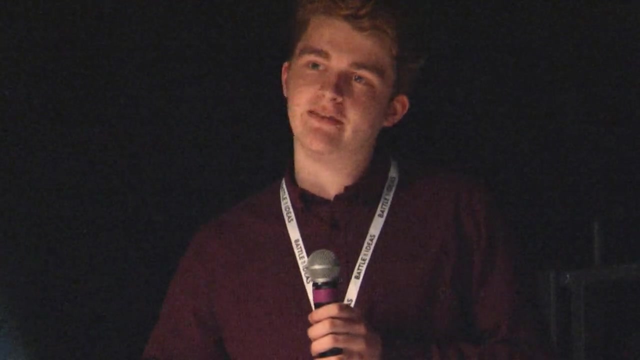 was cultivated when I was about 11, 12 in my religious studies classes at school when we started talking about things like the death sentence and that side of things- not necessarily all the argument- So a lot of our discussions in class came into philosophy. 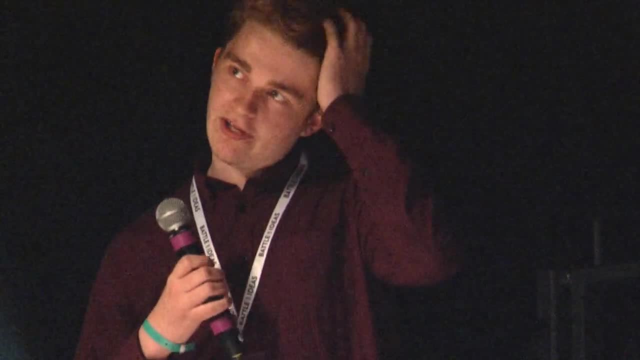 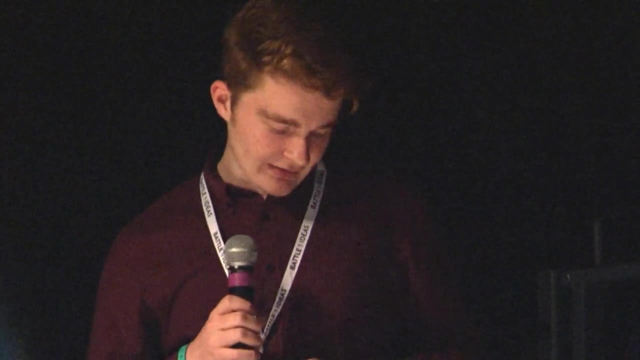 And I found the same when I was doing English literature when we started talking about Shakespeare and a lot of his plays focused on human nature and the philosophy side of things in there, and I think that in a lot of the subjects that children do at school 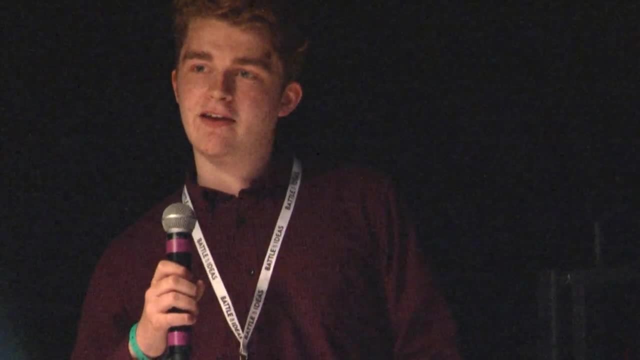 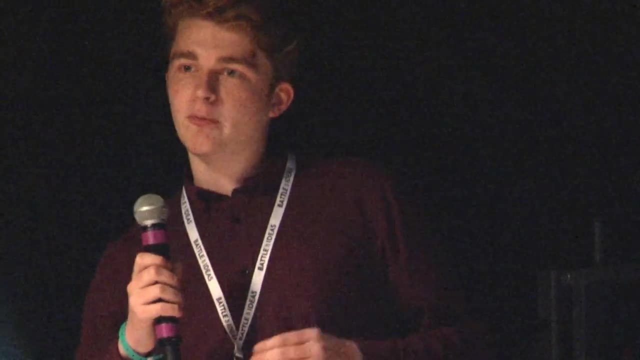 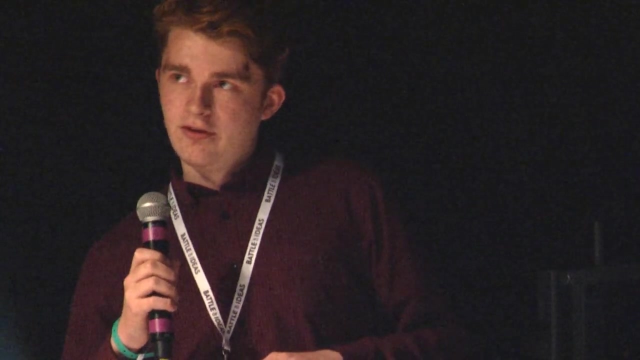 already touch slightly on philosophy and they touched in the very basic areas and they almost act as introductory lessons. And I think it's the point that Harker touched on but nobody else really thought about was that. And introducing philosophy in school in a subject like for young children, it takes it out of those other lessons. 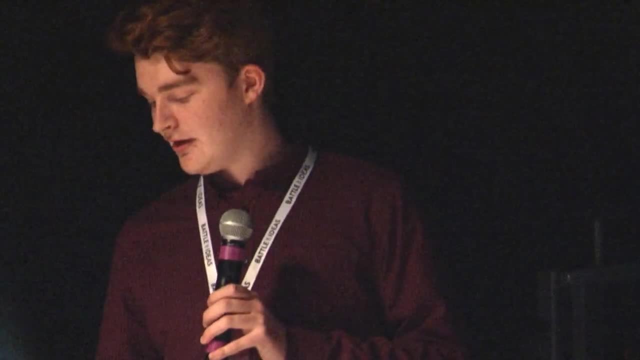 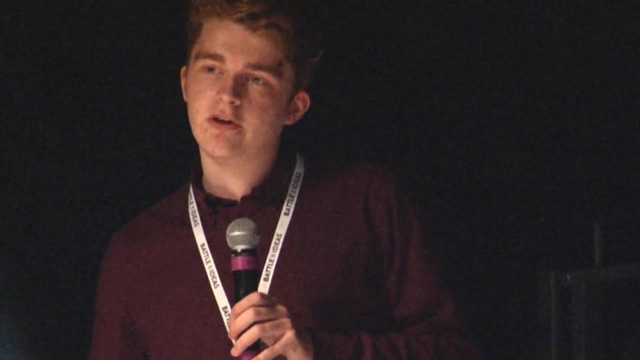 And I don't think we really need it, because she also mentioned childhood and a lot of the issues that people focus on in philosophy, Just like a lot of issues that people focus on in religious studies later on. They're quite traumatizing to some. 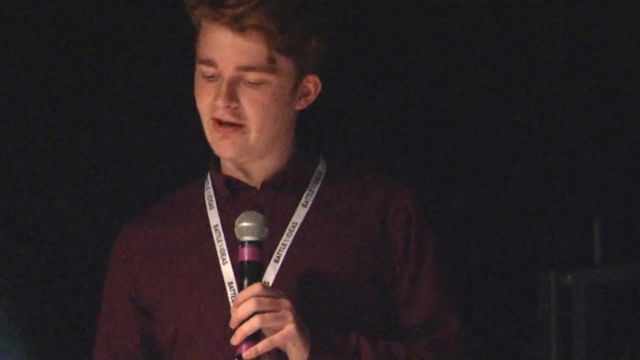 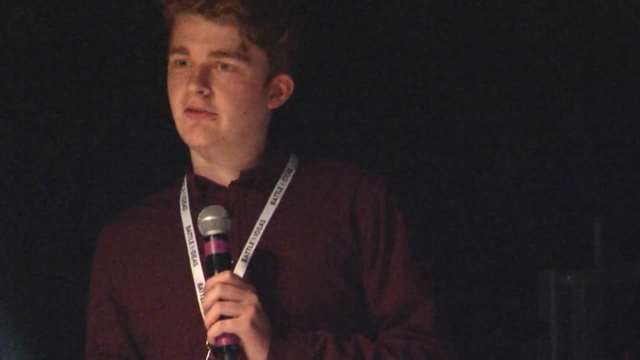 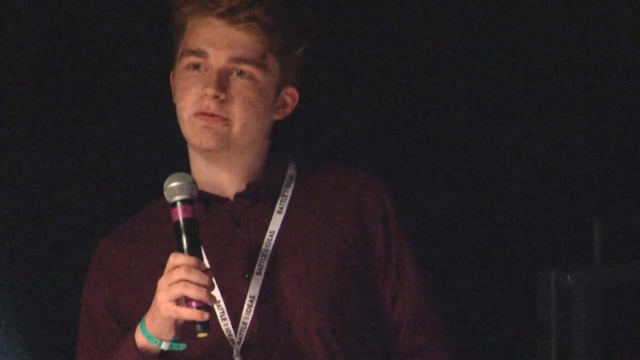 They're quite deep, that require a lot of just general life experience And I question whether you lot think that the introduction that you get in an English literature or a religious studies lesson is enough for a child from the age from 12 to 16, until choosing philosophy becomes an actual option. 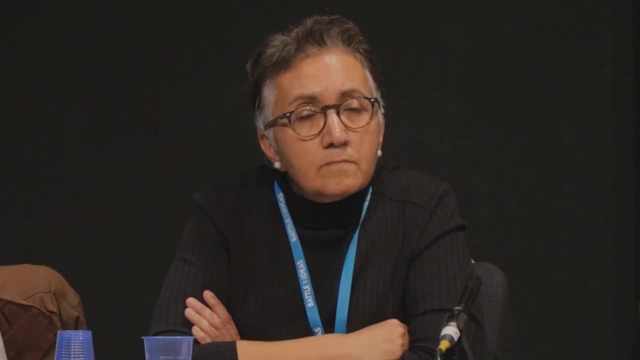 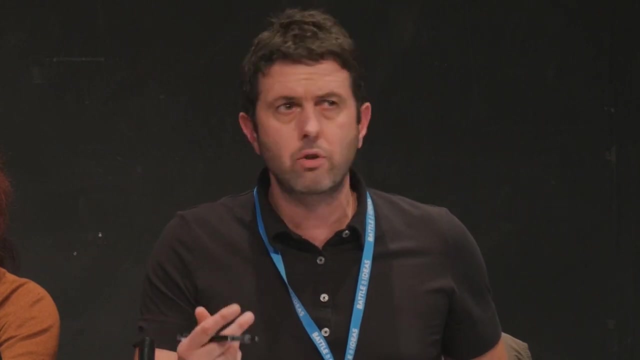 And if you don't think it's enough, why I'm going to bring the panel back in. just to recap, We've got a lot on the table. We don't feel that you need to come to all of these. We've got a question of indoctrination. 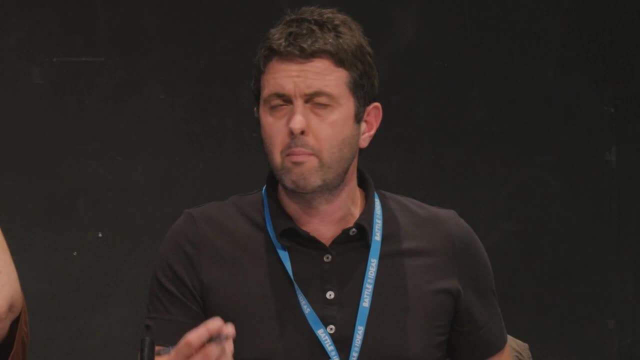 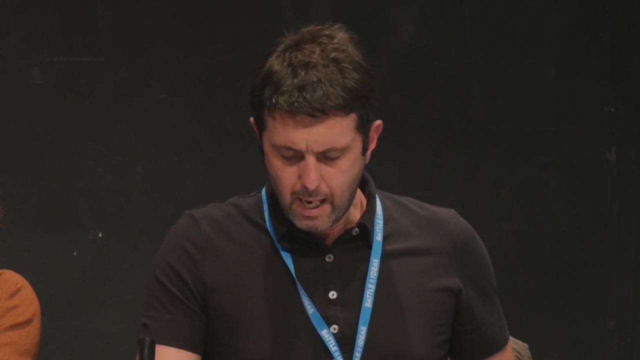 How do we involve, avoid indoctrination? Are young people growing up quicker now and therefore need The critical skills of reasoning that philosophy might offer them, And I'm interested. There's a very important debate here about, I think, knowledge and skepticism, and education. 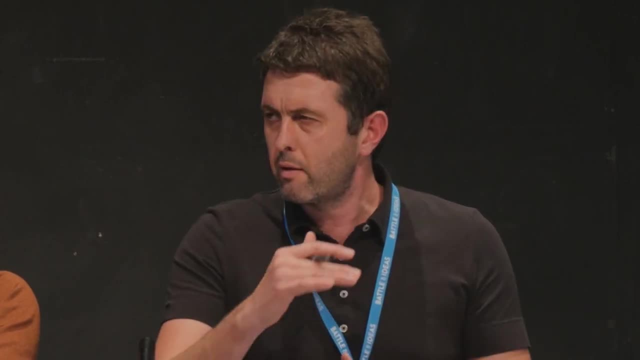 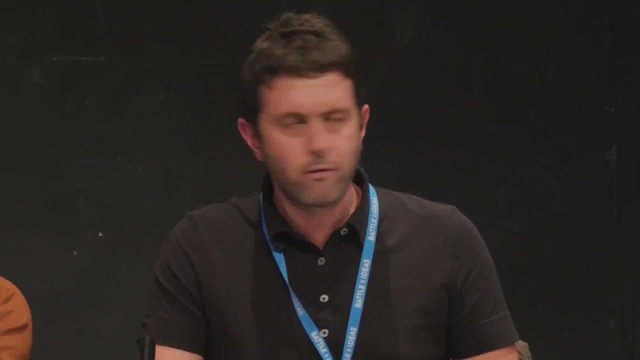 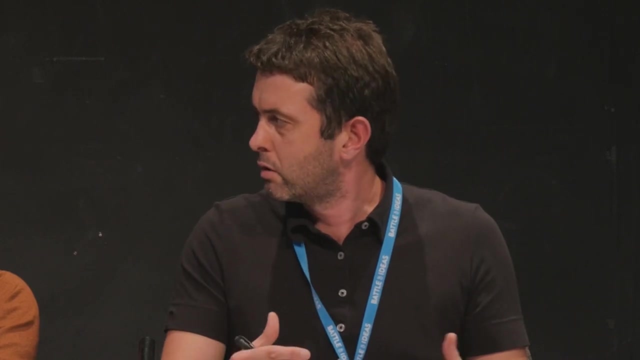 And you know in part, do we want to differentiate different levels of education? I mean, do we want five year olds to be skeptical? Would that be a healthy thing? I mean, I'm not a philosopher but you know, is there an issue here about settled knowledge and, you know, actually getting in some substantive knowledge of the world? 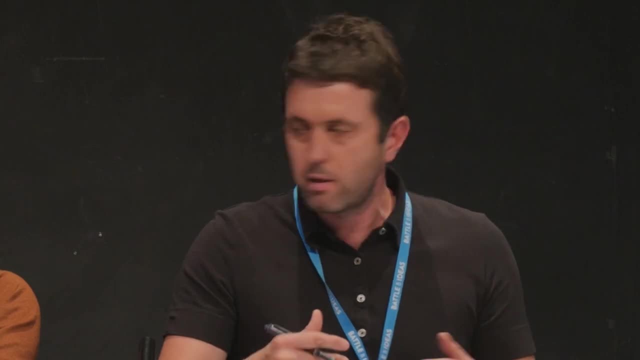 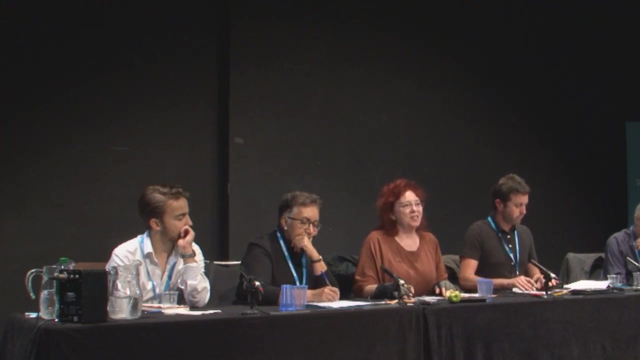 And you know, When we introduce that level of questioning and skepticism, you know when would that be appropriate. Catherine, feel free to come back on anything. OK, thank you. There's a couple of things I would like to sort of clarify. 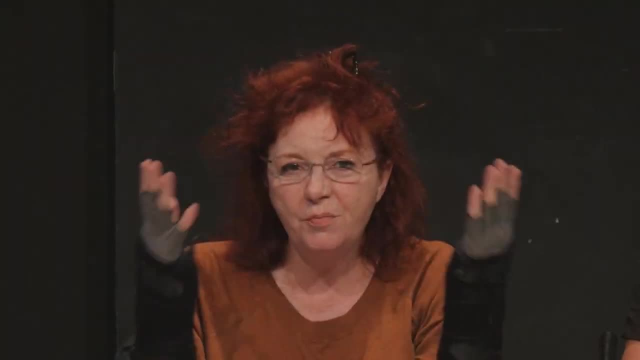 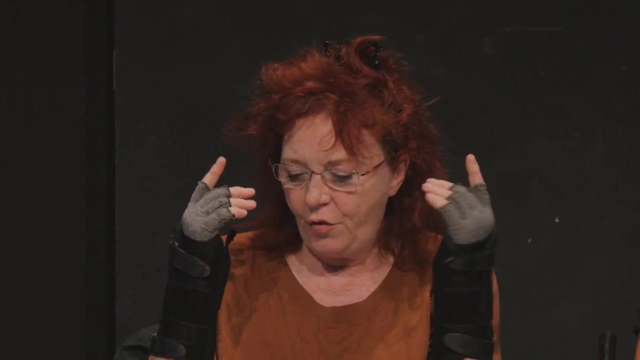 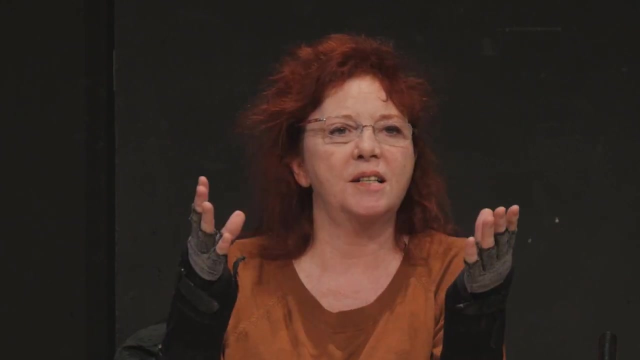 And, as usual, I'm really speaking for the practice that I've been doing for 40 years, not other practices that might not be the same. So, but first of all, we never introduce a topic. So when I give the example of FGM as a topic, 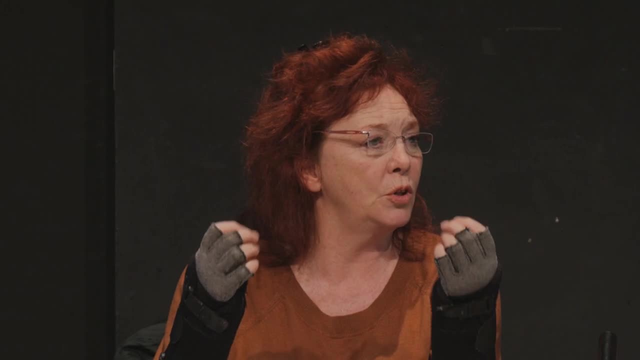 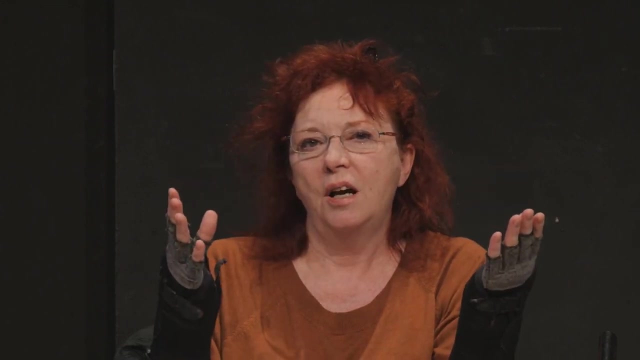 That might arise. it arises from the children or the young people or the adults, because we start with their questions, So I'm never introducing anything. I will go. you can't prepare for this because you don't know what topic is going to come up. 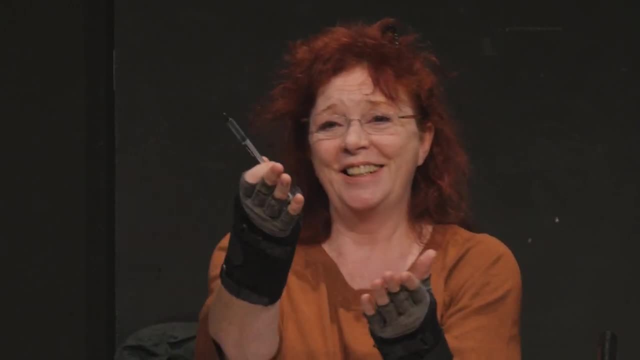 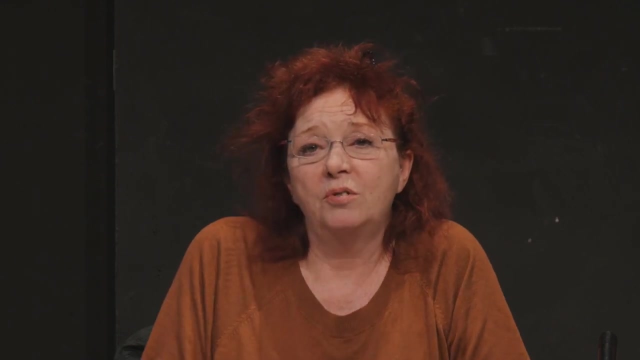 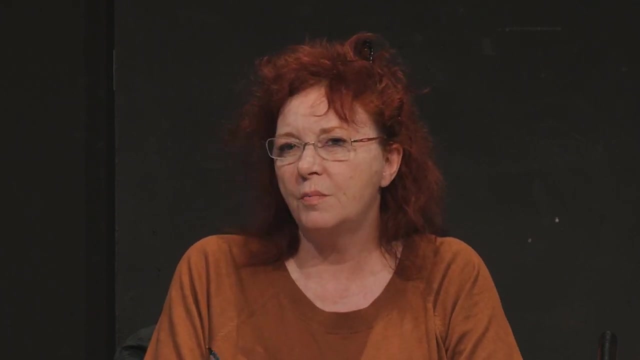 So the second thing I've really the lady here who is talking I just I really want to try and clarify about. I gave that example deliberately because I thought it is a controversial one. It is one that people will find It hard to speak about or hard to contemplate children speaking about. 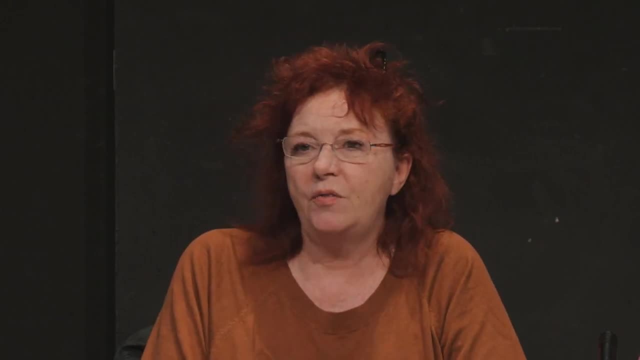 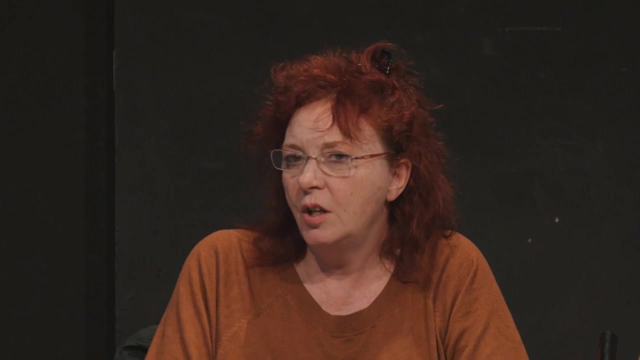 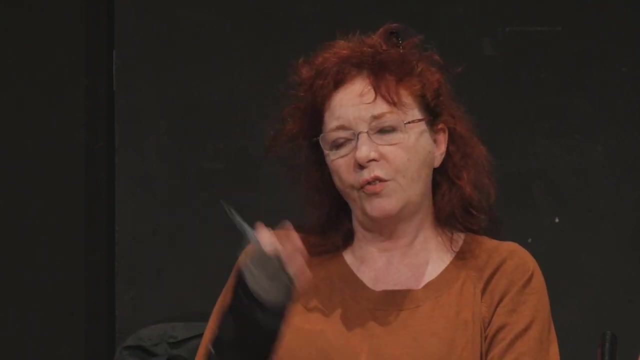 But the point of the example is that, within the kind of philosophy I do, we are not assuming this Western cultural approach. We are actually questioning that where everything is open to question, And one of the things about this kind of philosophizing where you go underneath the first example is obviously based in somebody's culture, but you don't have a person who isn't in a culture. 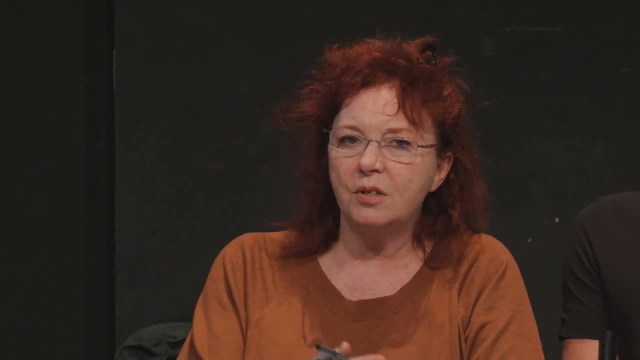 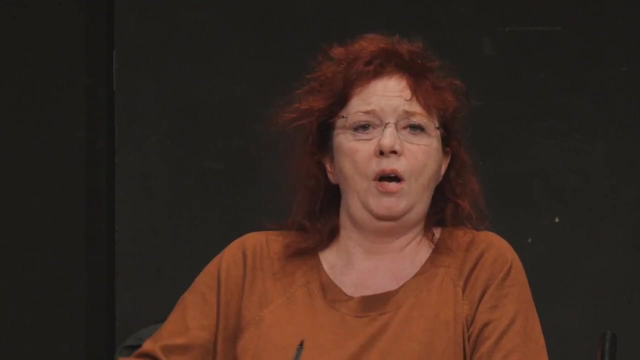 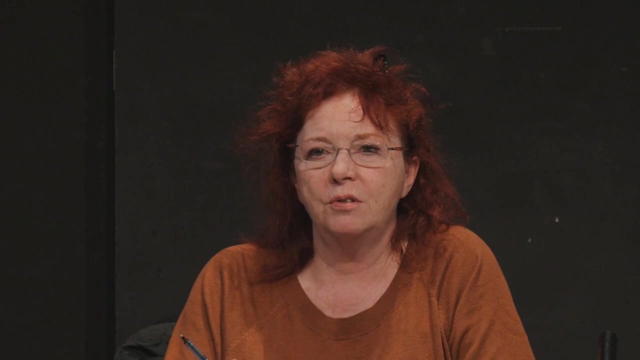 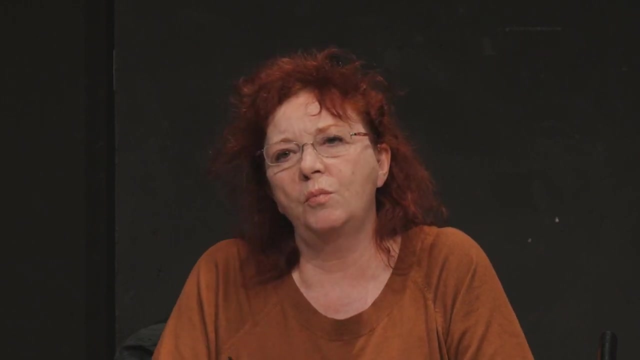 But as you dig deeper to the underlying Philosophical assumptions that underlie everything, These become universal across all cultures. So the question of how do we know what's true is the same question in every culture. The way people answer it will be different, but that will be different according to their language, their experience, their age, their proclivities. all kinds of factors will affect it. 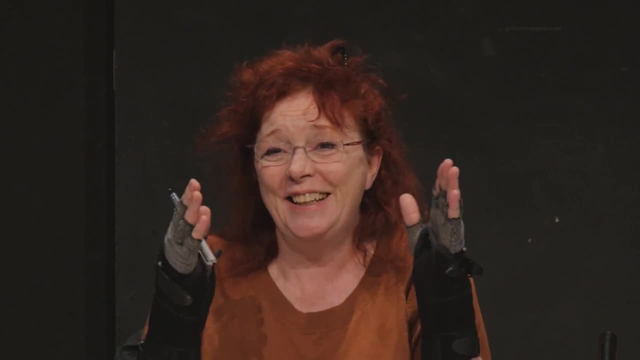 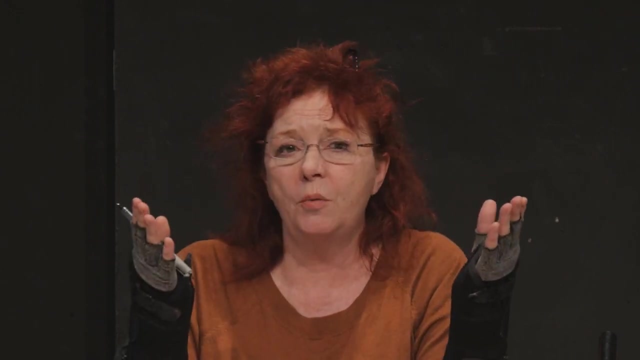 But it is one thing about doing what I might call pure philosophy in a sense is that it is universal, It can be understood across, And that's why it is all over the world working extremely well in all sorts of different cultures. I mean, I've worked in many different cultures and many different languages myself. 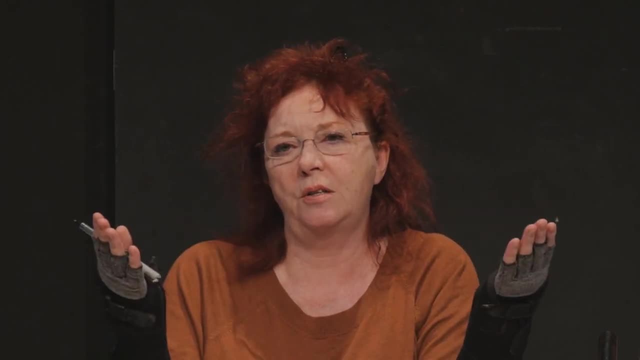 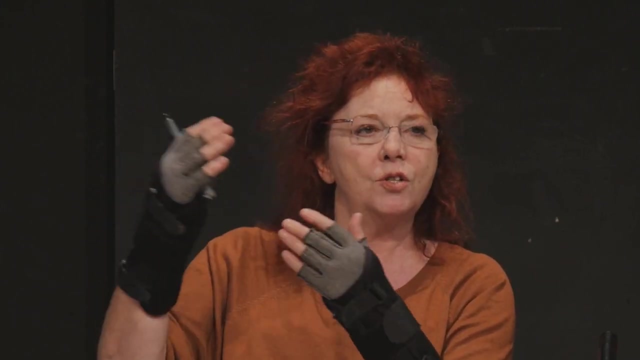 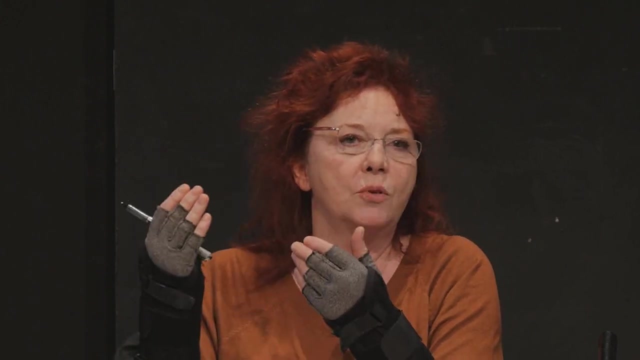 And it does it because it's not culturally dependent. When you get to the philosophy part, the bit that is are the examples, the real experiences that you're testing out. So, within the method I use, we test a philosophical theory with a few real life examples and say: well, so a counter. 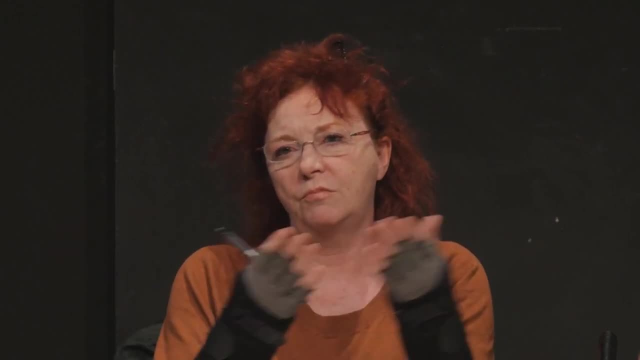 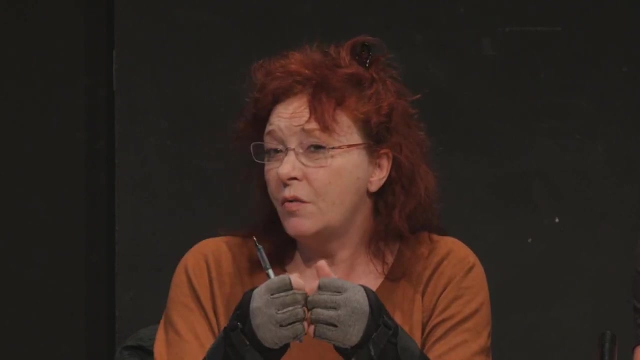 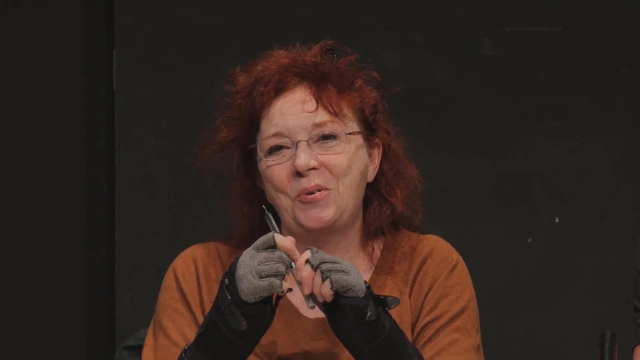 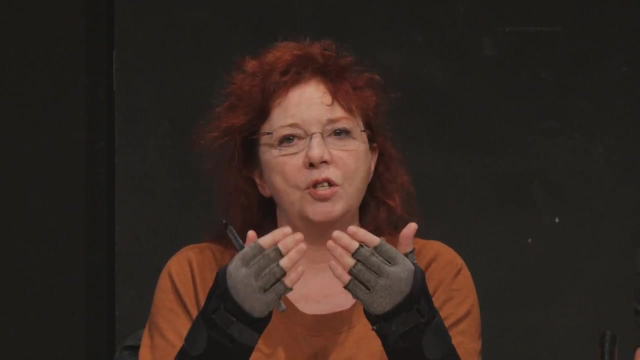 Example can say that can't be the case because here's an example that shows it isn't the case. So those examples will be culturally defined, obviously, because they come from people's experience, But the philosophy isn't, It's universal. So, and one other thing I wanted to add, which I didn't have time in my main talk, is that the issue of free speech and being able to say anything, anything at all, in argument, which is what we do in my practice- 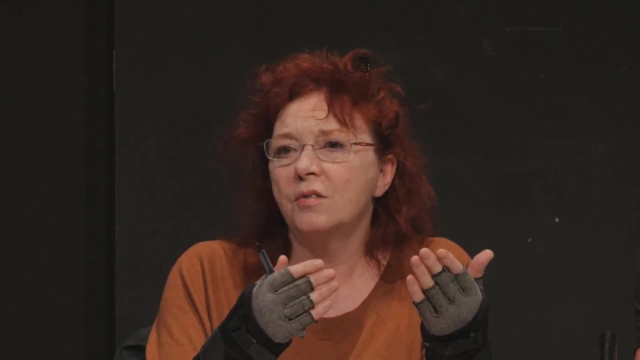 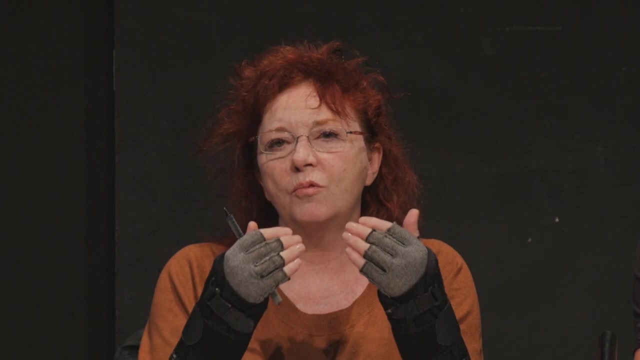 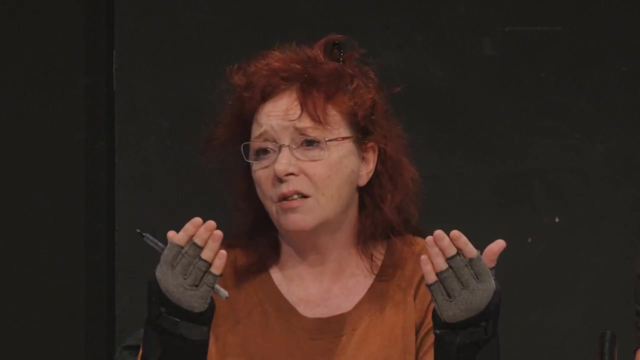 And I often get questions about- well, you know, but people are very Hurt by you know, some kinds of speech, so-called hate speech, and so on. Well, my answer to that is that you develop resilience. instead of being hurt by words, you, by doing this kind of practice, the children and the adults that I work with- develop resilience. 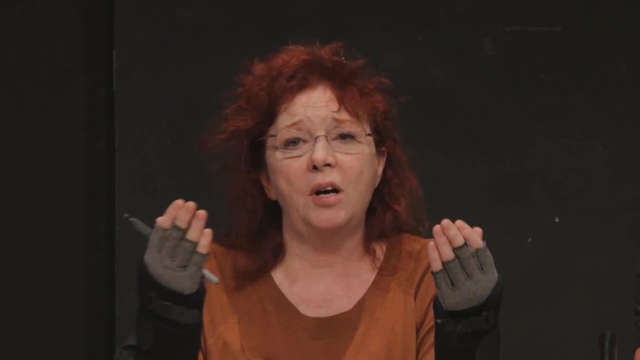 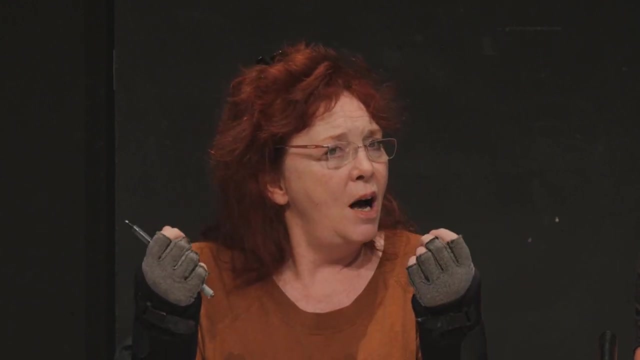 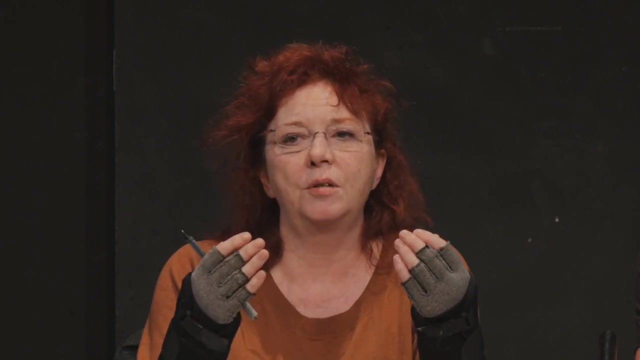 They're just not hurt by words, They are not upset by arguments that they totally disagree with. In fact, they look forward to them, They're challenging They're, they're something to think about, And I think that is the answer. And because free speech is our fundamental, fundamental freedom, you cannot really have anything without having free speech and free thought. 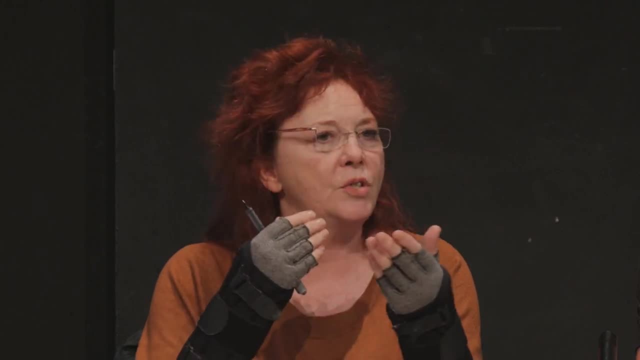 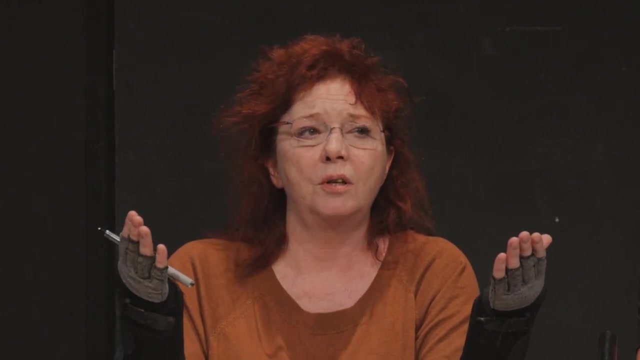 We'll have no scientific development, We'll have no artistic development, We'll have no technological development. We just won't. We'll go back backwards without free speech And we're really in danger at the moment in Britain of losing, especially in Scotland. 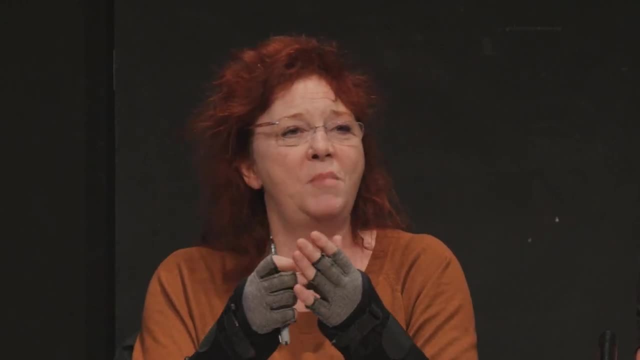 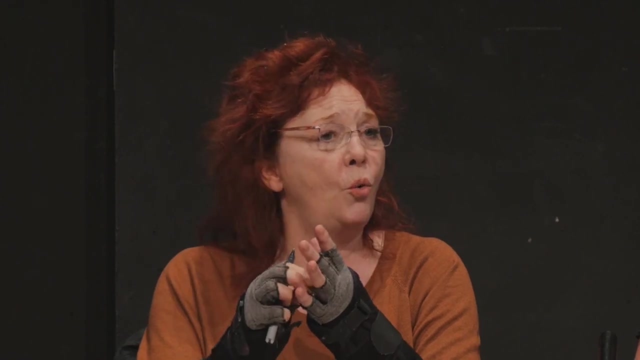 But I won't go on about the song crimes, men being put in prison for singing the wrong Song, where the police have had to be trained to recognize the wrong song so they don't even know which they are, so they can arrest people who are singing the wrong songs. 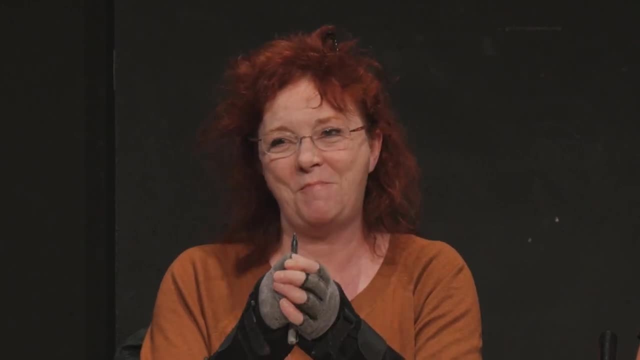 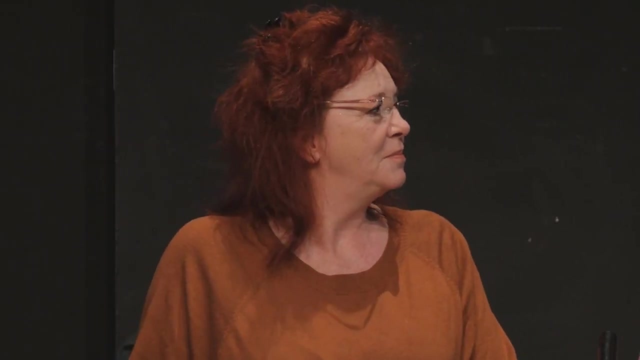 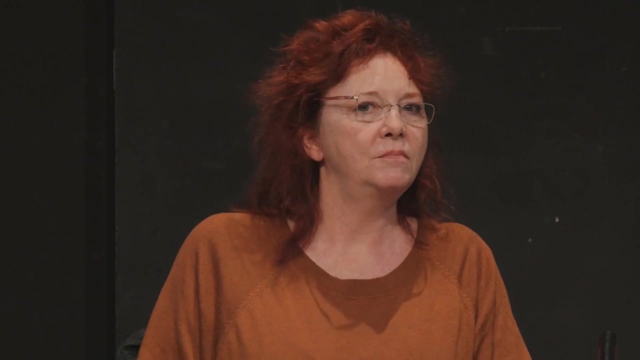 That's happening in the UK right now, So you can see why I'm a bit passionate about it. Catherine, can I just ask you just one question as a non philosopher? Yes, What substantive knowledge does the philosopher have of the world? And I'm interested: can you do philosophy, let's say political philosophy, without substantive historical knowledge of the world? 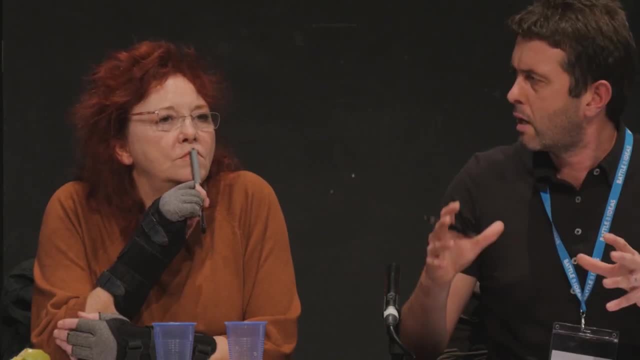 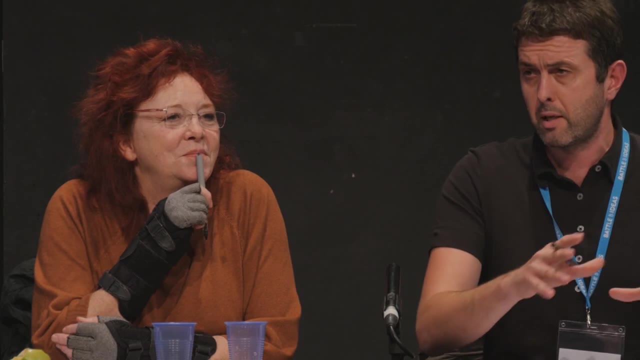 Yes, I mean, I'm just I'm trying to reconcile that in my own mind. I mean I've some experience of teaching philosophy. I wouldn't claim any kind of pedagogic expertise or disciplinary expertise. I did it for a while, I think, probably with mixed results. 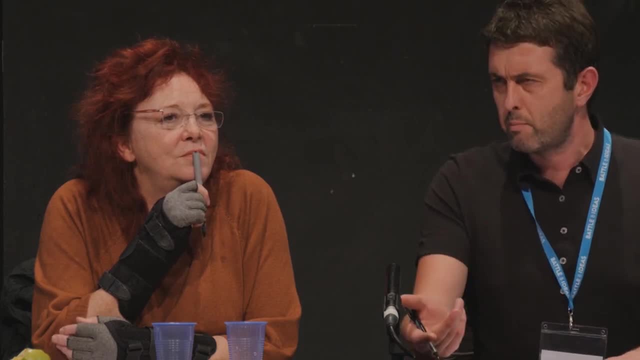 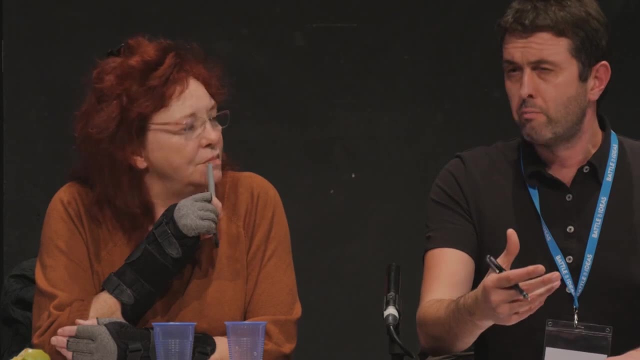 I did notice that certain students were. we did political philosophy first, then we did moral philosophy And I noticed that the moral philosophy worked better because I think I had more experience of moral questions and the political philosophy worked better with the older students, but not so well with the older students. 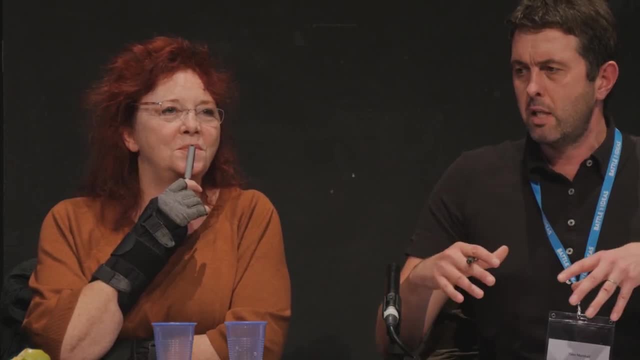 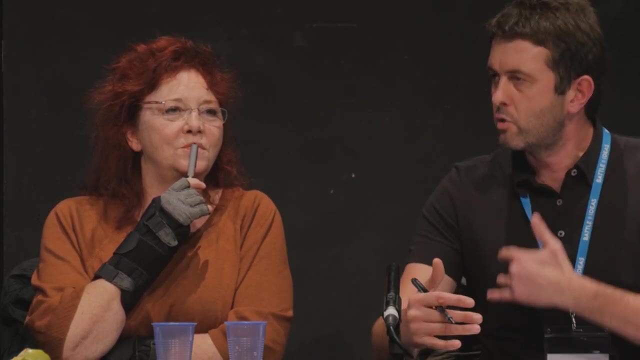 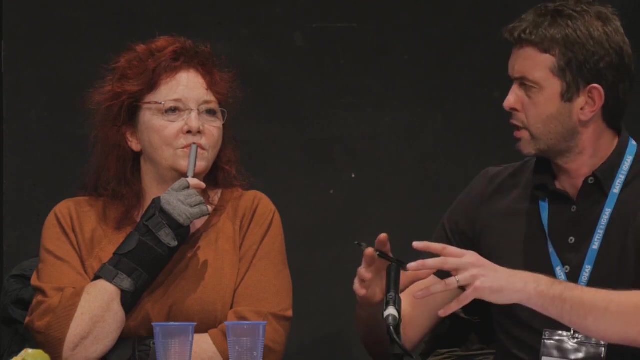 So I'm just: does philosophy just sit in a vacuum or does it require something else to be done? well, And that maybe helps us get to the educational question of what space should people do? sorry to abuse my position as a chair, but I'm just genuinely trying to work out what is philosophical knowledge, and how is that different from, say, history or sociology or arts or something like that? 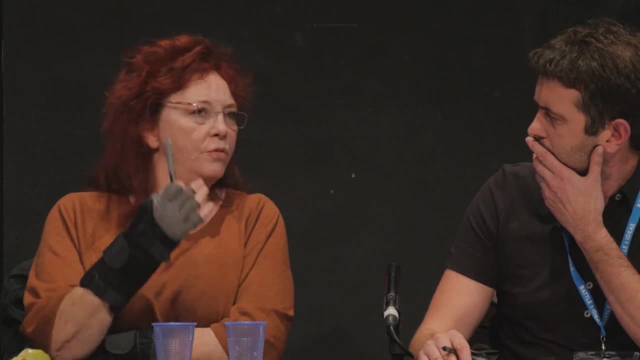 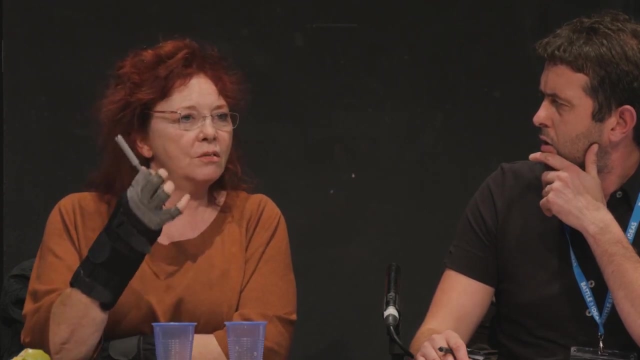 Am I making any sense there? Yes, And you could do philosophy of science, philosophy of politics, philosophy of art, philosophy. You could do philosophy of anything. So it doesn't require specific knowledge, just experience of being alive. I would say. 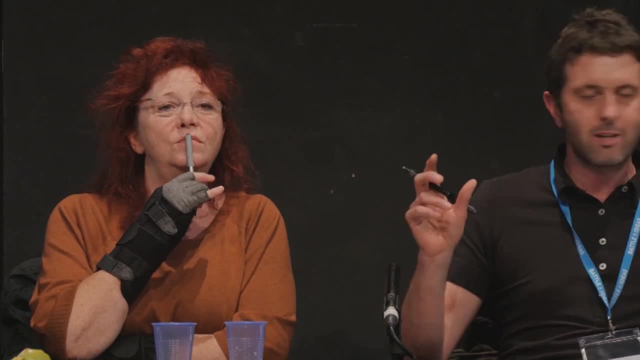 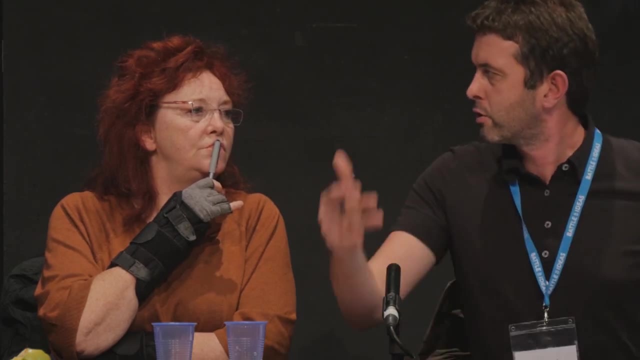 Just to be devil's advocate, because I know the panel is weighted in one direction. do we not need to do the subjects that we're doing the philosophy of first before we can do the philosophy of those subjects, ie history, to then do the philosophy of history? 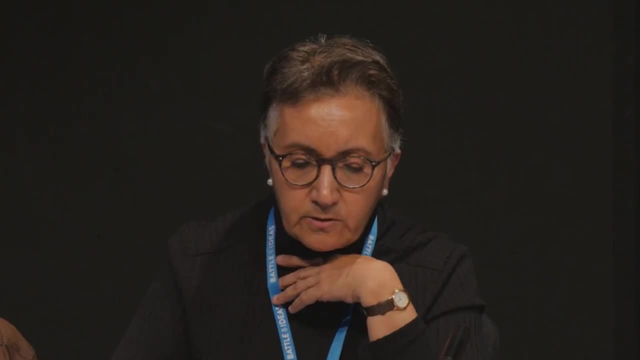 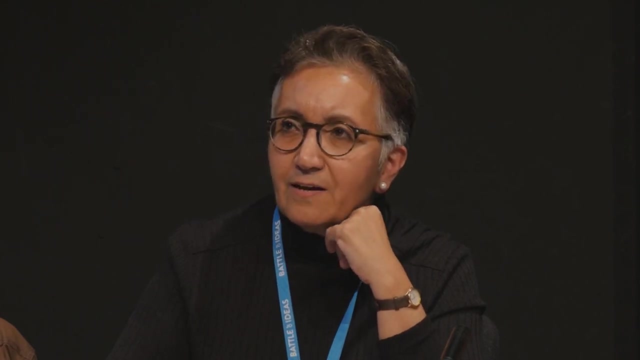 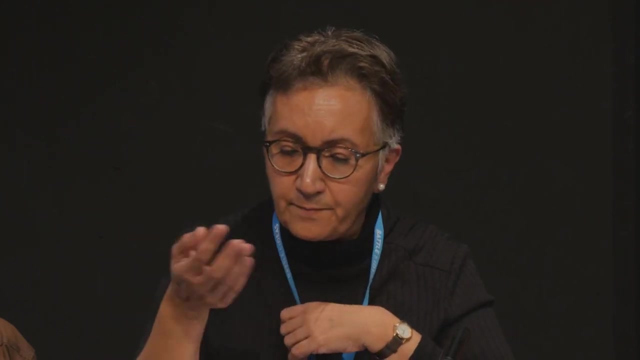 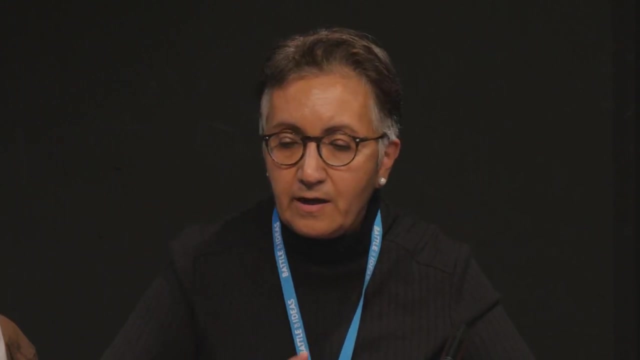 I mean, which I think is an educational Alka. did you want to The question quickly: Do children, Do children need to grow up quicker today? I think that's a. it's quite a tricky question really. I'm not going to try and answer it now, except to say in some ways you could look at some aspects and say yes, but then if you look at, you know how long children stay at home or you know how willing they are to sort of go out and try things independently, that there are other things that say you know that would indicate that they're, you know, they're not far from growing up too quickly. 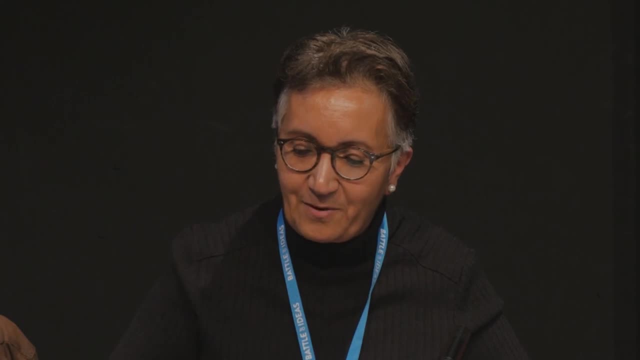 They're not growing up fast enough in other ways. So I think that That would to answer that you'd need to, really you'd need to, you'd need to refer to, you know, a whole lot of knowledge and ideas and thoughts outside this particular discussion. 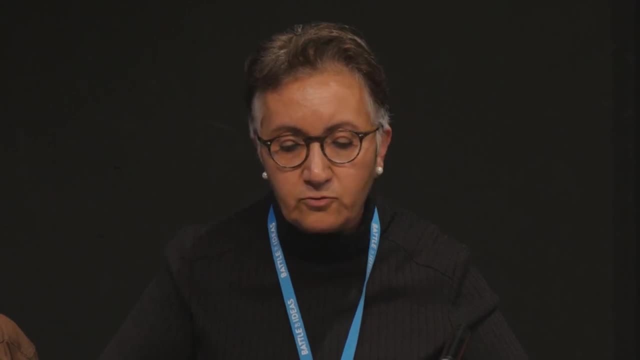 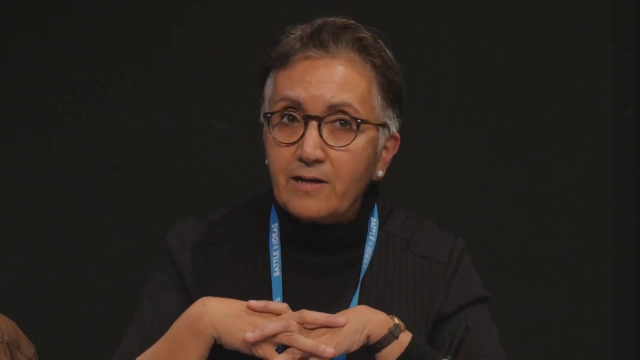 The person that asked wanted to ask. children should ask questions and we need to have a questioning. you know need more questions, I totally agree with. However, the main question I want to ask is: why is it that there's a real, real kind of urge to say: 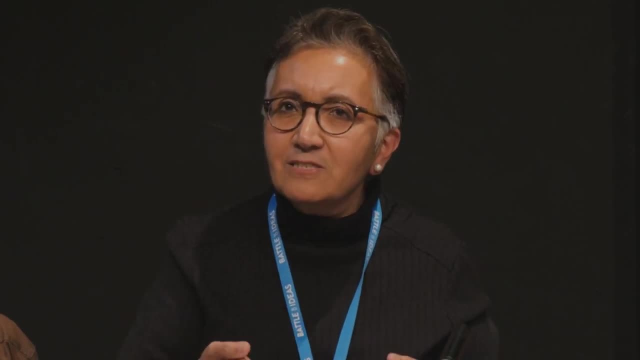 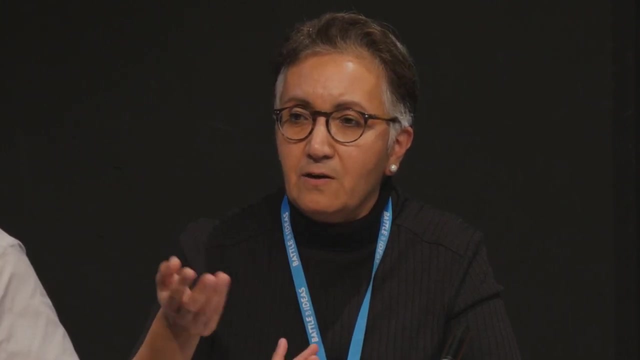 Children need to ask questions. Why? I would say it's not. it's not so much them, They cannot. they generally do that anyway. They're generally quite good at it. They do it fairly. you know you have to work hard to get them to shut up from asking questions sometimes. 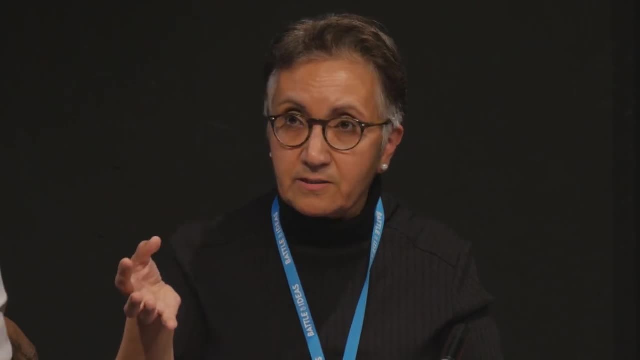 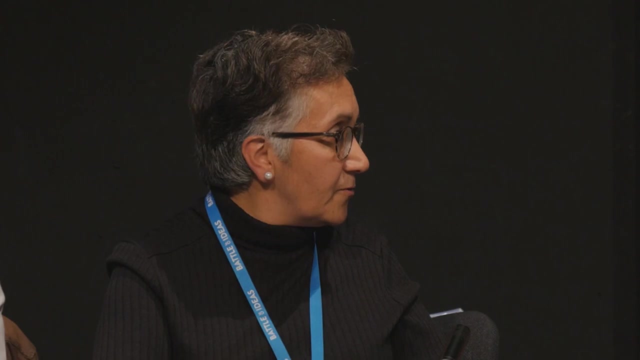 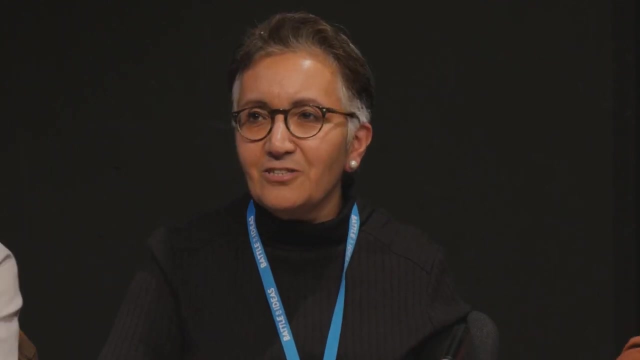 More of the question is why you know it's adults that need to be asking questions. Teaching philosophy for children in classes is not going to stop the Scottish government from being authoritarian, or any other government. That's going to need a political. It's going to need a political discussion in the adult world here and now. 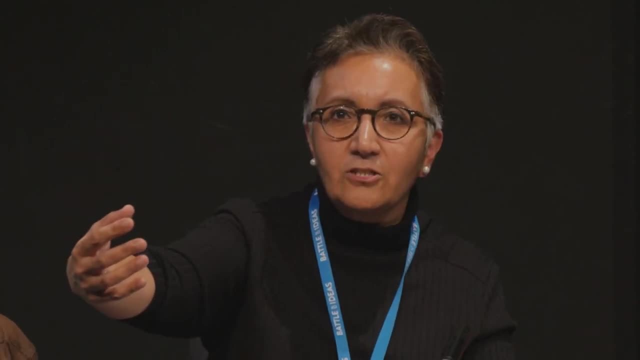 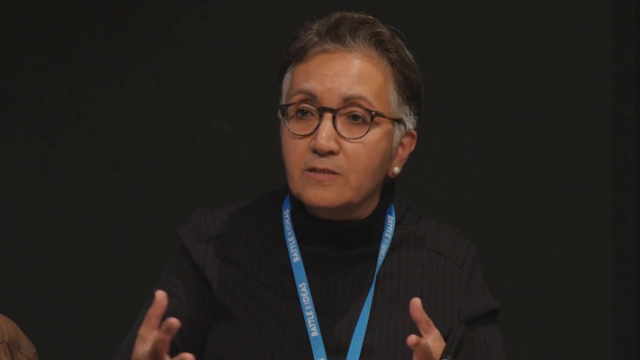 You can't sort of defer it to future generations by saying: you know, basically what it's doing is accepting an impassive or an inability, giving up on doing something in politics now and saying: well, you know, maybe we can get education better and the next generation will do it. 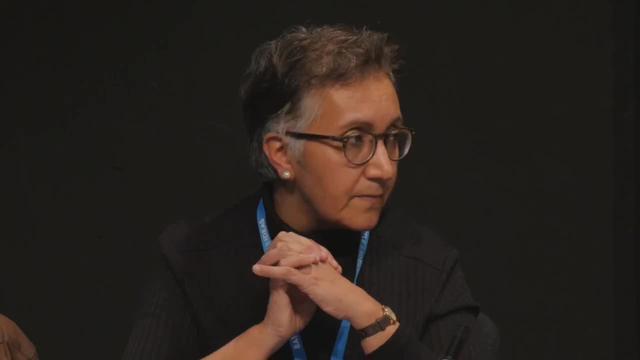 And I'm sorry, but to me that is, that's a cop out. OK, can I just Go on then quickly. I just want to say, I just want to say fast that I'm not concerned about the curriculum. 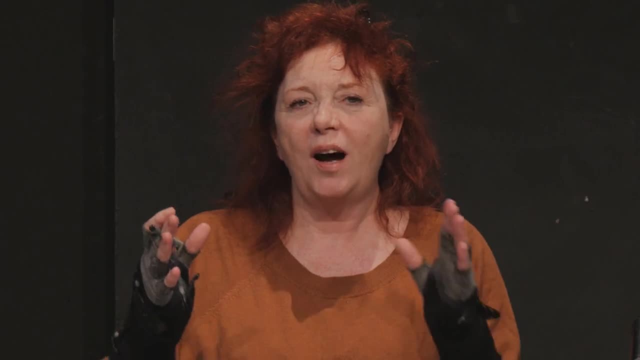 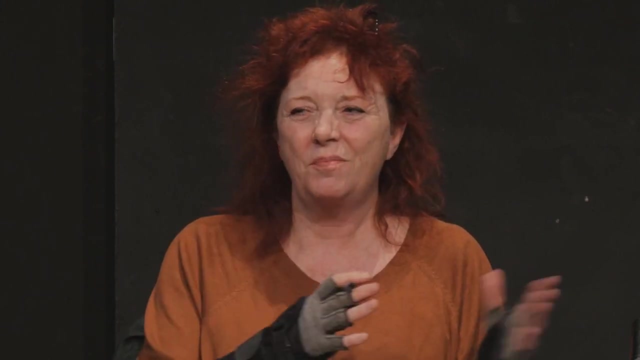 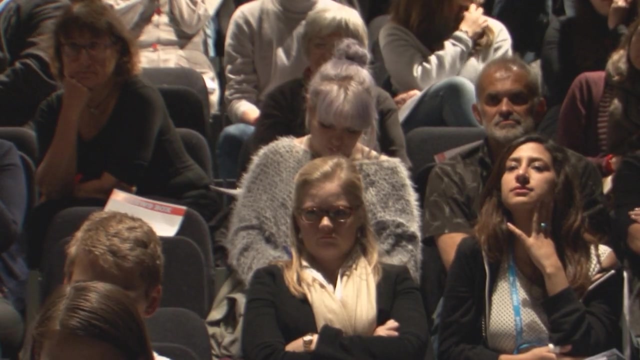 I'm a philosopher. I do philosophy with children anywhere. So I think the question here is whether children can do philosophy, not whether schools should have it. I mean it's curriculum questions a bit of a side issue, But I totally agree. adults, I do the same philosophy with everyone, whatever their age. everyone should be thinking well. 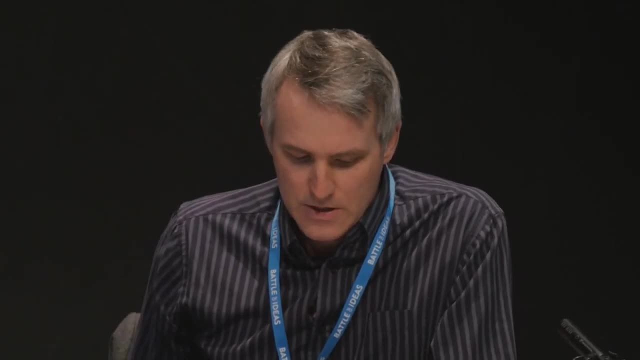 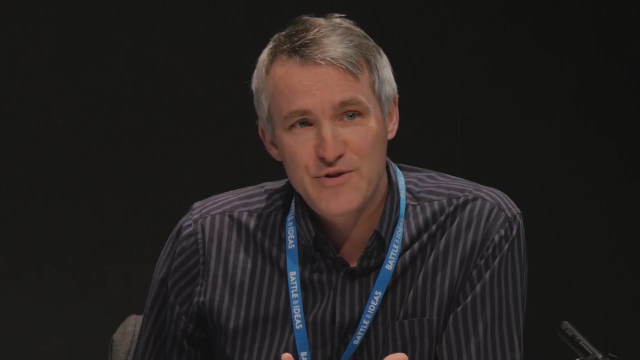 OK, so go back over a few other things as well. There was a couple of points that Alka made earlier about philosophy being about truth. I mean, it must be borne in mind. It's consistent with my re-evaluative principle that I mentioned earlier- that truth itself, of course, is a subject for philosophical investigation. 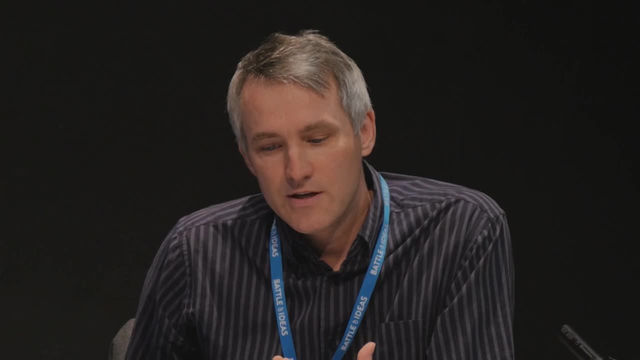 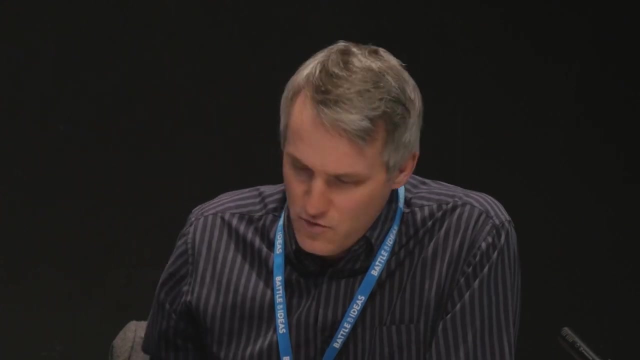 So we can't just straightforwardly say that philosophy is, you know, about truth- And of course that's a hugely problematic area- truth anyway. So that's one point. The other one that, Alka, you also mentioned this thing about reality and experience and how it takes time. 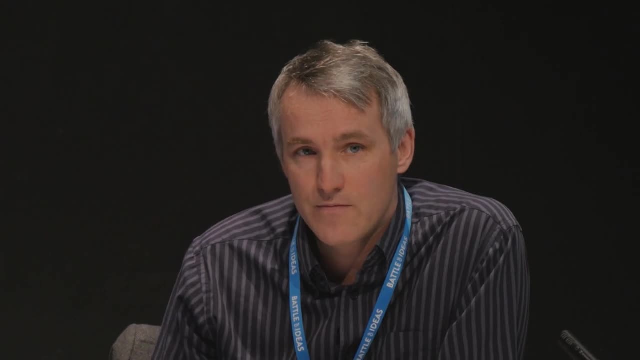 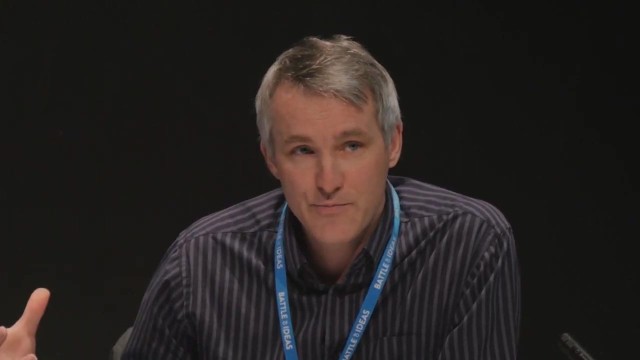 Well, one thing that children do have is they have an experience of reality- I mean, they just do From the moment they're born, And so they already have life experience to draw upon. OK, it's not the same amount of life experience as someone who's older, but it is life experience. 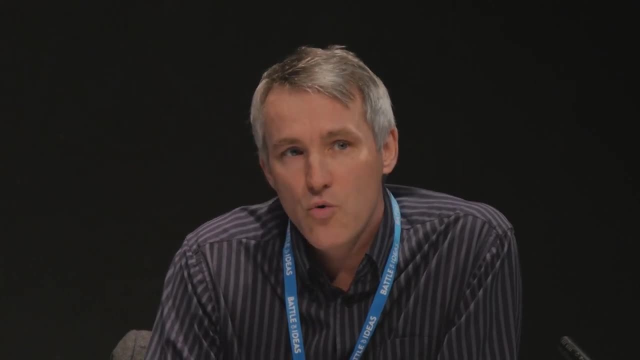 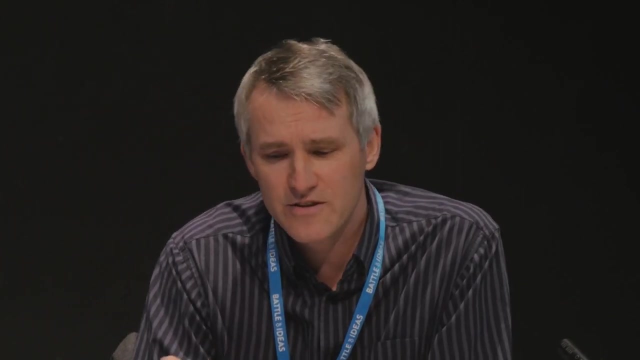 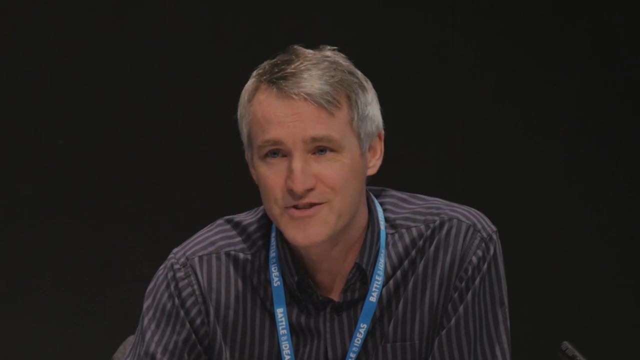 And I said that philosophy was responsive. What I meant by that was that they've got to come up against something which they respond to or have an opportunity to respond to. So, for instance, you know, I might think that time I might be young and I might think that time is constant, because my clocks go constantly and it's always the same time wherever I am. 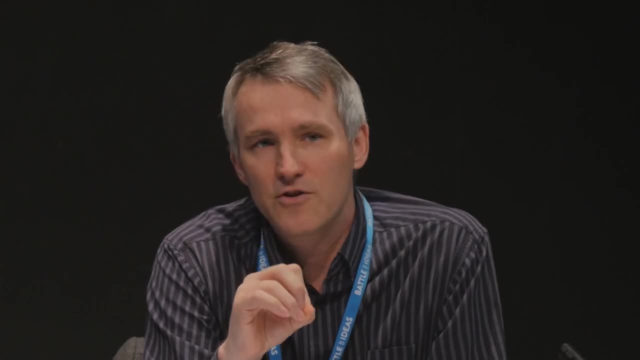 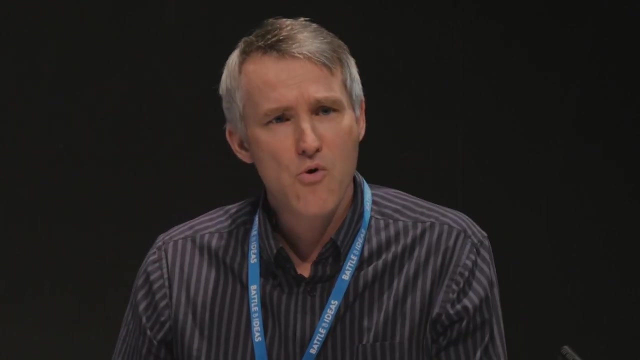 But I might also experience time as being inconstant. or unconstant, I might you know, because I might go to sleep and wake up quickly and think, oh, that was quick, What happened there? Or I might be bored like- hopefully none of you are now, where the time takes much longer than it would if you're having fun. 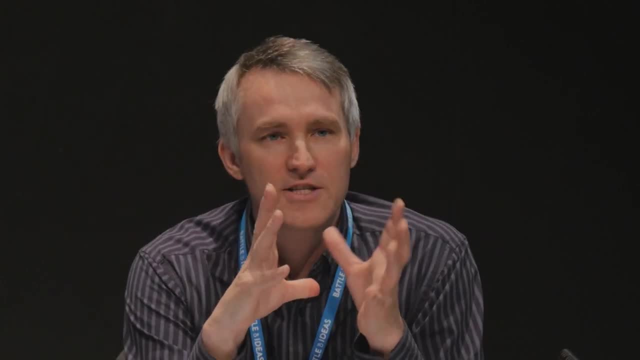 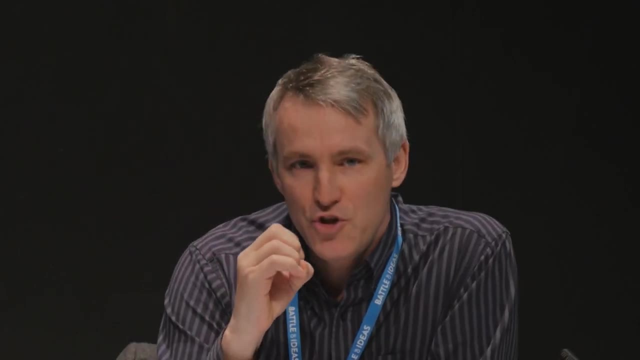 So these are clashes where our understanding of reality and our experience of reality kind of don't quite fit, And the moment you have that kind of experience, you have philosophy. Now, it's not philosophy yet. It's not philosophy yet, though, because you may just go: oh, that's interesting, wander off and play with your ball. 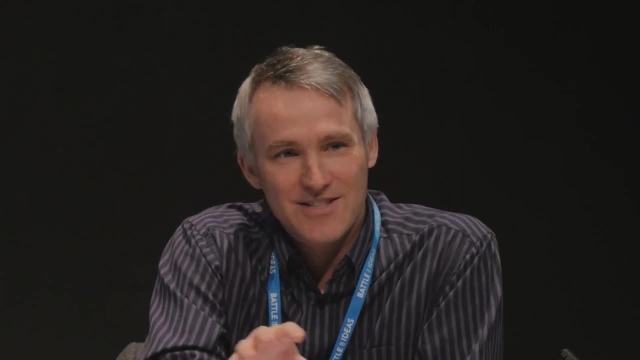 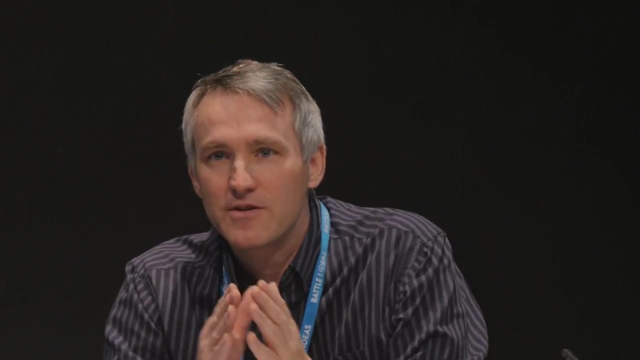 You might not respond philosophically OK, but some children do, And our young speaker earlier- or self-proclaimed young speaker earlier- said you know. and one other there as well said that you know they were asking these sorts of questions. 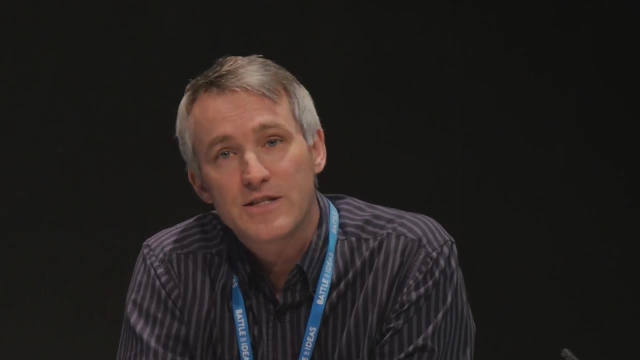 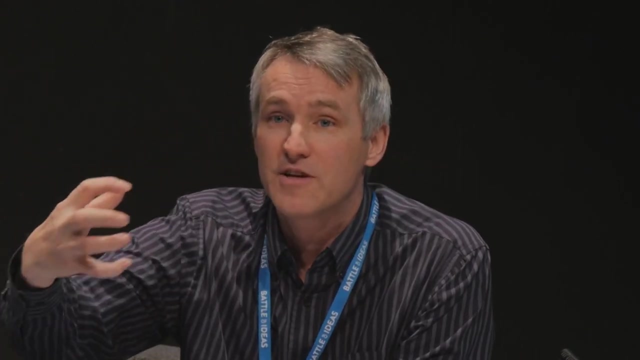 And some people do respond philosophically. They should be given the opportunity to take those ideas forward, And perhaps other children should be given the invitation to take those ideas further than they perhaps would have done before, Not by being forced to, You know, to go further, but just given an opportunity to think that through. 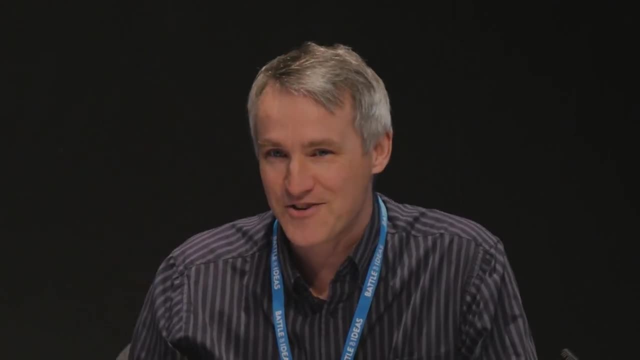 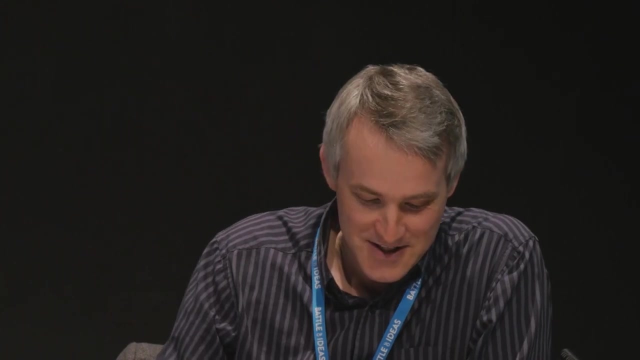 So I think that's a really important thing is that you know, because Plato famously said you can't do philosophy until you're 40.. I like David Shapiro's book. Plato Was Wrong Good title at the beginning there And that's the point about that. 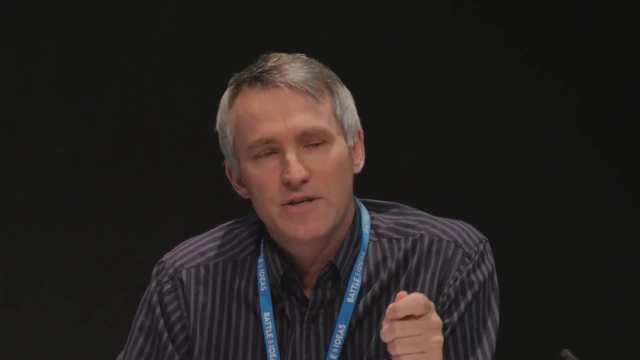 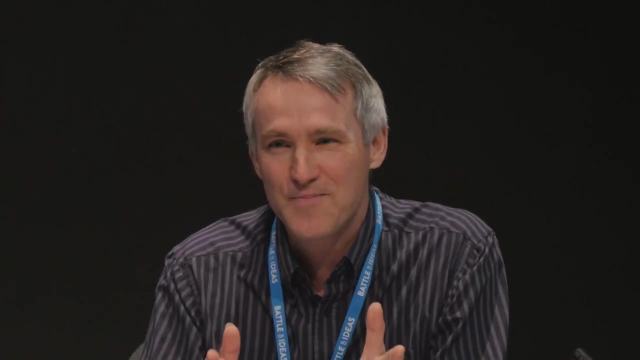 And I would also want to say something about: we want to be a bit more descriptive. I think about this rather than prescriptive, You know, rather than it reminds me of a Doctor Who episode in which they were stuck on a planet And there was a professor in the planet. 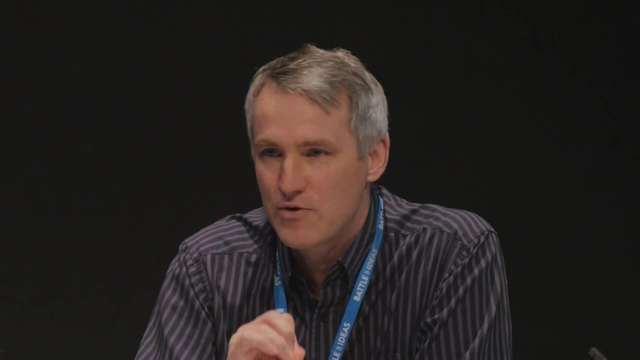 And the professor said: oh, there's no life on this planet, There's no way in which life could exist on this planet. And they get attacked by something. And the professor says, no, we're not being attacked by anything because there's no life on this planet. 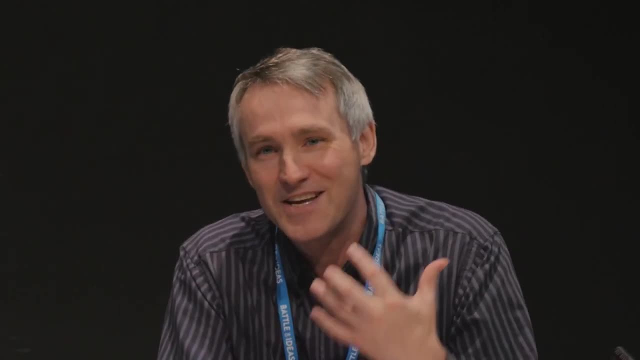 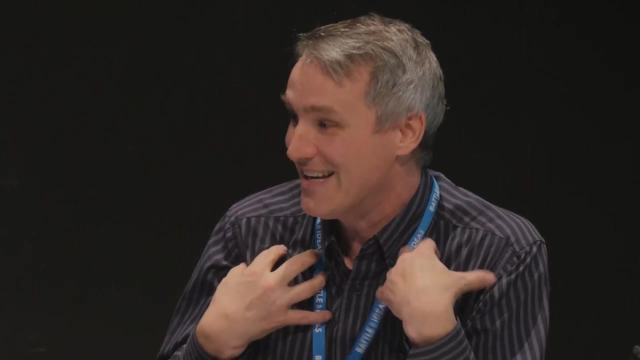 All the theories say so And it's quite funny because it parodies the sort of obsession with theory. And what we should do, I think, to some extent, is stop being a little bit over-theoretical- Not very philosophical of me here. 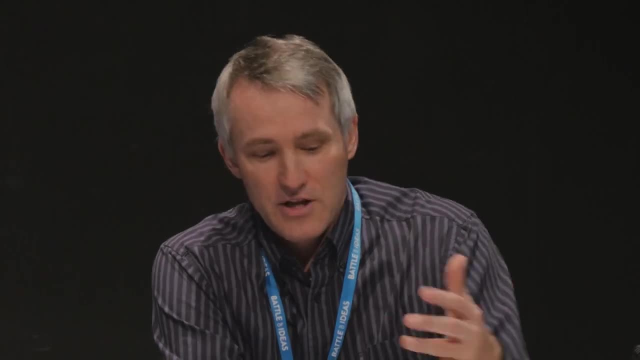 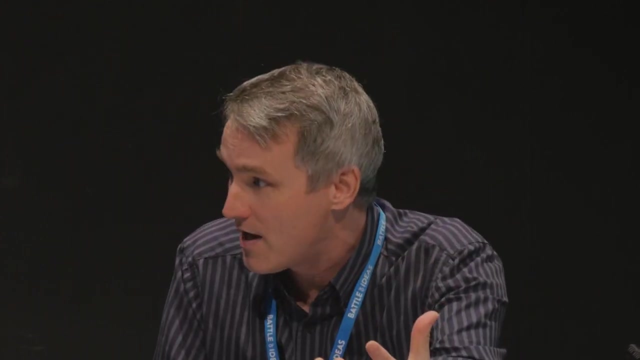 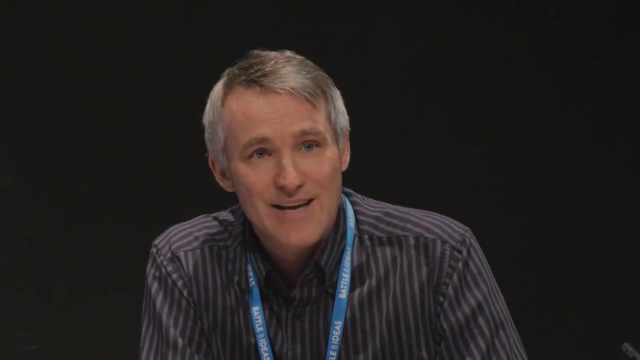 And say: let's look at what is going on. Do the children in fact have philosophical experiences? Let's not. Let's not tell them that they do or that they don't. Let's find out if they do. And then, if they do, I think we have a responsibility as an education system to provide the tools to be able to deal with that, if that's in fact what's happening. 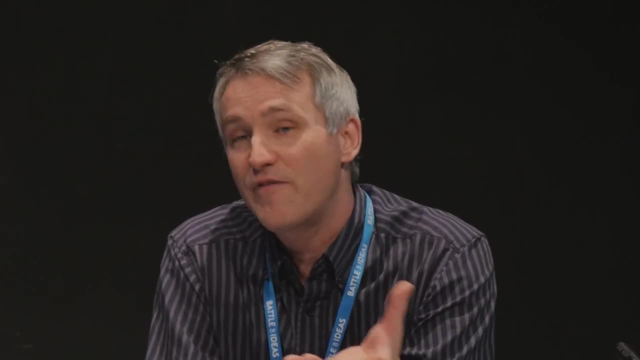 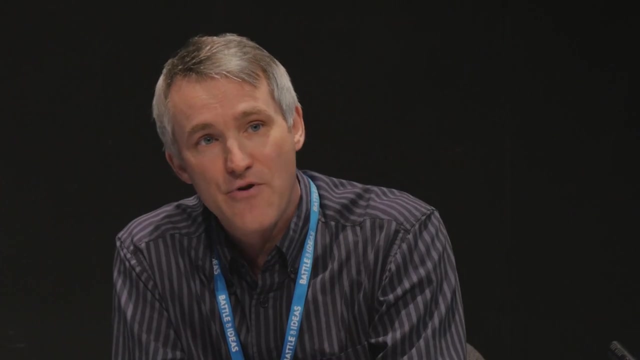 And I would say that any education system's duty is to provide the tools to enable anyone to deal with problems they might meet. And if it's true that young children experience philosophical problems, there's a sense in which, just descriptively, there's a sense in which perhaps we should give them the tools to 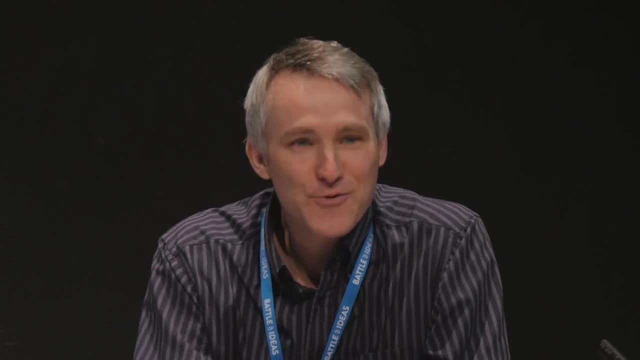 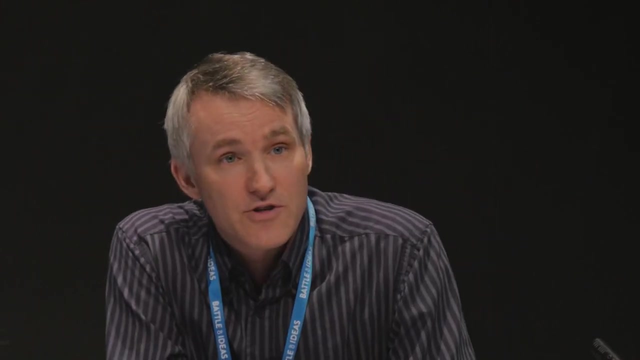 To perhaps deal with that. And last point about triviality. I was talking to some colleagues over here before the talk. Shakespeare was accused of being trivial. Okay, And it was through some of his most trivial insights and plays that some of the deepest insights came. 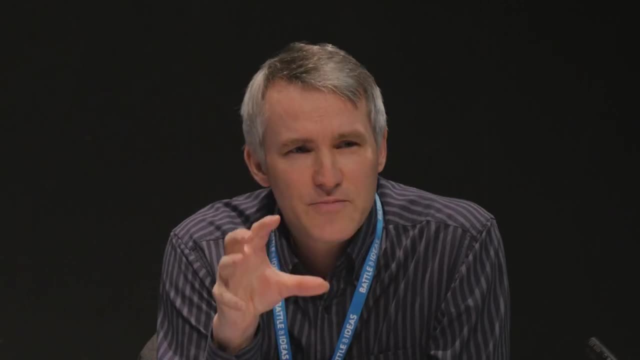 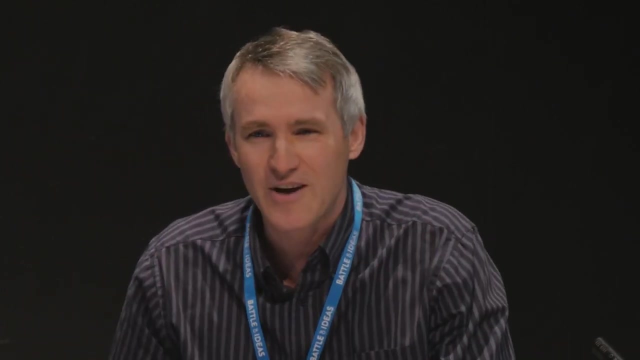 And just to give you an example, I often ask young children: does the hole in a donut, does it exist, Or is it part of the donut? Now, this might seem incredibly trivial And I've had philosophers say to me: I just don't see the point of this. 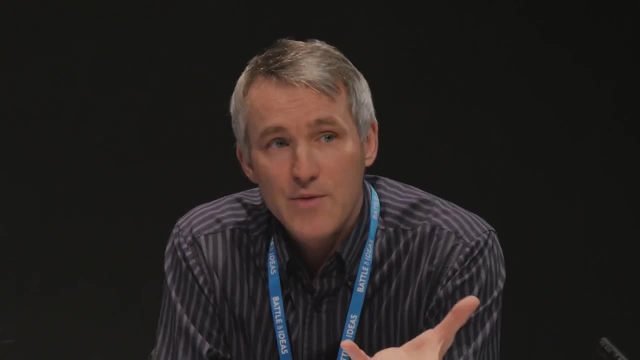 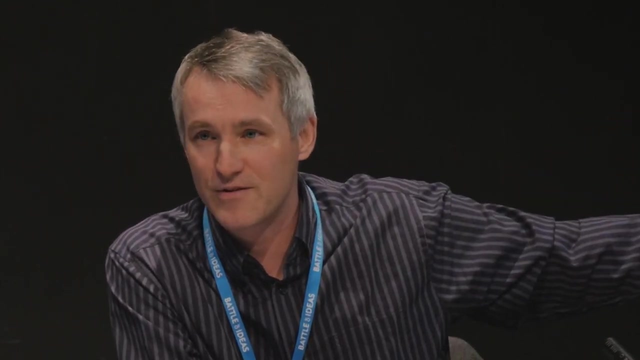 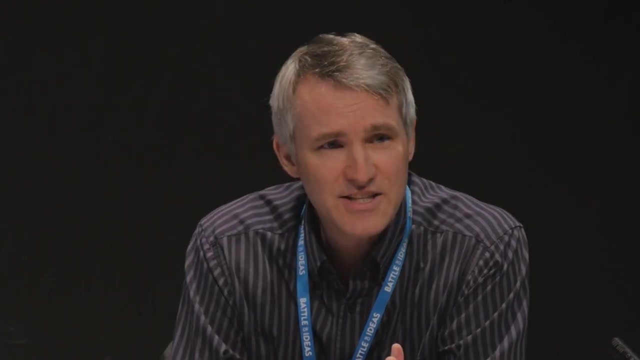 But when the children- and, by the way, I find that children are just as able to abstract about metaphysics as they are about ethics- It's a myth that children can only do ethics, philosophy questions. I've had children sort of get into the notion of a priori space, which is a Kantian idea, using the donut. 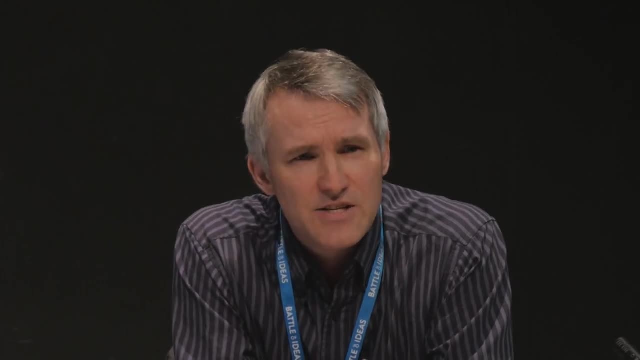 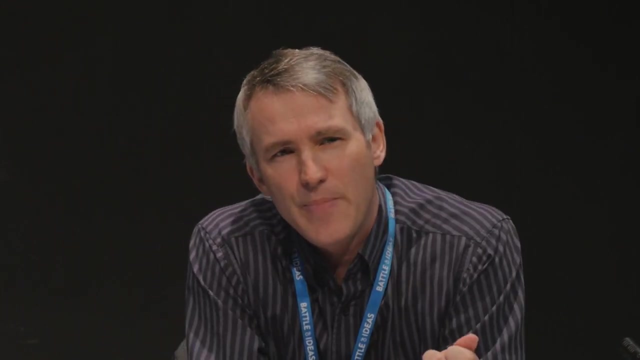 So one child said: the donut, the hole in the donut surrounds the donut. So how big is it? They said, well, it's the size of the entire universe. The next child said: ah, but the donut, the hole isn't just where the donut is. 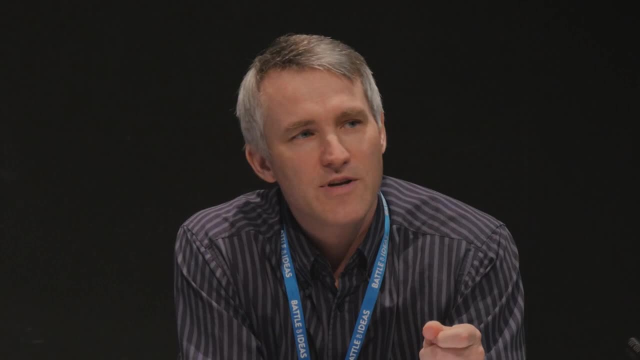 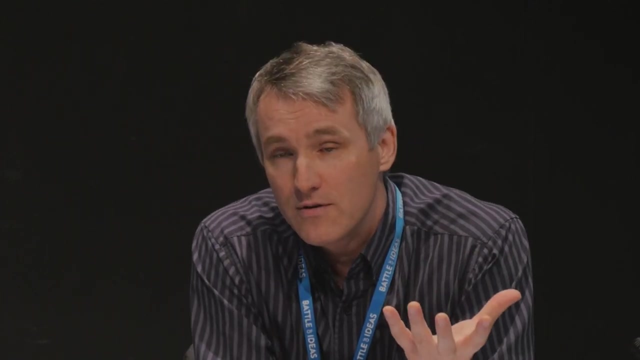 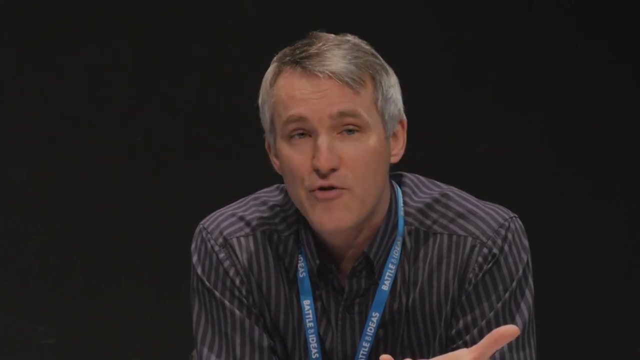 The hole is also where the donut is, Because otherwise there would be nowhere for the donut to be All right. So the child has moved from the trivial into something philosophically deep and insightful, namely the notion of a priori space. 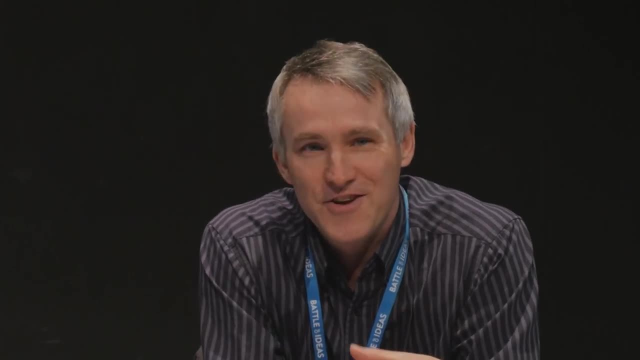 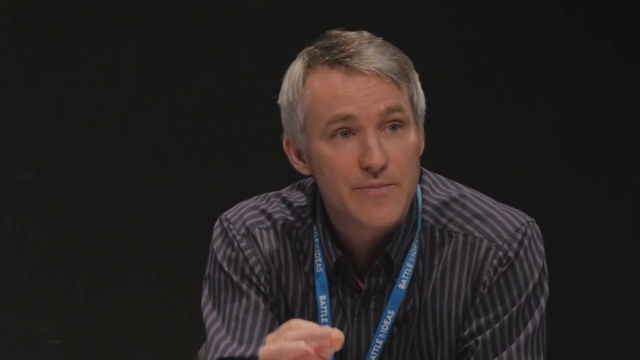 So I do question the notion that we can just say that you know I mean. OK, the example of strangling a Smurf is deliberately chosen to sound trivial, But in fact that could well lead to some deep philosophical insights. Just a few steps. 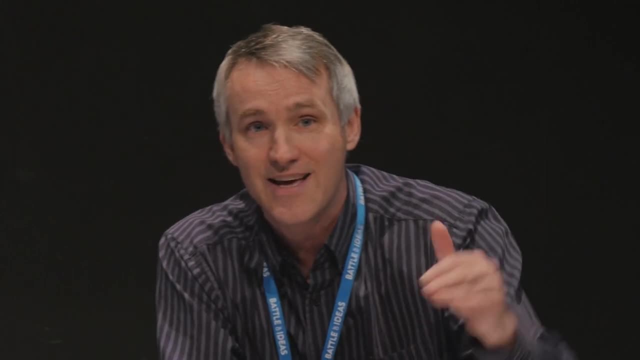 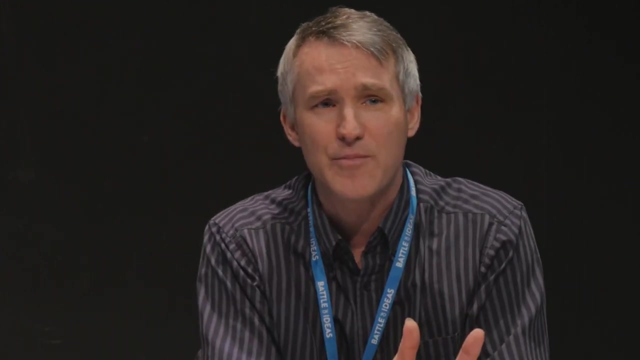 If you let that happen, if we're too prescriptive about it and say this is trivial rather than descriptive and say, well, let's find out if it is or not, Then I think we stop things happening before they can happen. So that's my big message here is let's be a bit more descriptive than prescriptive. 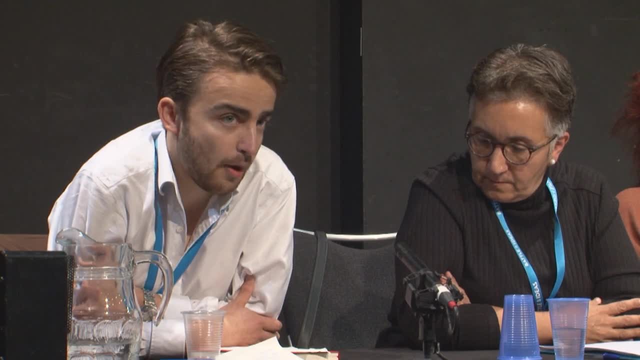 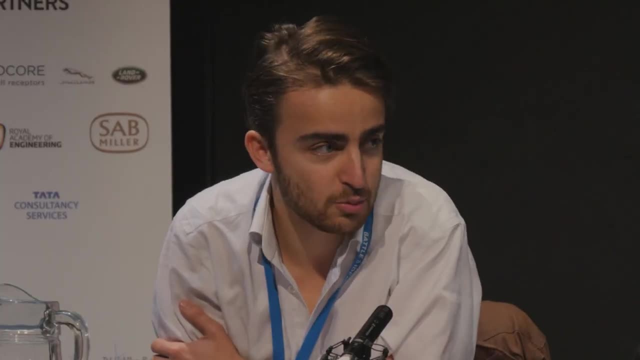 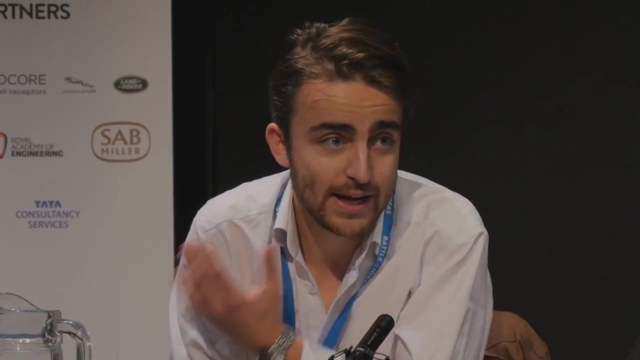 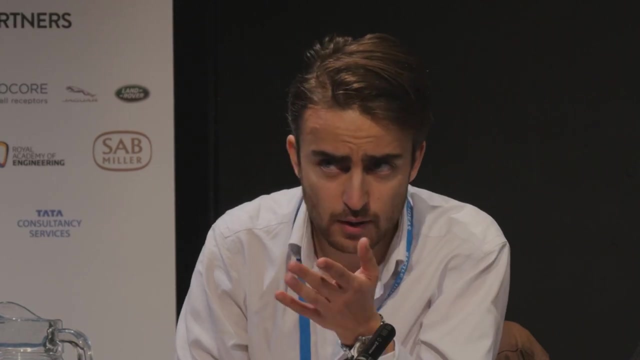 OK, thank you very much, Did you want to? Yeah, Just to respond to one of Alka's points directly about having questioning adult population, I'm sure all of us would think is important. Sure, The way to Sure We do have an adult population is to have an education system which, through things like philosophy and nurtures questioning and inquisitive minds. in terms of one of the points raised by the audience about children having these questions, 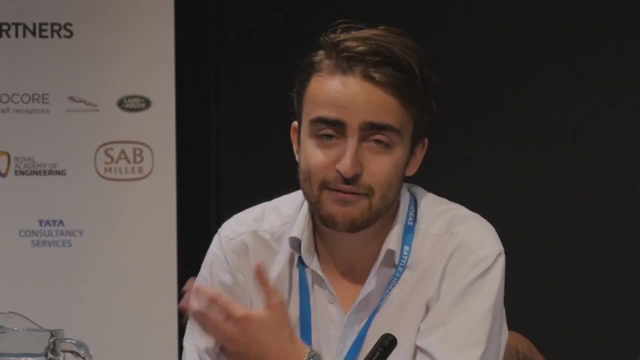 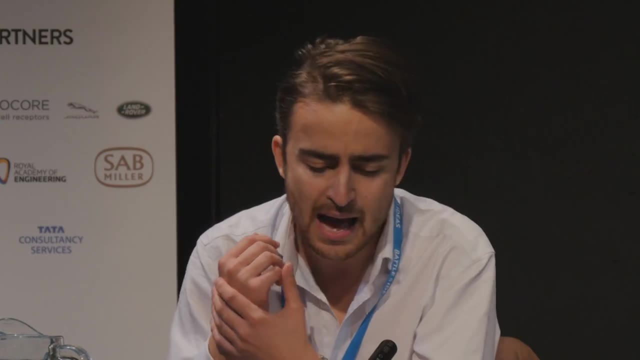 Children do have these questions and philosophy isn't a way for them to explore them and also for a way to build up more of a critical understanding of those kind of questions which they have, And it would be a great shame if children aren't allowed to explore these questions. 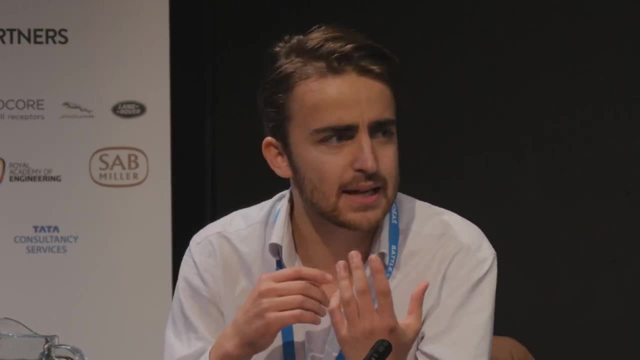 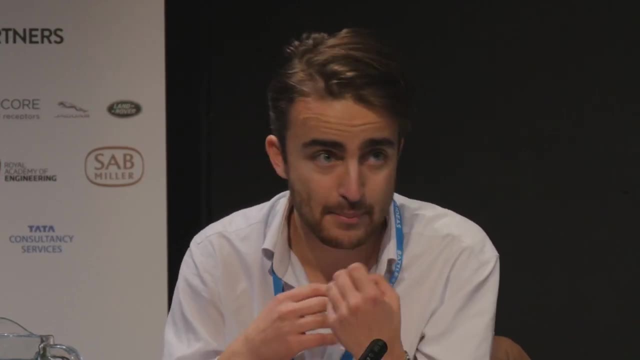 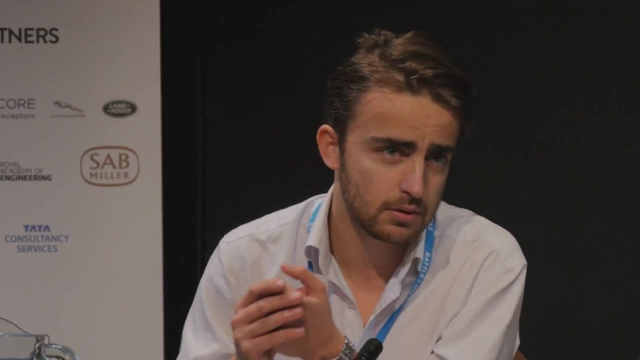 They'll leave school with a sort of numbed perspective on themselves and the world and that questioning in them is shut down rather than let loose. And in terms of the one of the points was made about being worried about scepticism, about children being too sceptical. 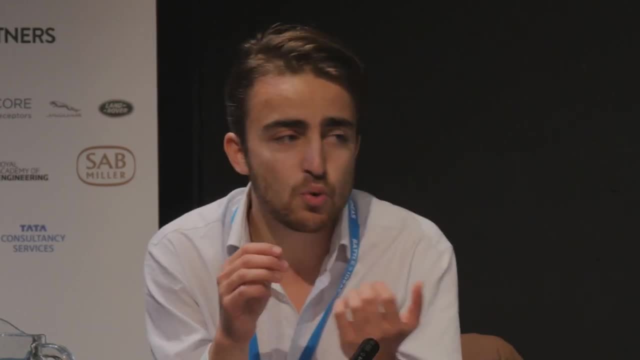 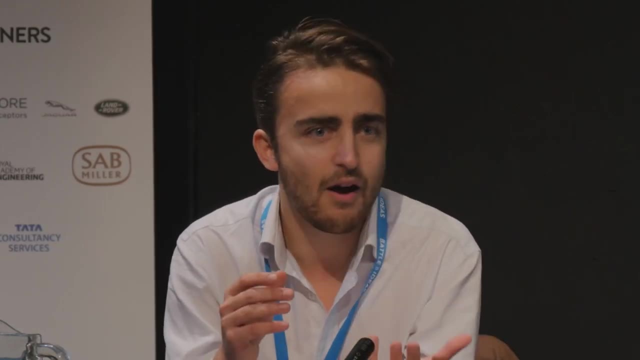 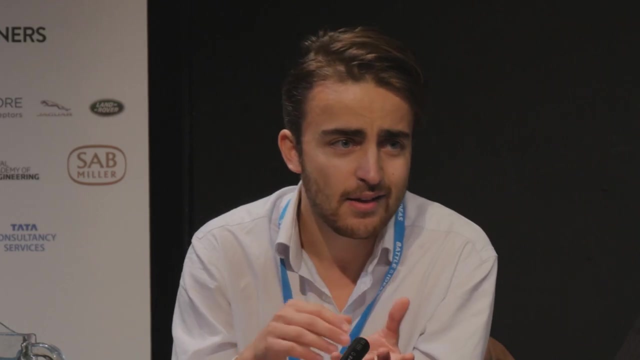 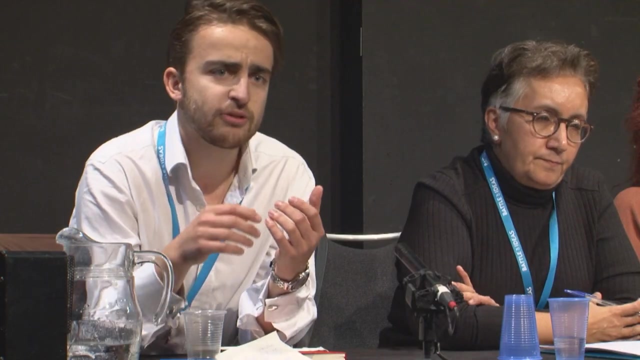 Well, I think if if parents or schools are insecure about the idea of sceptical, questioning children, then that's their problem. You know, it's Clearly very important that we have children who are questioning and who are sceptical, And it shouldn't be the concerns or insecurities of of an adult and faced with a questioning child that should. that stops children's capacity to be sceptical. 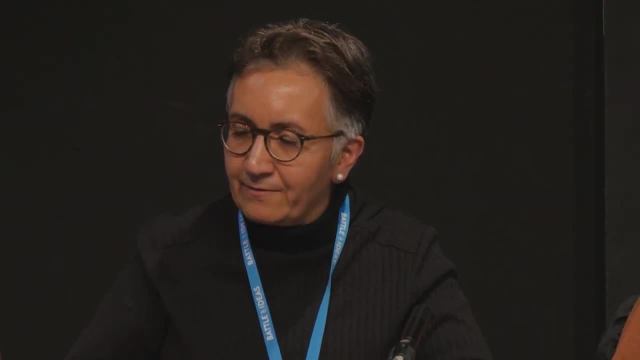 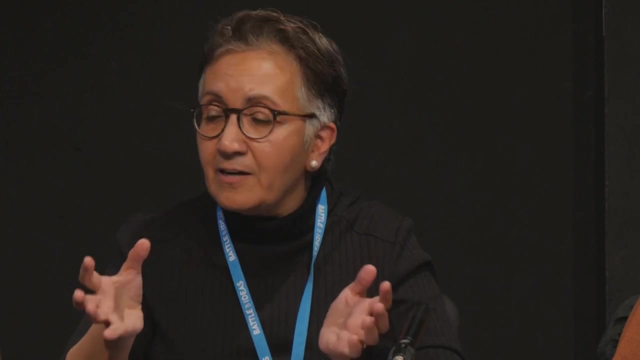 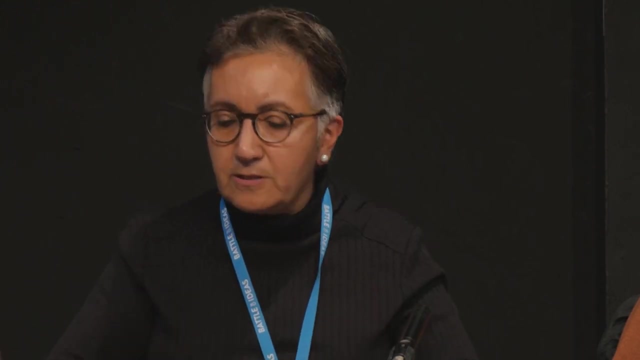 No, really, Honestly. just please read Kant Right. We do not want children to be this, that or the other. The whole point is: we want children. They decide as adults, Right As children, To say: we want your prescribing and not your idea of what you want a future citizen to be like and expecting, wanting schools to produce that. 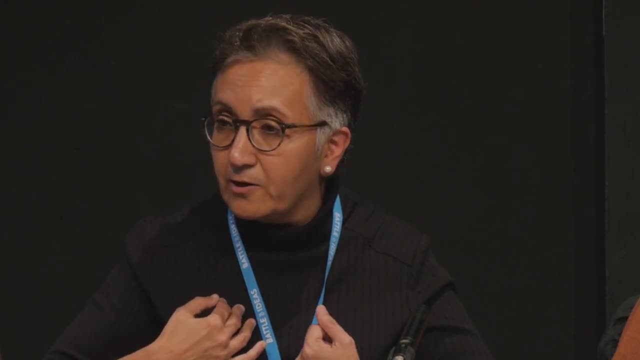 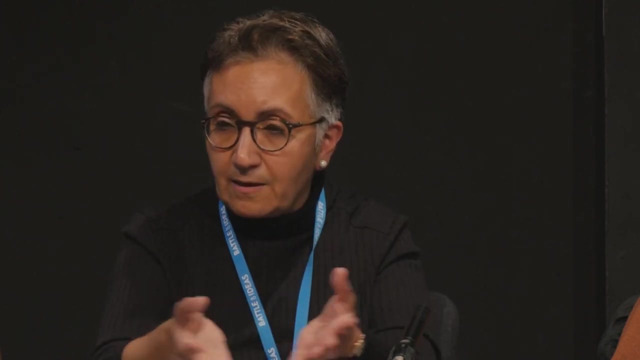 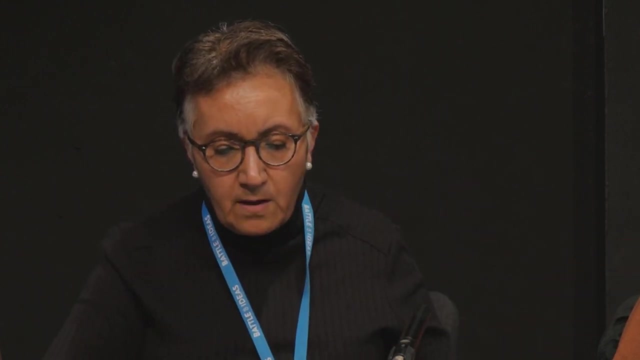 I might like children, I might like the idea of an adult population being critical, but I hate the idea of school teachers be thinking that their job is to create some model citizen according to their views. now, And the thing what your question, Toby, about and what you were saying, Peter: children, no reality. 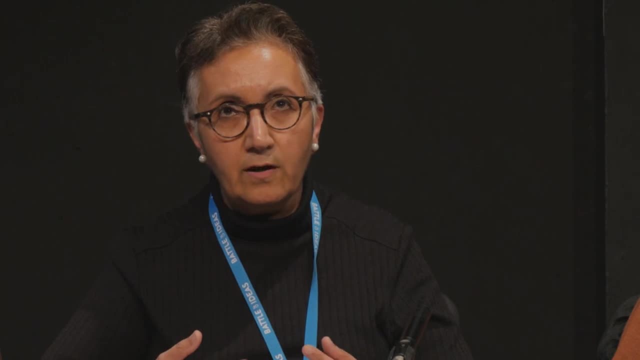 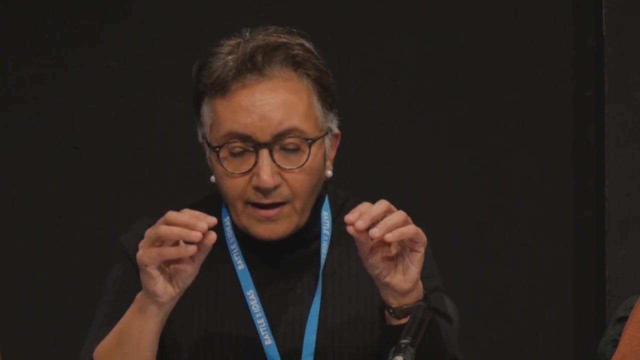 Right, So we can talk to them about reality through the holes in doughnuts or through asking them questions about take an umbrella out when it goes in the rain or you'll get wet. if you go out in the rain, That is true, But in there. that's the answer. 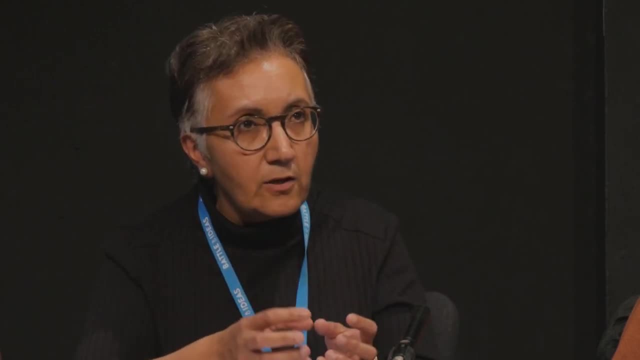 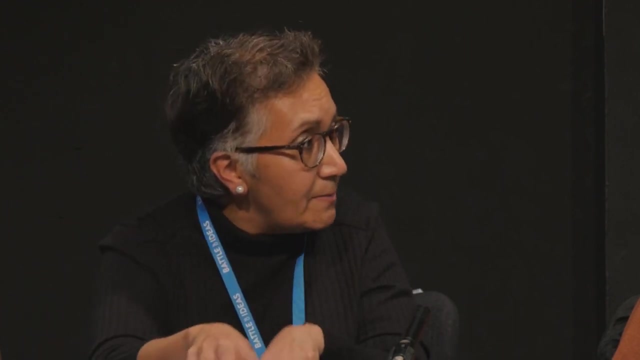 You look at it. You're using it's the orientation, the language, and your orientation to meaning in those kinds of discussions is towards the contextual. That's how it's been meaningful for young kids You use it's a language that is referring to their everyday world as they know it. 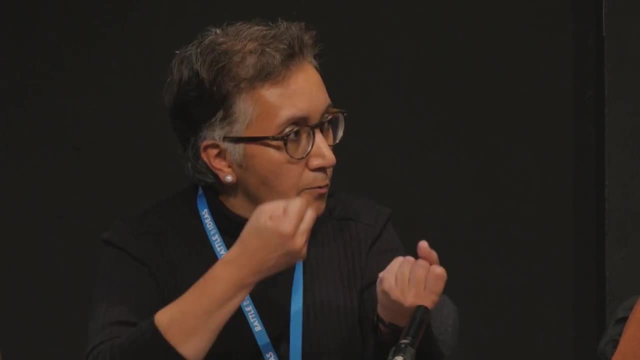 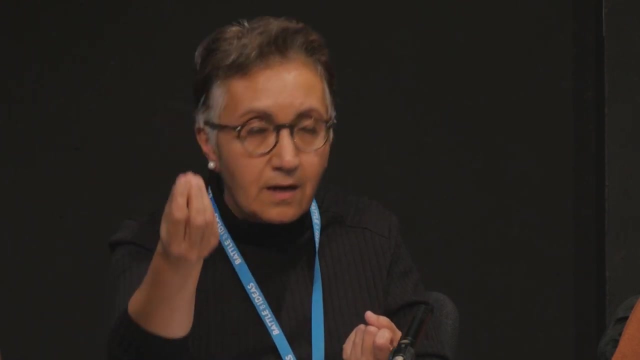 And that's how it makes sense And you can begin to then, you know, pull out a bit and make it a bit more abstract. But philosophy is different. Philosophy is when you can, when you can enter with abstract discussion without the meaning being context dependent. 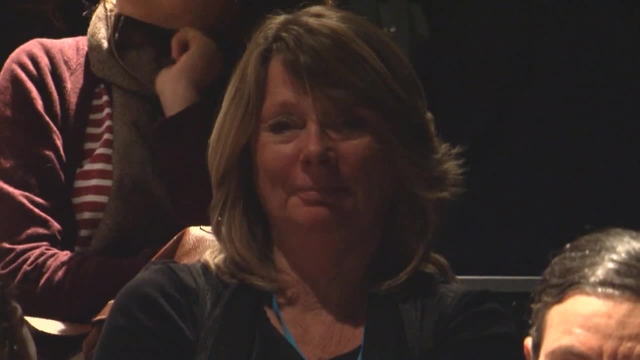 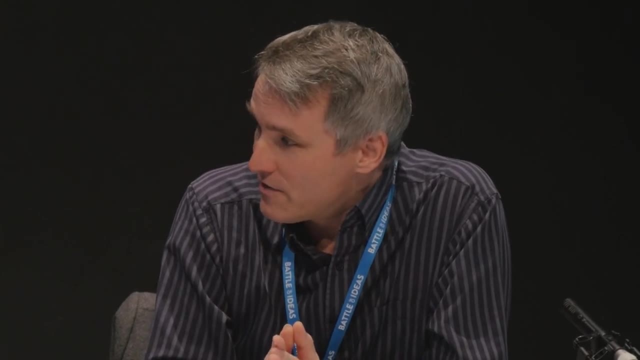 That requires a lot of formal knowledge. Yeah, very quickly. You must remember that I mean Socrates. Socrates made exactly the opposite claim of you, and a lot of people practicing philosophy will say that, in fact, philosophy only matters. 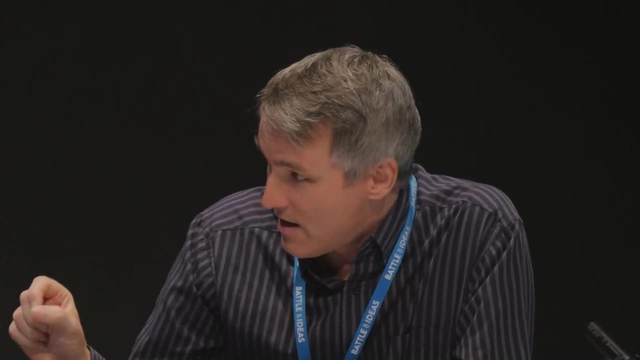 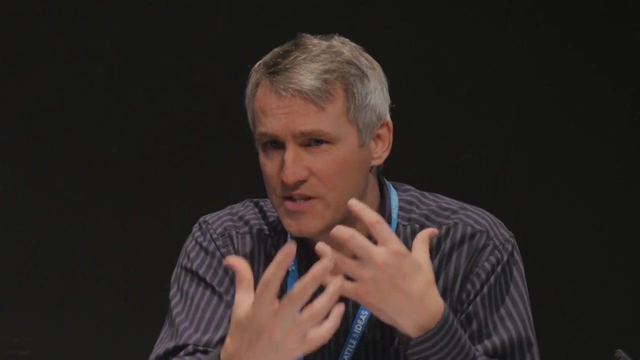 When, When it's grounded in reality. Now I'm not making that claim, I myself am not saying: you know, Socrates, for instance, would say what is beauty? And then he would ask people to define beauty, And then he would, then he would seek examples in the real world. 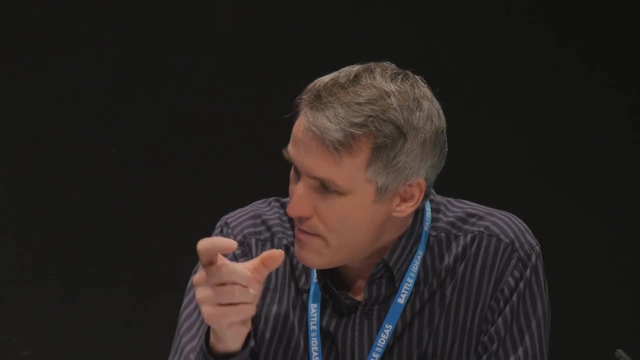 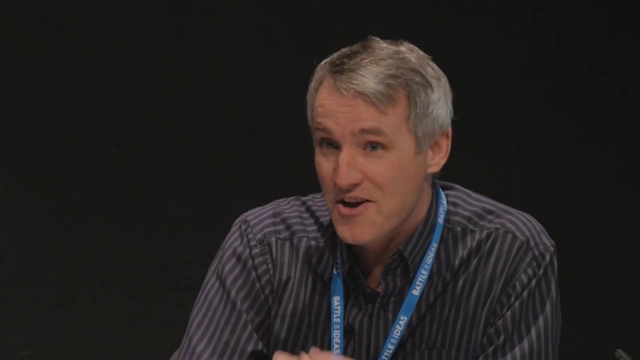 And there's a whole method of approach which is based on making sure that it always in some way relates to reality. Now, I'm not saying that philosophy is reducible to that necessarily, But it's certainly a huge great part of philosophy is this, this whole tradition of making reality and and abstraction. 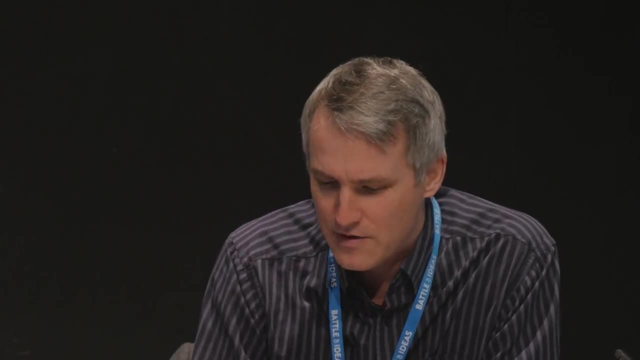 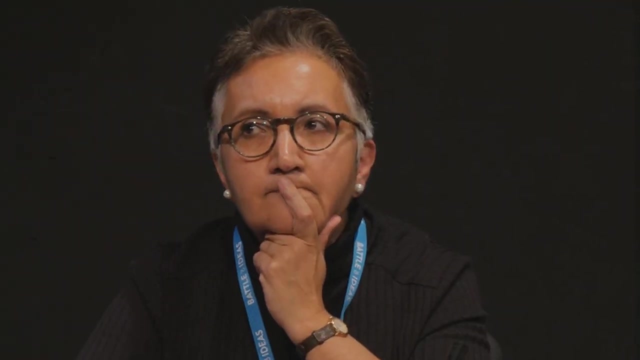 Related So. so I think it's straightforwardly false to say that philosophy is not that. OK, let's get out there, because there's lots of people to speak or point. one thing I wanted to see from this panel address, which I have yet to see, is about schools. 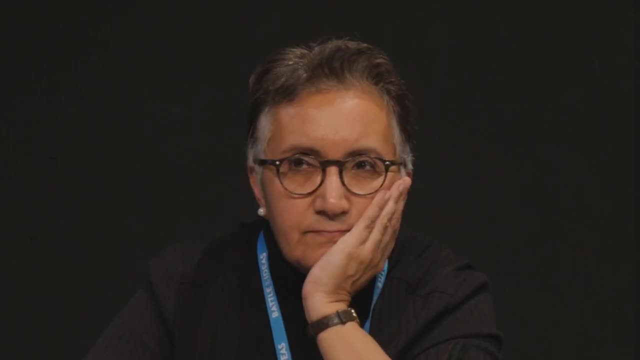 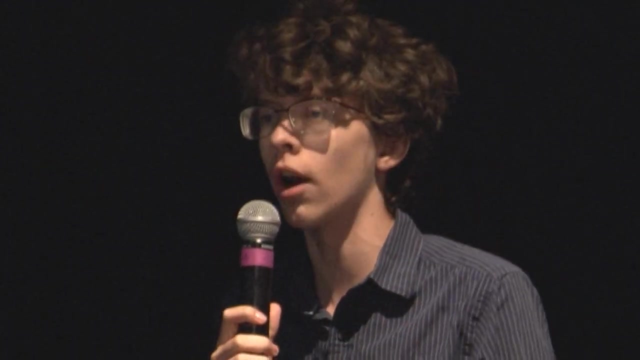 And we've heard about educational charities and summer schools And I'm not bashing that. I think that's amazing work, But if we're talking about educating children, we need to talk about schools and we're not. schools are not all carefully constructed environment for talking about philosophy. 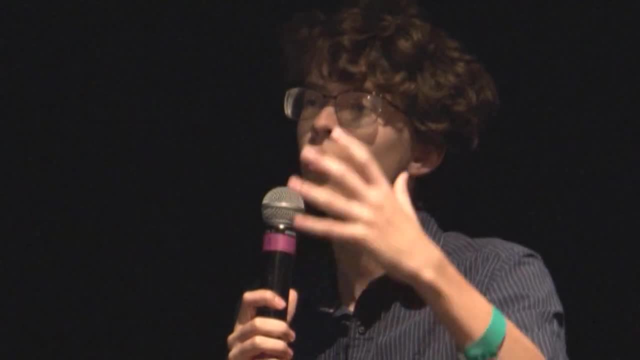 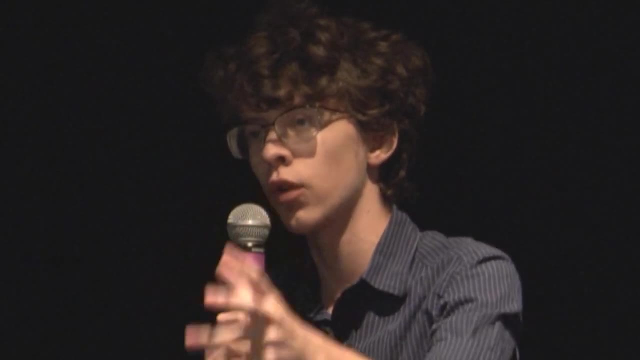 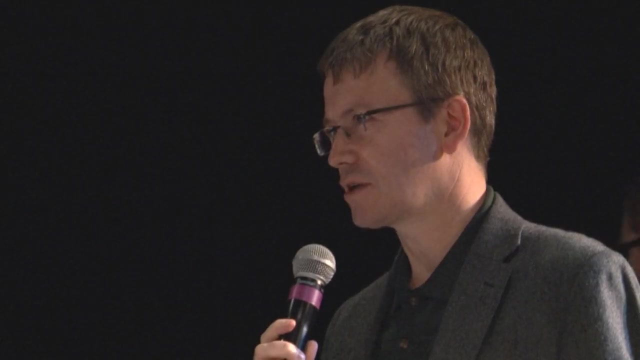 It's an incredibly broken system. So if we take that system with all of the flaws that it has, I would. I would like to. But how in the system? what would be your model to put philosophy into this environment? OK, something that struck me was that we normally, in any subject kind of deal with the kind of provisional nature of that subject, the knowledge that that subject is based on. 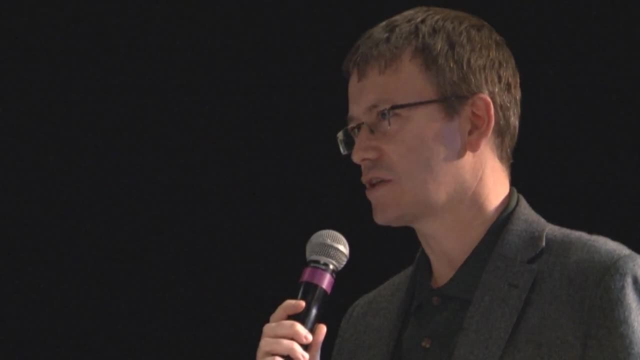 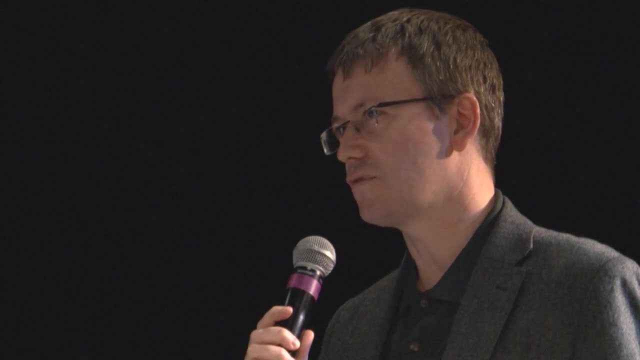 And we normally relegate or relegate, We normally leave that to the advanced stages of that, of that subject. So where we're kind of, We're kind of touching the boundaries of of that kind of subject based knowledge. The point was raised about the philosophy of science. 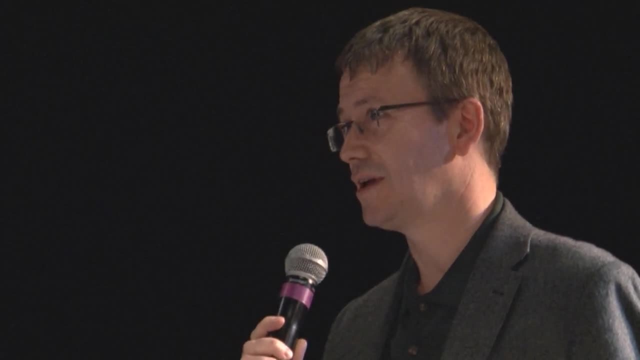 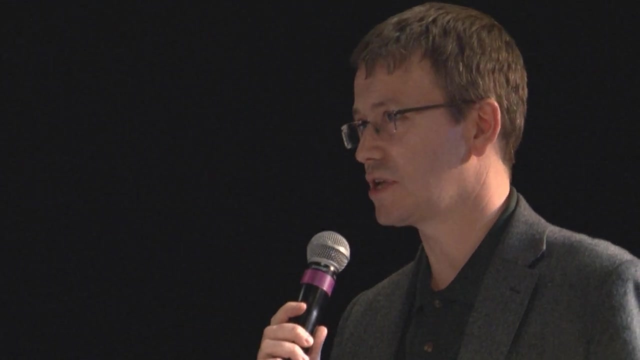 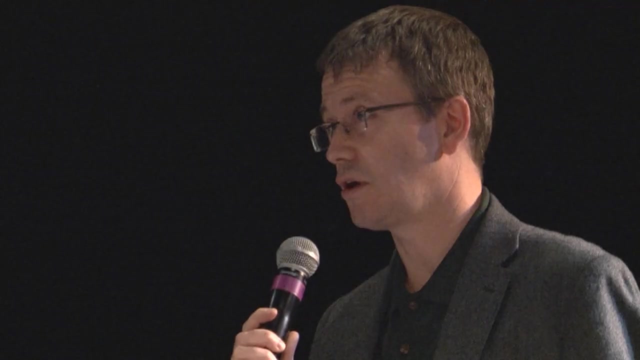 So normally, whilst you don't need to be a scientist, I would believe, to undertake philosophy of science, you do have to have a grounding in a scientific method. You need to understand what what scientists are doing and then to consider what may be the kind of philosophical underpinnings of that practice. 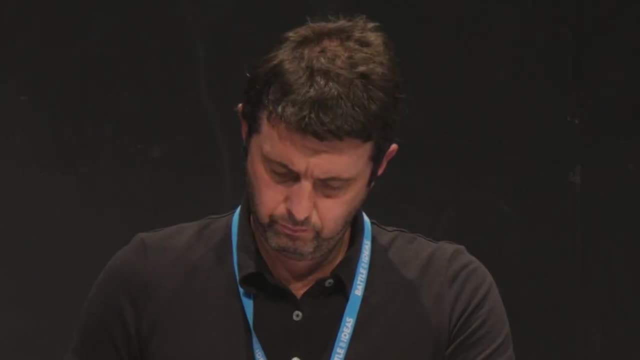 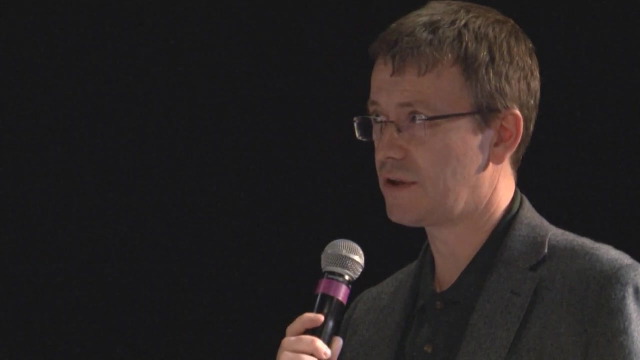 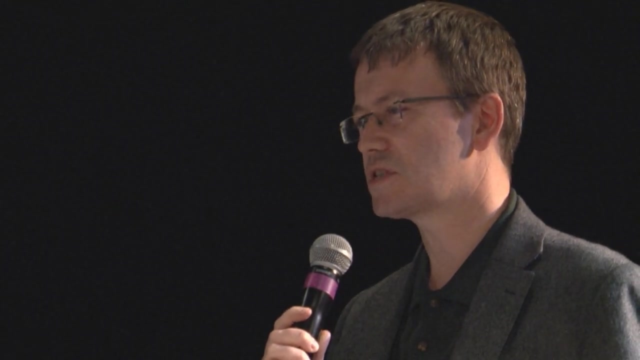 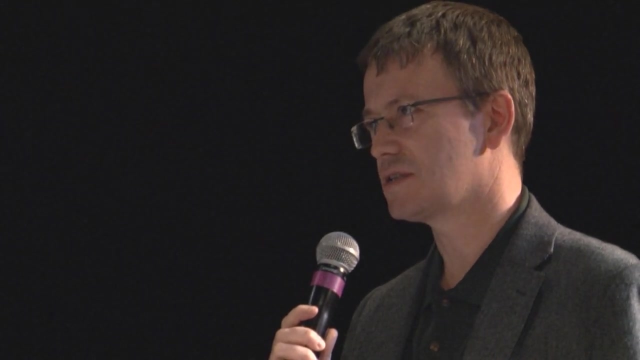 But it presupposes that you've communicated the knowledge That scientific method is grounded in beforehand. It struck me, Peter, that I think you were saying you know it's kind of the process is descriptive rather than prescriptive. It makes me really worried that the way you're describing the teaching of philosophy to children is really you know- this is where we've been here before to an extent- which is, you know, kind of education is creative play is how it's kind of striking me at the moment. 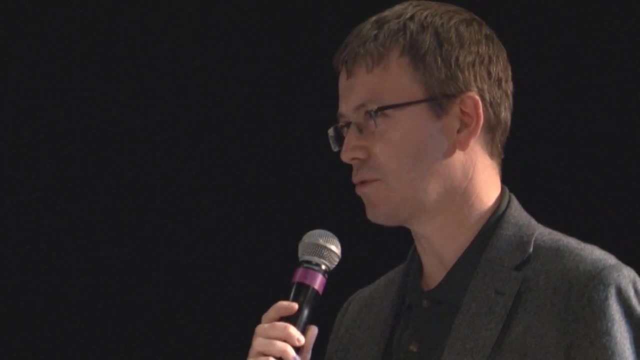 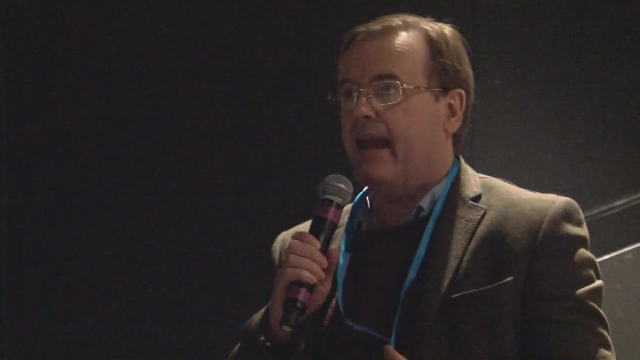 I know that's not how you see it, but I really worry that that's what. that's really what you're advocating. Thank you very much. On the question of teaching to children, the obvious question is to ask- maybe it's been raised already- how old? 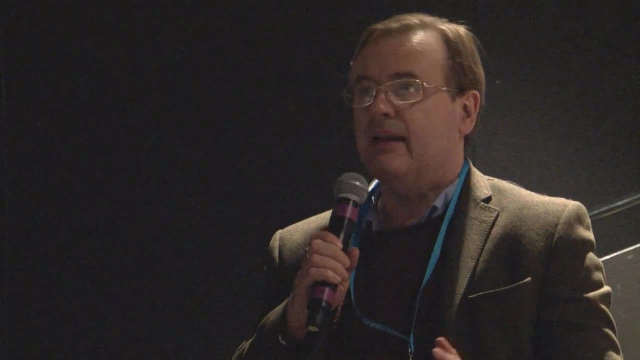 I mean there's a great difference between 5 and 10,, a great difference between 10 and 15, and a great difference between 15 and 20.. I've spent many years teaching 20-year-olds, but they're obviously more advanced than, say, 10-year-olds. 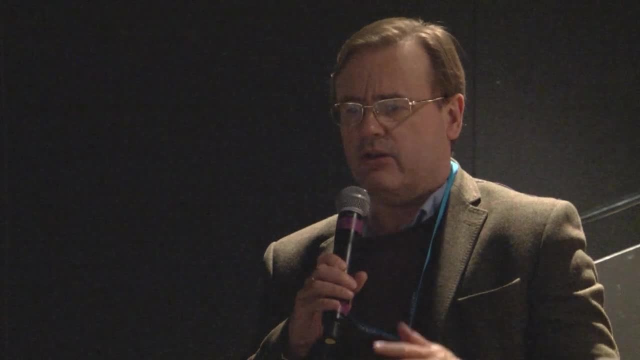 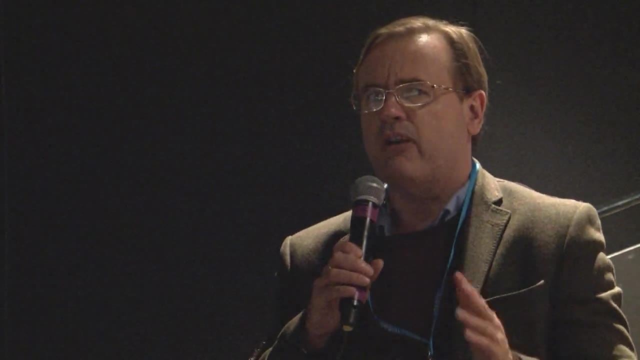 The other question is: about what is it that we're teaching? Because if you look at what philosophy journals contain, the kind of discussions which are going on in the academic journals are about things that are quite far removed in many ways to what the general reader thinks philosophy is. 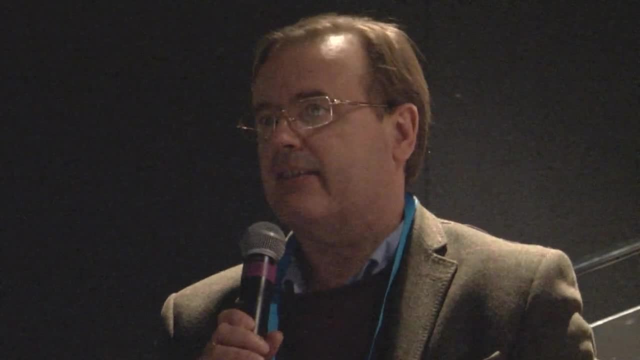 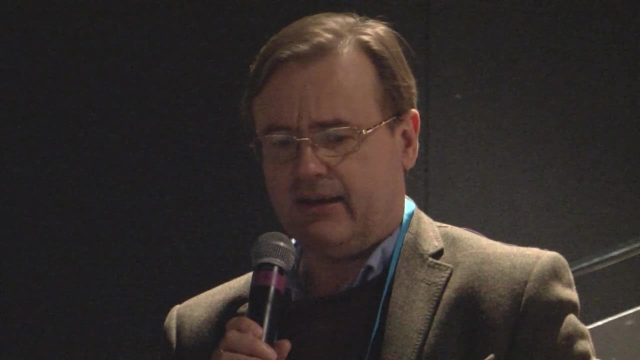 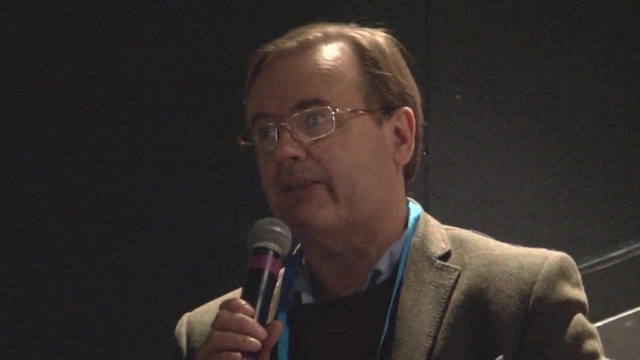 And what's presented as philosophy in the sense of, you know, ethics and politics and religion. They're both important, but there's a difference. I suggest that what schools should be doing, to the extent they can, is teaching in an age-appropriate and ability-appropriate way: the ability to ask good questions and the ability to offer good reasons. 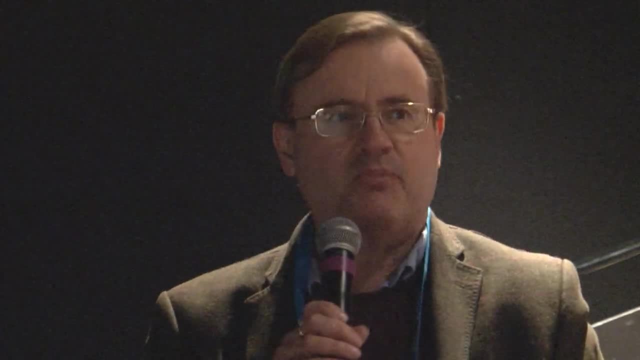 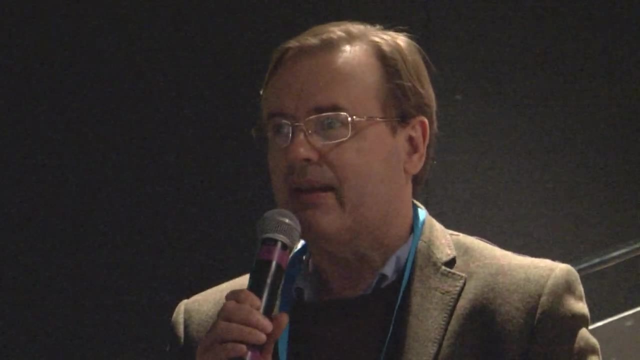 I'm worried about the idea it's all about questioning things or questioning the establishment, because that just turns philosophy teaching into a kind of dogmatic exercise in discovering some establishment and then saying what's wrong with it, And that would be rather an uncritical thing to do. 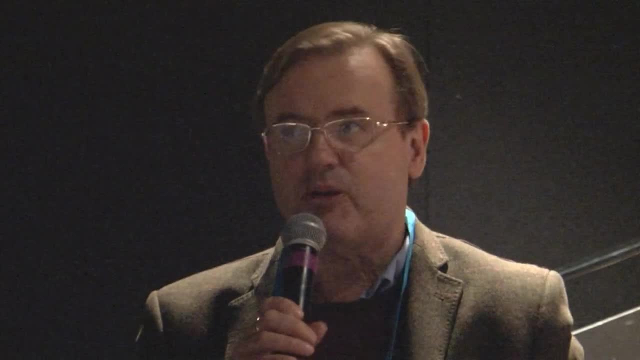 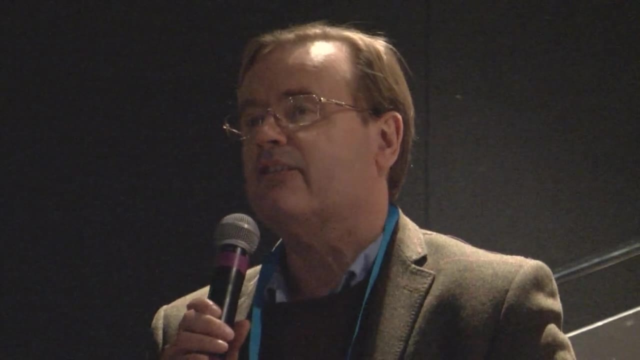 It might be quite important to see what's right about the establishment- if there is an establishment, But the ability to ask good questions that are relevant, to give reasons that are relevant, to listen to other people, to recognize that intelligent people can disagree. 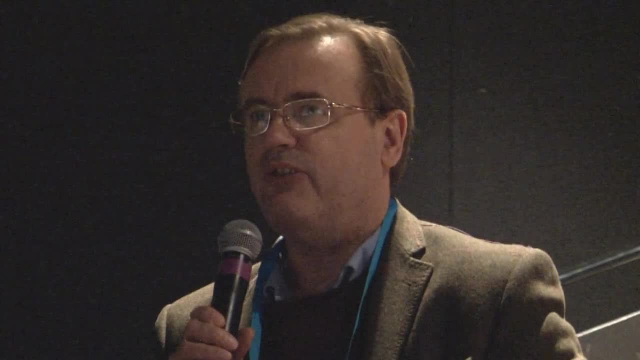 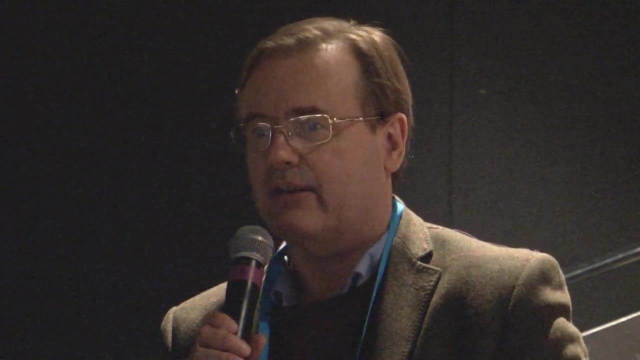 These are all processes that occur over time and philosophy can help people do that without going into the route- which, unfortunately, schools have gone down in the A-level as far as I can gather- Of just telling people facts about what philosophers have said and expect them to regurgitate. 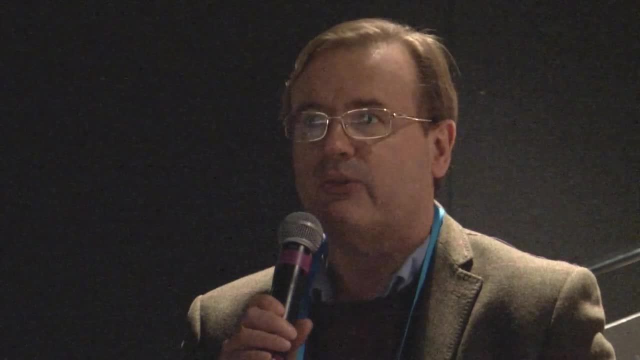 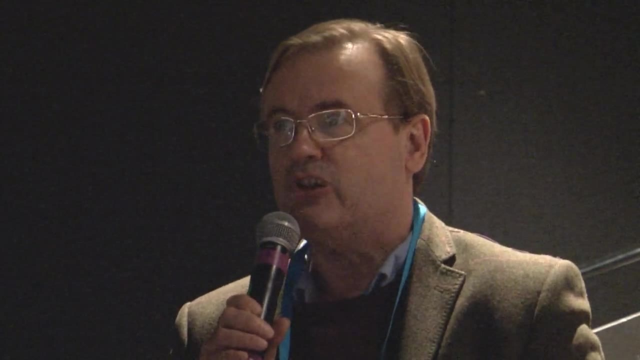 I mean for my undergraduates. I can always tell somebody who's done A-level philosophy because they regurgitate things about what Socrates said. They show no sign of understanding it, They just regurgitate it And I think that school philosophy shouldn't be like that and unfortunately it has got like that. 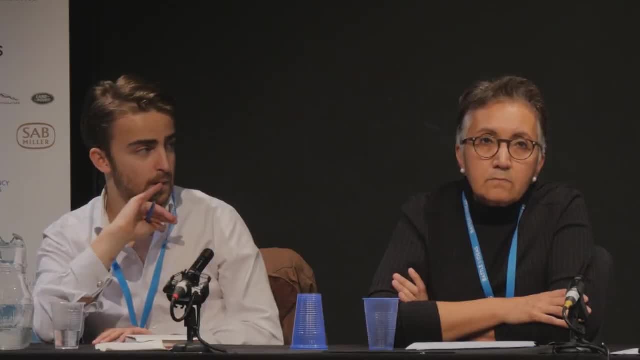 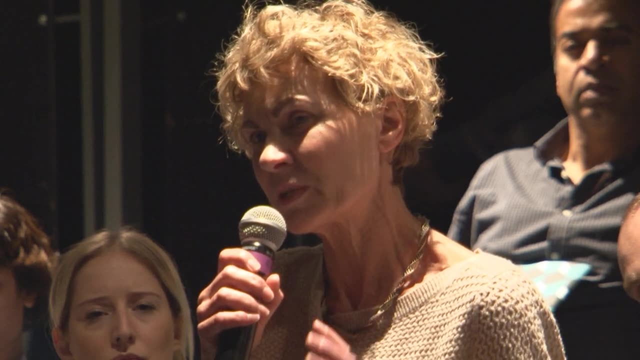 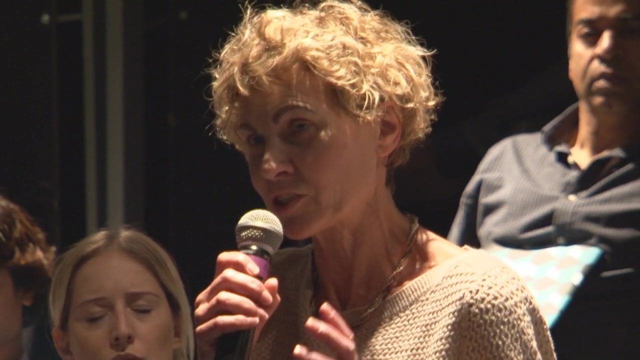 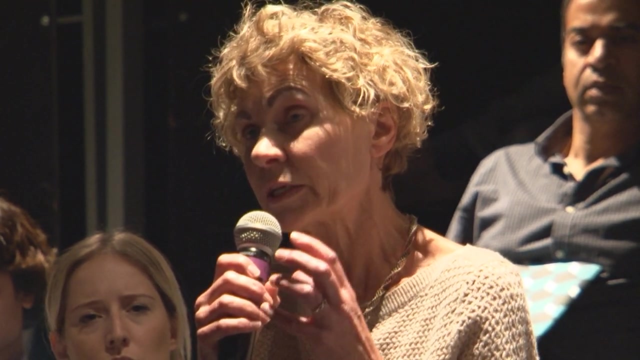 I think the statement that children are capable of abstract thinking is a very misleading place to start, actually, Because I think it does diminish in triviality, I think it does diminish the whole concept of abstraction, because all of education actually is- I would say as a non-educationist- is directed at enabling children to reach a point where they are capable of abstraction in whatever field. 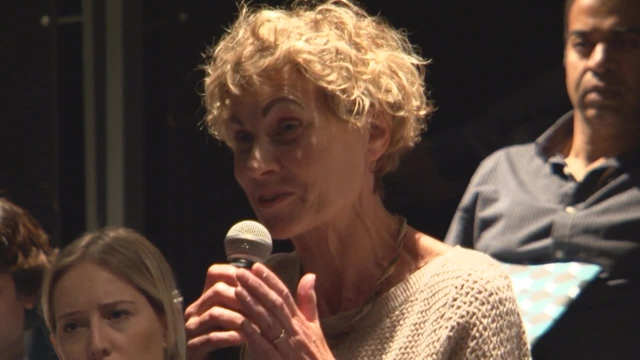 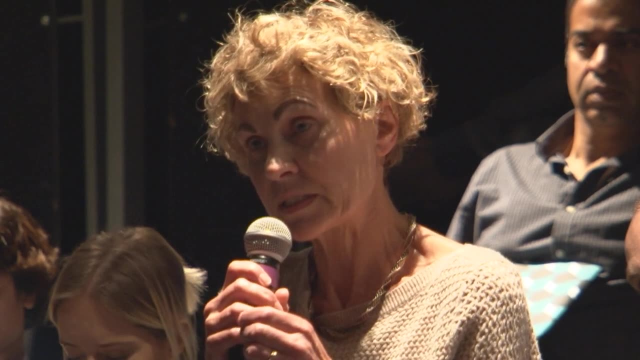 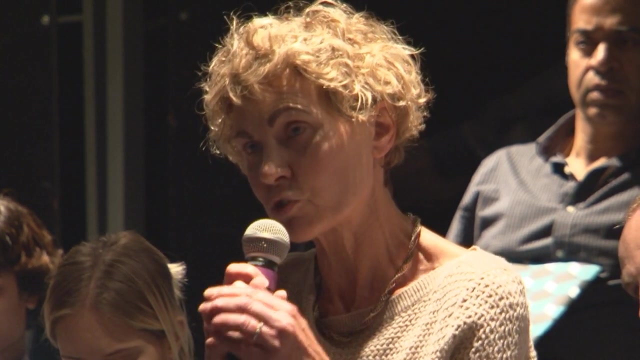 So when someone said- sorry, I think it was you, Catherine- that the curriculum is irrelevant, I would say no, I completely disagree. I got interested. I got interested in Catherine's work because I was fascinated about the idea of how children develop and become capable, ultimately, of abstract thinking. 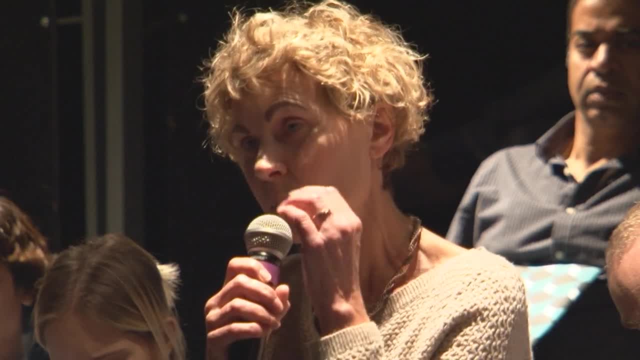 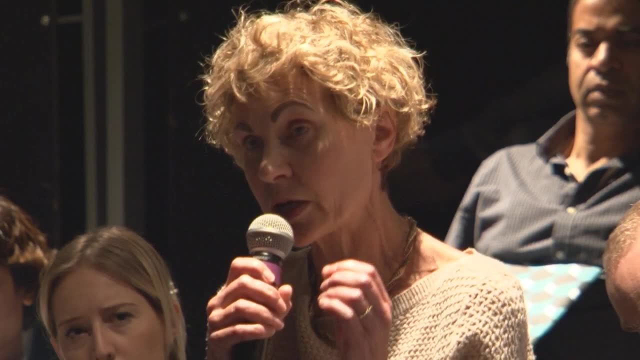 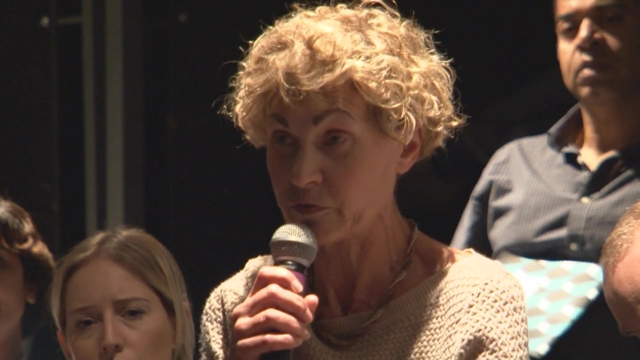 And I started from Vygotsky, who made the point that all the curriculum subjects could be used to allow children to develop abstract thought. And to give you just one simple example, At the level of a five-year-old, there's the whole thing of reading right. 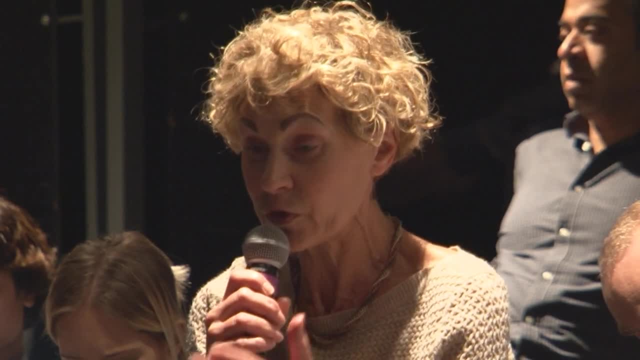 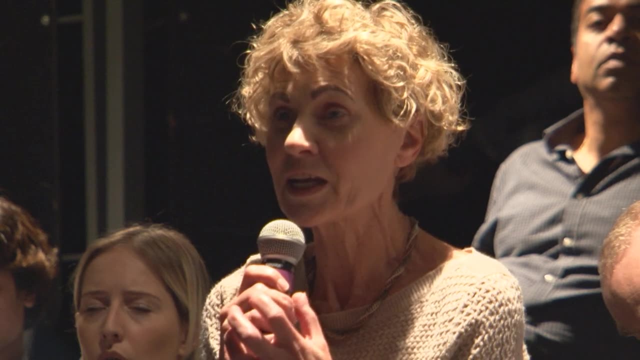 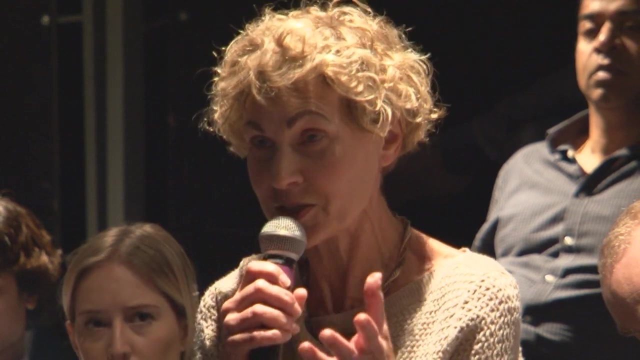 And Margaret Donaldson, the educationist, made a very, very neat point- that children come to school very, very able to talk. They talk about a lot of things. They're able to ask questions, answer questions and all sorts of things. 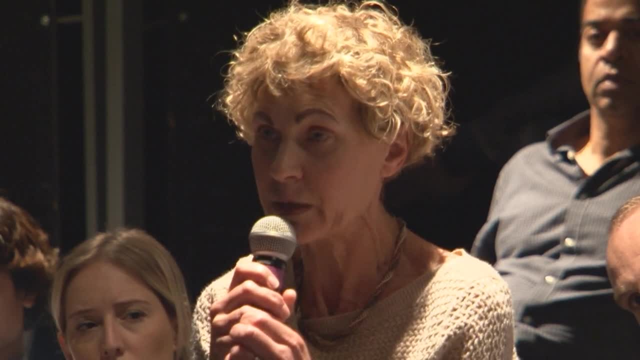 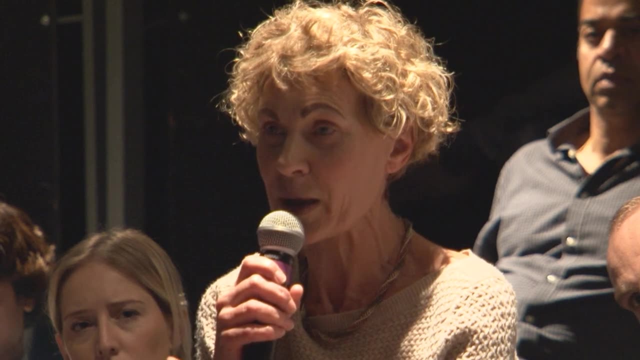 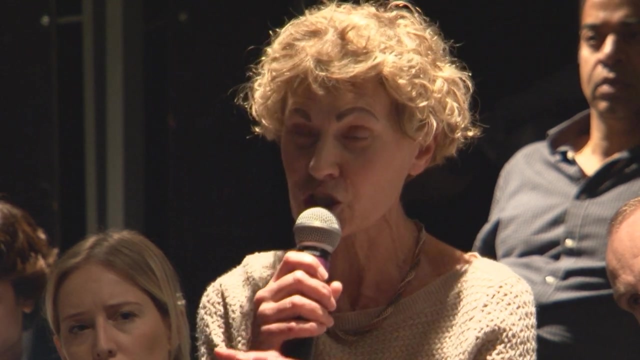 But it is only children from middle-class families who have Any idea that behind what they're talking about is a system of grammar, And it's really that first critical stage in which children can actually become aware of the system behind what they're verbalizing. 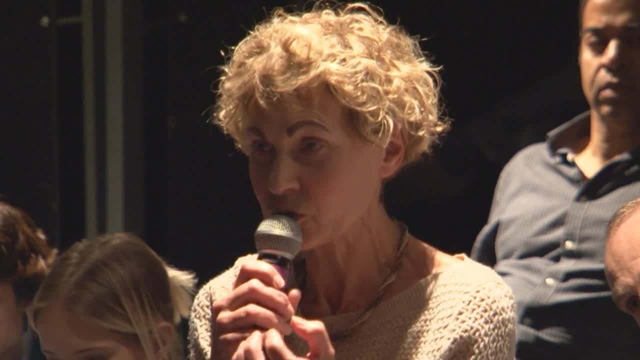 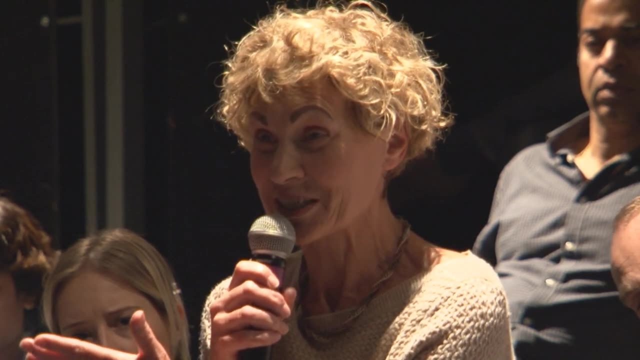 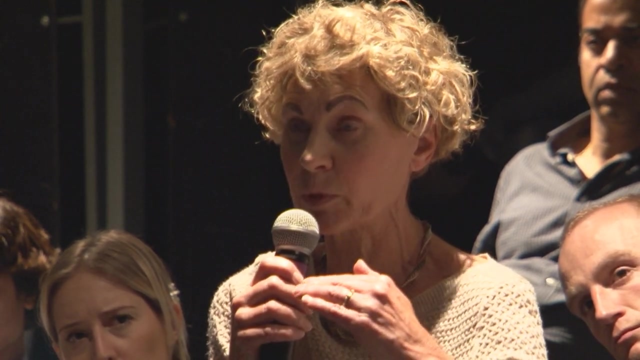 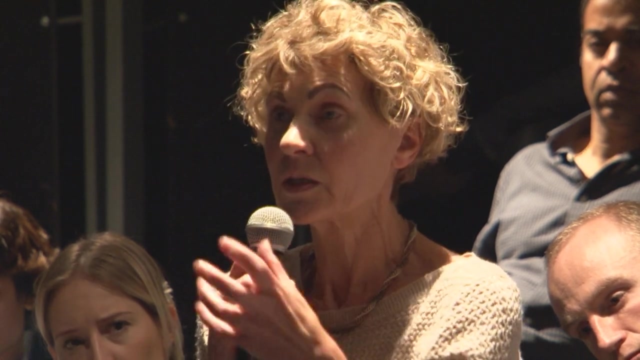 That is the first step towards abstract reasoning, But that is a very elementary thing, As people, I think, have made the point. you have to grasp an enormous amount of empirical knowledge before you then become capable of taking the next step, which is abstracting from the general to an abstract concept or system. 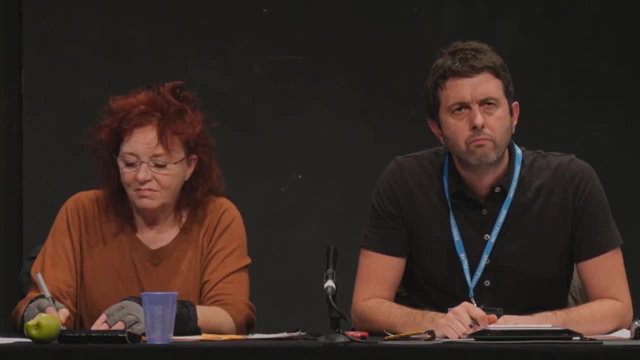 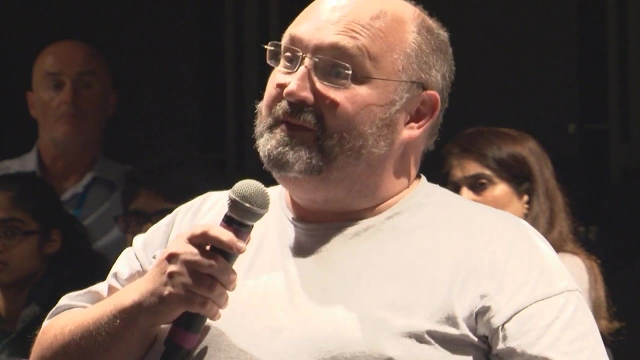 Yes, I'd like to agree with Alka about quite a lot of what she was saying. When you were saying, Catherine, about what the word can meant, the one you missed out was permissive, as in: should children be taught? Well, that's the thing. 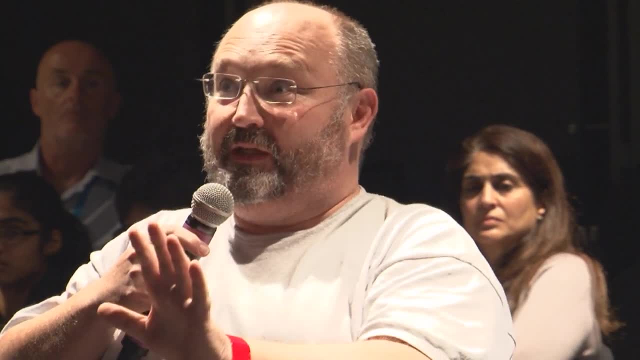 I mean this is about. I'm not sure I agree with the way the question's gone, but it's whether they should be taught or not, or the idea of being taught, And philosophy doesn't have a stranglehold on higher-order thinking. 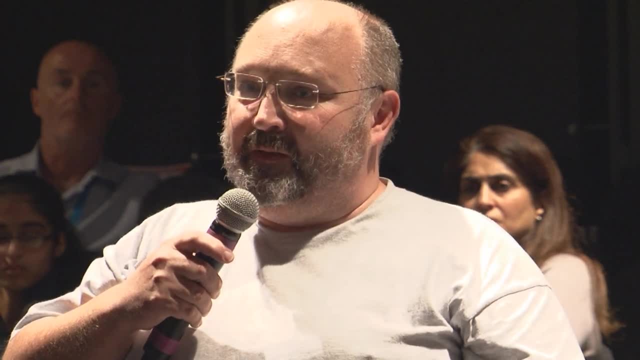 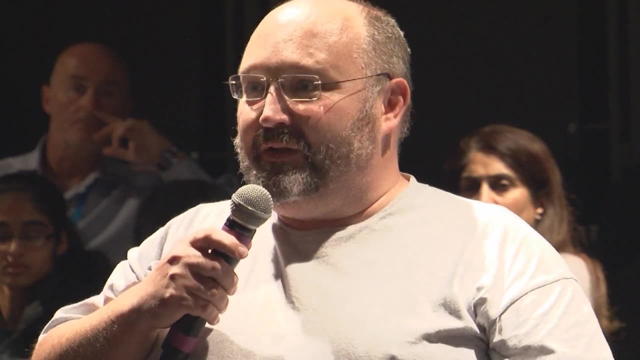 And what I worry is that- and I agree with what Alka was saying- that if you look at the way the education system's going- and I'm actually from Elgin, so I know all about Scotland, the education system there- One of the things I worry would be: 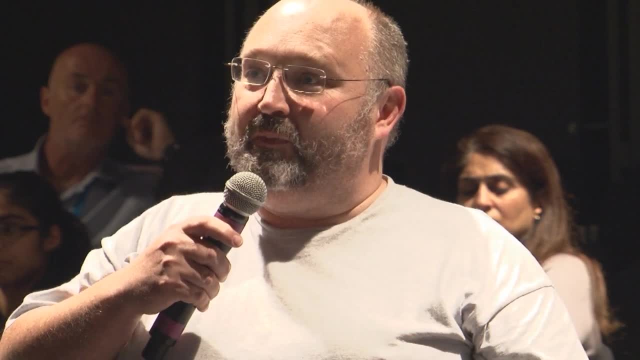 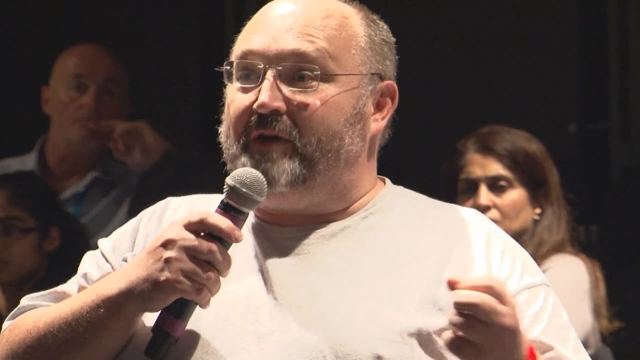 if it were to be a case that children were to be taught philosophy, it would be as a sidecar, It would be slapped on the side And it would allow the governments and the education departments around the country to extract the higher-order thinking from other subjects. 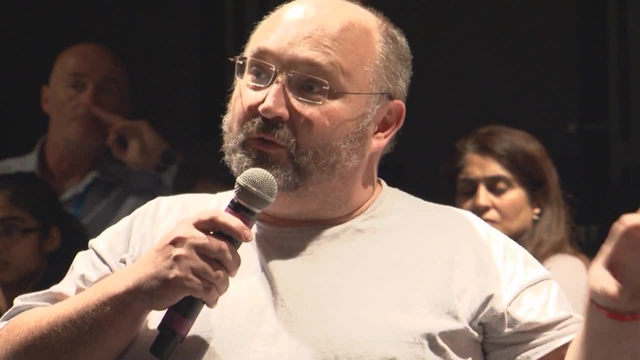 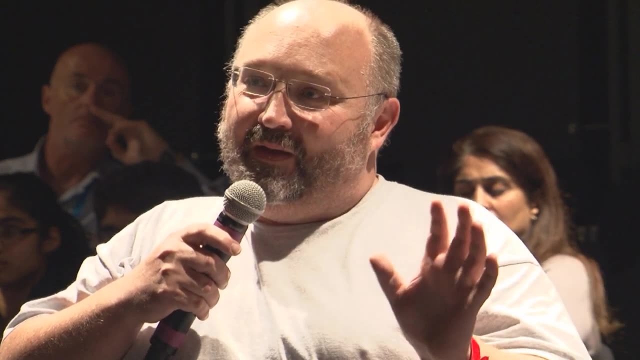 and put it on to the philosophers and say: and that's your job to do, And I think that would do a disservice to the children and to the study of philosophy. So I just think that if we could maybe move the argument back to 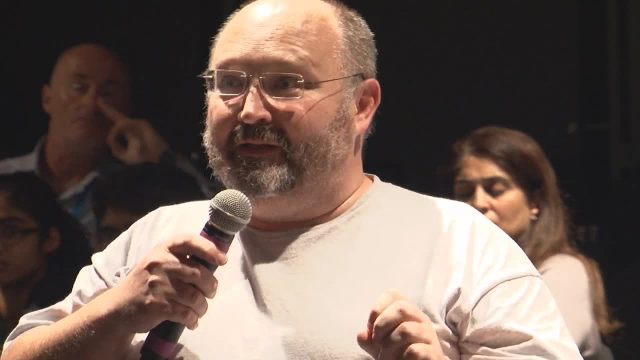 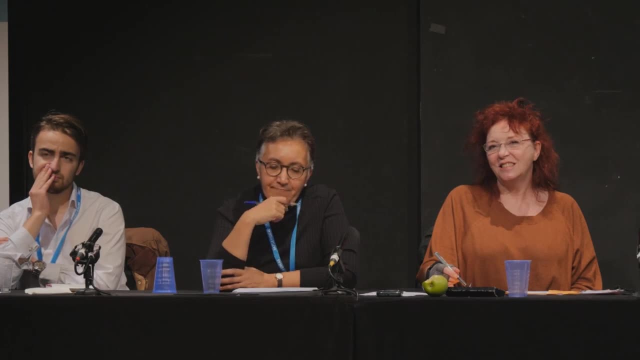 can they do it? I think they can, but can they do it rather than should they do it? I think that might be more slightly less contentious maybe. I've got three Fs to respond to some of the questions. The first one is fear. 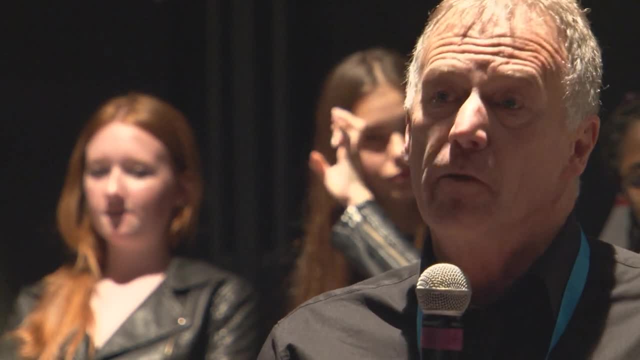 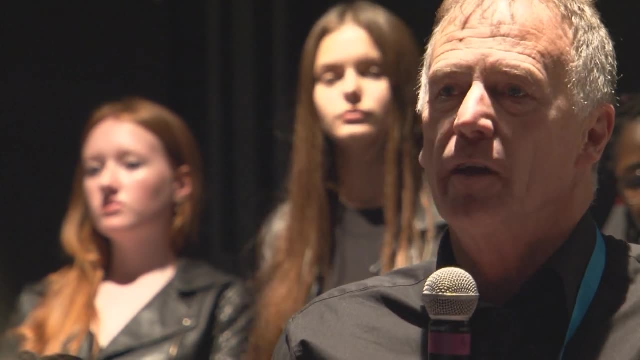 I recommend you Paul Boghossian's book Fear of Knowledge- You can get it as a PDF- And the climate we live in, where there is a fear of knowledge- and he says it's a cultural mood, right, We fear knowledge. 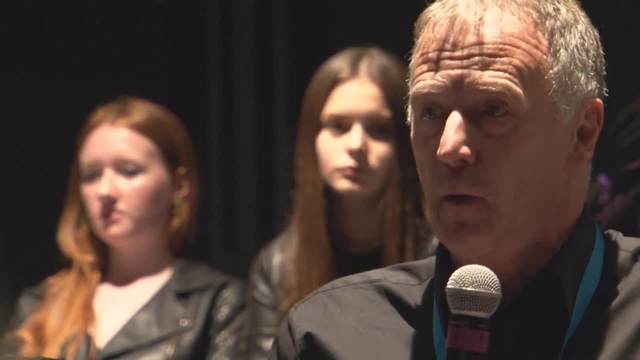 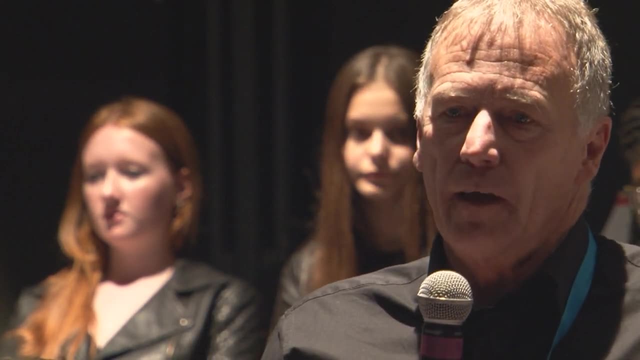 And into that cultural mood philosophy seems to fit very well. You know, Angie Hobbes pops up every ten minutes on the radio using Plato to try and solve some contemporary problem. But the other F I've got. I think it's flattering. 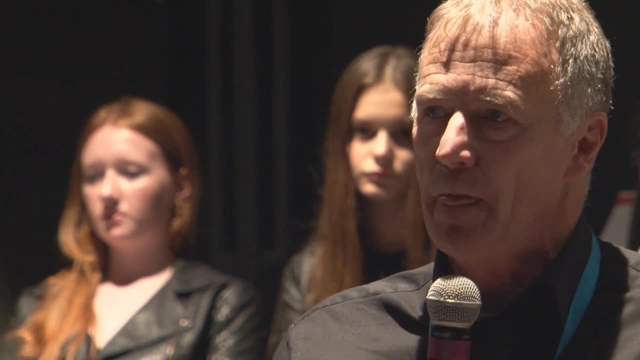 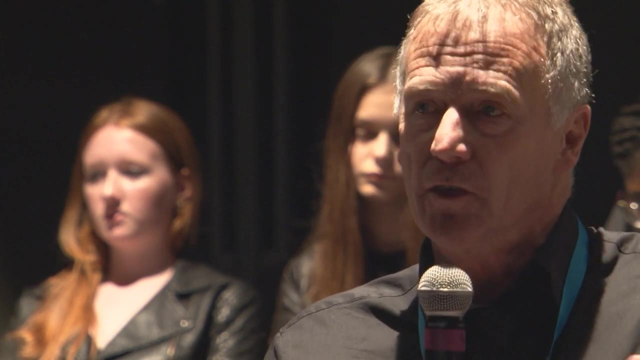 The great motivation here. it's flattering both to teachers and to pupils, Because a contentless subject where you're just questioning and thinking flatters pupils. I remember an A-level student who dropped French in favour of philosophy, because you don't have to learn all the verbs, you can just argue. 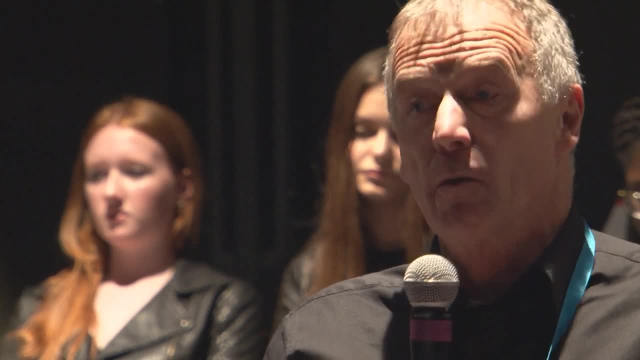 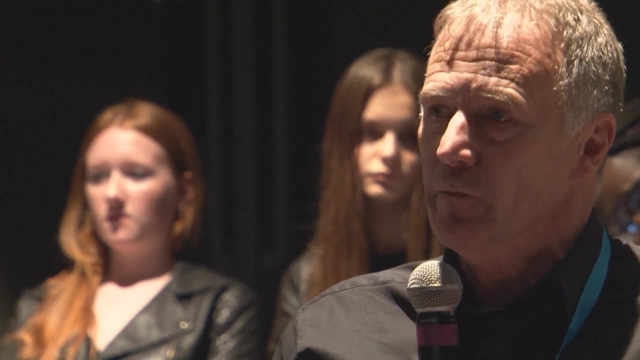 It's a very appealing thing. You think you know something when you don't know anything. you just argue and talk. It's very flattering. Very flattering for teachers who seem to think they've got the secret of the universe in their hands, you know. 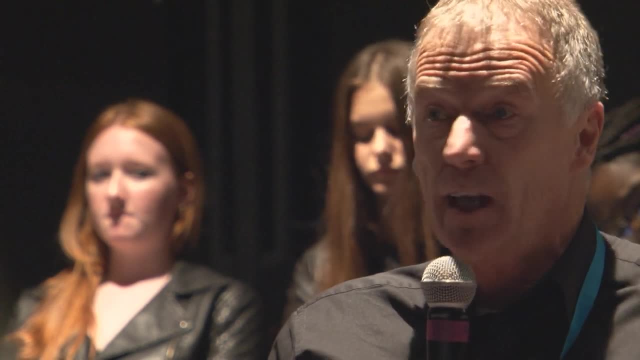 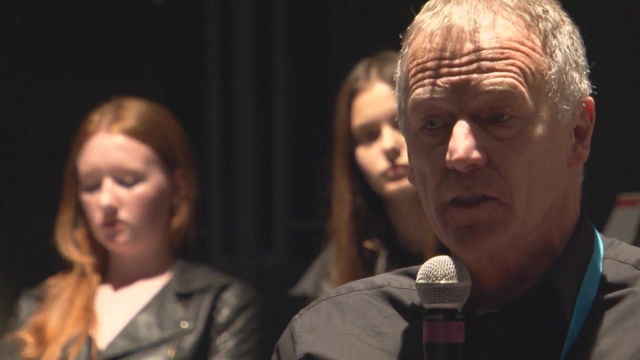 Get children to think critically and adults will be able to think critically. I think there's too much criticism about, by the way, there's too much political cynicism about everything. It's dead easy to criticise, right? I just think it's completely wrong. 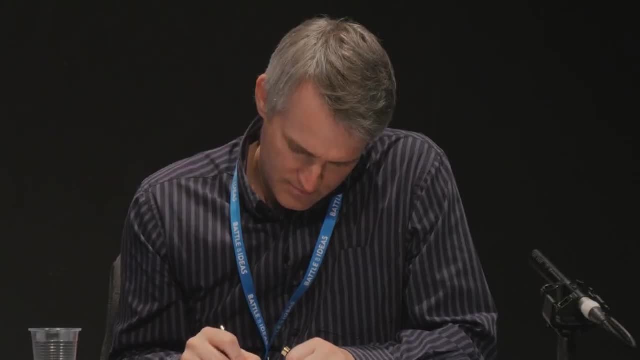 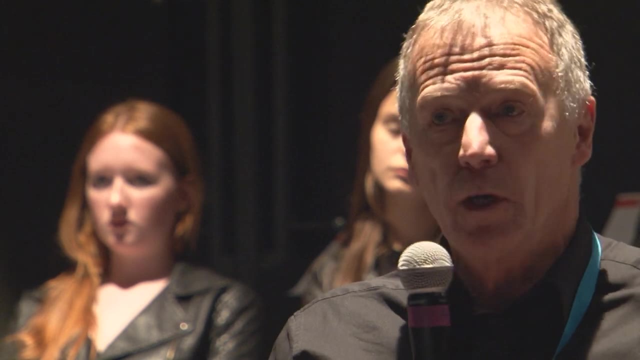 The third F is flummoxing. I was quite interested in philosophy, I'm a philosopher, But the more I hear you talk, the more I'm confused. And what's happening to those poor kids when they're asked these questions and you know, you lead them down the garden path. 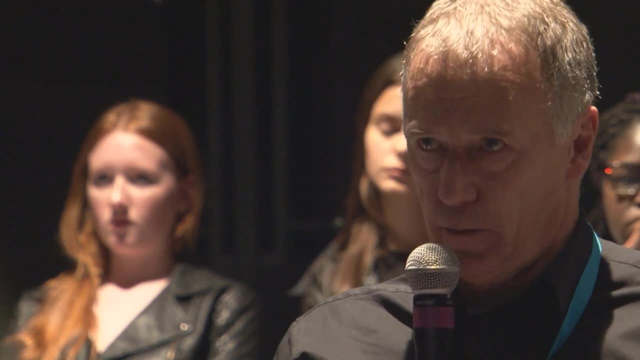 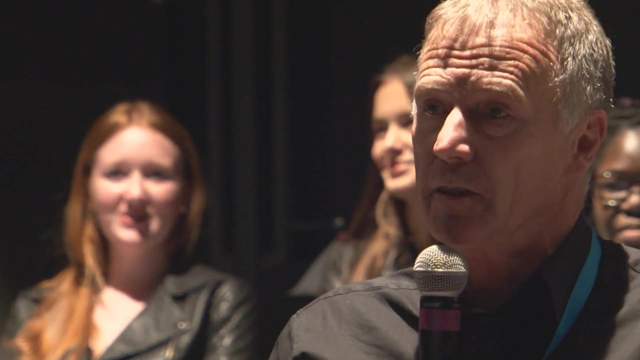 talking about holes in doughnuts. It's almost childhood used to me. I'll just tell you that. And I've got a solution to the question of what philosophy is. There isn't a solution. There is no philosophy. There are philosophers. 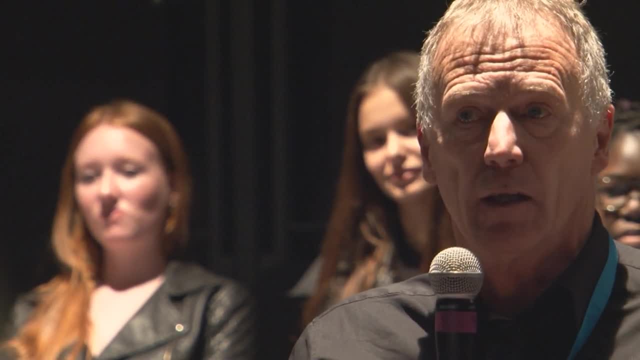 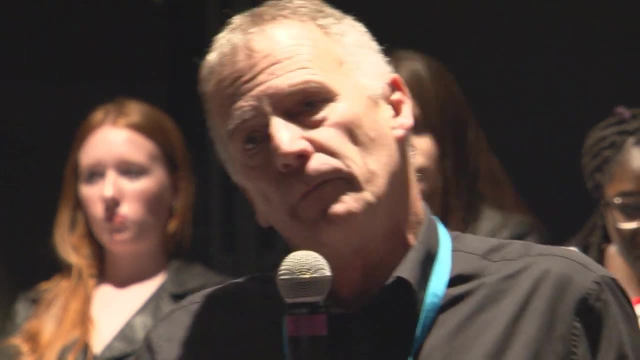 And I spent a lot of my time studying Wittgenstein, later Wittgenstein, Wittgenstein for a while. So I wouldn't say you could teach philosophy, but you can teach philosophers, And one of the things I would do- in contradistinction to Piers- 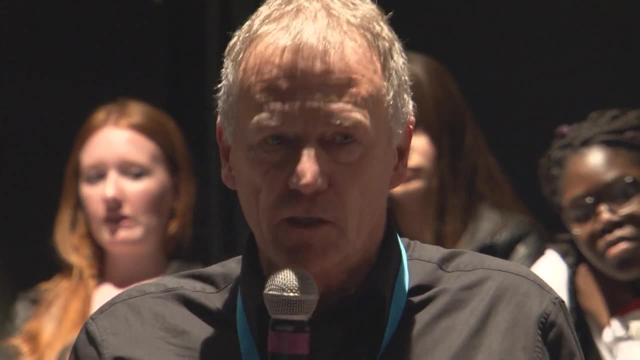 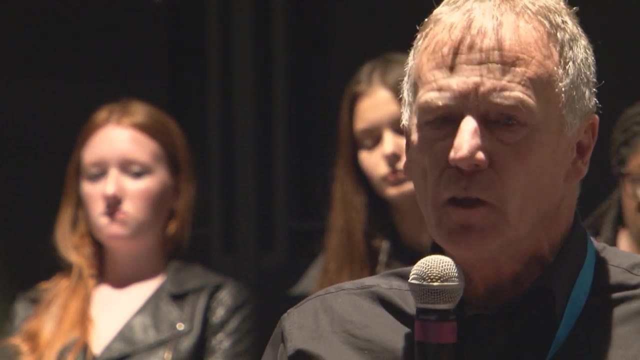 is teach the history of philosophy. Have kids knowing things. You can do Emile in French, you can do Plato in Classics. You can keep them in the subjects, but they'll actually know something. I've stopped banning students who want to have a discussion. 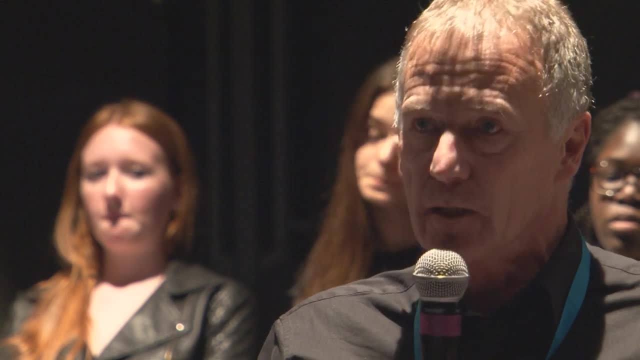 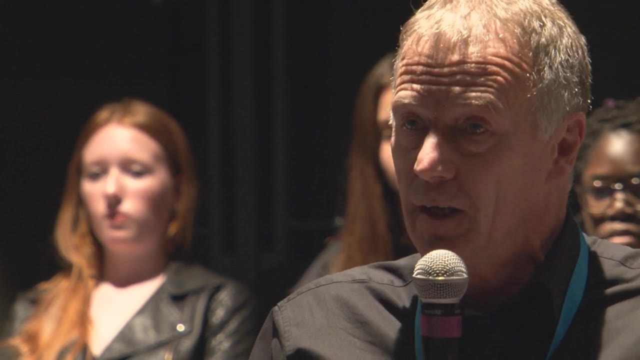 with Plato when they haven't read him. Never mind, they haven't got any ancient Greek. That's where the problem lies in interpretation: If you don't read it, you can't talk about it. So get people to talk when they've not read Plato or anybody. 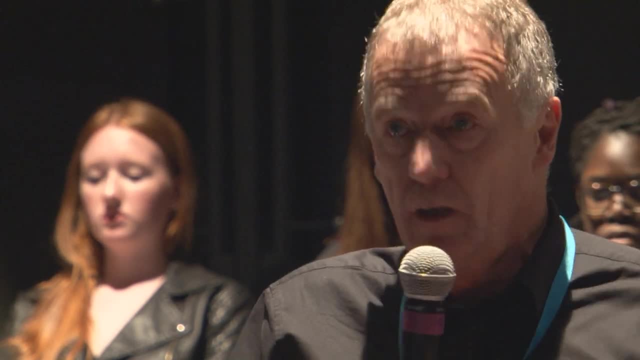 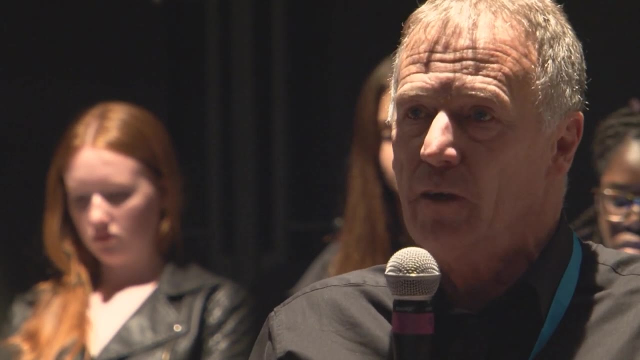 It's pointless. So let's go back to the things that Plato did, where you got pupils to learn the heuristic. just go through the heuristic arguments and have some real understanding, And that would be much more beneficial than just doing this, which in the end. Catherine used that awful word. 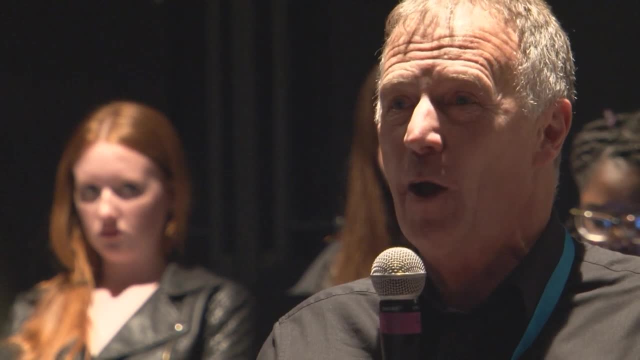 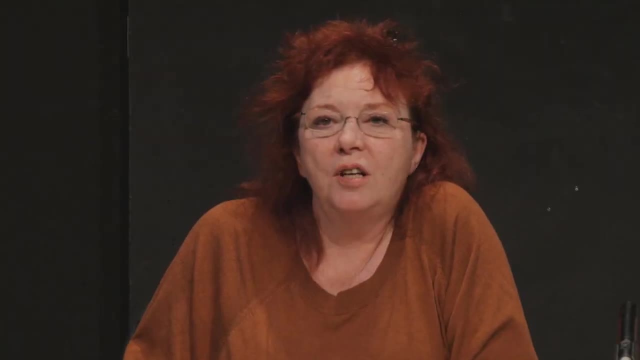 make them more reliant. It's a sort of therapeutic thing about all these things. I'm all in favour of teaching children the history of philosophy and myths of ancient Greece and Latin and Greek and lots of, But that's a question for educators, for schools. 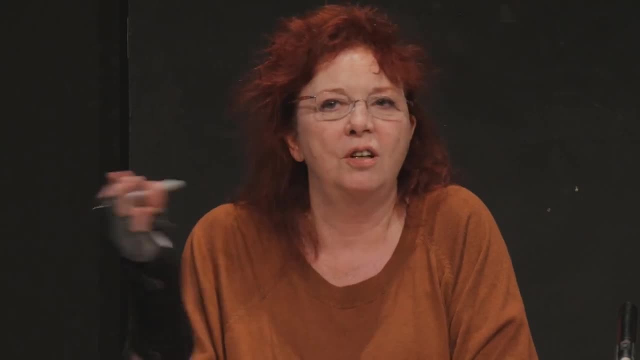 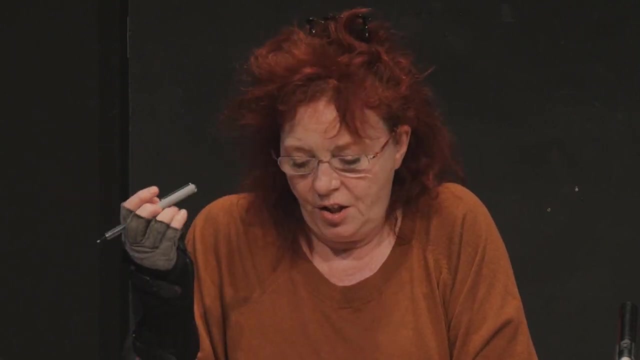 I'm not. I'm not a teacher. You know that's their choice. They want to decide what they want to do. I will advocate philosophising for everybody, for children, wherever children are. If they're in schools, they're in schools. 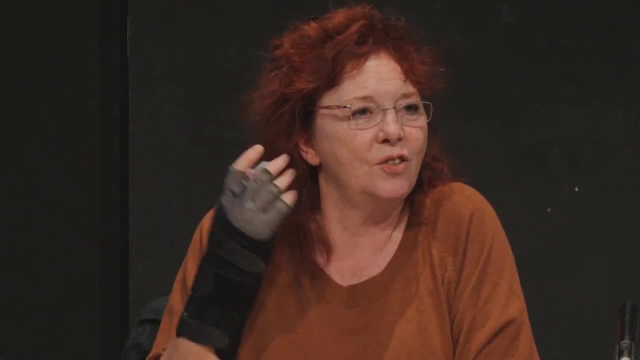 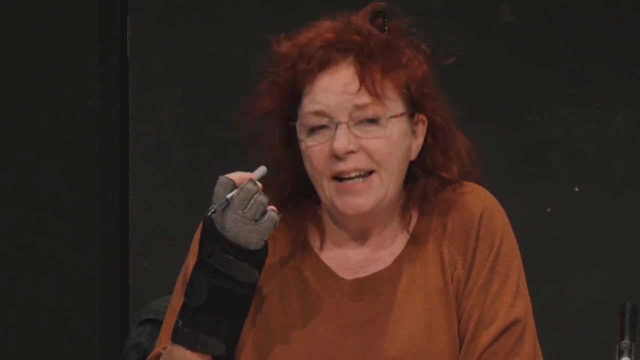 If they're not, I do that. I'm on the other side of schools, So I don't think it's necessarily an education question. this, This is much bigger. It's a life question. Now the question was: can children do philosophy? 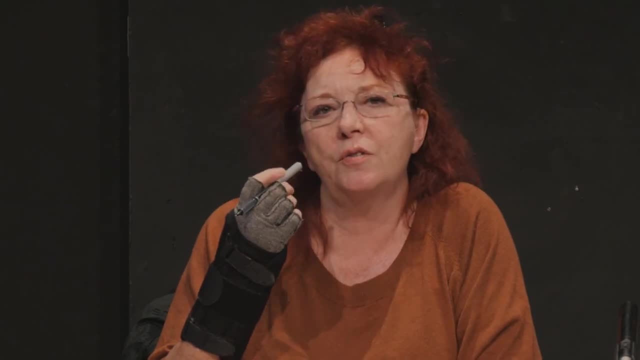 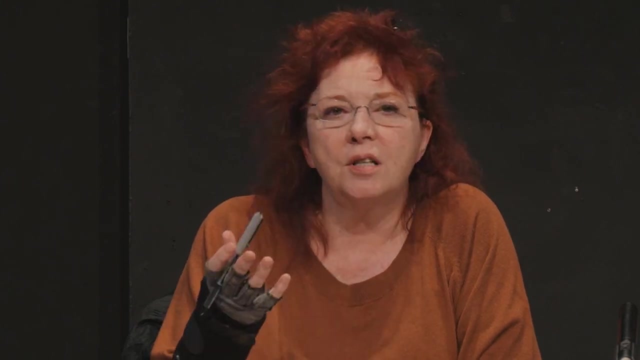 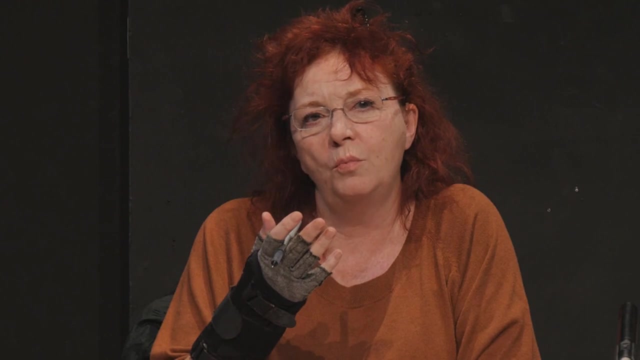 Now, doing philosophy is not the same as learning philosophy. It's more like philosophising. It's not discussing Plato and Kant and comparing, you know, seeing if Kant really responds or adequately answers Hume, It's doing philosophy. And I could tell you just a little story as the origin of this. 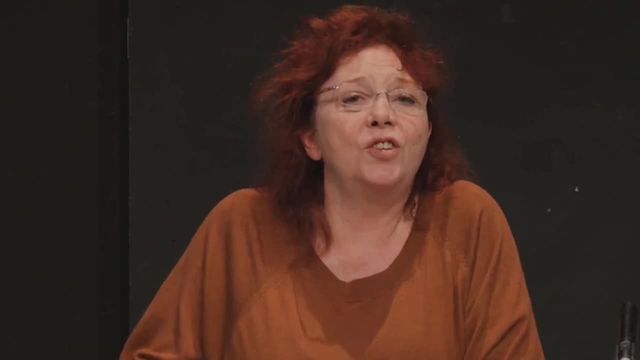 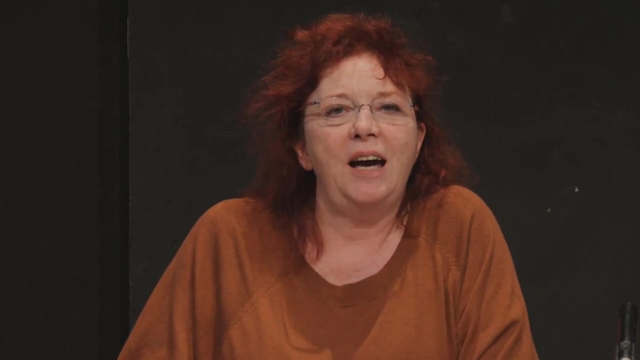 Again. you could read it in my book Transforming Thinking, The origin of the method that I used back in 1970s as an honours philosophy student. I wanted to capture something of what professional philosophers did amongst themselves, not what they wrote in books. 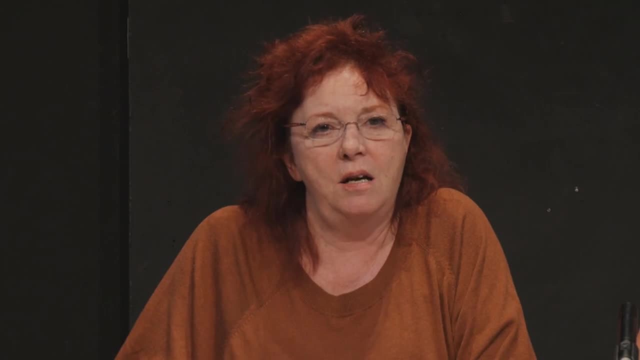 not what they lectured to us, But there was something missing in our philosophy degrees And I studied pure philosophy nothing but for four years at Trinity, And this is how I developed this in the metaphysical society at Dublin University. I developed it first for adults, not for children. 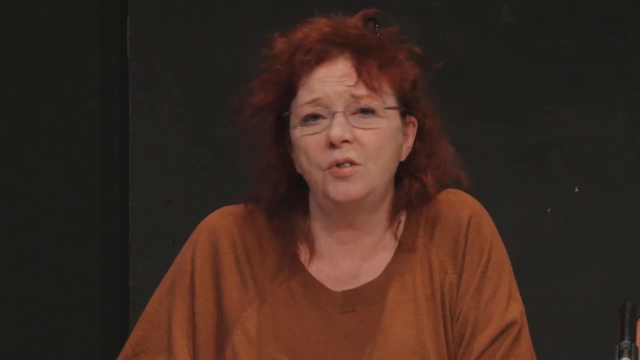 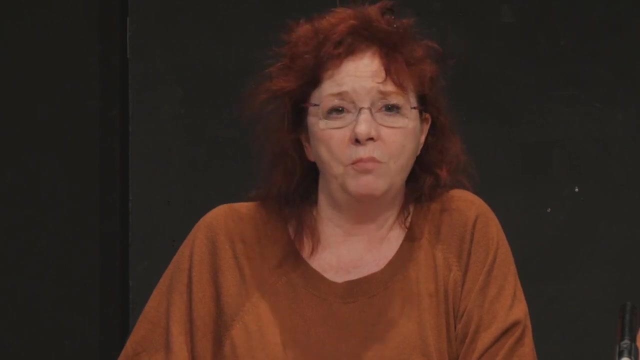 I just adapted it a little bit for children, because I see no difference between children and adults. They're just different ages to my mind. But it's something that was missing from university philosophy And when my son went to study philosophy at university, having done COPY most of his life. 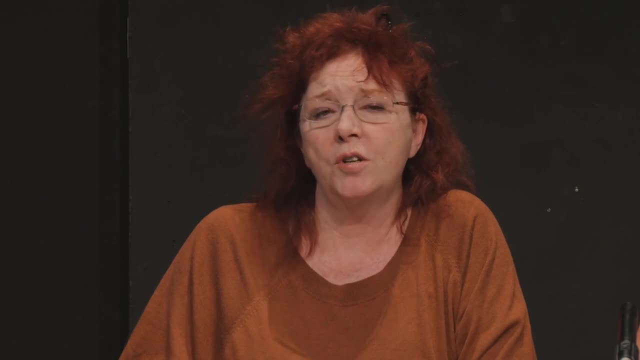 he was really disappointed because he really wasn't. Although the lecturer said: we want you to do your own thinking, they didn't. When he did his own thinking, he was penalised And I said: look, they say that, but what they really want is for you to regurgitate their opinions. 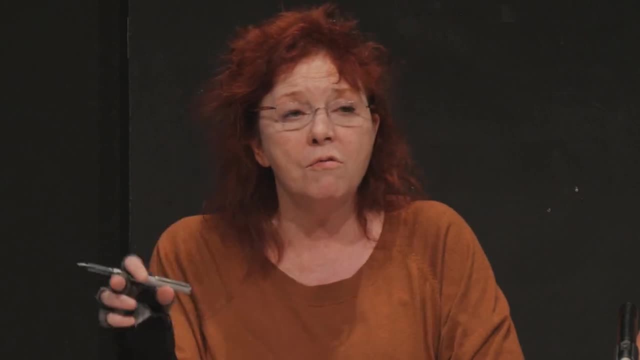 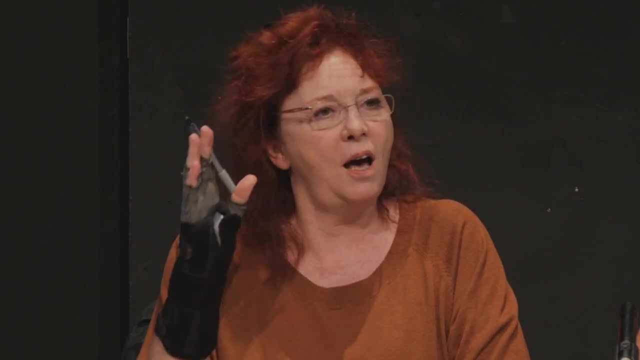 their lectures in your language, So they see their own thoughts coming back to them, but in your language. that will flatter them. He did get a first. He won all the philosophy prizes. But what, What? it reminded me, and I remember saying something to Pete about it at the time. 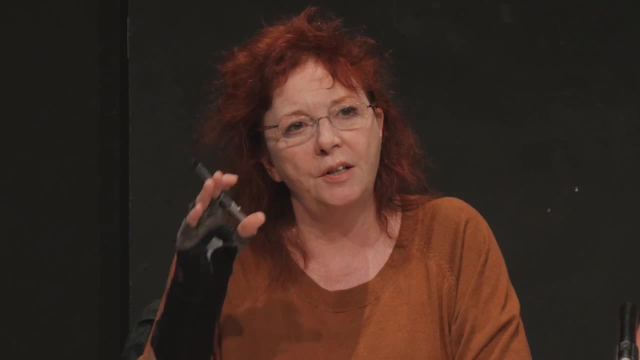 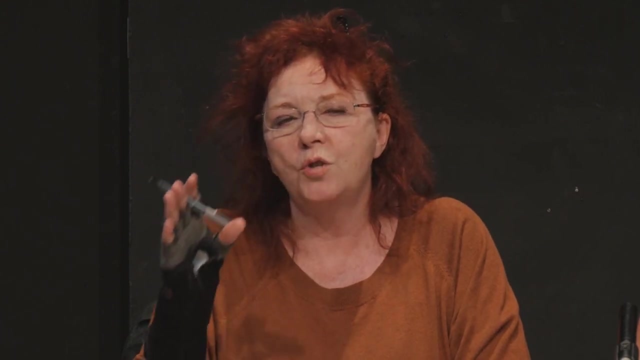 that actually part of the origin of COPY- that I do with little children, as you can see in Socrates for six-year-olds- was what was missing from university philosophy, which was students philosophising for themselves, which is only what the professors and serious you know. 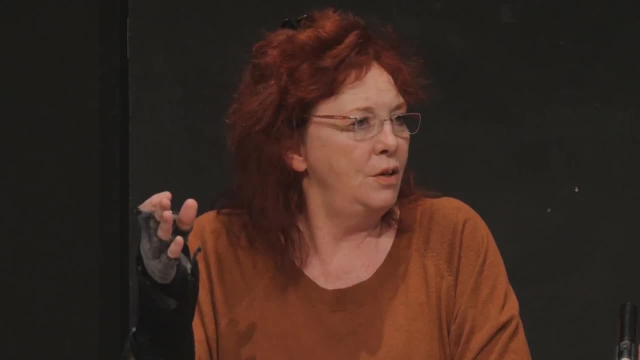 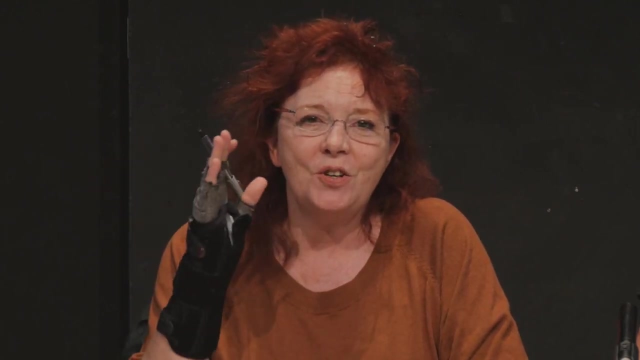 you can't do that yet. you can't do that yet. you have to do your. you know, finish your degree. you have to get a PhD before you can do your own thinking, And So it's not the teaching of philosophy. 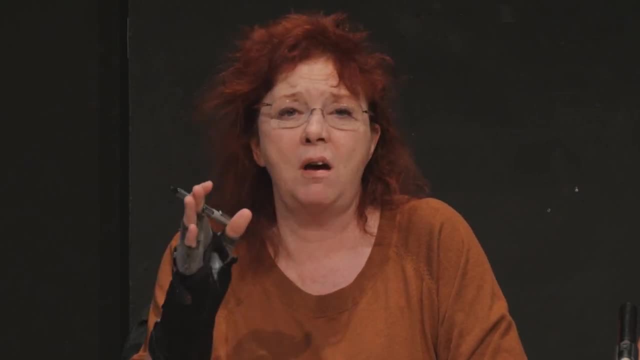 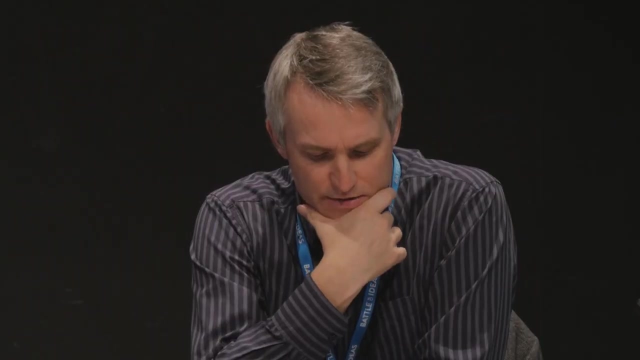 It's not the history of philosophy, It's philosophising, which is something else, I think. Pete, did you want to come in there? Yeah, I'm really confused as to why the gentleman who spoke last would say that that's a form of child abuse. 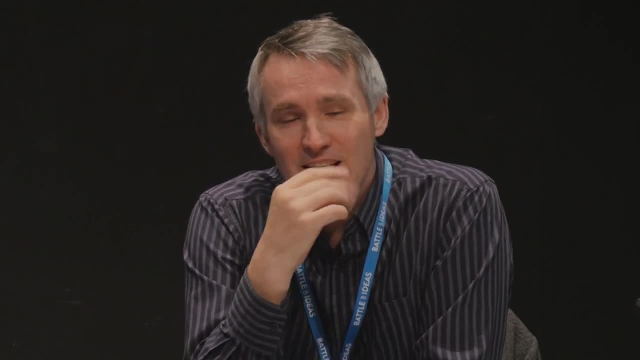 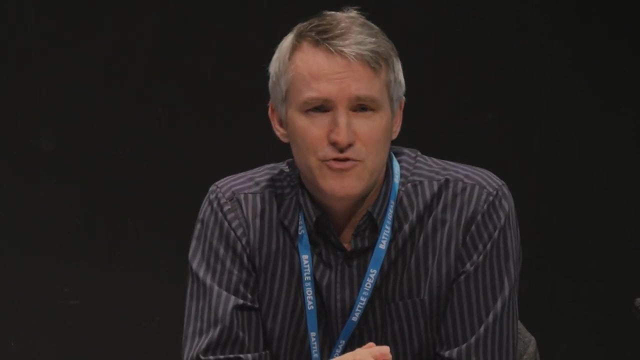 It's a strong thing to say, for one thing: Oh, I didn't hear that. Secondly, OK, right, We could do one of two things. I could go in and teach them Kant and the notion of Kantian a priori space. 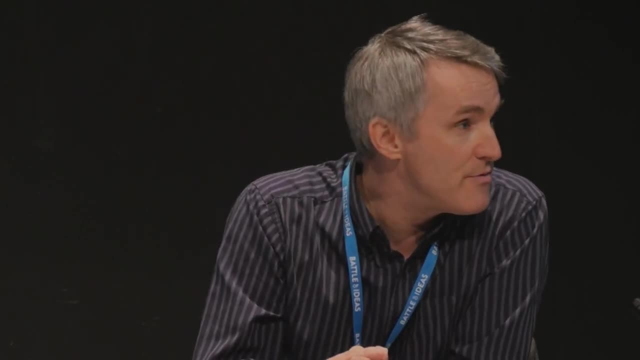 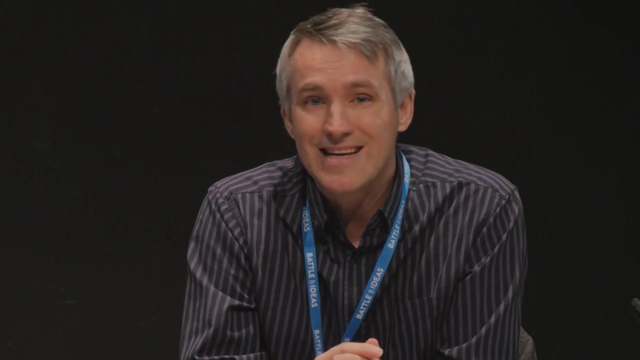 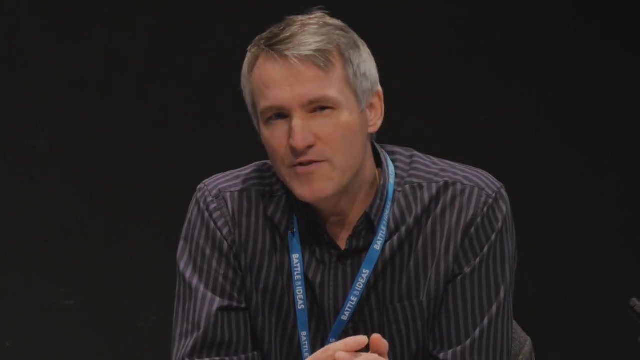 And then next week I can come along and test them, see how well they remembered it. Alternatively, I could give them the opportunity and the conditions to identify it for themselves, to actually come across these concepts for themselves, And if they're five, six years old, 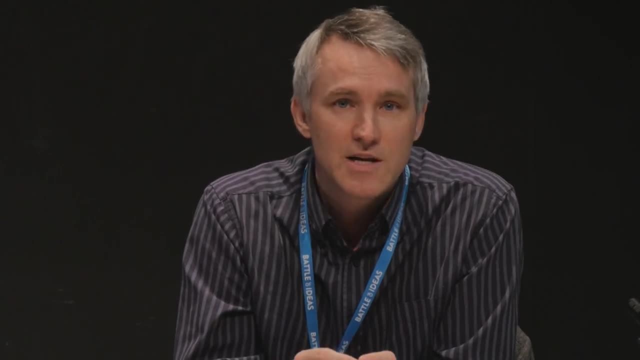 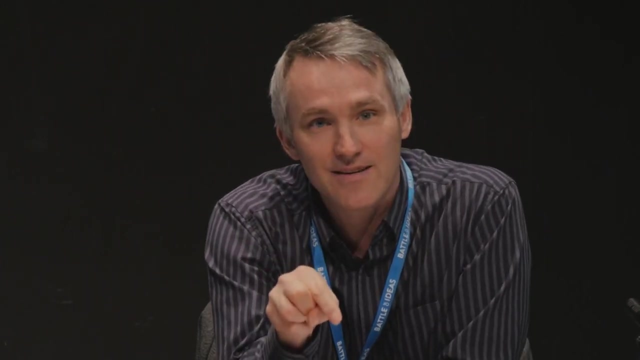 I'm pretty impressed if they start to come up with those, to outline those kinds of ideas, And actually that might be a really good time to start telling them about Kant. yeah, That's the time to do it. So now there's a distinction between subjects. 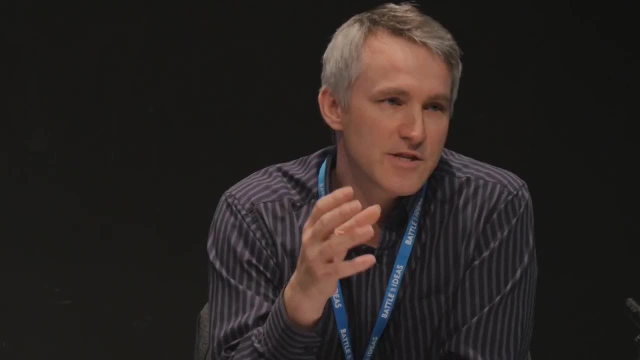 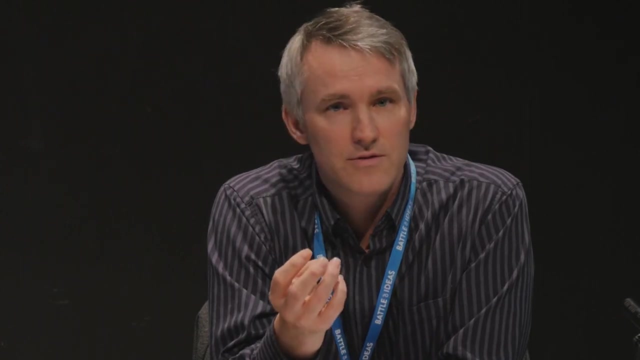 and process. Philosophy is two things. There's a subject and a process. As a subject, it's relatively new. I think it's Kant was probably the first professional philosopher, So it's not that old. So, being tested on what we know about philosophy, 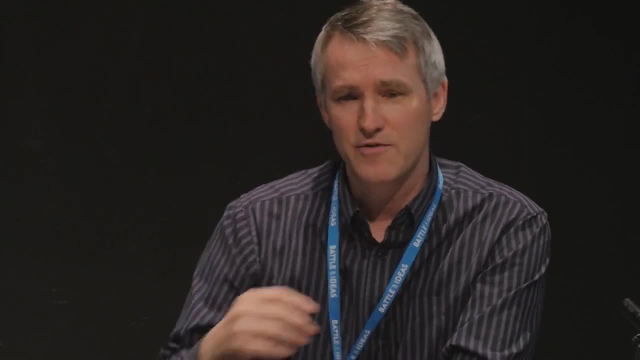 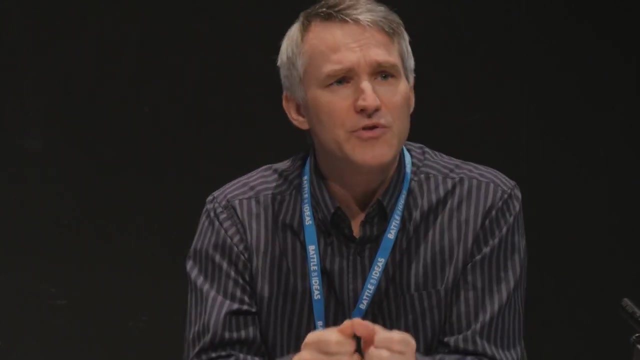 hasn't been going on that long. However, the process of philosophising is old, So let's take Plato as an example. right Plato, We could be reading Plato to them and introducing them to Plato and getting them to learn Plato and regurgitate Plato. 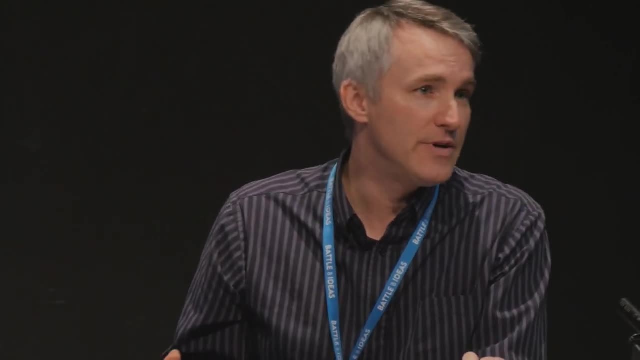 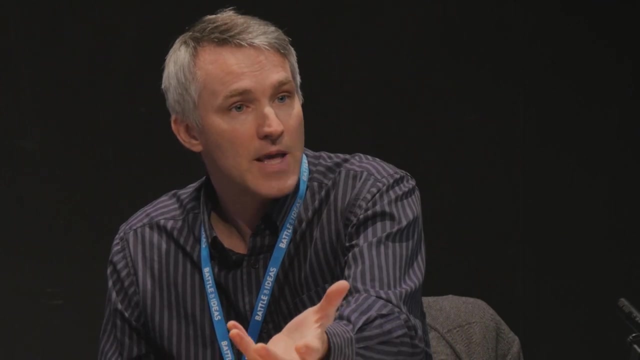 or even critique Plato, Or we could be doing them and getting the children doing what Plato is in fact showing us what to do. Dialogue In Plato's dialogues. he's not wanting us to just learn his stuff and regurgitate it like they did for a thousand years. 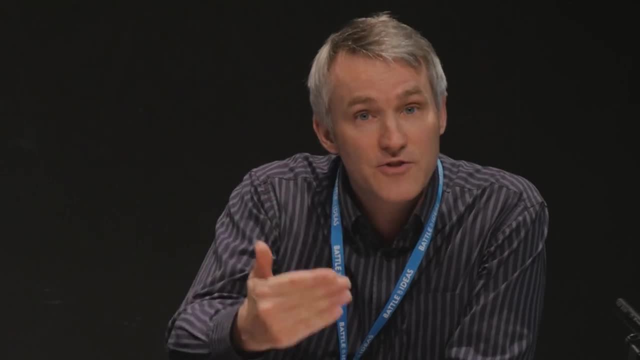 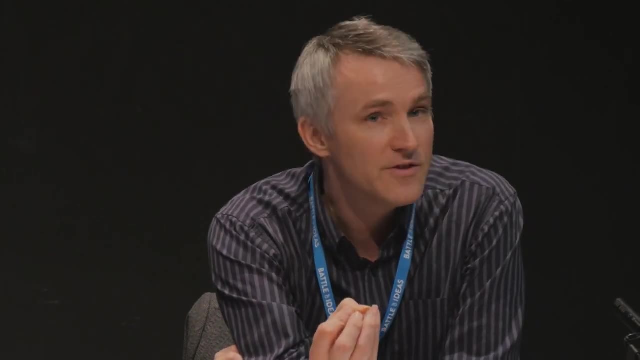 He wants us to read this and start to do what he's modelling for us. That's one of the reasons I believe that Plato's dialogues are largely aporetic. In other words, Plato doesn't reach conclusions very often, And the conclusions that we ascribe to him 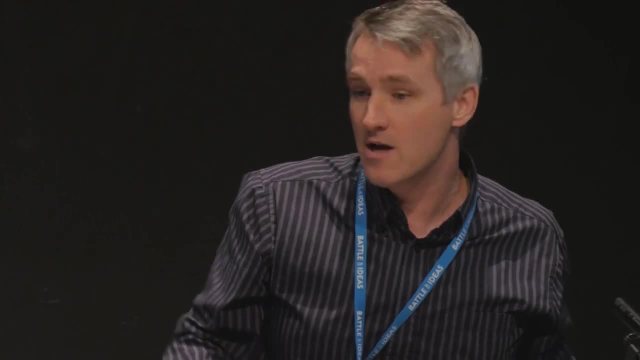 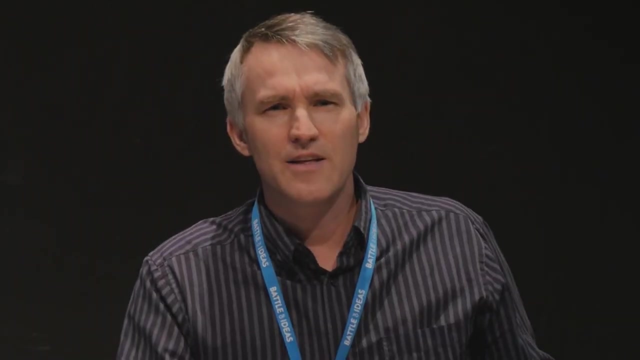 are usually false ones. Plato thinks that Plato says this because it says so in the Republic. Well, in the Parmenides he completely tears down his theory of forms. that's outlined in the Republic in the photo. So I would much rather be learning. 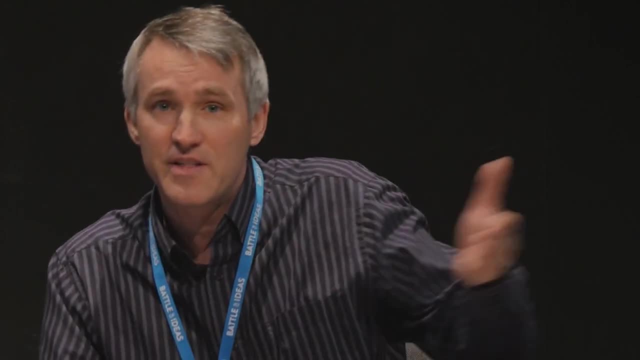 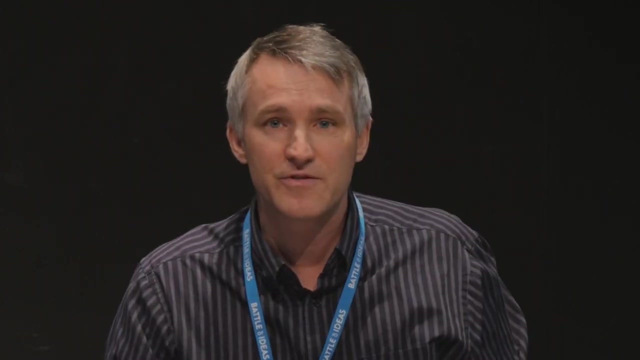 to do what Plato is showing us to do, and I think that's what we do through philosophising. That's what the doughnut enables the children to do, much better than just testing them on a bunch of how well they can regurgitate stuff. 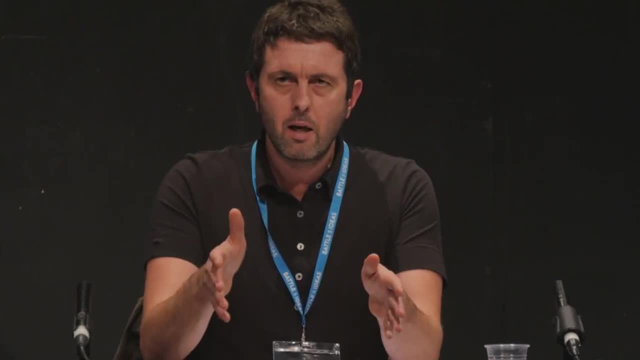 Excellent. I think we've identified our prey, We've finally got to it, which is: are we talking about philosophy as a subject or a process? I think that's framed it for me. I'm not saying, I haven't decided myself. 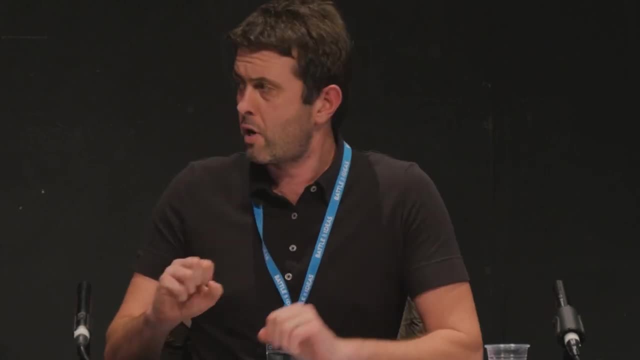 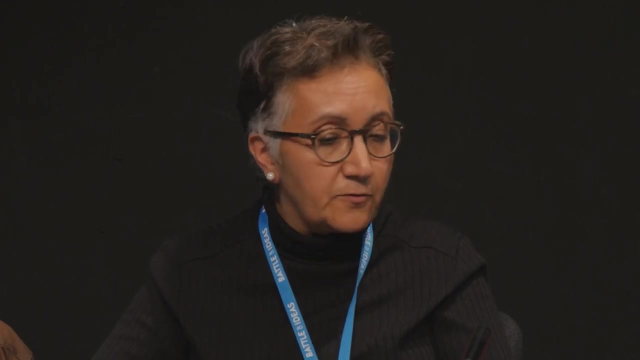 Alka, A subject or a process, I mean, I would agree with the. for me meaningful philosophy is. it's not about being tested on, you know, the life of Kant, or the fault of Kant, or Plato or whatever. However, 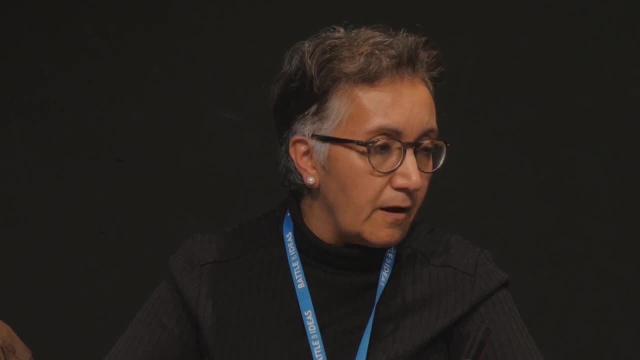 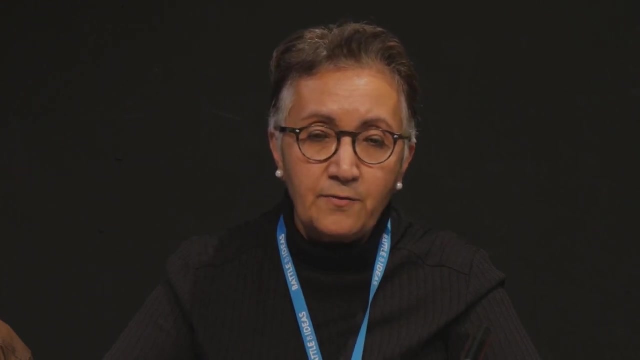 I do think that it's an adaptation of the philosophy of Plato and the philosophy of Plato and the philosophy of Plato and the philosophy of Kant. It's an adult thing. It's as simple as that. I think you're really missing a very important fact. 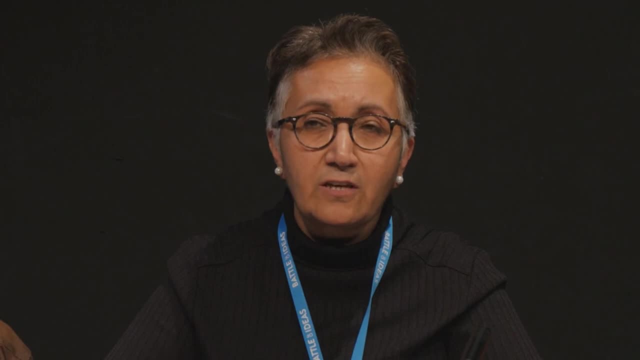 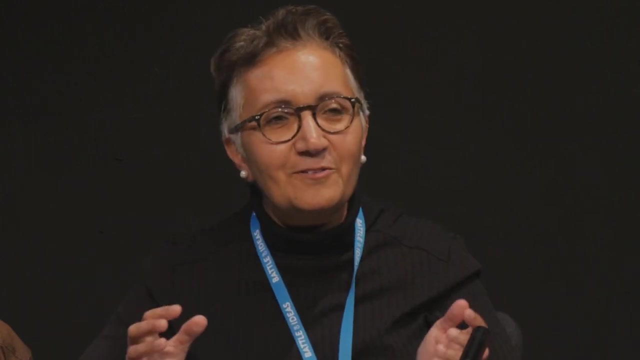 that Plato and Kant and other philosophers understood, which is education. It's, if you like- I've come across this word and I love it- propodutic, Propodutic. It's that idea you're into, you're. 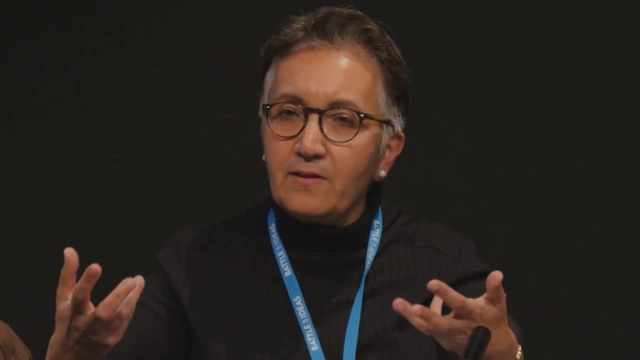 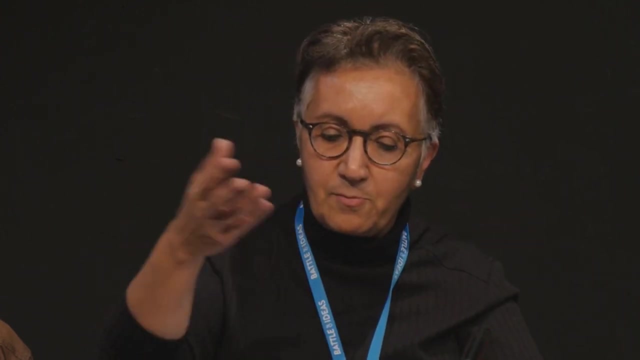 it's an introduction to something, a preparation for something that they then equips them to go on and do in later life. So I've got no objections to it, but I wouldn't want it to be tested because there's too much testing anyway. 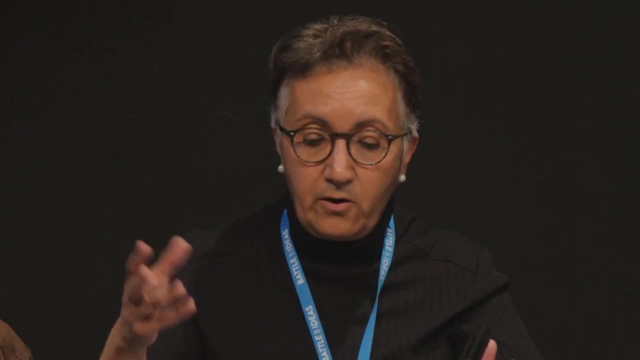 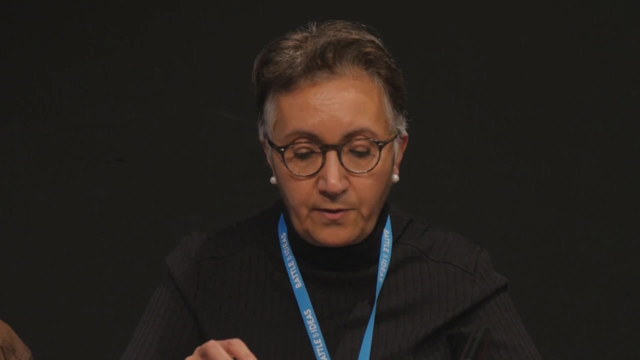 and I'd love them. you know an idea of you know learning about the philosophers and some of their key ideas, But the philosophising I think is an adult thing, for the reasons I said at the beginning to do with. 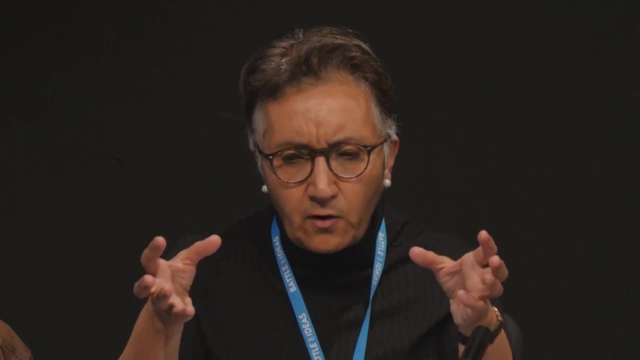 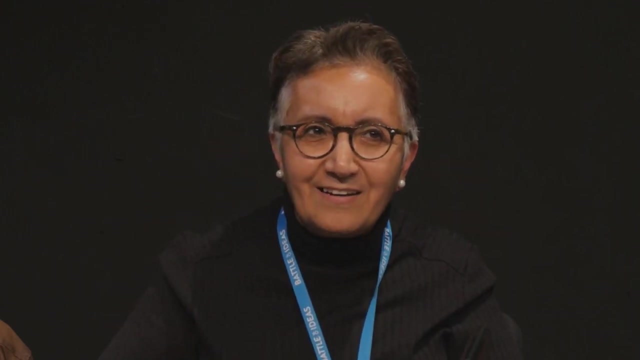 it's and it's to do with. I think there's a real, not just a fear of knowledge, but a real kind of forget, an amnesia about actually what knowledge is. But it's, it's not just facts. 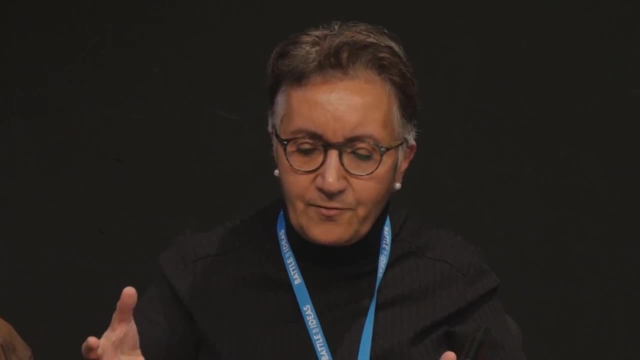 It's these, the forms of knowledge that we have, which I think is about not through education, but through what I've done in philosophy many years later, through looking at things to do with epistemology. They are formal concepts. 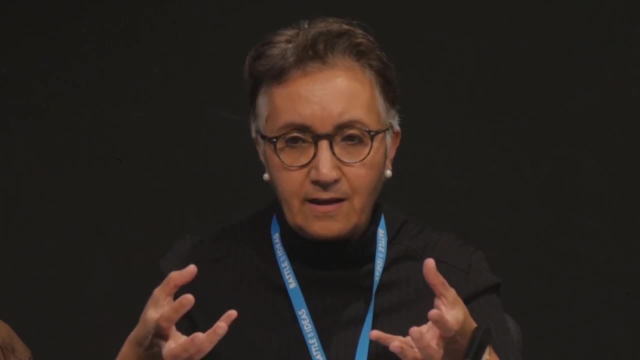 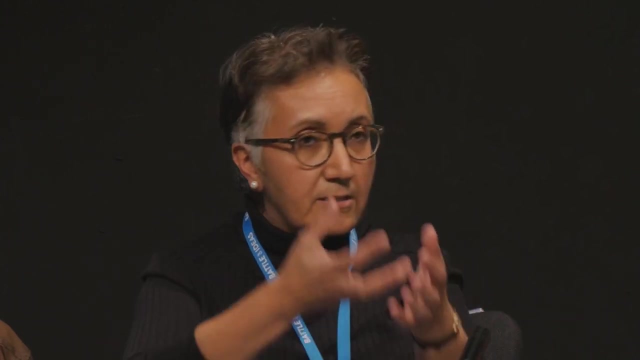 with a formal language that are related systematically And, although they're formalised and abstract, they come from our experiential world. Yeah, they're rooted in that, but they're they're, they're formed and shaped to in a way that they lose. 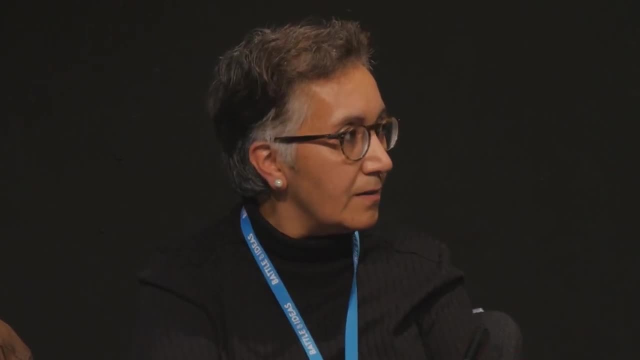 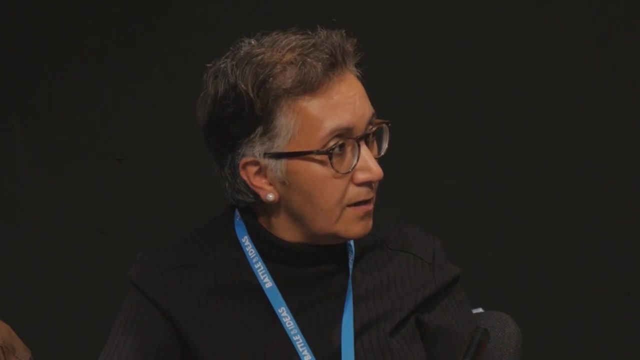 if you like, the trappings of the empirical and become more conceptual And those and you need those two bases to to have a proper critique Critical thinking. people think critical thinking is just criticising things, but just criticising things within the term. 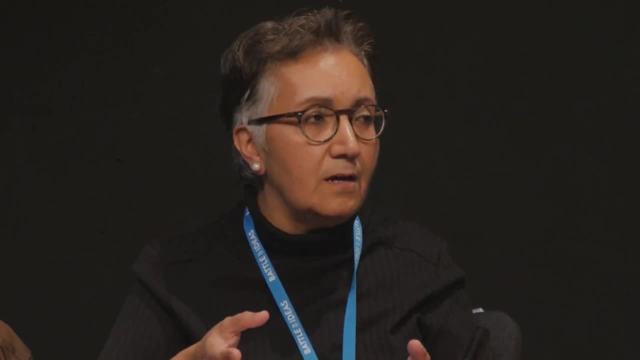 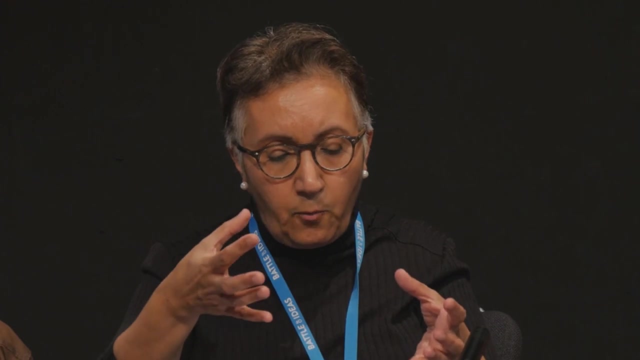 of the debate is not real critique. To have that real critique, you need two bases. Yeah, you need the empirical and that conceptual. And what my argument is that that is is is a very difficult and long process. That's why Plato said: 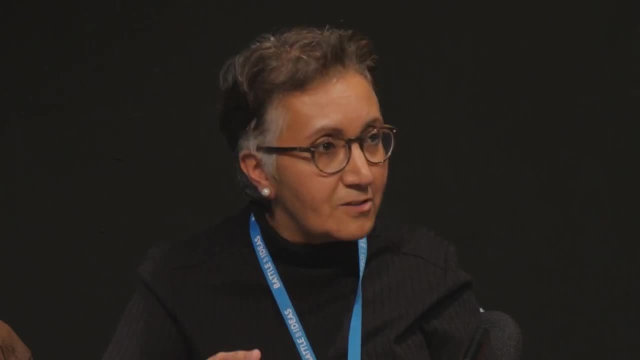 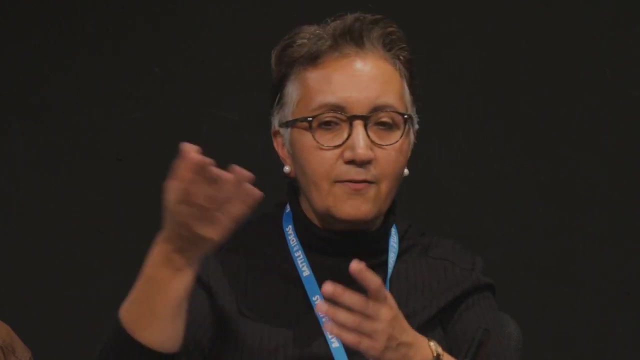 you can't do. you know dialectics was only done after you've had at least 20,, 24 years of learning that You need mathematics, astronomy and the other things, plus three years of military training where they didn't read any books. 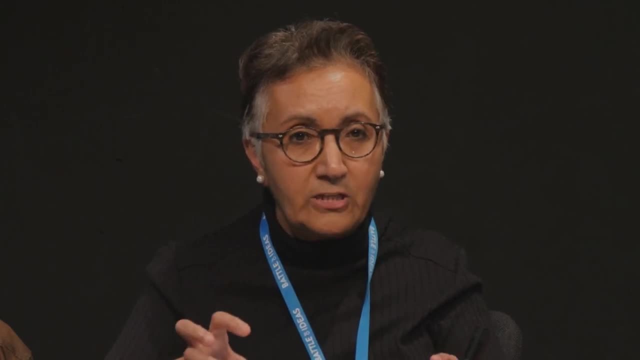 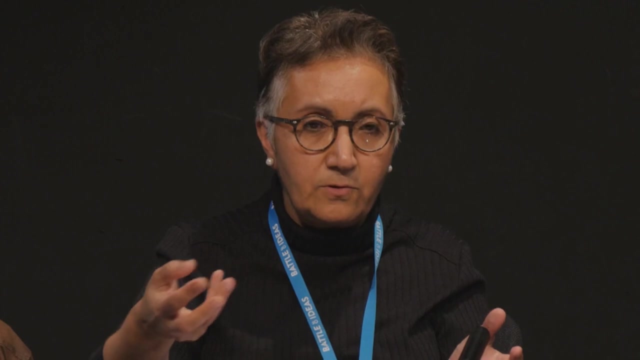 So they had. you know it was. it was on the basis of an awful lot of substantive knowledge. That knowledge, if you like, represents you know you gradually move through it to higher levels of complexity and abstraction, But it's a way. 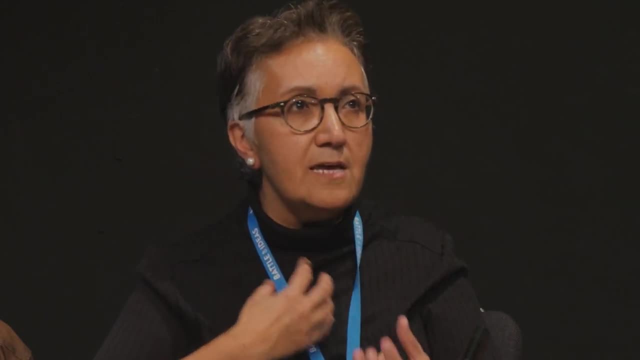 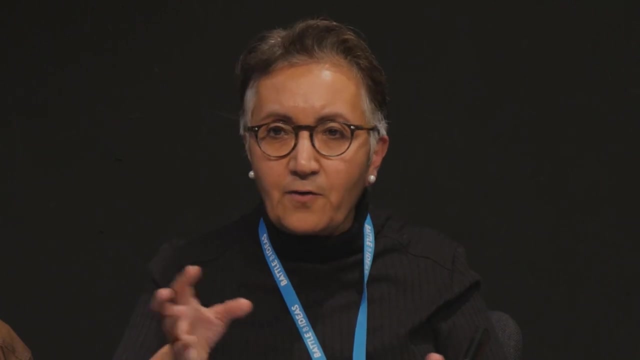 of understanding your experience in a in a distance way. It allows you to take an objective position and I'm sorry, but the most delightful insight that a five or six year old can offer on a donut or an umbrella or anything is not. 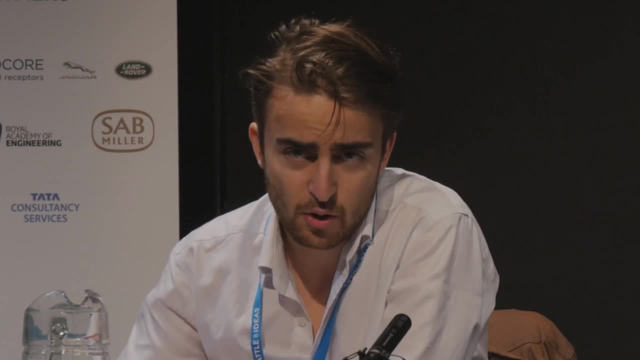 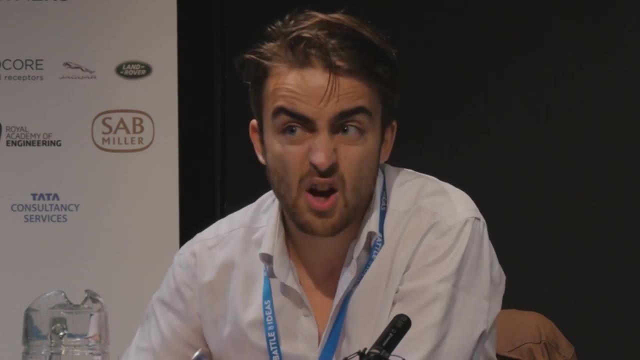 is just not the same thing. Okay, thank you, Adam. did you want to say anything? Maybe? I think we should be slightly wary of creating a false dichotomy between, on the one hand, questioning and being sceptical and, on the other hand, 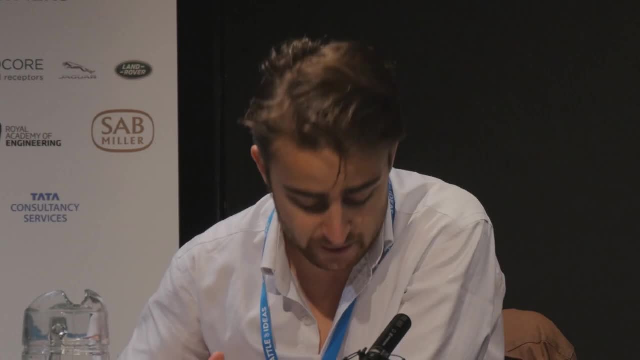 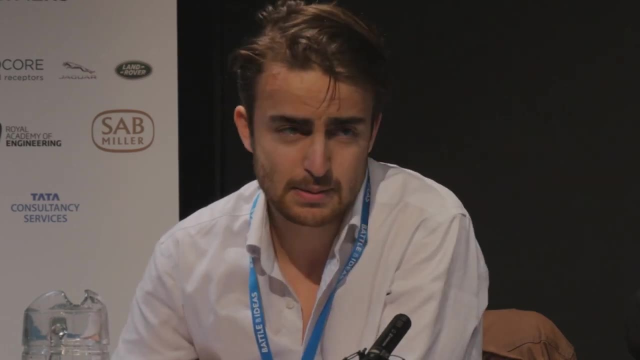 learning and knowledge. I'd actually argue that the very process of learning and understanding is a very complex process, In terms of the point that was made about- about the danger of where philosophy introduced in schools might take away from the philosophy of English or maths- 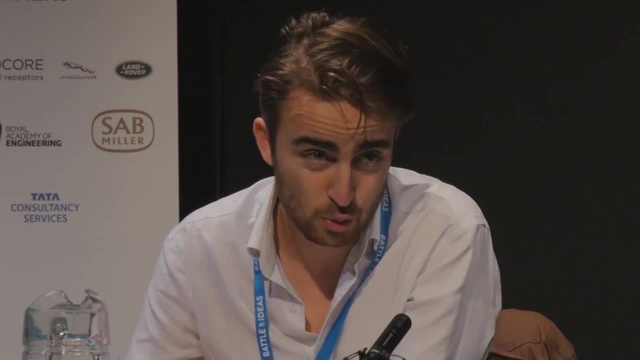 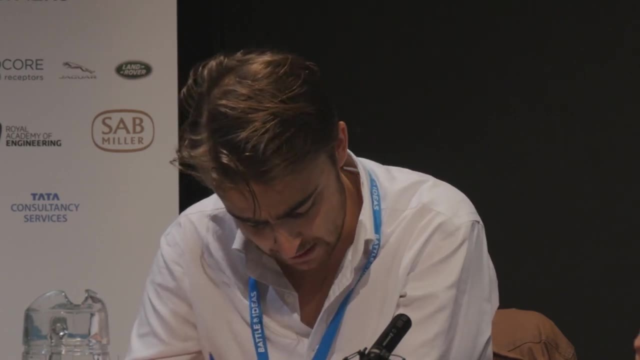 I think that's really true. A recent report by the Education Endowment Foundation found that doing philosophy in schools actually helps with results in philosophy- sorry, in English and maths. And then in terms of the point that was made about middle class children maybe having 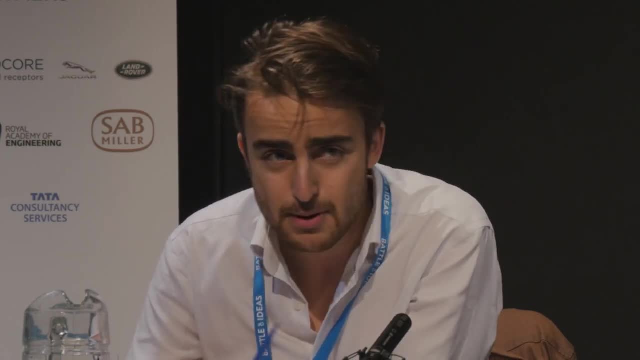 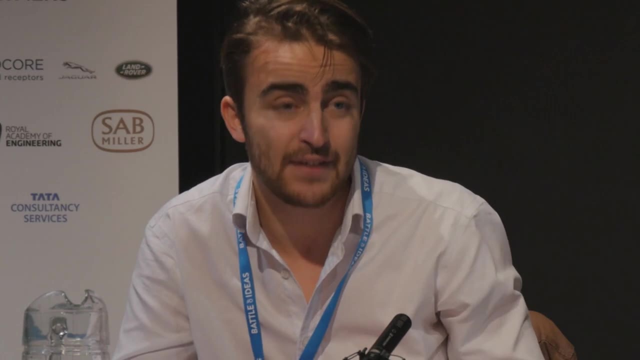 to deal with social justice perspective. often middle class children have these questions and they can discuss them at the with their- you know, with their families. but often that opportunity isn't available for socio-economically disadvantaged children. So, through doing things like philosophy, 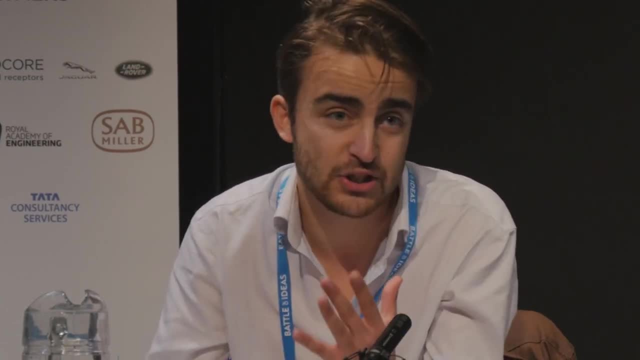 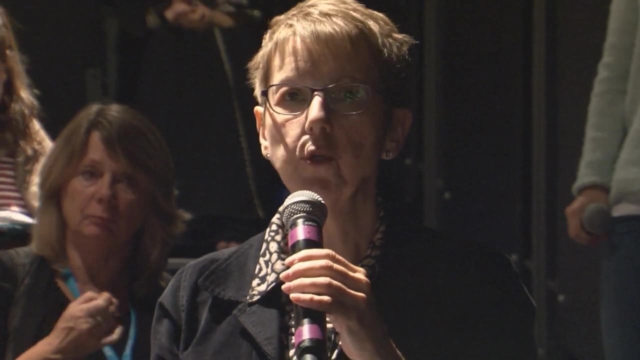 for children. it's a really fantastic forum for them to question, to ask the questions that they have. I agree with what you said, Alka, about the problem of knowledge having been hollowed out. The whole philosophy for children is part of a process. 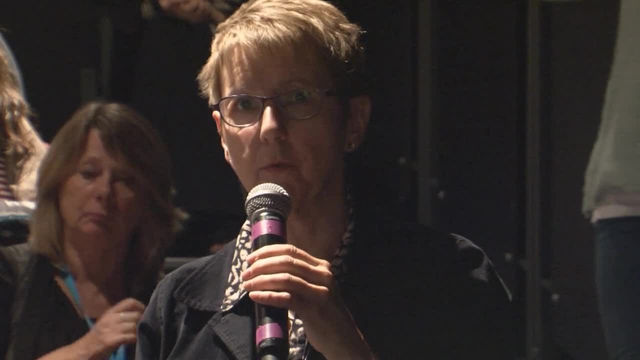 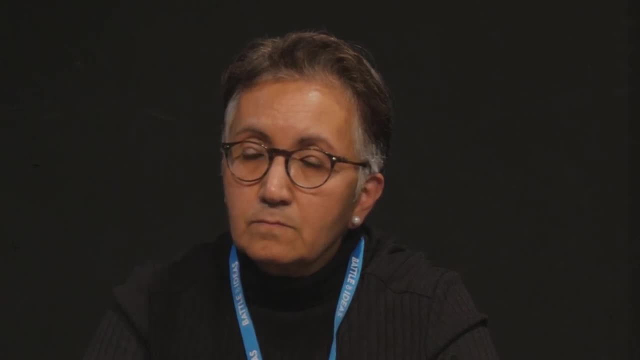 of the hollowing out of philosophy from the adult perspective, and is there a relationship between the two? Thank you very much. I'd just like to really quickly. I actually went to a school where philosophy was compulsory from the age of five, along with Sanskrit. 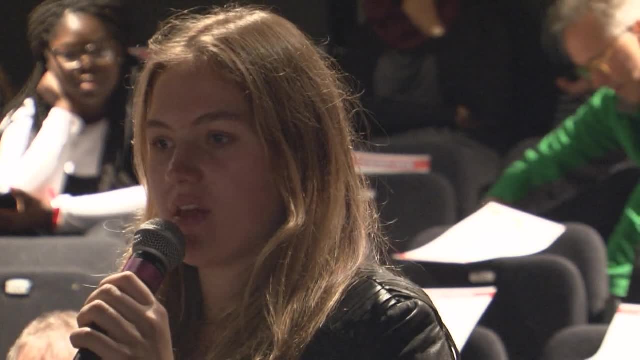 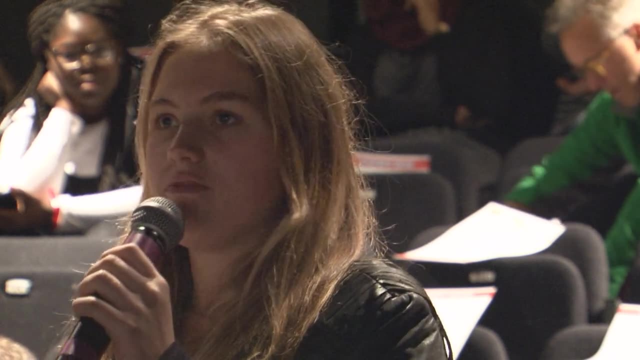 Philosophy until you're 18, even if you drop it for A2.. I think what you do realise is that philosophy is something that connects with some and not others in the literature. The people that already find that interesting and that's why they're here. 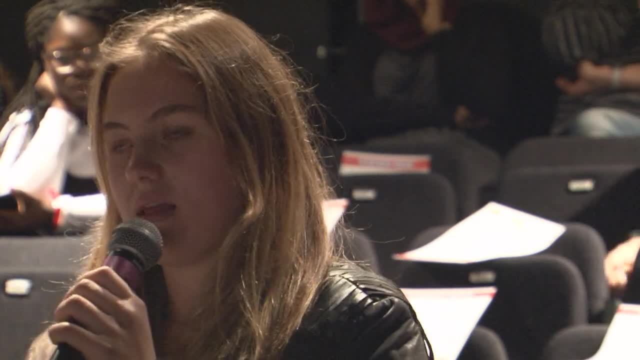 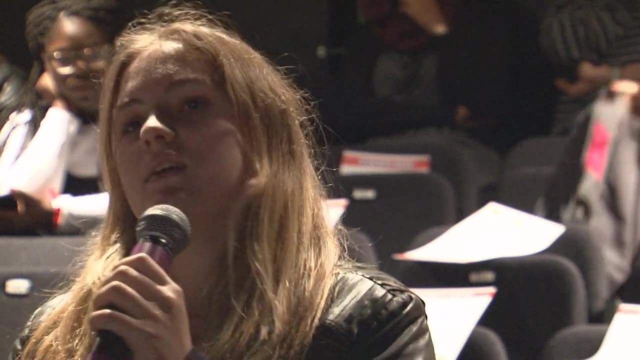 and I think philosophy's like that: you either connect with it or you don't. but I think it's something that, therefore, I came here. I've changed my opinion. I don't think philosophy can be taught, and I think, how your gentleman at the end said, 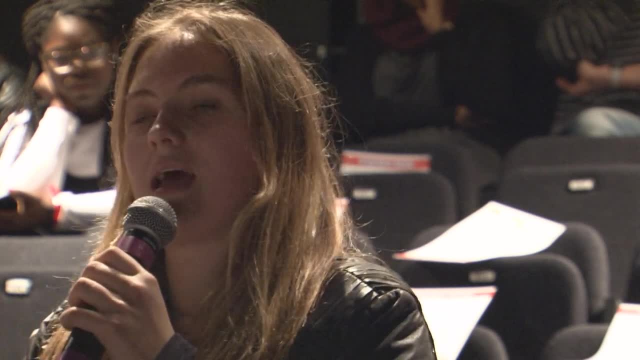 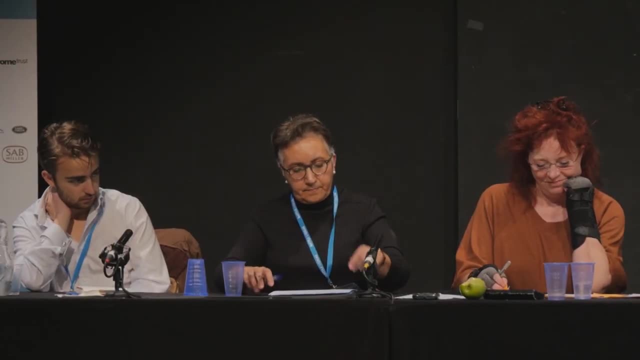 I think that you're choosing the creme de la creme of children from disadvantaged backgrounds who already think like that, who are already very academic, and I think you either think like that or you don't. Okay, so our speaker's in reverse order. 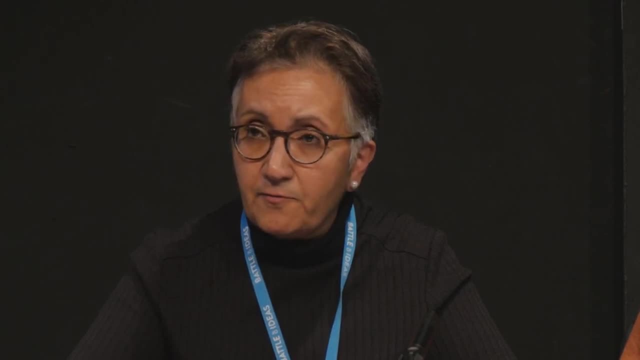 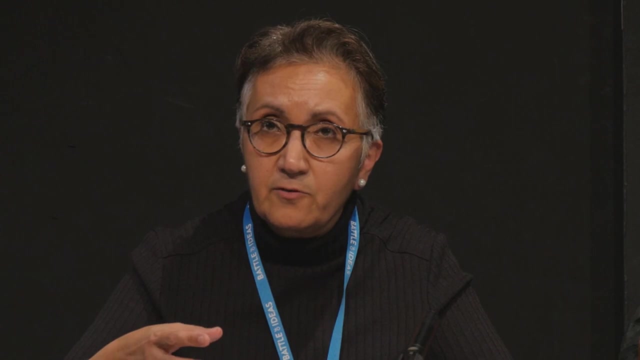 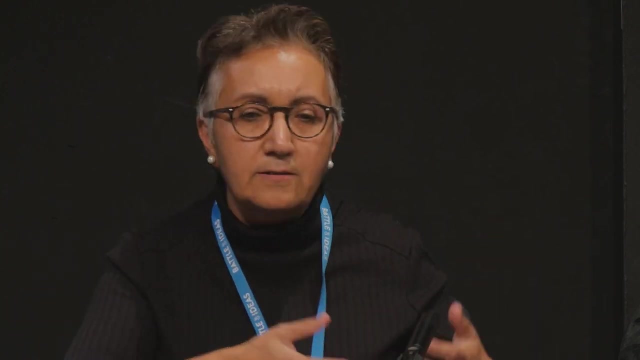 Alka? I think probably. yes, it certainly reflects. philosophy isn't immune from that. I recently read in a very esteemed philosophical journal an argument for philosophy and ethics and character and why it should be taught in schools. and when I looked and they were saying, going back to the Greeks, 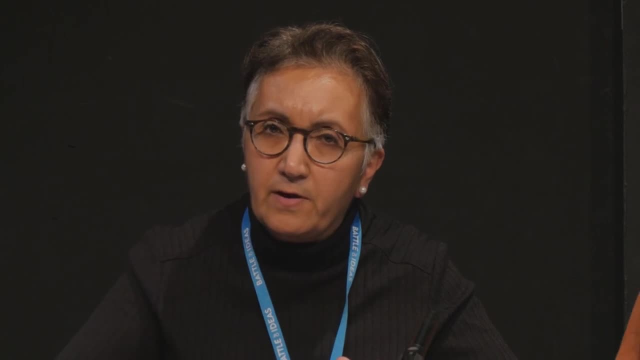 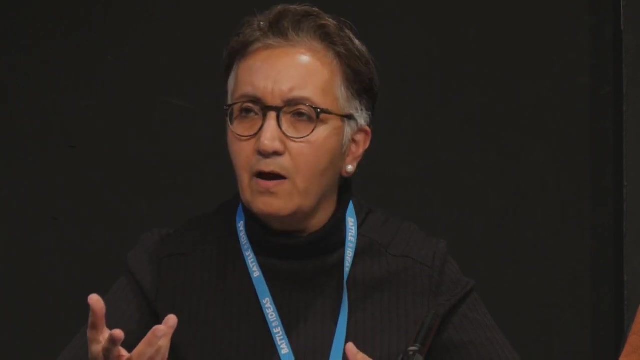 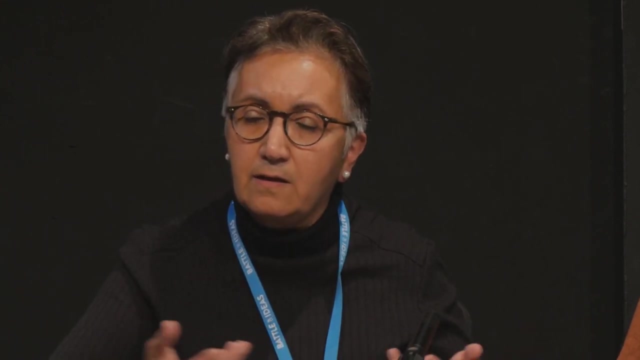 and classical things. I looked at the literature review, his bibliography. there was nothing earlier than 1988 on it. So this man was writing and advocating, you know, a whole set of policies and strategies based on theories going back, claimed to go back to the Greeks, and yet there was. 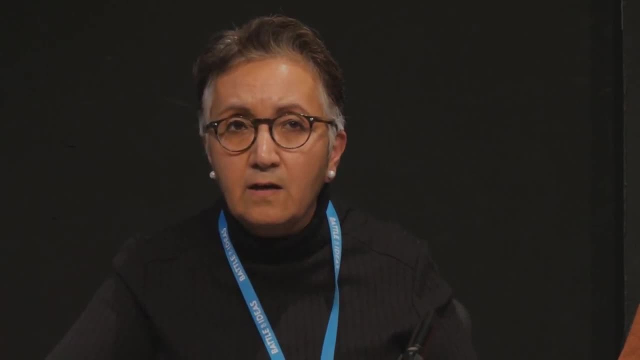 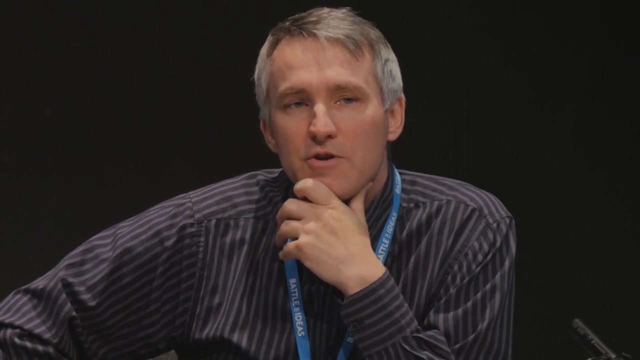 you know, Foucault 1988 was the earliest thing that he'd read. That is a real problem. I'll stop there as we're short for time. Thank you very much. The worry about the curriculum and the separation of philosophy from the curriculum. 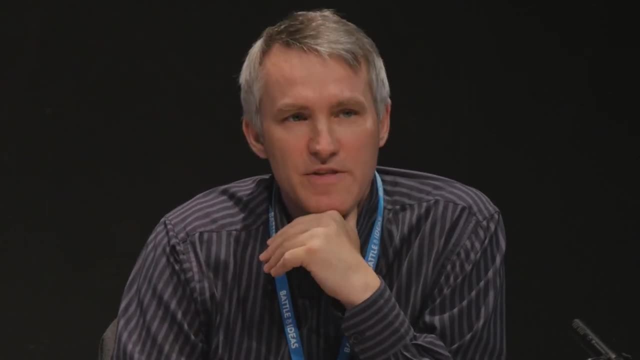 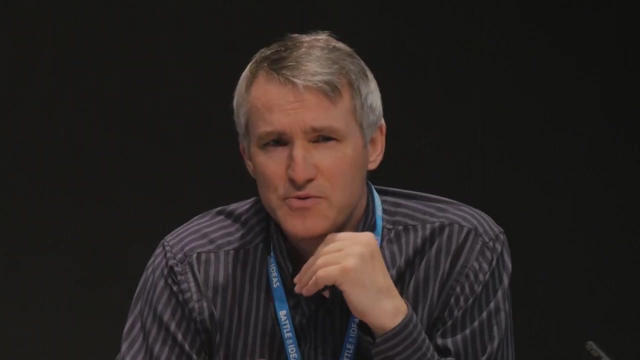 and stuff. I think that's a legitimate one and, for instance- you know, you may be aware of this buzzword at the moment- the idea of trivium. there's three parts to education. there's the grammar, the dialectic and the rhetorical part, and I think what's 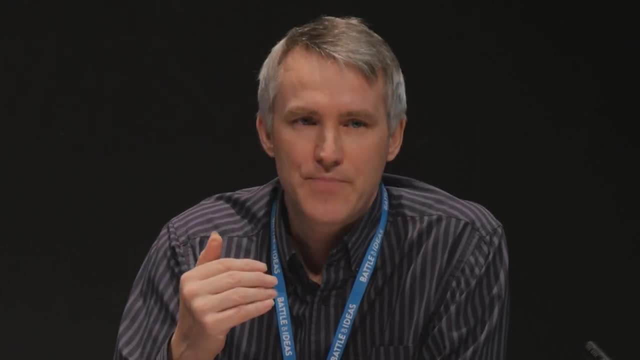 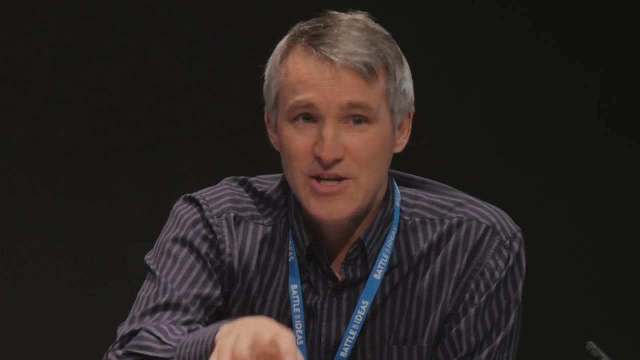 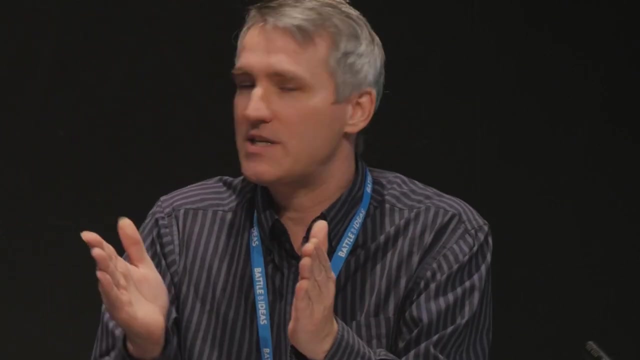 really important is that we must try to bring the philosophy in line with the curriculum. in other words, it's the dialectical part of education, especially if we understand it as a process or activity rather than just a subject. so the process of philosophizing enables us to have the dialectical 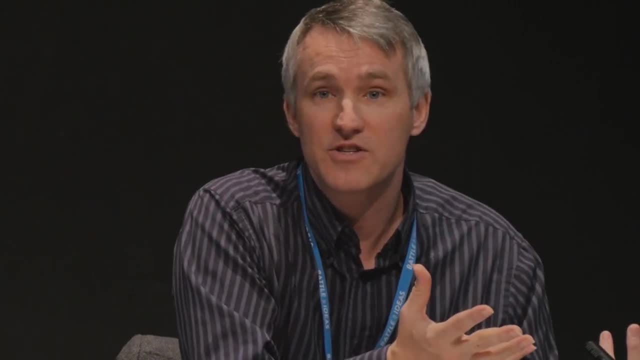 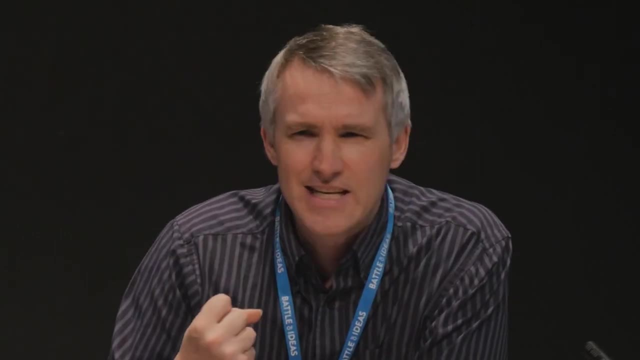 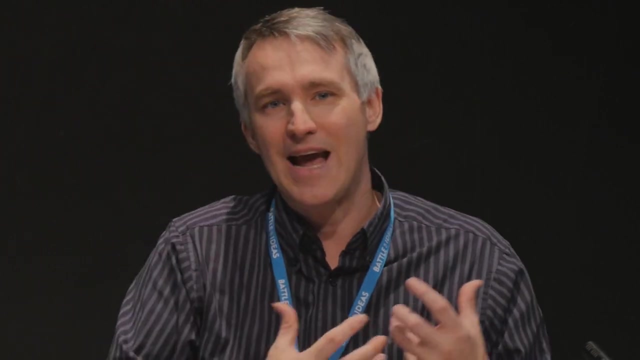 attitude towards the knowledge stuff. trivium is known as grammar, towards the grammar stuff, so that we are learning the knowledge and, at the same time, questioning it, testing its weaknesses, so that when we come to create our own thoughts on it- which is the rhetorical aspect- we're in a better place. 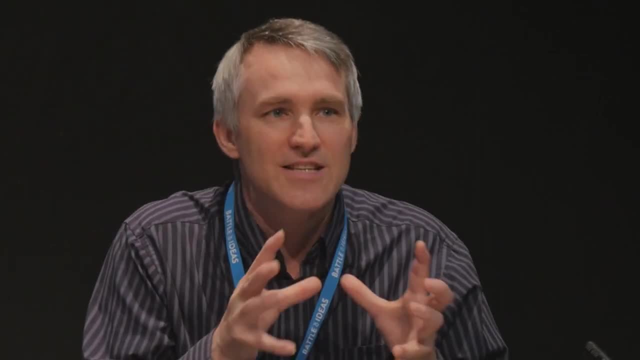 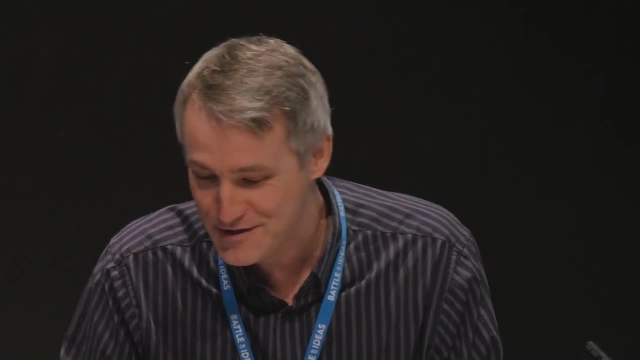 because we haven't just, we're not just regurgitating- we've already to some extent tested our knowledge base. so the integration of philosophy with the curriculum. it just so happens that my book's title is philosophical thought adventures across the curriculum, so I think it's a good 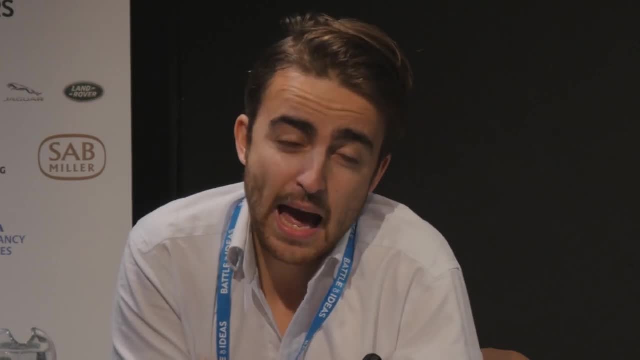 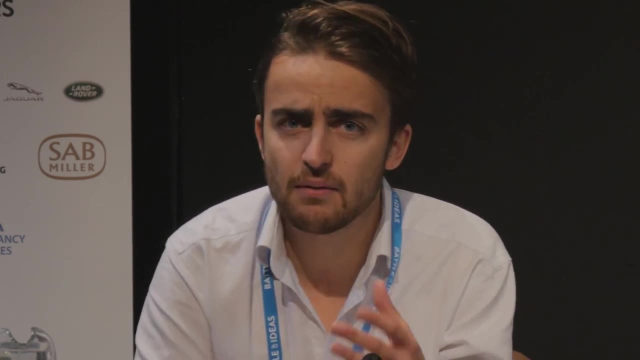 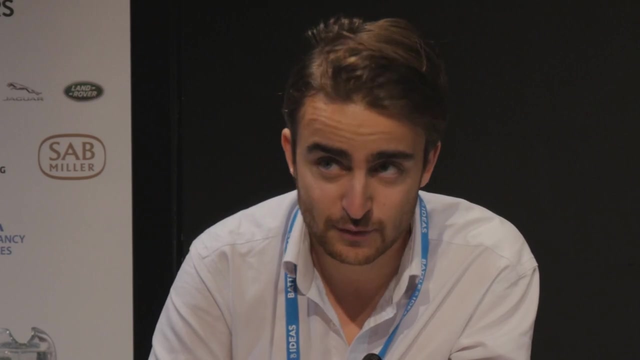 example of all reputable booksellers. Adam, as my final point, maybe considering where in the debate the question of child cruelty lay, because that point was made as an argument against teaching philosophy to children, I say actually, what would be cool would be to say to a child that you can't. 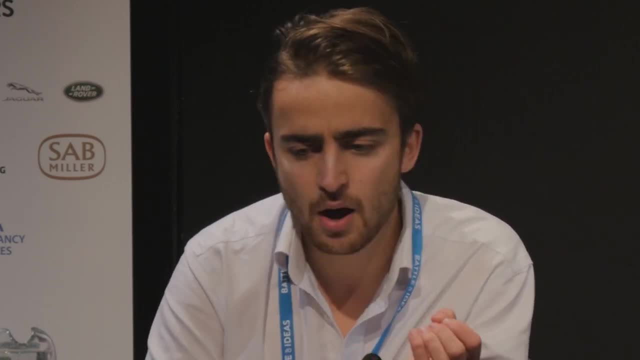 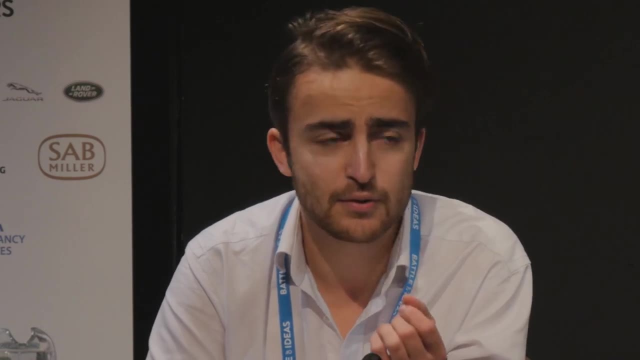 do philosophy, you can't explore those questions, you can't think critically about the world than you currently are. and so I think- yeah, I think it would be a massive shame if we said to children: you can't do philosophy. okay, Catherine, okay, I'm perfectly happy if educators 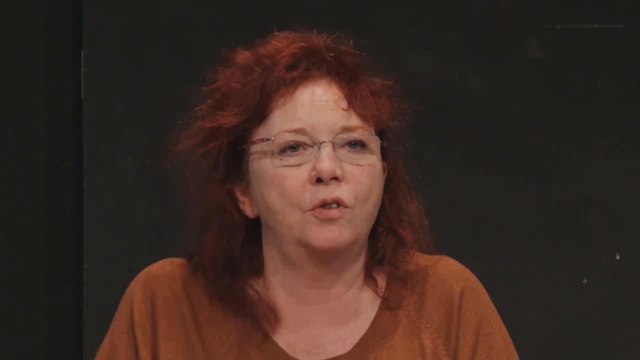 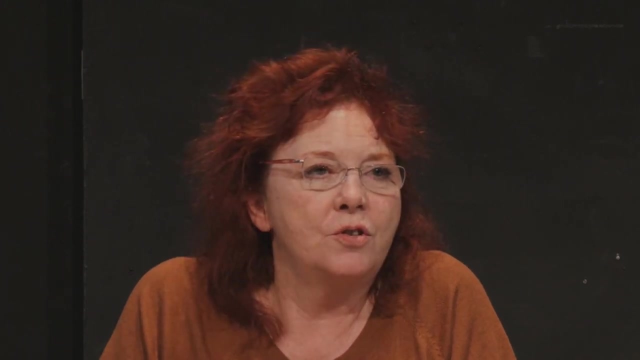 schools and teachers decide that school is not the place to do philosophy for children. that's your choice as educators. if you think that it should, school should concentrate on something else, that's fine. I would just advocate philosophising as an activity in a reasoned way, in a reasoned, structured way.